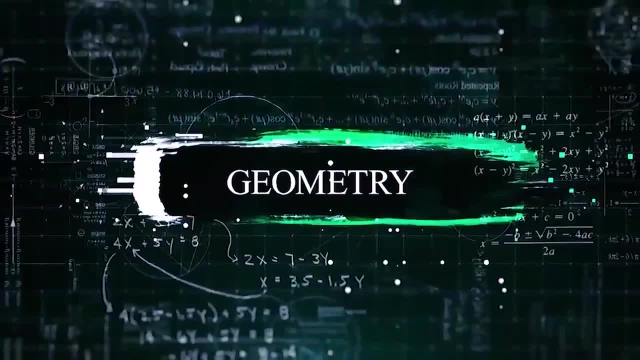 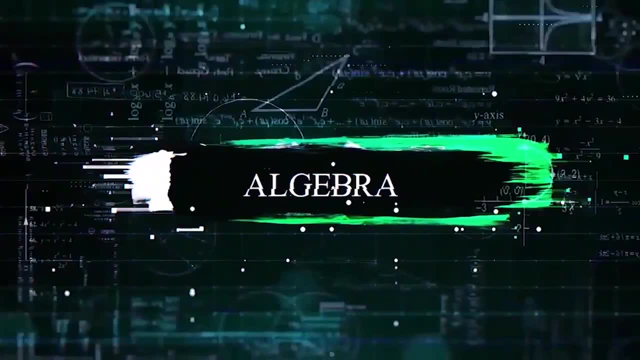 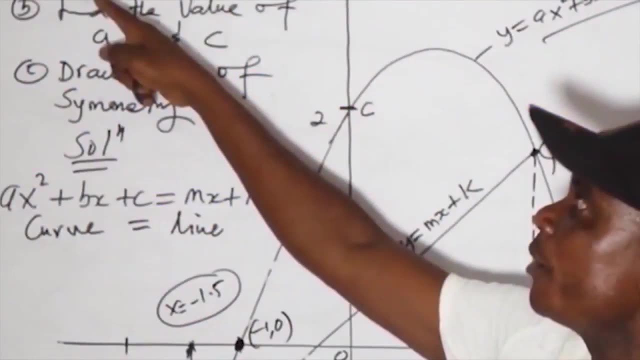 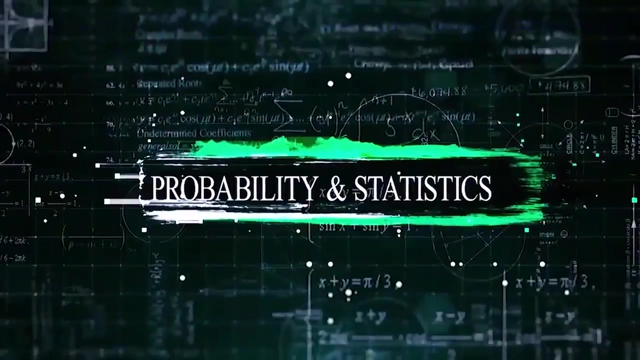 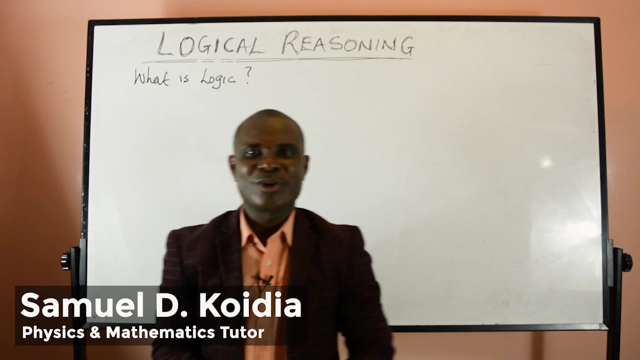 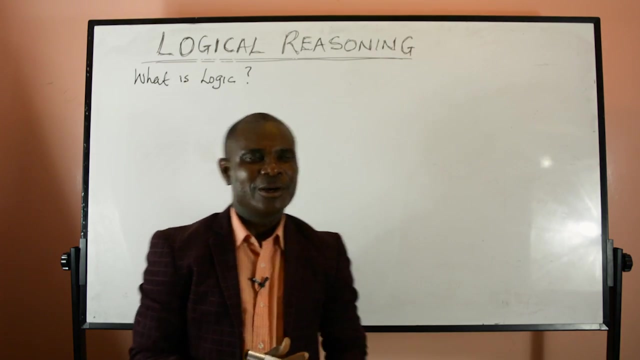 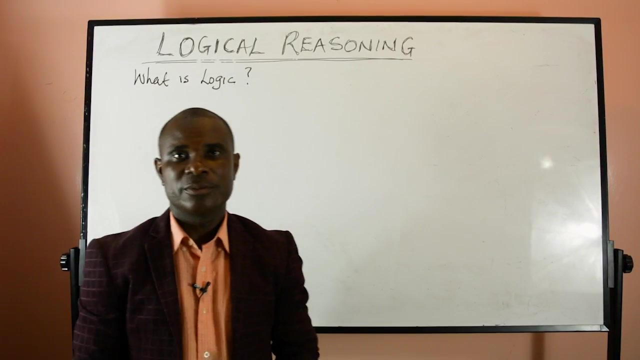 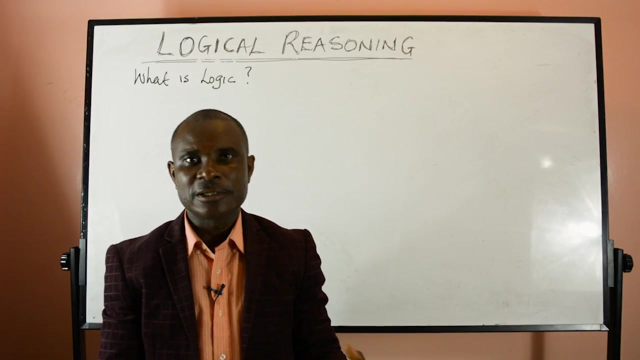 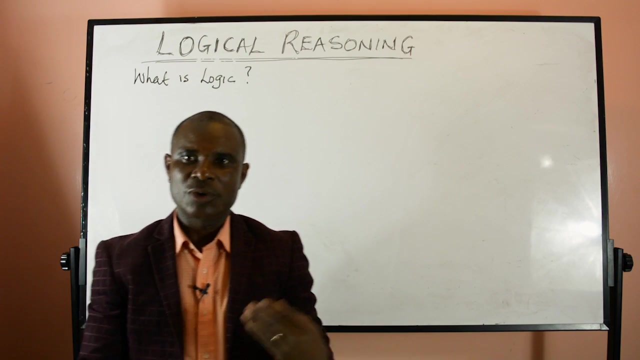 Thank you for watching. All right guys, welcome back to this math tutorial Today. we go along with math and our topic of discussion today is going to be logic and reasoning. And it's a very interesting topic because scientists believe that you have to work with data to collect information. We know that data is a piece of information gathered And if you collect this information, you have to hypothesize And in the process of hypothesizing, you now draw conclusions. 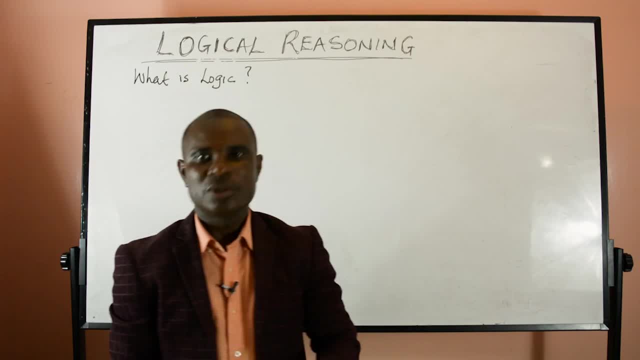 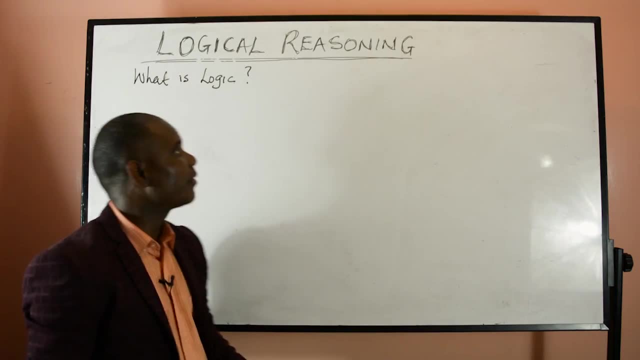 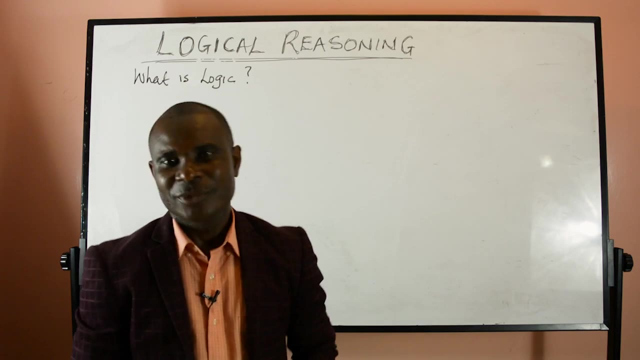 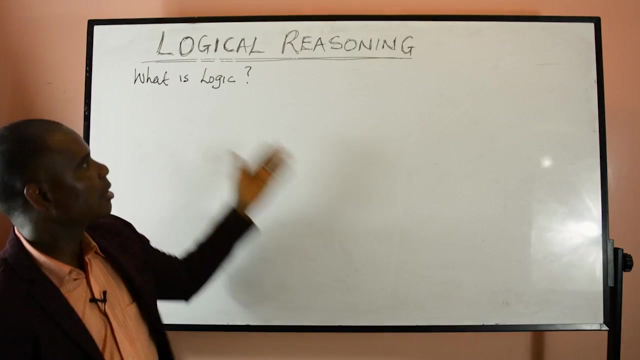 And when you draw a conclusion, then you base a conclusion. You are going to base your conclusion based upon what you've seen. So this is a very relevant topic in math and even in science. So we want to look at logic. So what's the big question? My name is Samuel D Quaidia. Now I want to first start by defining the word logic. What is logic? Logic is actually the science of thinking correctly. 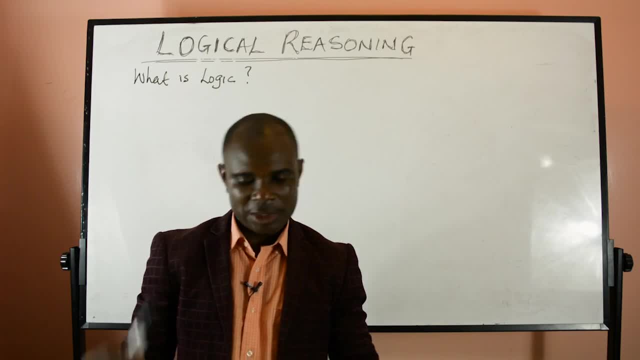 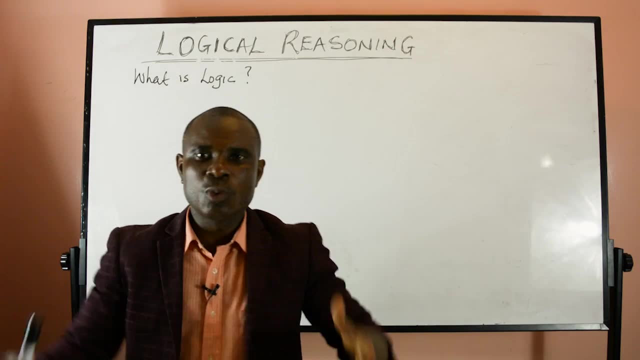 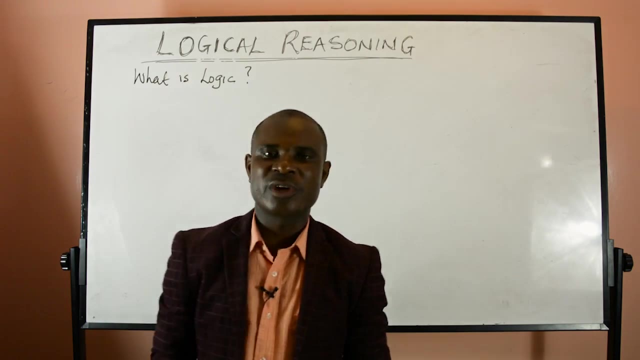 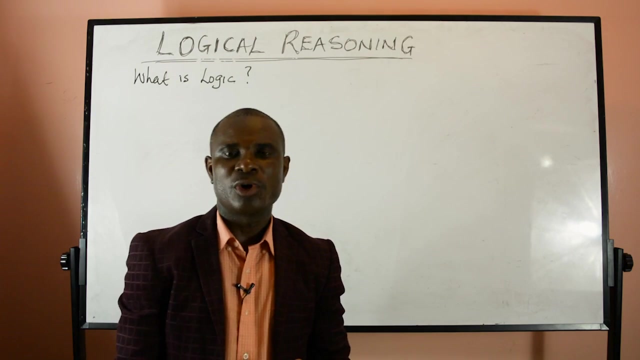 You know, it is the building block of argument And because, if you think correctly, that is how you'll be able to develop your argument And somebody will say, yes, you have a reason. power, And this word around us now is explained based upon rationalism. You must explain things based upon reasons. That is the moral reason why this topic is very important around our background. So let's look at it. What is logic? We say logic is the building block of argument and it's also the science of reason and thinking correctly, if you like. 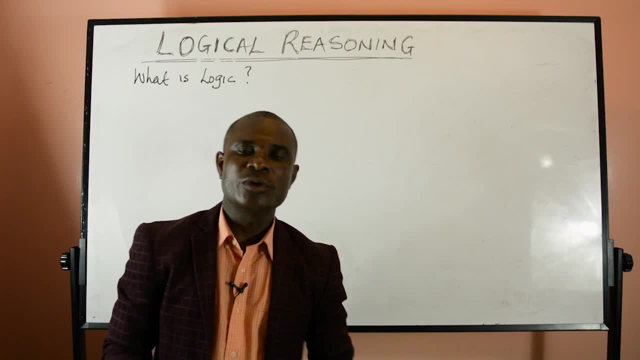 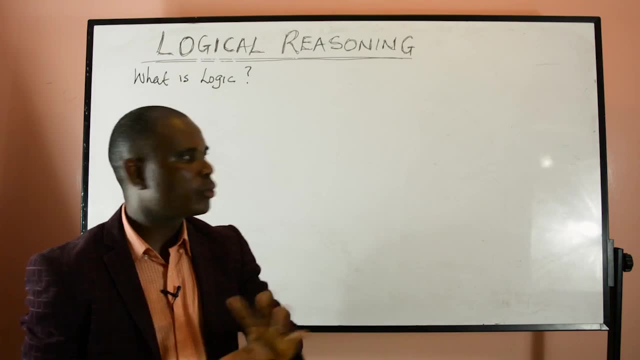 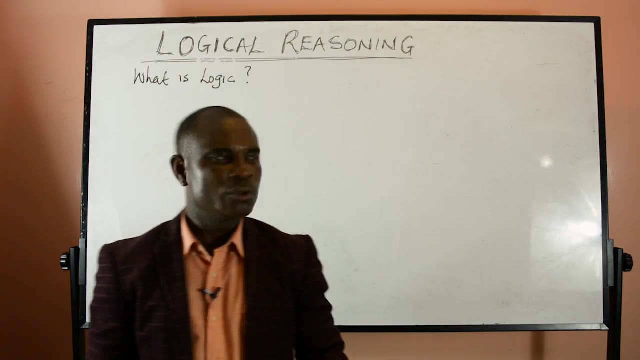 So what is the key thing here? If we want to talk about logic, we have to talk about statement, And I can categorize it first of all in two broad topics. This first video is going to just give you one part of this discussion on logic, And the next video, as you subscribe, you follow up as you move to the next definition of most, the next dimension of logic. 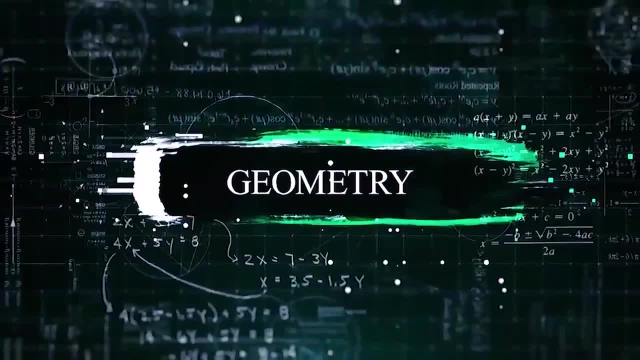 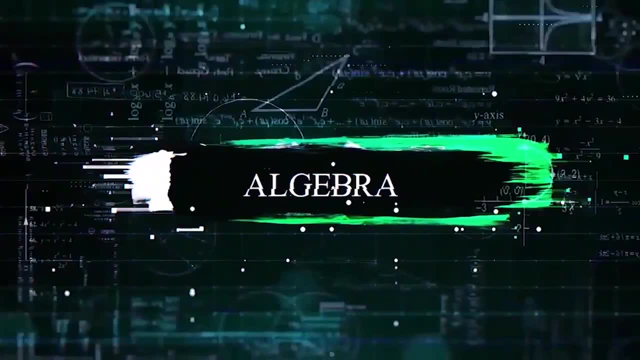 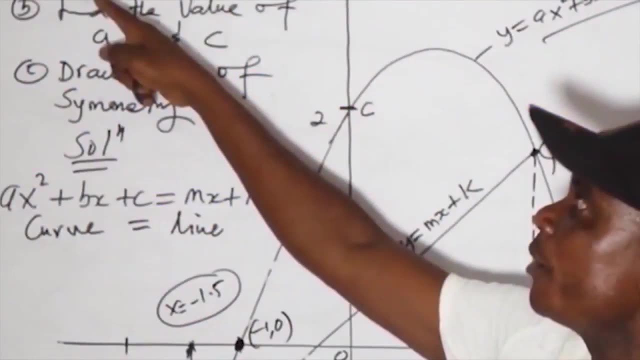 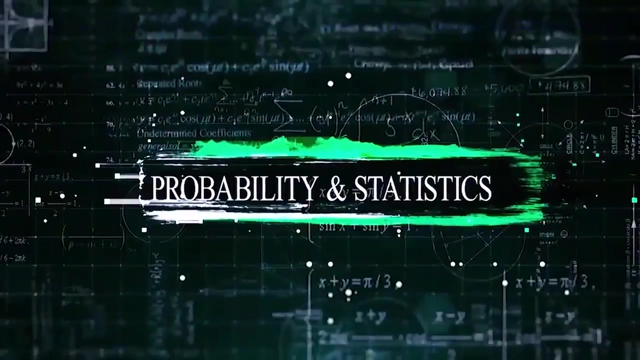 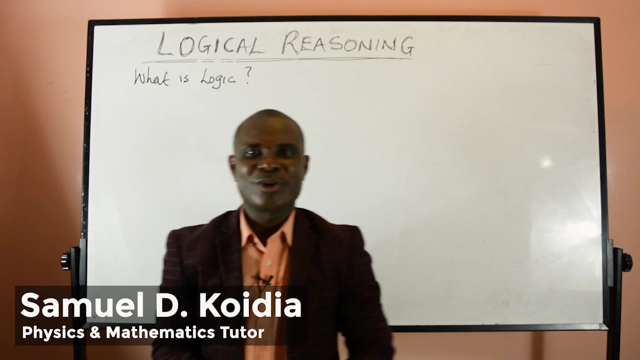 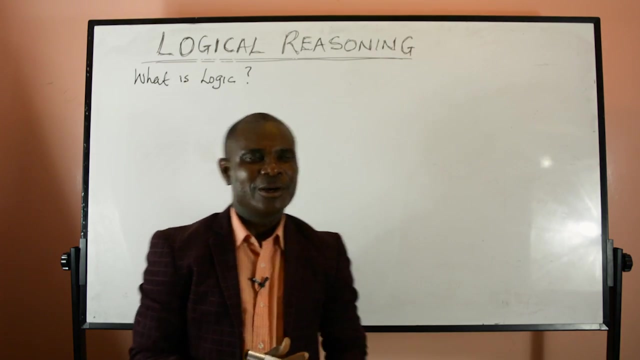 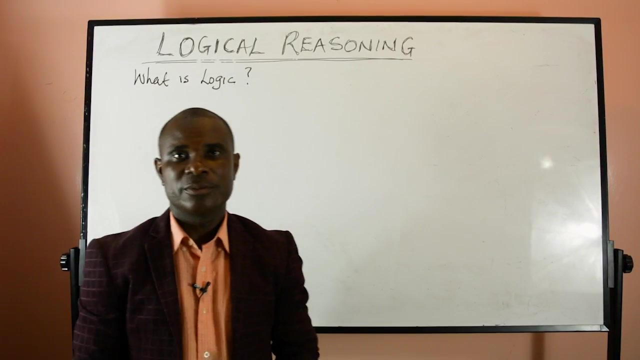 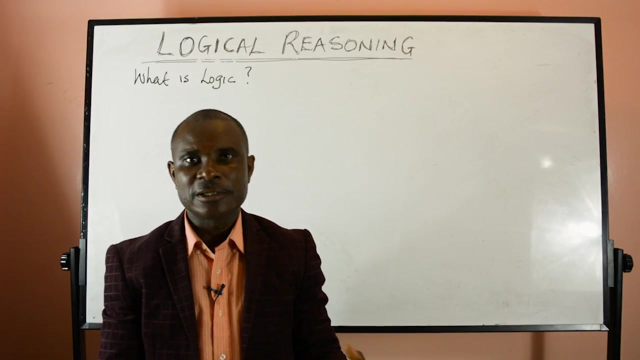 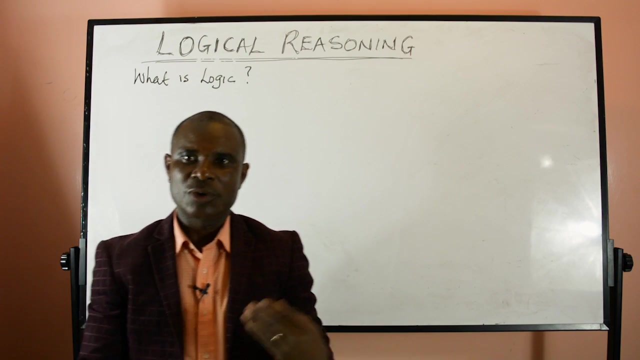 Thank you for watching. All right guys, welcome back to this math tutorial Today. we go along with math and our topic of discussion today is going to be logic and reasoning. And it's a very interesting topic because scientists believe that you have to work with data to collect information. We know that data is a piece of information gathered And if you collect this information, you have to hypothesize And in the process of hypothesizing, you now draw conclusions. 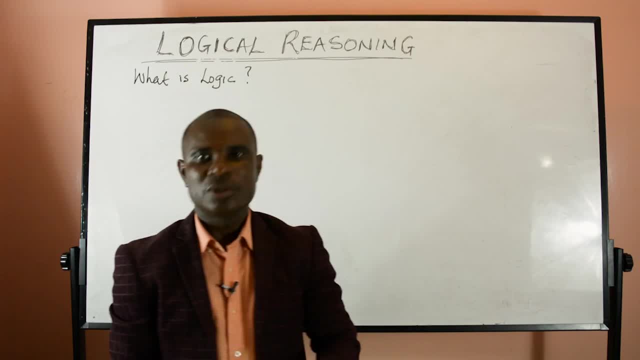 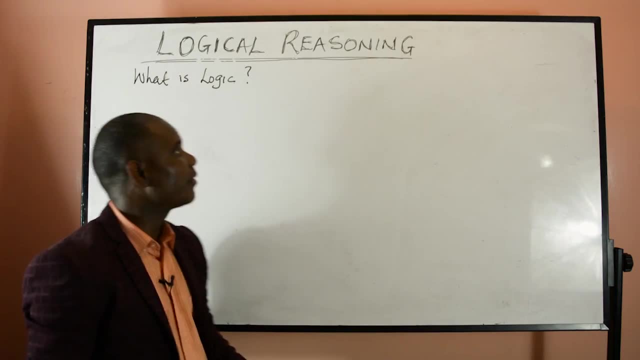 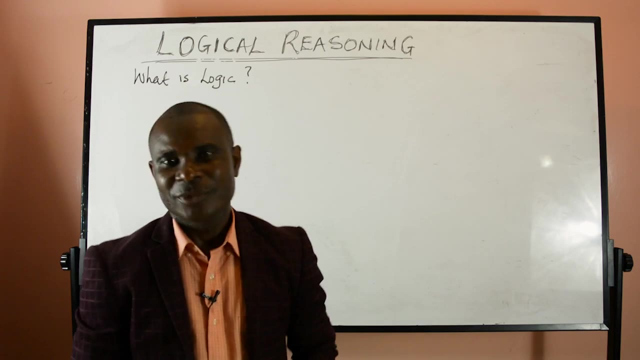 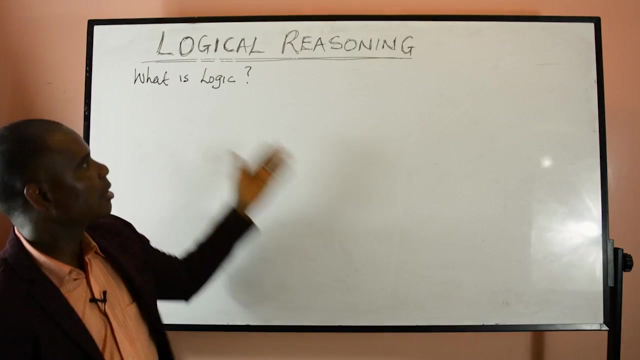 And when you draw a conclusion, then you base a conclusion. You are going to base your conclusion based upon what you've seen. So this is a very relevant topic in math and even in science. So we want to look at logic. So what's the big question? My name is Samuel D Quaidia. Now I want to first start by defining the word logic. What is logic? Logic is actually the science of thinking correctly. 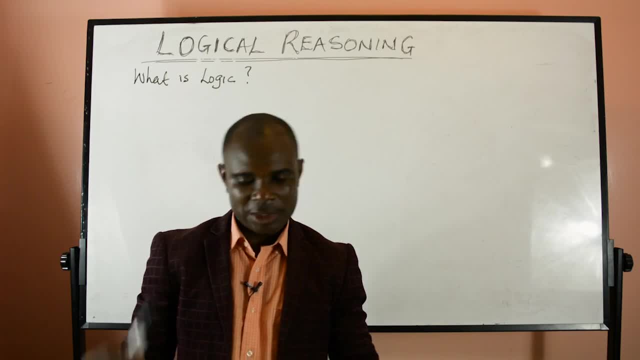 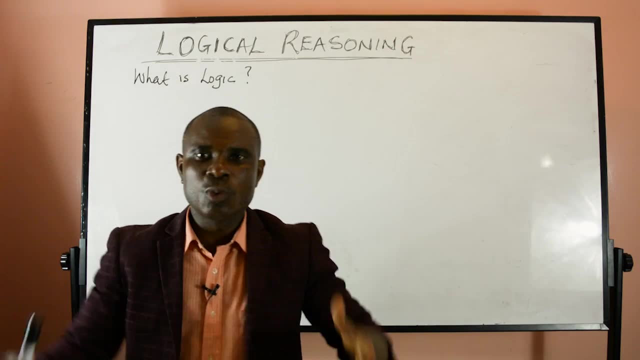 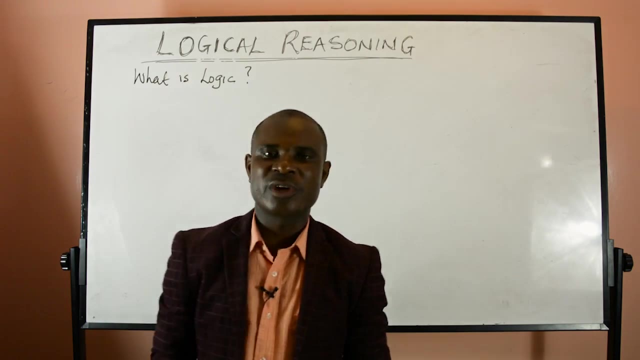 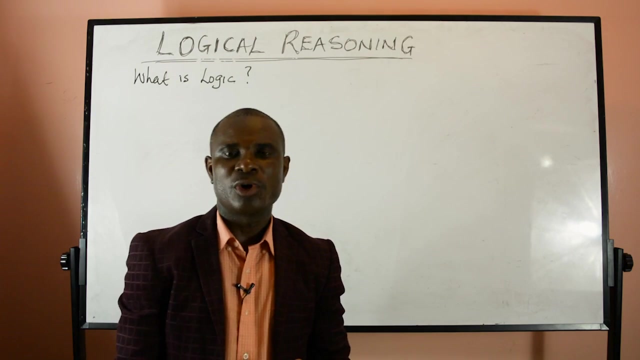 You know, it is the building block of argument And because, if you think correctly, that is how you'll be able to develop your argument And somebody will say, yes, you have a reason. power, And this word around us now is explained based upon rationalism. You must explain things based upon reasons. That is the moral reason why this topic is very important around our background. So let's look at it. What is logic? We say logic is the building block of argument and it's also the science of reason and thinking correctly, if you like. 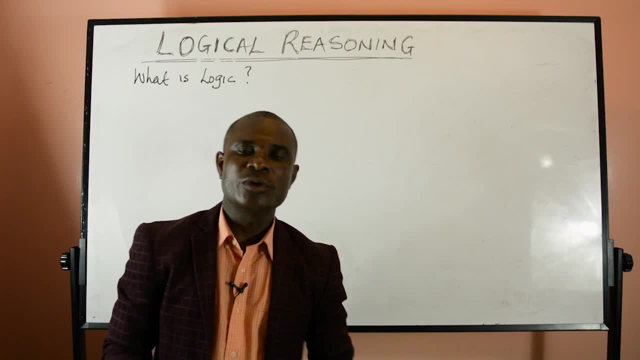 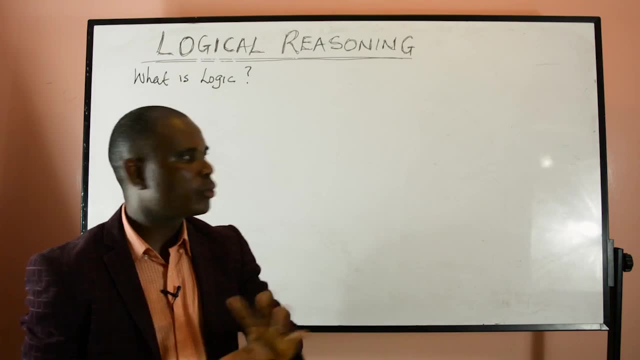 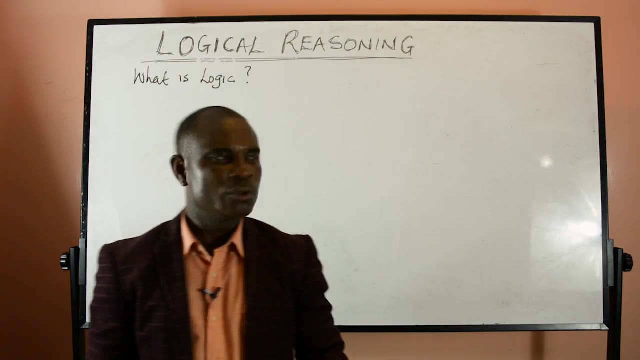 So what is the key thing here? If we want to talk about logic, we have to talk about statement, And I can categorize it first of all in two broad topics. This first video is going to just give you one part of this discussion on logic, And the next video, as you subscribe, you follow up as you move to the next definition of most, the next dimension of logic. 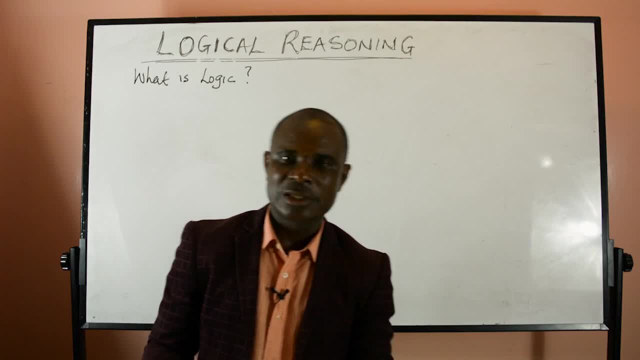 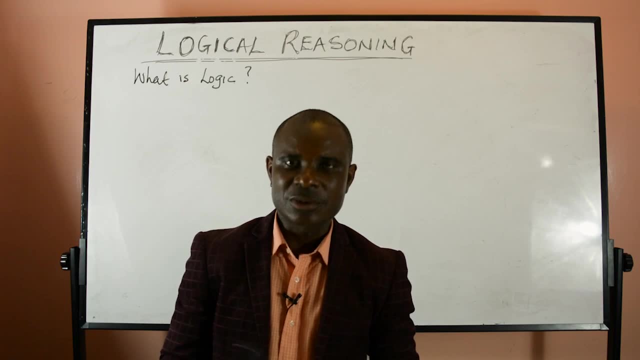 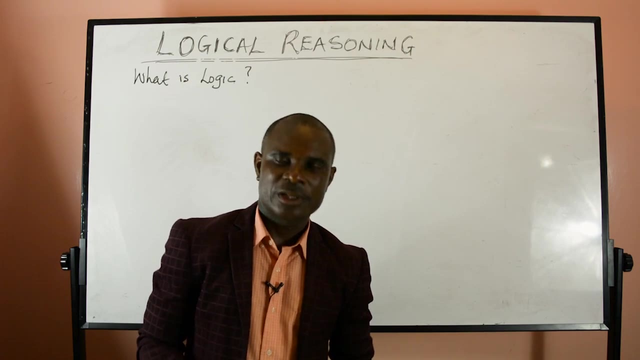 What the first dimension we want to look at is actually looking at the argumentative part of logic. Actually, logic is all based upon argument and so on and stuff like that. So let's look at the word itself. We said it is the science of thinking and reasoning correctly And it is also the building block of argument. 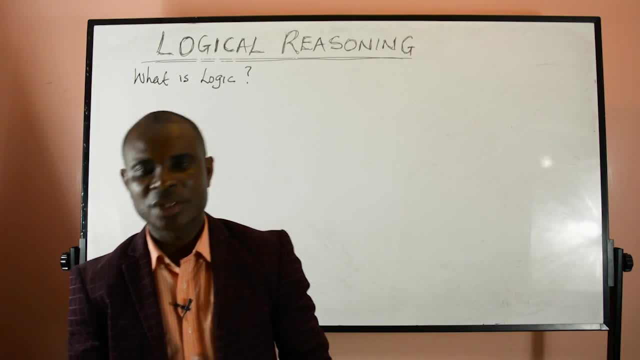 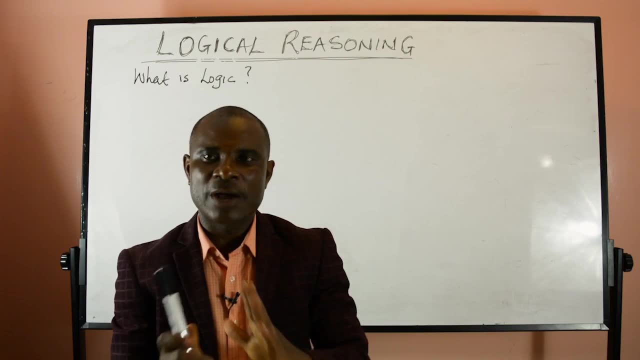 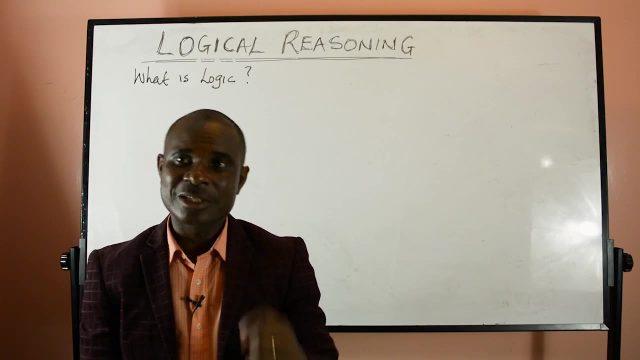 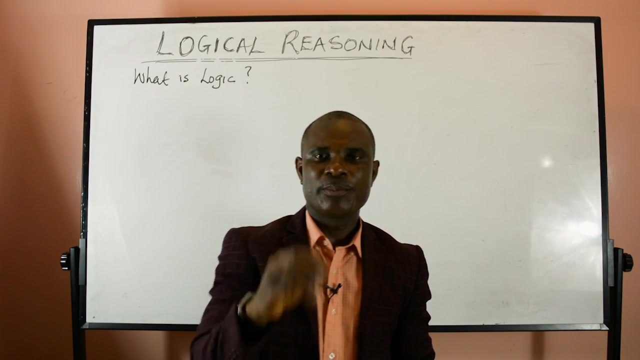 So what is the important thing in logic? The important thing in logic is that you have to draw a statement And that statement will presuppose something And we have to look at that statement and we'll be able to draw a conclusion. The first thing we look for in logic is a statement. What's a statement? A statement is a declarative sentence or a proposition which can be ascertained, can be allocated to be true or false. 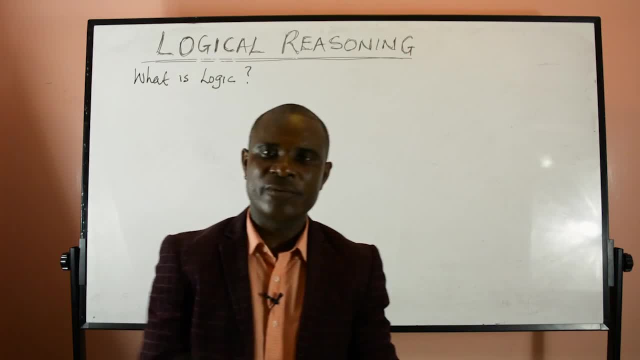 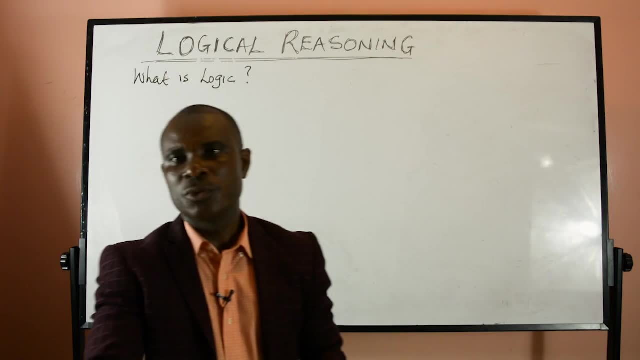 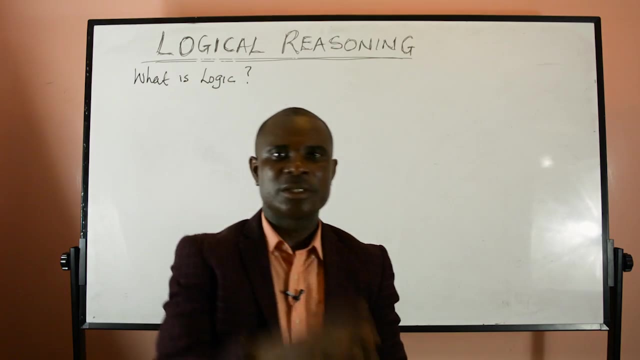 Or it's a statement, declarative sentence, that can either be true or false, but not both of them. In other words, it is a proposition which we can either confirm as a true proposition or we can also condemn it. it is false or true. so it's a statement, is a declarative sentence that is either true or false. 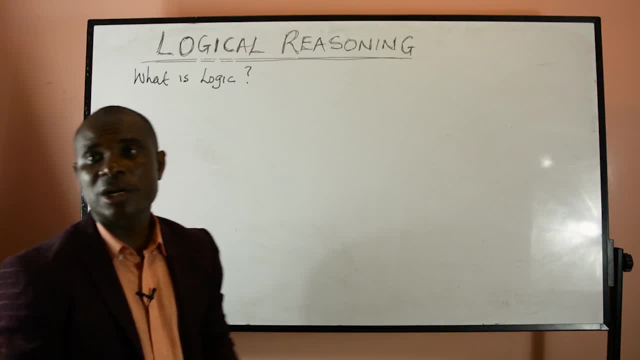 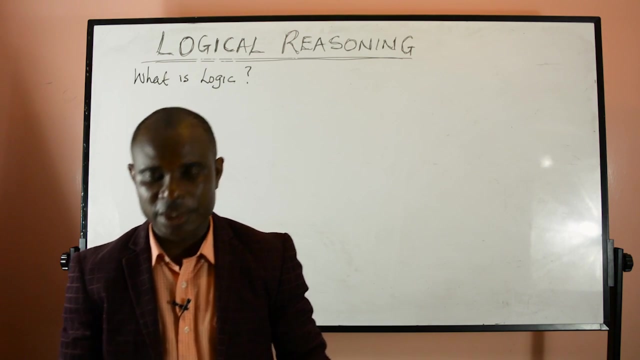 but not both of them. and in statements we can look at the, the types of statements. yeah, so we said the logic is a declare, logic is a science of thinking and reasoning correctly and we have already established the definition. we said it is the foundation. now is the building block of 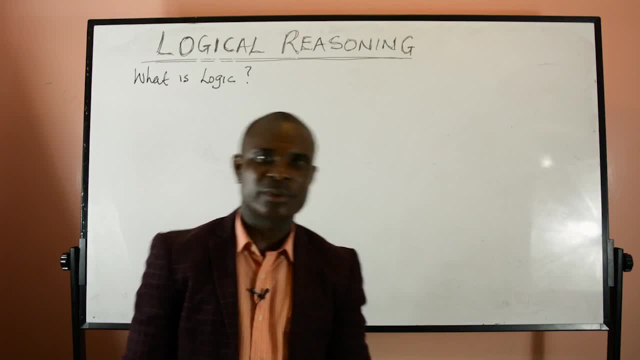 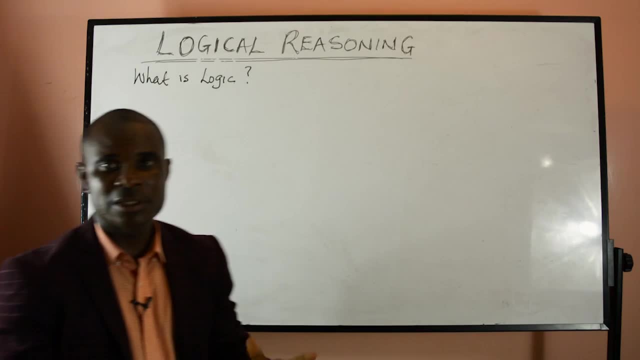 argument, and it is a science of thinking and reasoning correctness. but now we want to look at the fundamental thing we look for in logic: we look for statement. what is a statement? as i just told you, it is the declarative sentence. that is either true or false, and that cannot be two. 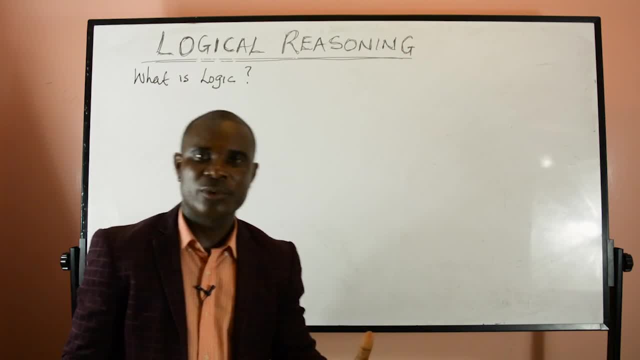 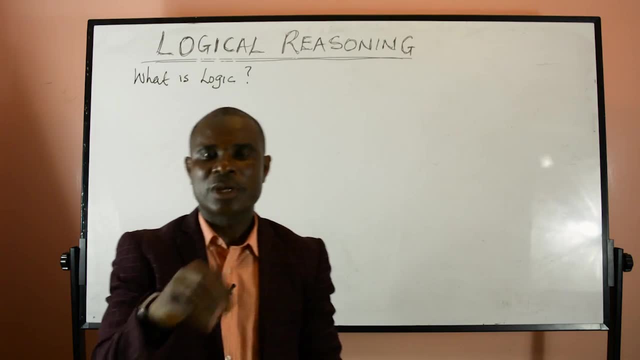 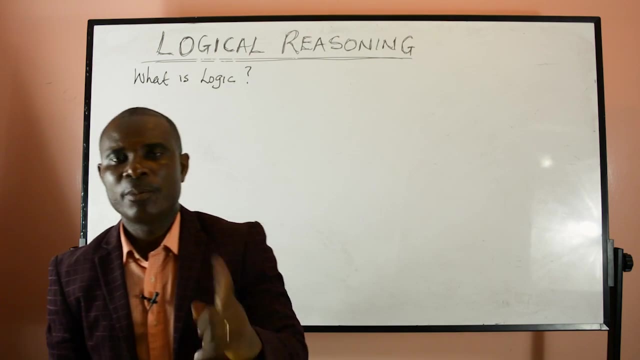 cannot be the two of them. it can be either true or false. example is: you say: all mass teachers are tall. so that's a statement which we can assert, we can affirm it all by by putting through values to it. if all teachers are mass teachers at all, then we can. we have verified that it is. 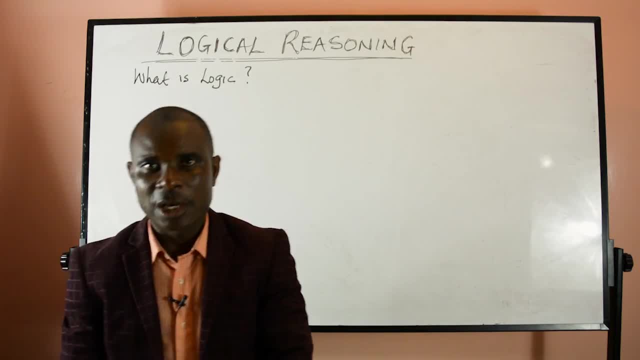 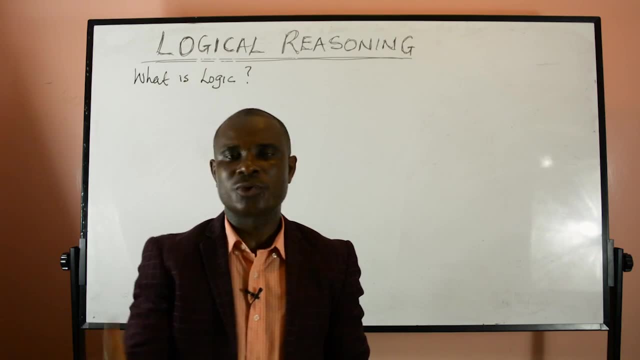 actually true, then we can ascertain the truth value true to it. and but we know that, no, all masters are not. all we can say that statement is: it's not valid, it's not. uh, for it's not true, it means it's false. so it is a declarative sentence that is either true or false, but it cannot be both. 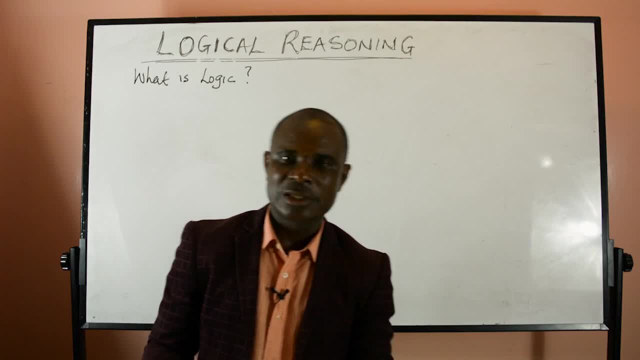 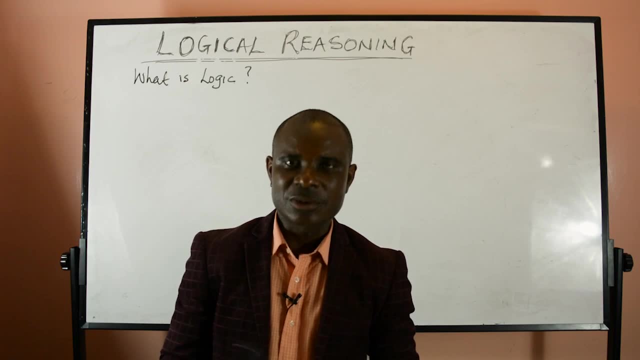 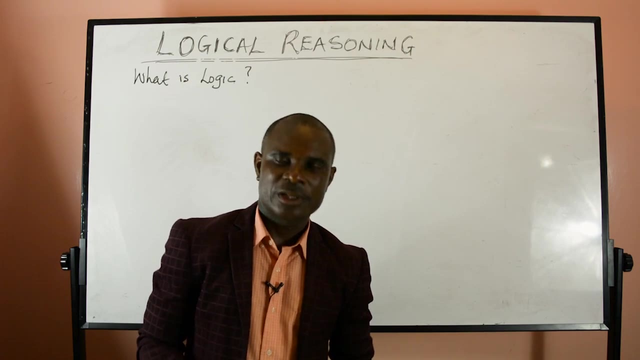 What the first dimension we want to look at is actually looking at the argumentative part of logic. Actually, logic is all based upon argument and so on and stuff like that. So let's look at the word itself. We said it is the science of thinking and reasoning correctly And it is also the building block of argument. 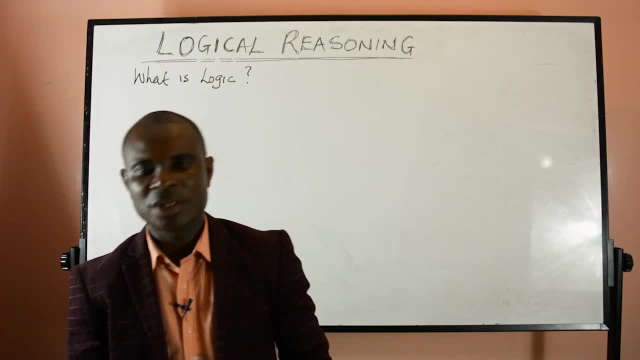 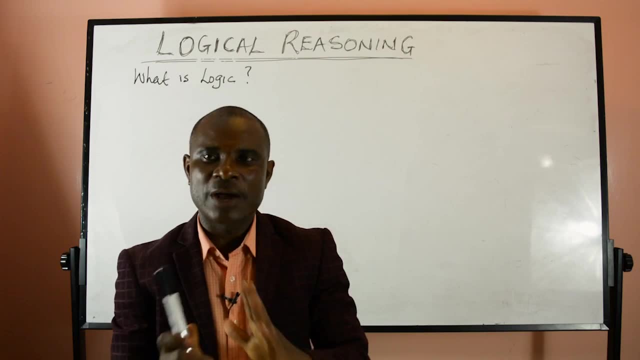 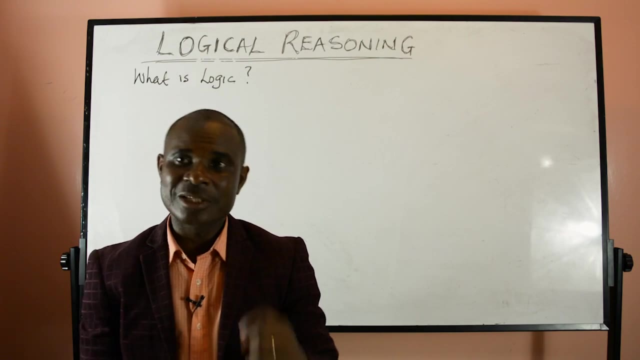 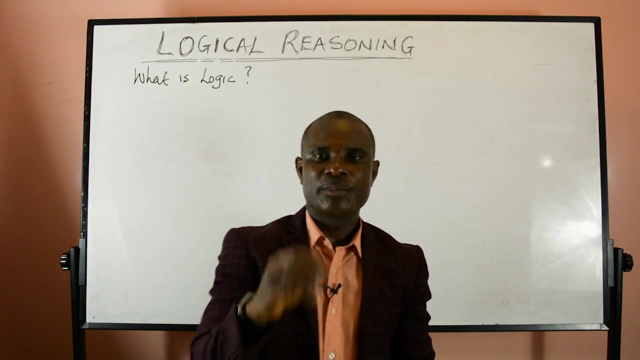 So what is the important thing in logic? The important thing in logic is that you have to draw a statement And that statement will presuppose something And we have to look at that statement and we'll be able to draw a conclusion. So the first thing we look for in logic is statement. What's a statement? A statement is a declarative sentence or a proposition which can be ascertained, can be allocated to be true or false. 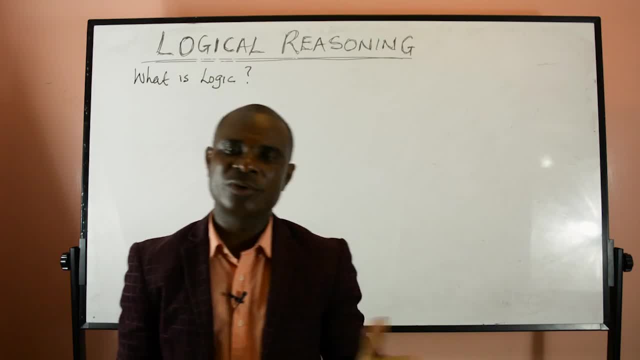 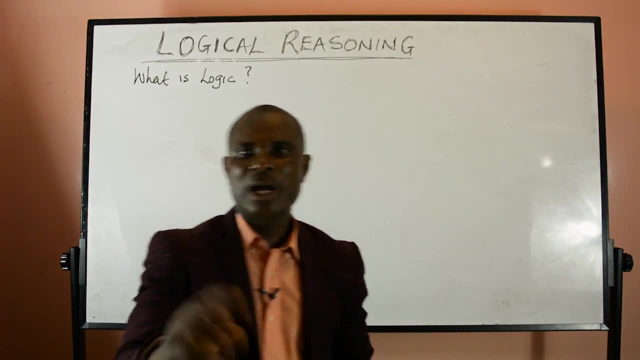 Or it's a statement, declarative sentence, that can either be true or false, but not both of them. In other words, it is a proposition which we can either confirm as a true proposition or we can also condemn it. it is false or true. so it's a statement, is a declarative sentence that is either true or false. 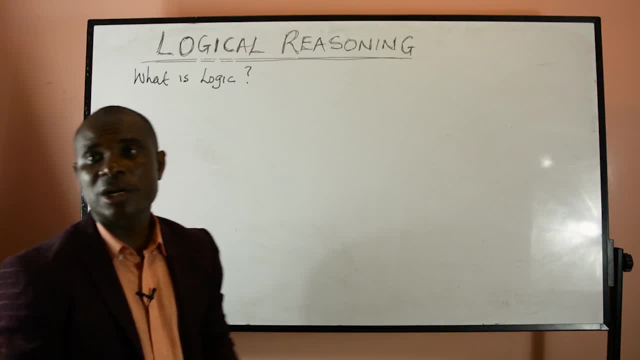 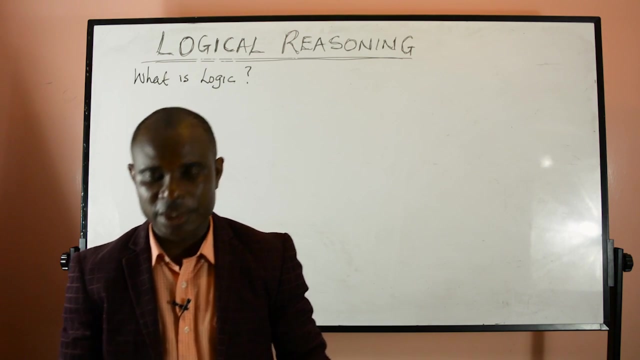 but not both of them. and in statements we can look at the, the types of statements. yeah, so we said the logic is a declare, logic is a science of thinking and reasoning correctly and we have already established the definition. we said it is the foundation. now is the building block of 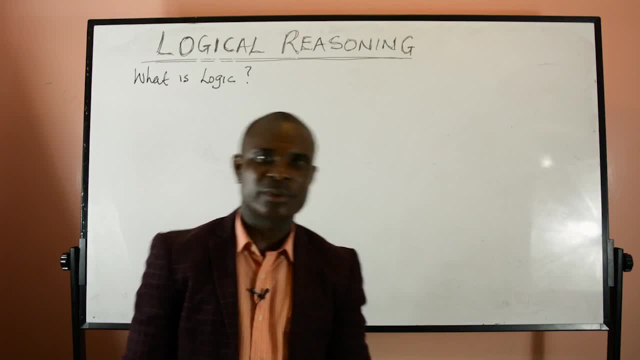 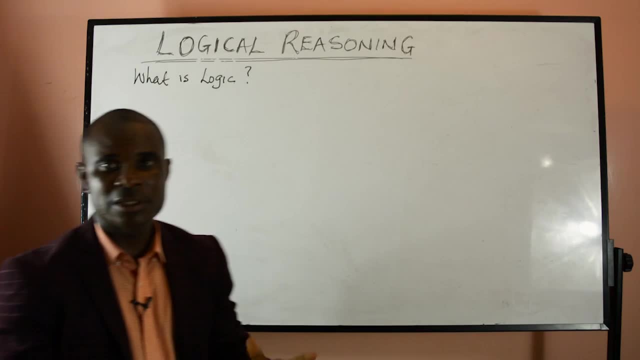 argument, and it is a science of thinking and reasoning correctness. but now we want to look at the fundamental thing we look for in logic: we look for statement. what is a statement? as i just told you, it is the declarative sentence. that is either true or false, and that cannot be two. 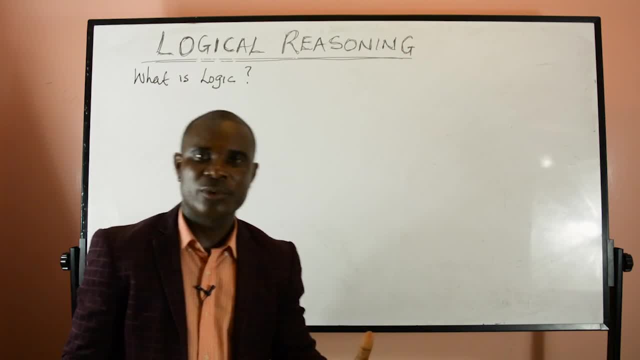 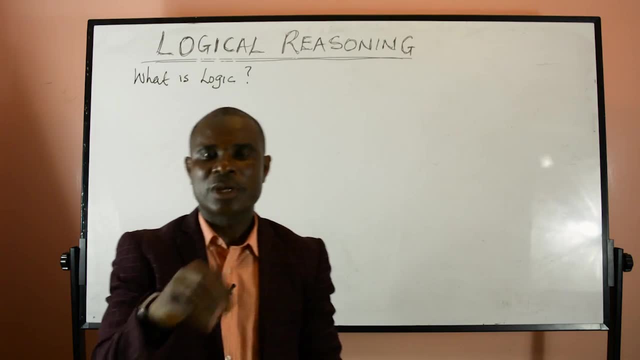 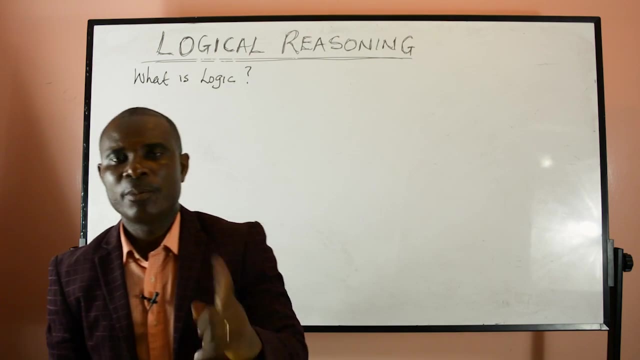 cannot be the two of them. it can be either true or false. example is: you say: all mass teachers are tall. so that's a statement which we can assert, we can affirm it all by by putting through values to it. if all teachers are mass teachers at all, then we can. we have verified that it is. 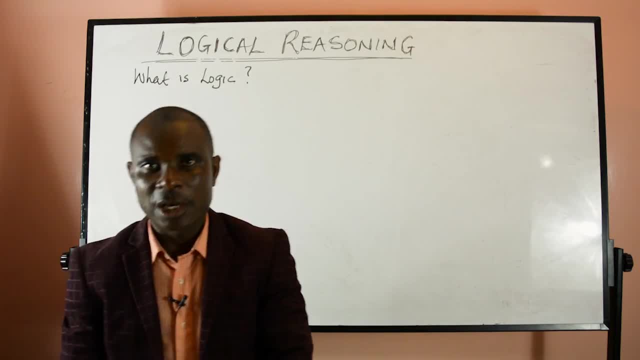 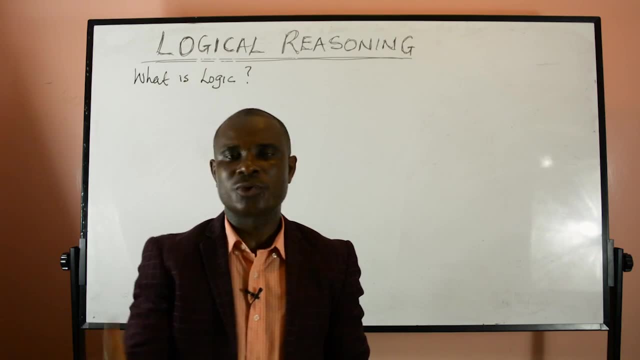 actually true, then we can ascertain the truth value true to it. and but we know that, no, all masters are not. all we can say that statement is: it's not valid, it's not. uh, for it's not true, it means it's false. so it is a declarative sentence that is either true or false, but it cannot be both. 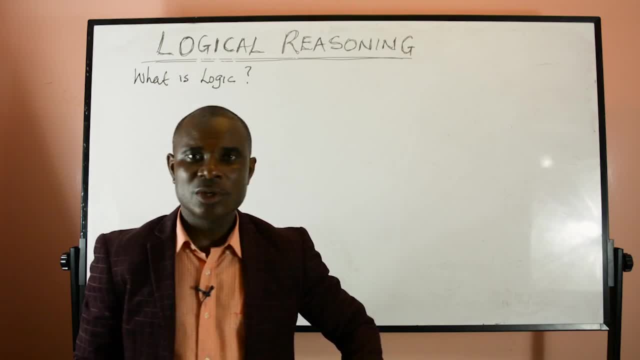 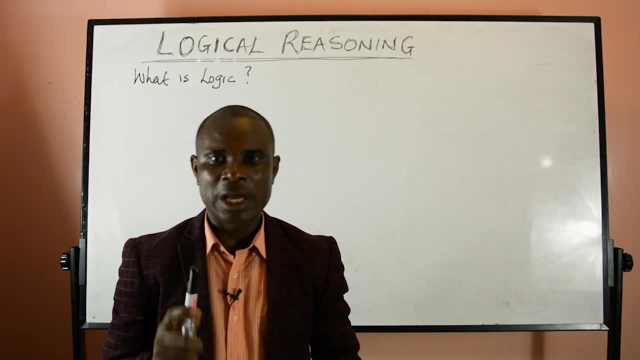 of them. so you have to ensure that it is either a true statement or it's going to be a false statement. so statement not everything we say, we say, we we consider to be a statement if i cannot ascertain or cannot confirm the validity of that statement either by putting a truth value. 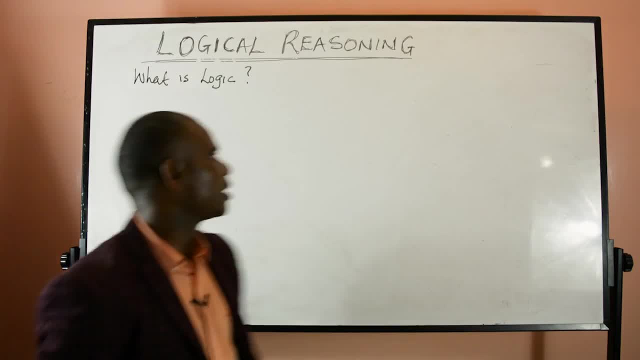 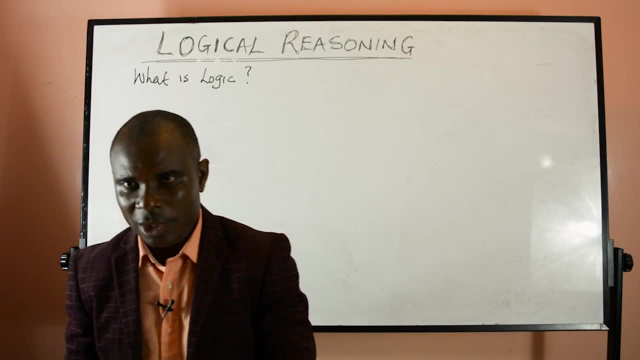 to identify whether it's true or false, then we can not call it a statement. so we have declarations that are not statements actually, but normally because of our normal conversation we consider them our statement. for instance, if you see no packing, no packing with a, normally see all of those writings along the highway or along parking lots, we see. 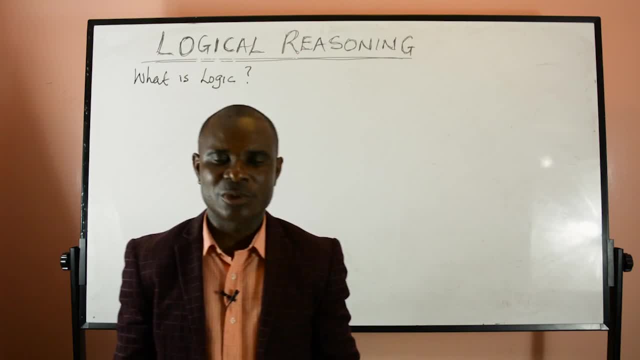 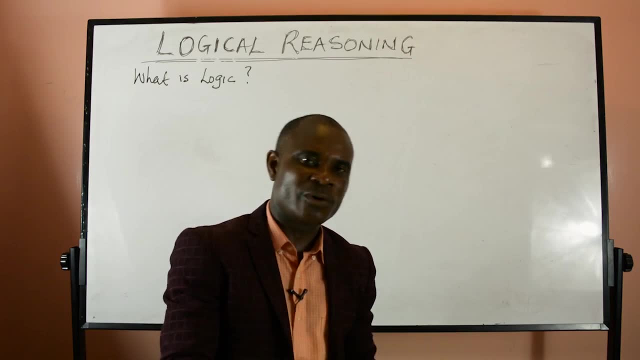 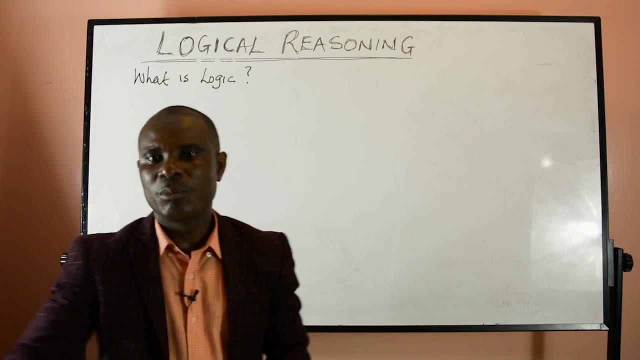 no parking, no parking. what's that? is a statement or not? we cannot affirm, we cannot attach true value to that. you cannot say it is true or first so. because you can't say it is true of us, that statement is not a statement, it's just a declaration. so we can also. we have more of them in in our day-to-day. 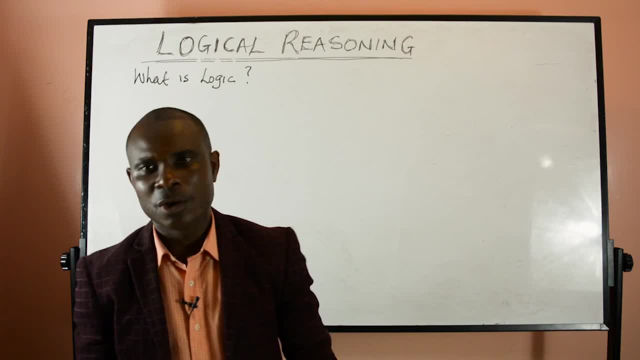 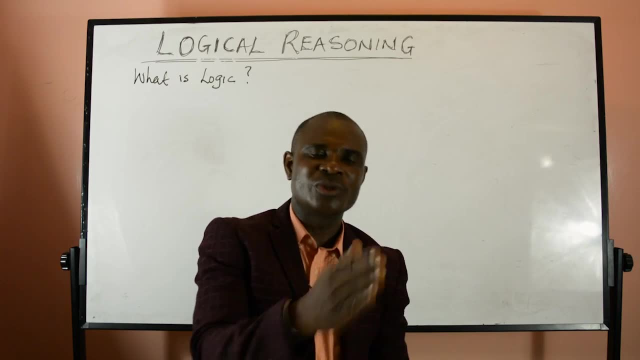 discussions like what you see in the bank when we get to the bank is: it: counts your money before you leave the counter. what is that? it's not a statement, but we refer to it as a statement because you cannot put a truth value on that statement: counts your money before you leave the counter. you. 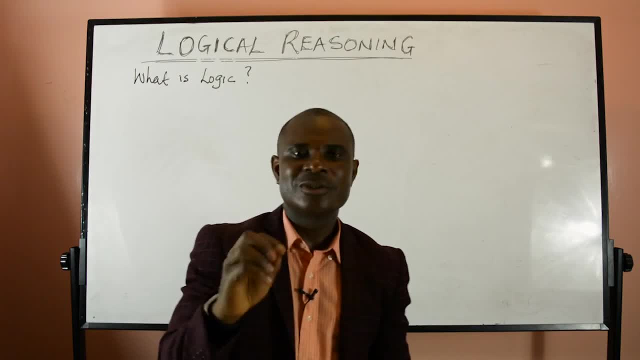 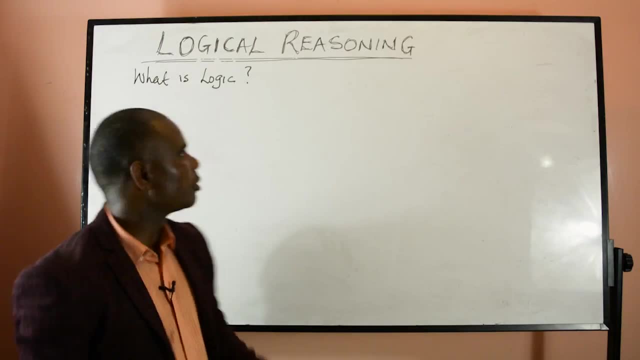 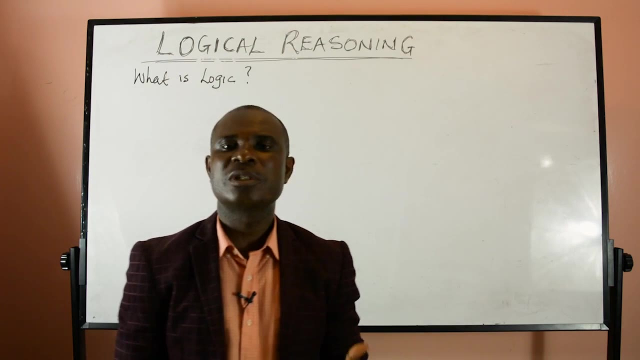 can't put true or false on that statement, so it is not a statement, it is a non-statement. but sometimes we use them as often as we can. but today we want to look at statements that are, or declarative sentences, which you can refer to us as statements, as those ones that we can attach true to value, to 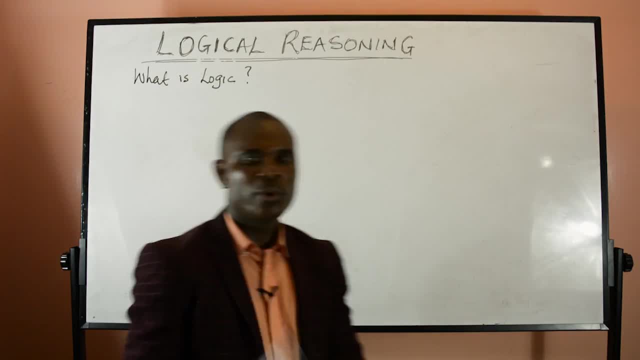 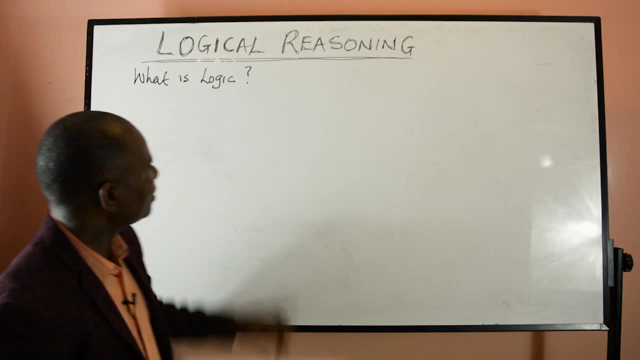 meaning, we can affirm whether it's true or false. when, once, we cannot put a truth value to it by indicating whether it is true or false, then that statement is not a statement. so I can now go to the types of statements. now, what are the types of? 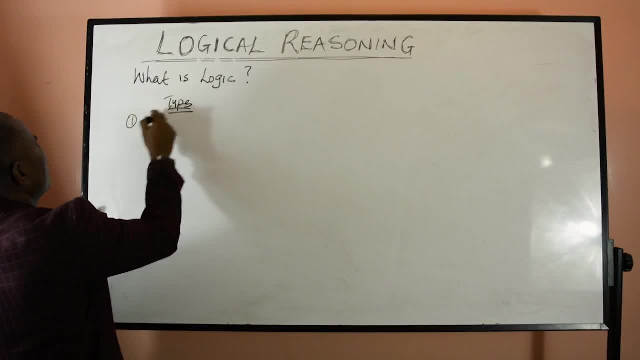 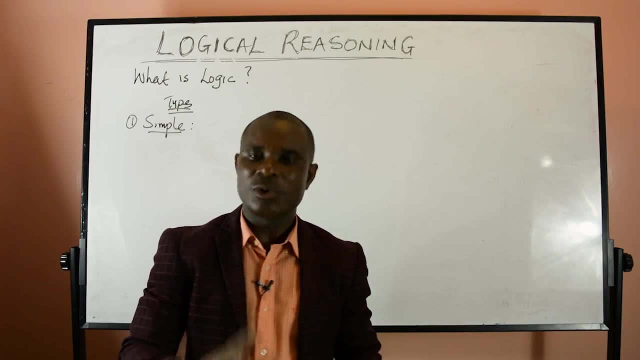 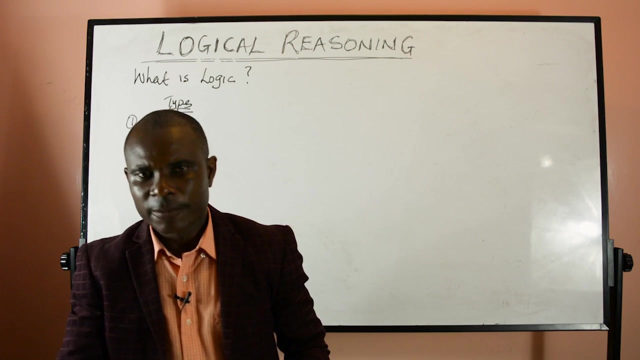 statements. so we said: we have types first, we have a simple statement. what is a simple statement? a simple statement conveys only a simple or single idea. it is giving us only one idea. for instance, if I say John is a boy, John, what about? what about John? John is a boy. this is gender. 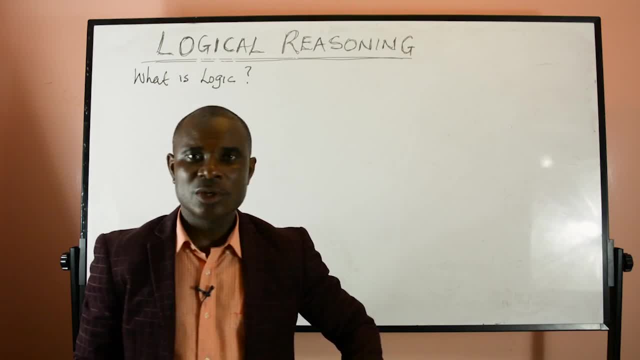 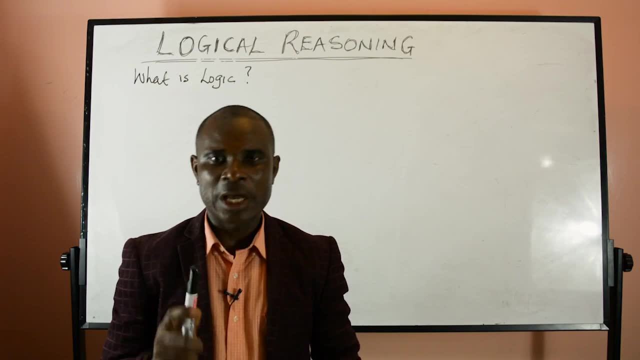 of them. so you have to ensure that it is either a true statement or it's going to be a false statement. so statement not everything we say, we say, we we consider to be a statement. if i cannot assert more, i cannot confirm the validity of that statement either. by putting 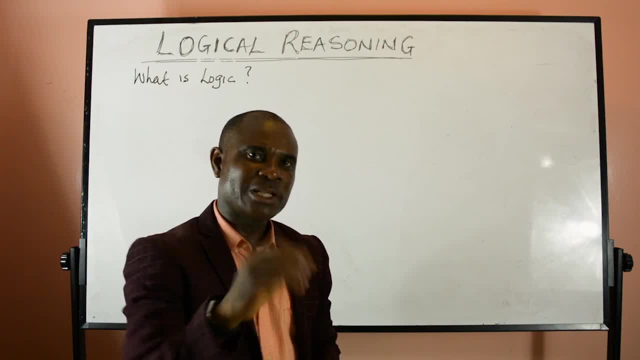 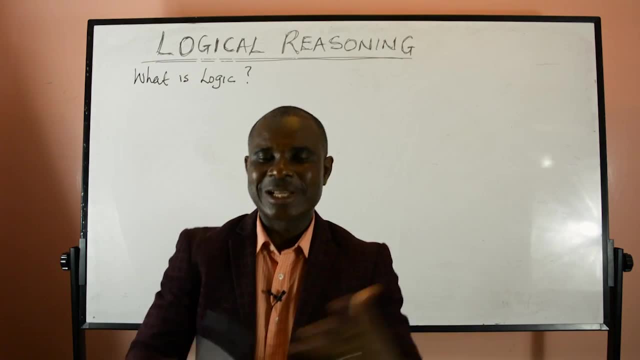 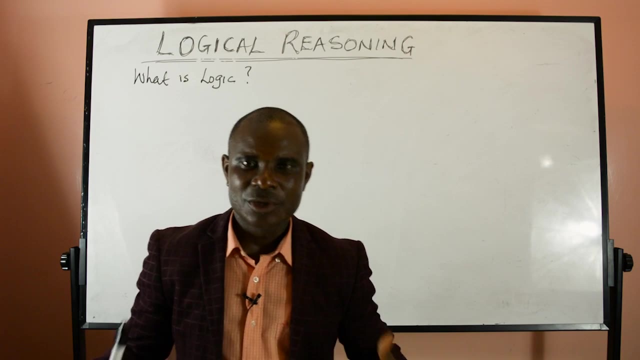 a truth value to, to identify whether it's true or false, then we can not call it a statement. so we have uh declarations that are not statement actually, but normally because of our normal conversation we consider them a statement. for instance, if you see: no packing, no packing, we'll. 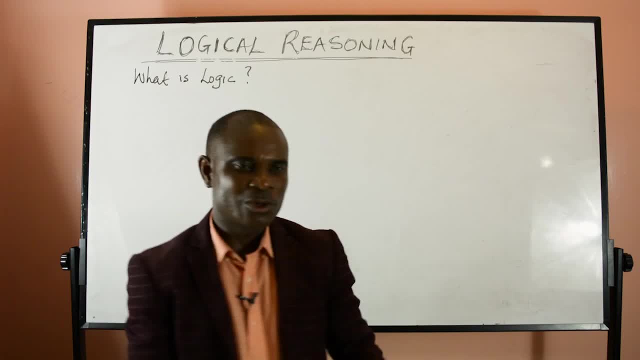 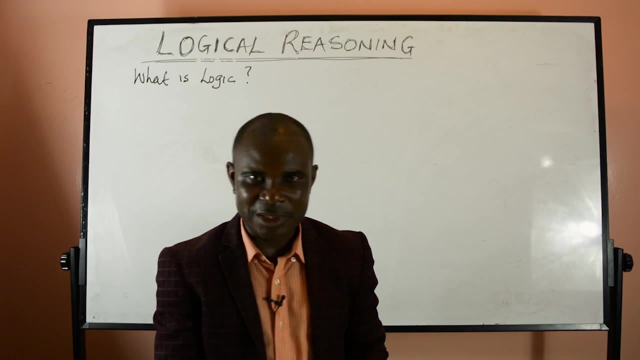 normally see all of those writings along the highway or along parking lots. we see no parking, no parking. what's that? is a statement or not? we cannot affirm, we cannot attach true value to that. you cannot say it is true or first so because you can't say it is true of us, that statement is not a statement, it's. 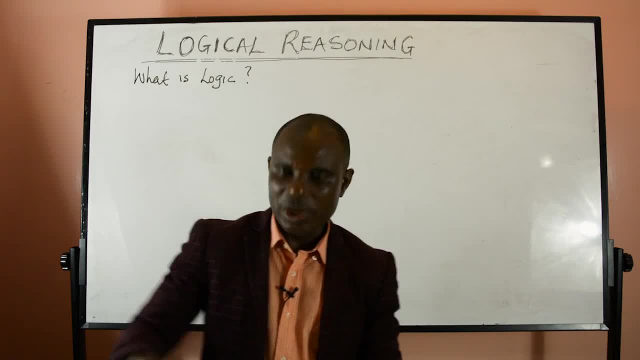 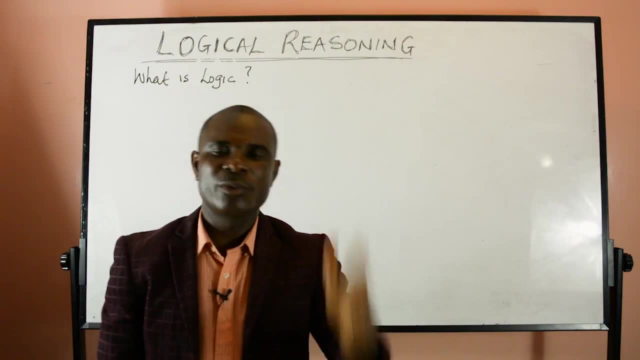 just a declaration so we can also. we have more of them in in our day-to-day discussions. like what you see in the bank when we get to the bank is it counts your money before you leave the counter. what is that? it's not a statement, but we refer to it as a statement because you cannot put a truth. 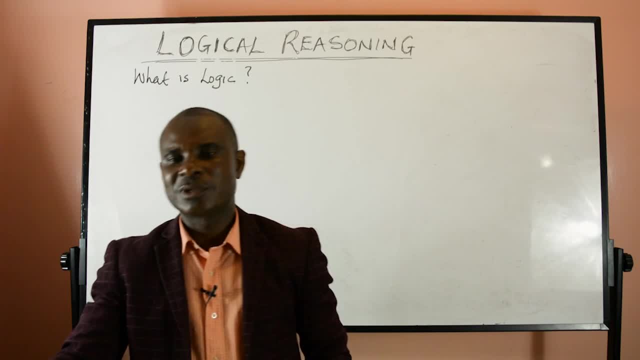 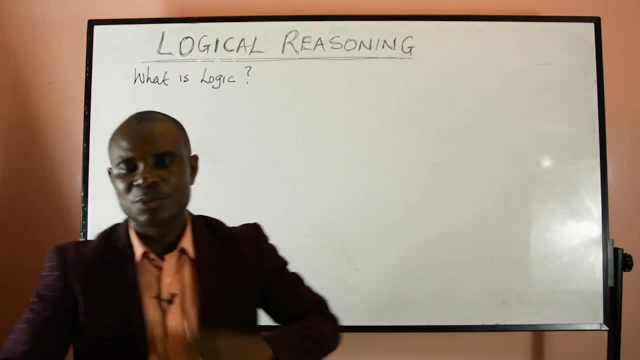 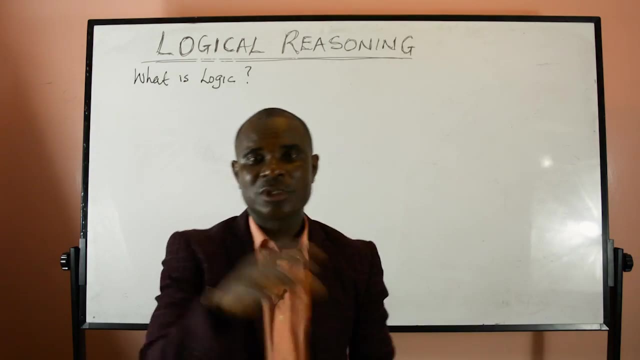 value on that statement counts your money before you leave the counter. you can't put true or false on that statement, so it is not a statement, it is a non-statement. but sometimes we use them as often as we can. but today we want to look at statements that are, or declarative sentences, which you can. 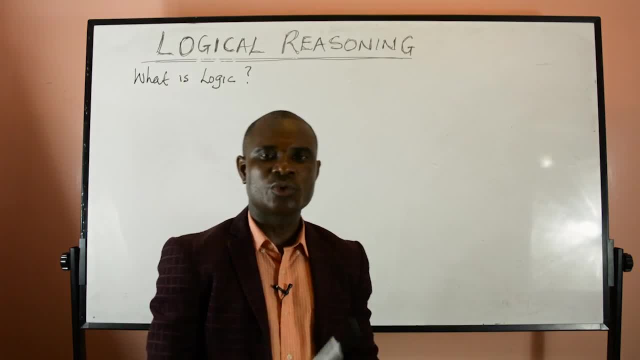 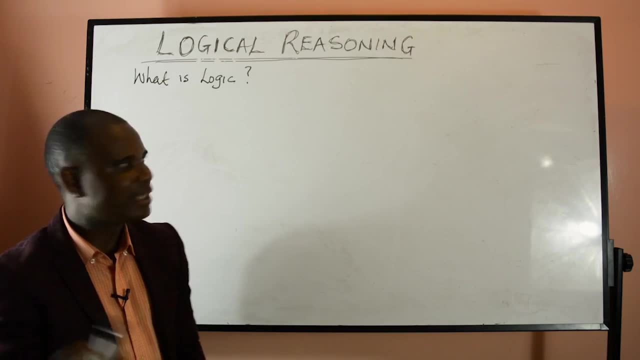 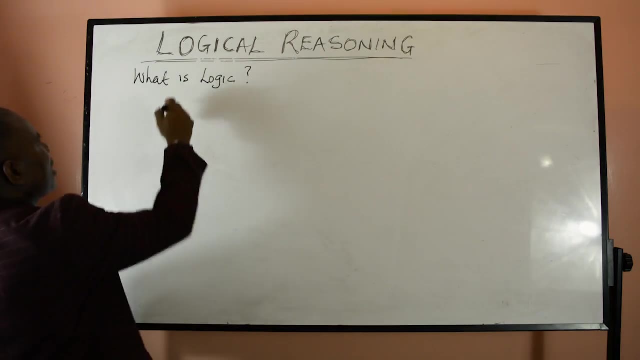 refer to us as statements, as those ones that we can attach true to value, to meaning. we can affirm whether it's true or false. when, once, we cannot put a truth value to it by indicating whether it is true or false, then that statement is not a statement. so I can now go to the types of statements. now, what are the types of? 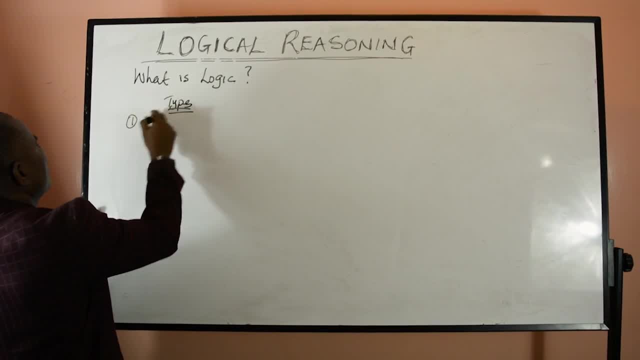 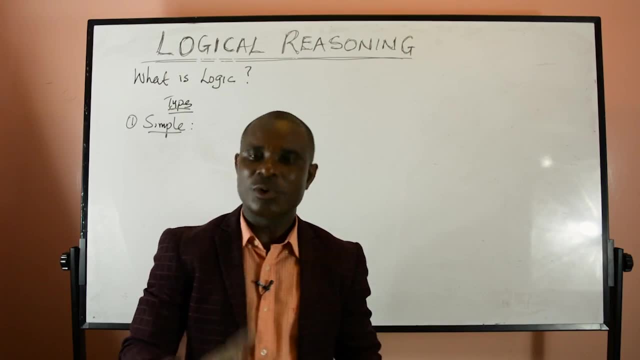 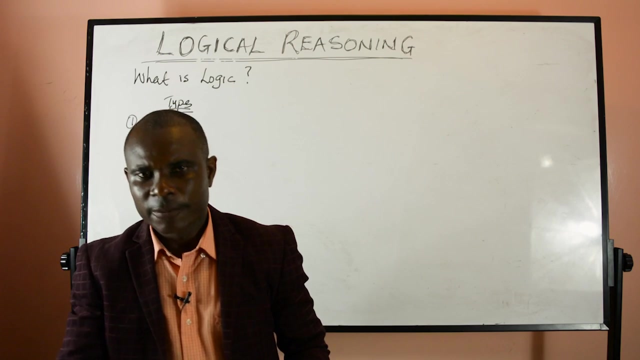 statements. so we said: we have types first, we have a simple statement. what is a simple statement? a simple statement conveys only a simple or single idea. it is giving us only one idea. for instance, if I say John is a boy, John, what about? what about John? John is a boy. 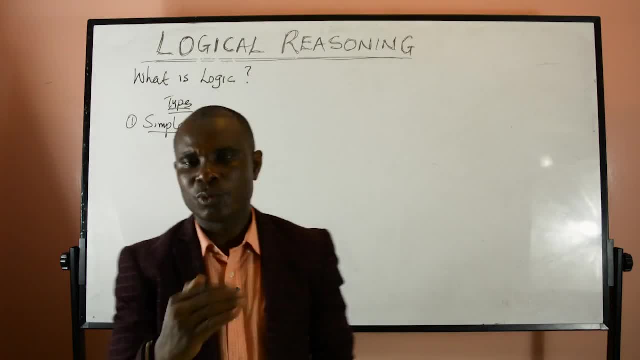 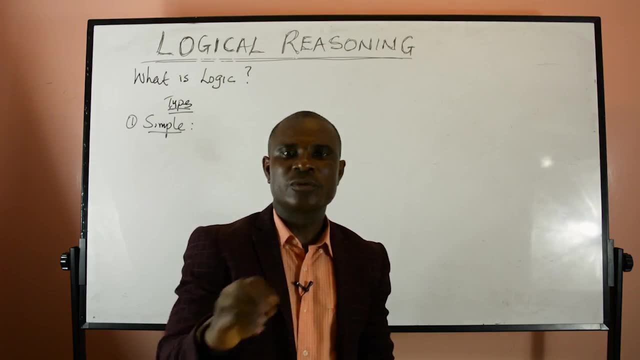 this is gender. this is all one idea I just want to know about John. John is a voice and when I look at the statement, John is a boy, if I can attach truth value there. so I look at John. if John is actually a boy, then I know that that. 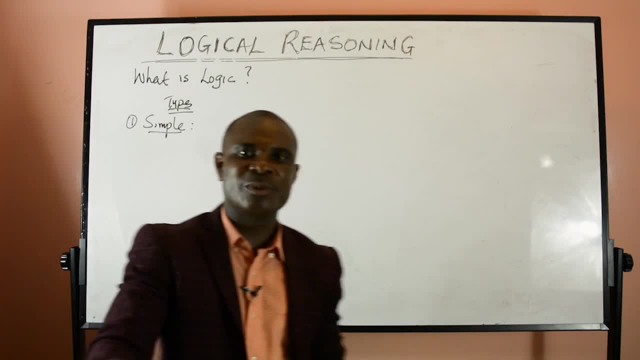 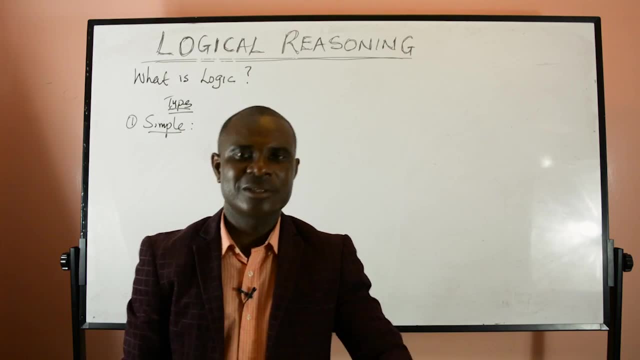 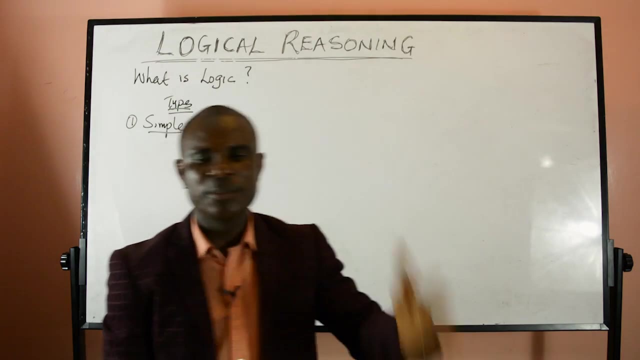 statement is true. but if I look at John, John is not a boy. that means that statement is false. so I can put a truth value on that statement and that statement is conveying only a single idea. because it is conveying a single idea and we can put true or false value to that statement. we call it a simple statement, a simple. 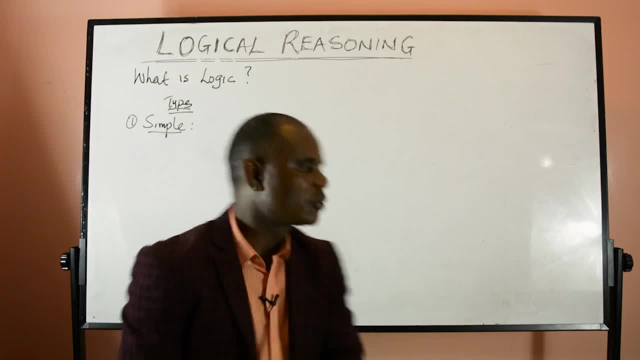 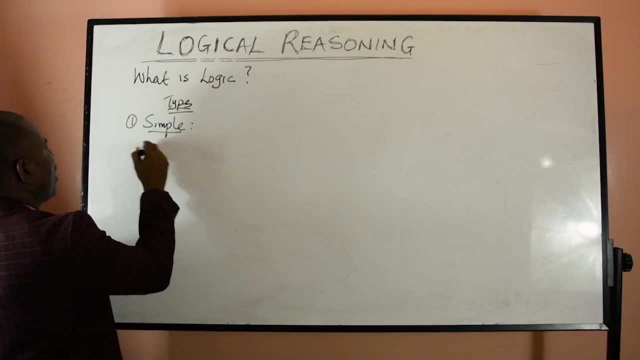 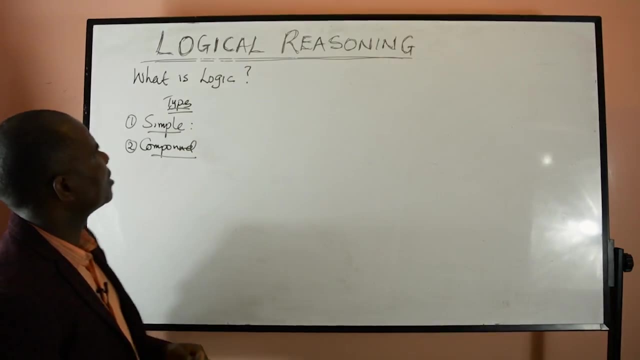 statement convey only a single idea. so that is what we call a simple statement. and i'll just give you an example. what about the second type? we have a compound statement. we have compound statement number two, the other type of statement is a compound statement, so we have simple statement. 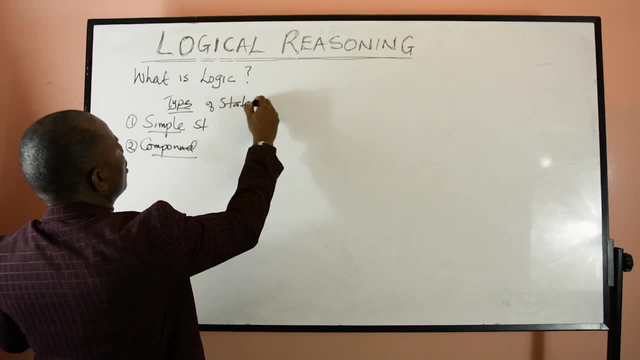 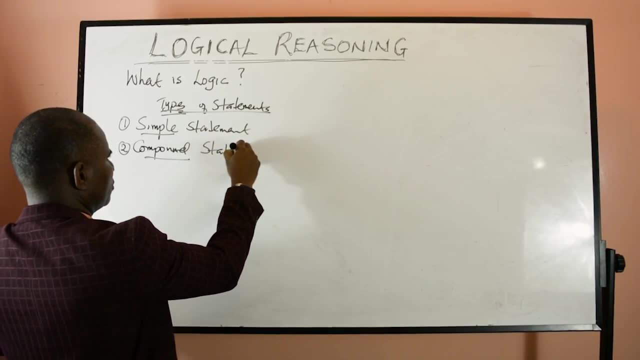 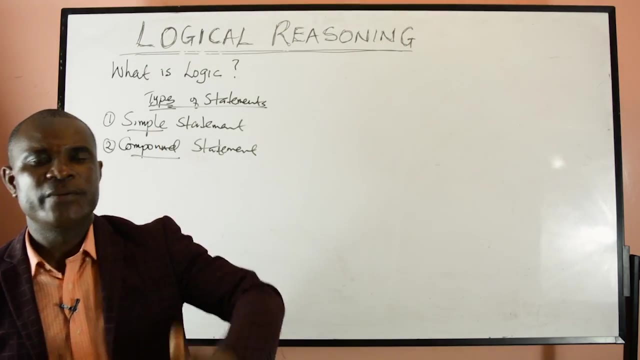 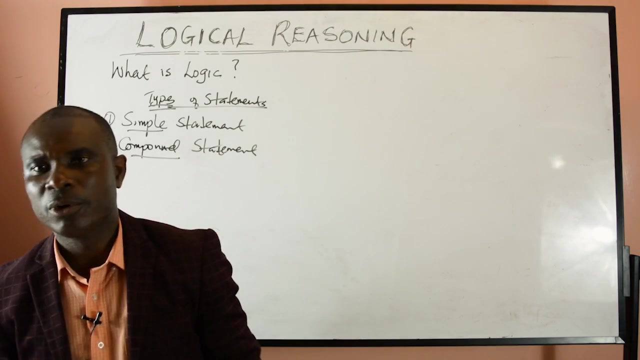 types of statements. let me just put them there. i have simple statement, i have compound statement. so what is a simple statement? i just said a simple statement convey only a single idea, or one idea, and it could be john is a boy like my, my example. or this book is black, or mary is. 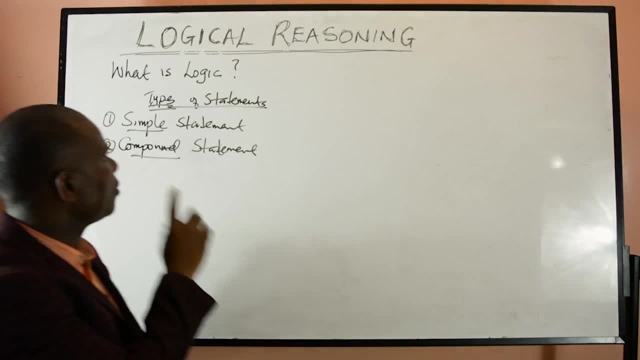 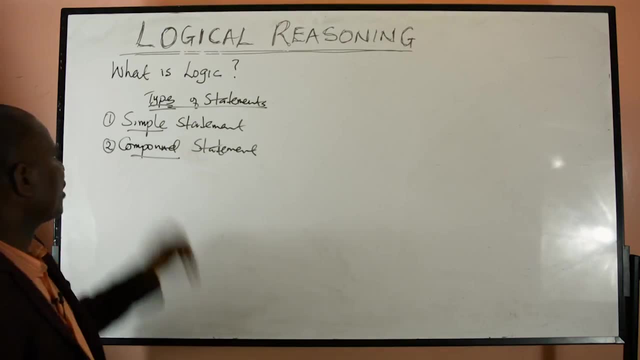 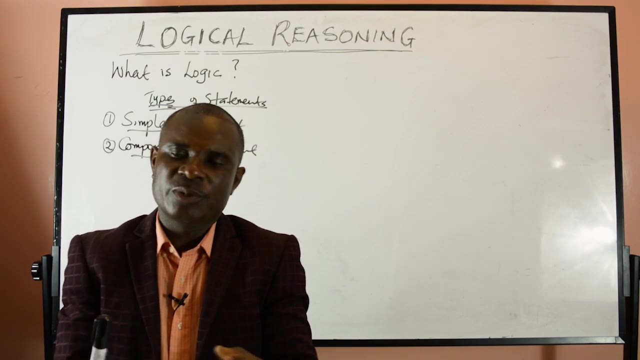 eager. these are single ideas, single thoughts that are conveyed in that declaration. so a simple statement only has one idea, single idea. all right, we have a compound statement. what is a compound statement? you see, it's a composite form when we put two or more simple statements together. 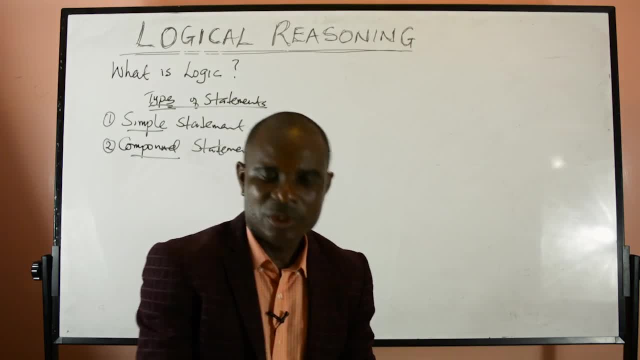 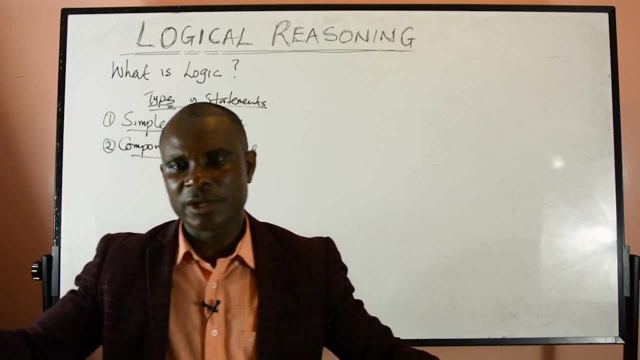 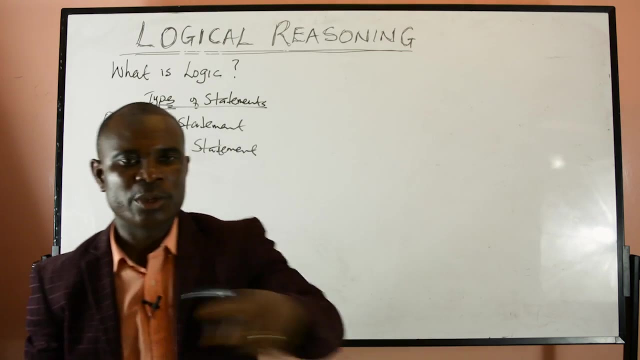 by connective terms like and but. so, for instance, if i say john is a boy and john is clever, so and has connected john is a boy and john is clever. john is clever is a simple statement because they can attach it to gravity, there john is clever, true or false. john is a boy- true. of course i can put 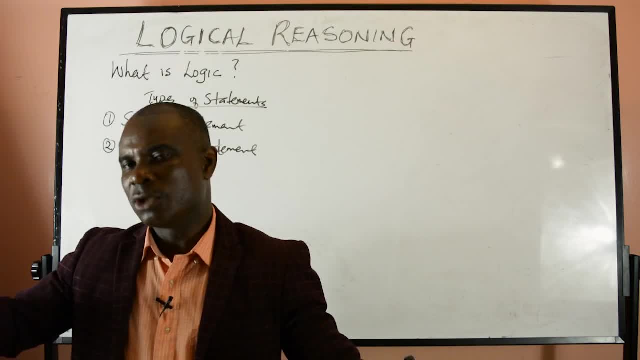 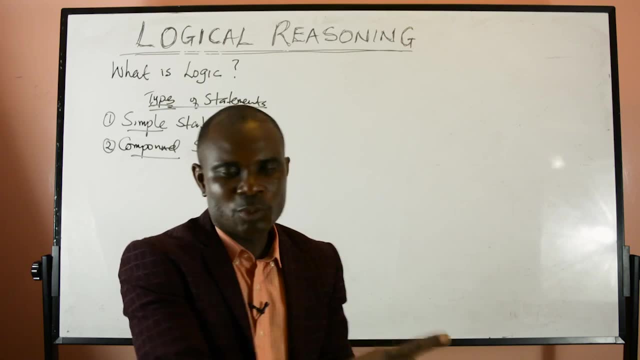 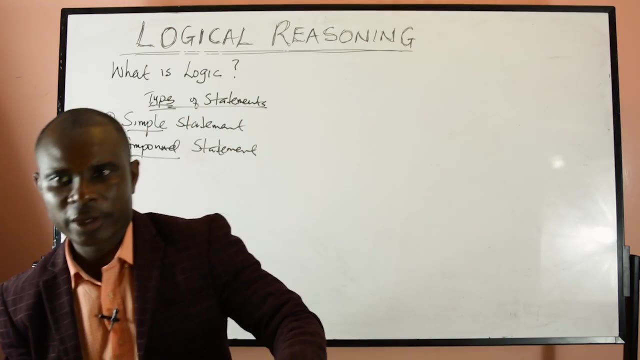 two or fours on this statement. i can put row of us on the other statement here, so, but the two statements, which are simple statements, are joined together by a connective term, and that's what i just said. said: john is a boy and john is clever. if i can put true value on john is a boy, then that: 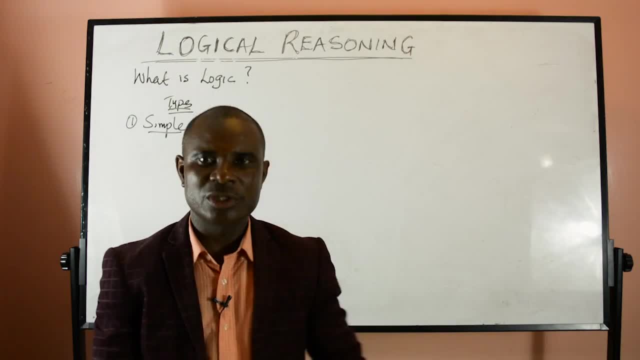 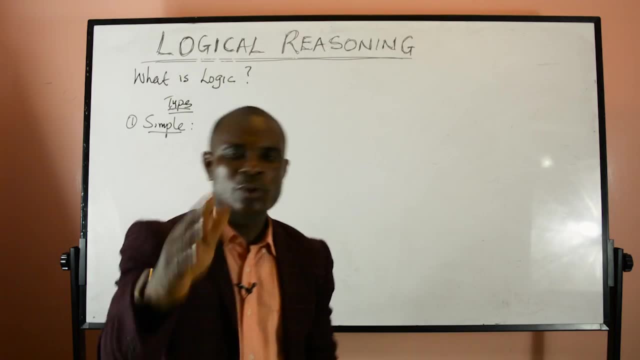 this is all one idea I just want to know about John. John is a boys and when I look at that statement, John is a boy, if I can attach truth value there. so I look at John. if John is actually a boy, then I know that a statement is true. but if I 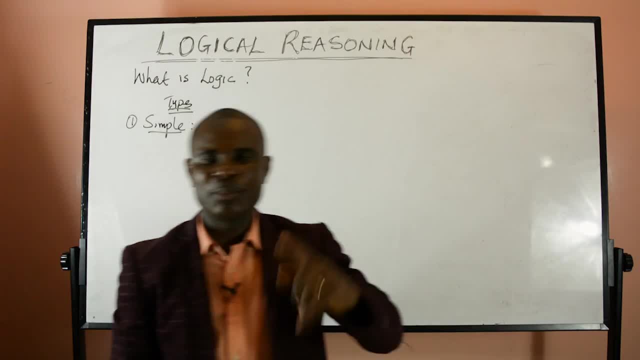 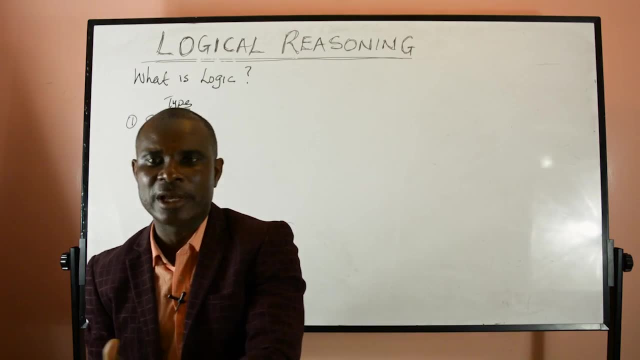 look at John. John is not a boy. that means that statement is false. so I can put a truth value on that statement and that statement is conveying only a single idea. because it is conveying a single idea and we can put true or false value to that statement. we call it a simple statement, a simple. 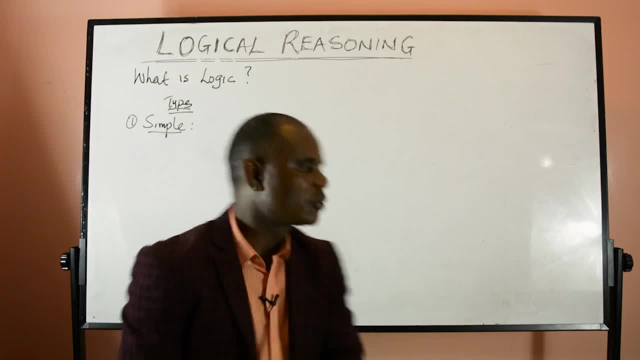 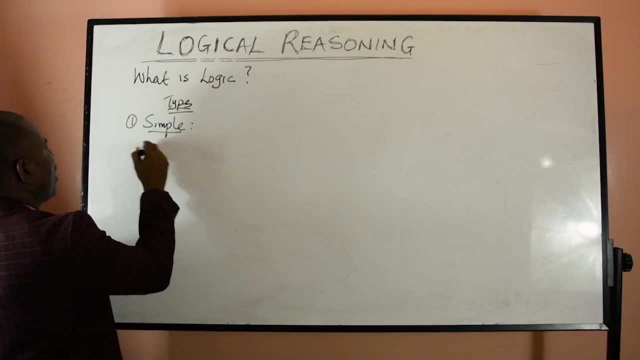 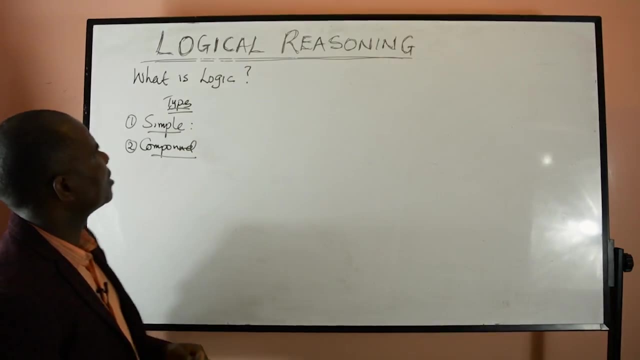 statement convey only a single idea. so that is what we call a simple statement. and i'll just give you an example. what about the second type? we have a compound statement. we have compound statement number two, the other type of statement is a compound statement, so we have simple statement. 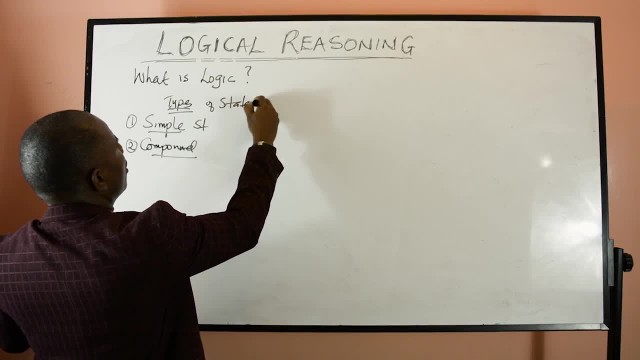 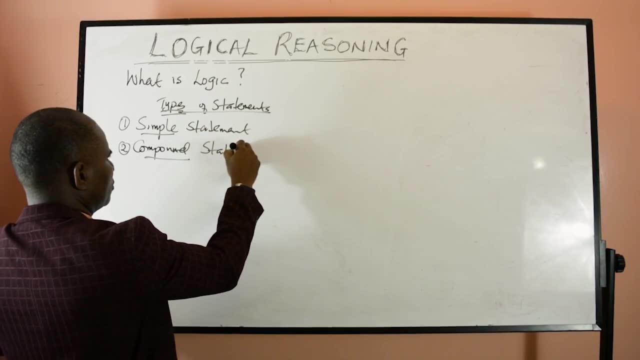 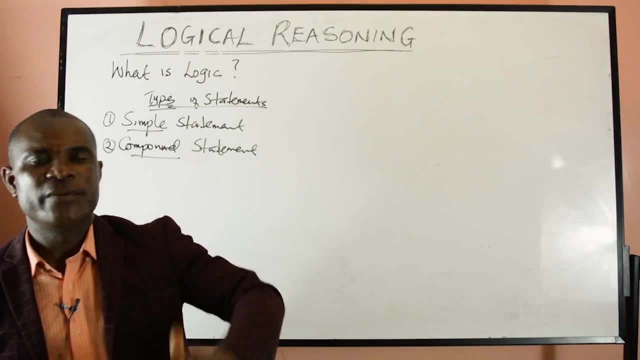 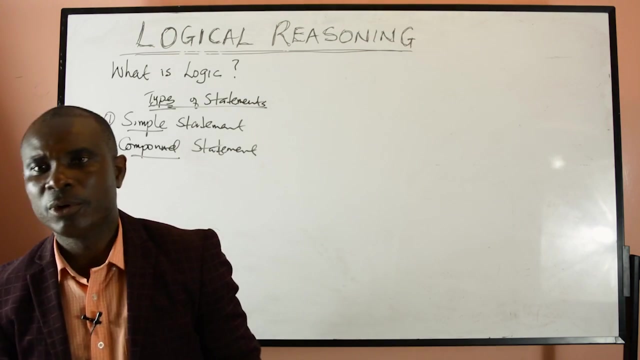 types of statements. let me just put them there. i'll have simple statement, i'll have compound statement. so what is a simple statement? i just said a simple statement convey only a single idea, or one idea. and it could be: john is a boy like my, my example, or this book is black, or 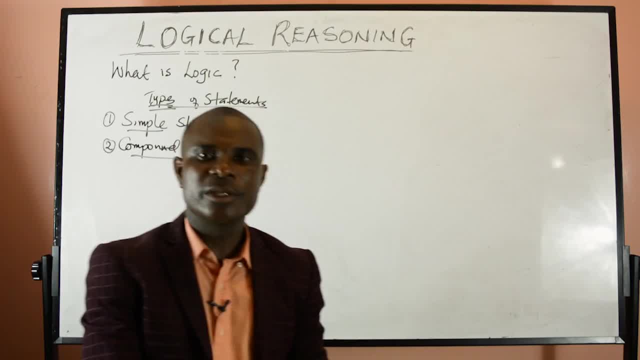 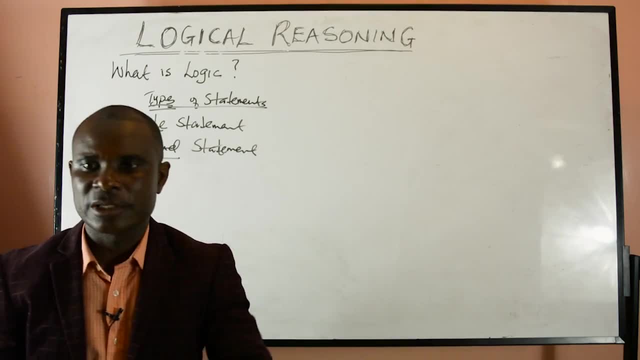 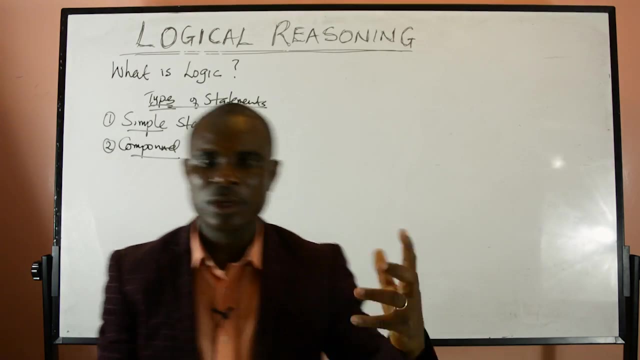 mary, is you are eager? these are single ideas, single thoughts that are conveyed in that declaration. so a simple statement only has one idea, single idea. all right, we have a compound statement. what is a compound statement? you see, it's a composite form when we put two or more simple statements together. 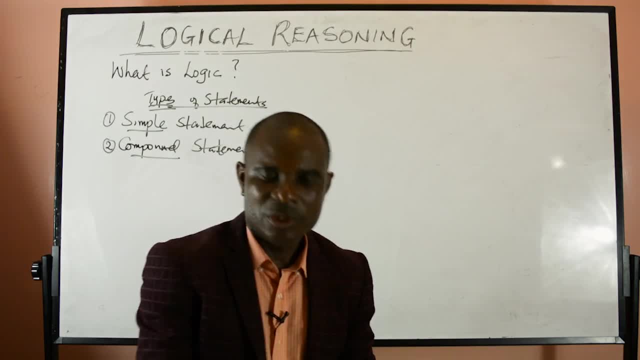 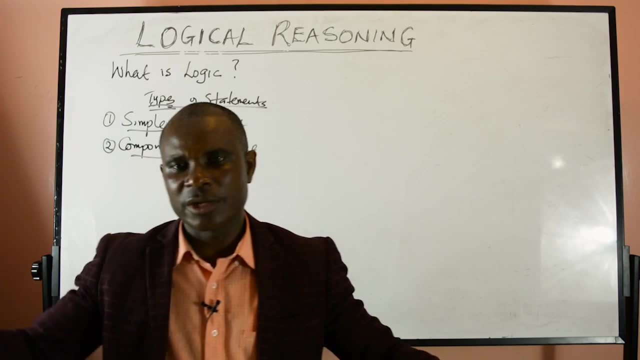 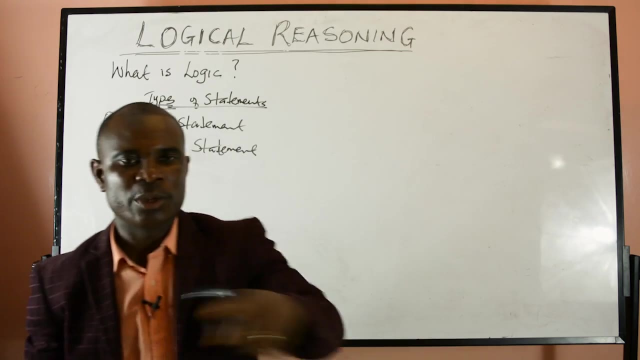 by connective terms like and but. so, for instance, if i say john is a boy and john is clever, so and has connected: john is a boy and john is clever, john is clever is a simple statement because i can touch it to draw it there. john is clever, true or false. john is a boy, true or false, i can put. 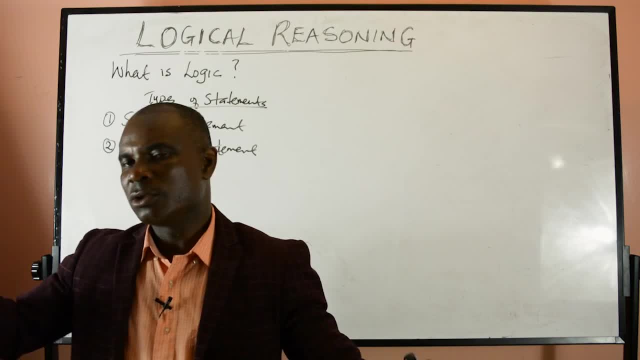 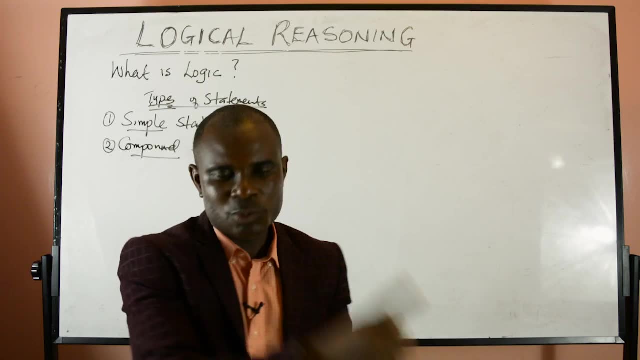 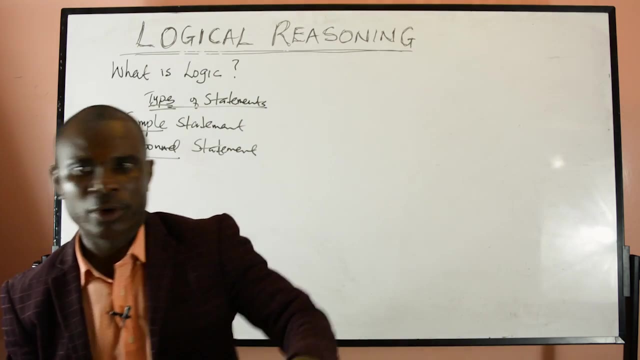 true or false on this statement. i can put true or false on the other statement here. so, but the two statements, which are simple statements, are joined together by a connective term, and that's what i just said. said john is a boy and john is clever. if i can put true value on john is a boy. 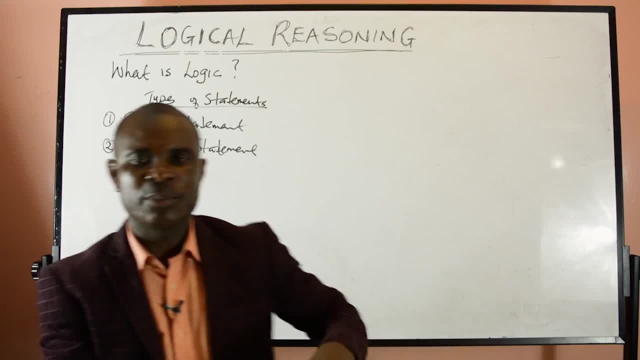 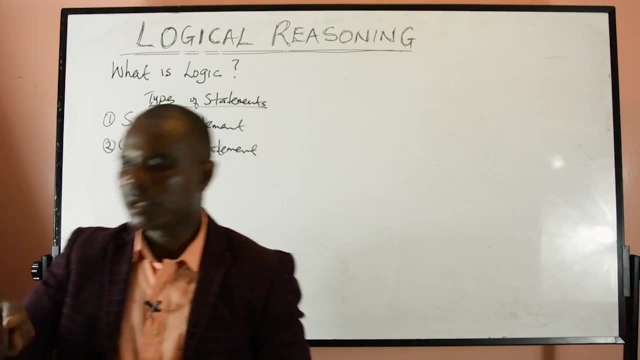 then that becomes a simple is a statement, because i can put a truth value there and it is a single state, a simple statement because it's conveying only one idea: john is a boy and the other part of that statement is: and john is clever. john is clever is another simple statement. i can put a truth value. 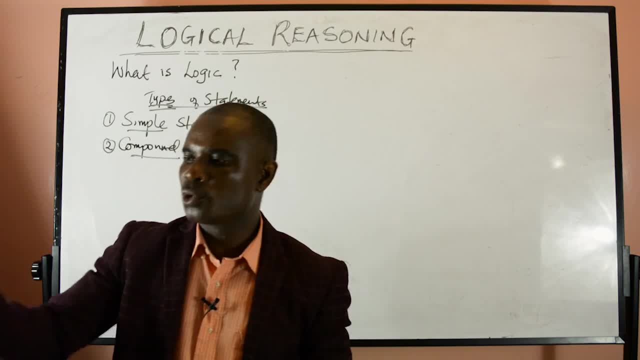 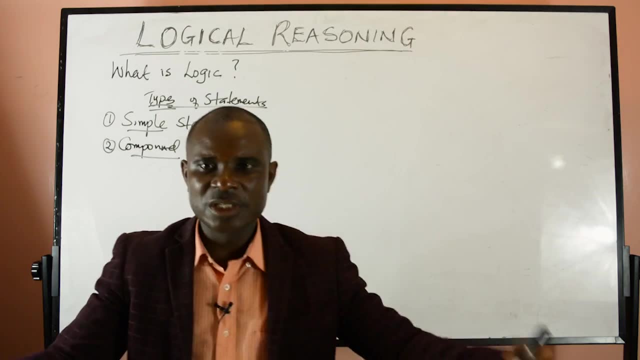 on that. i can test whether john is clever or not, so i can put true or false there. but those two statements- simple statements- are joined together by a connective term, which is end. so because i'm joining them together with a connecting term, it makes them a compound. 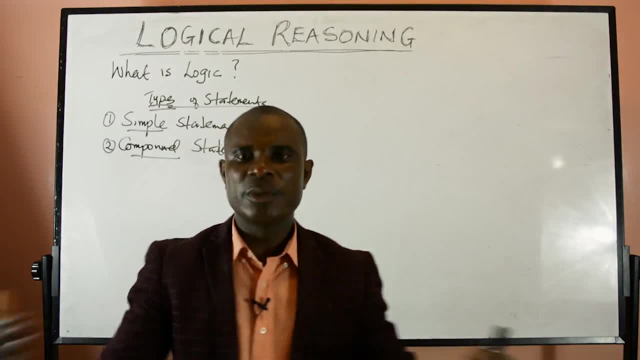 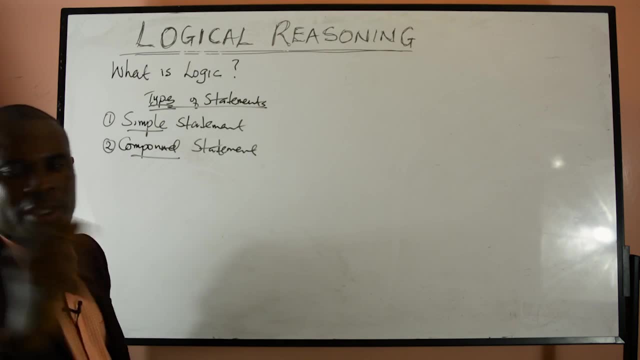 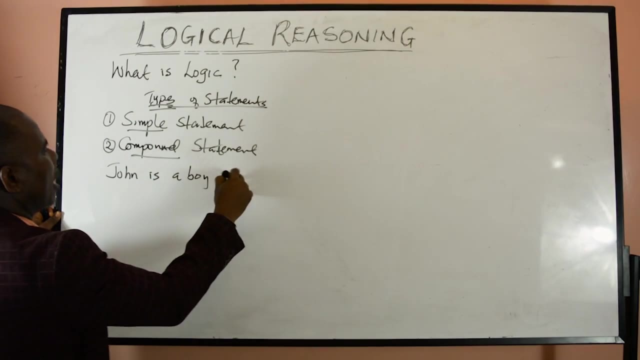 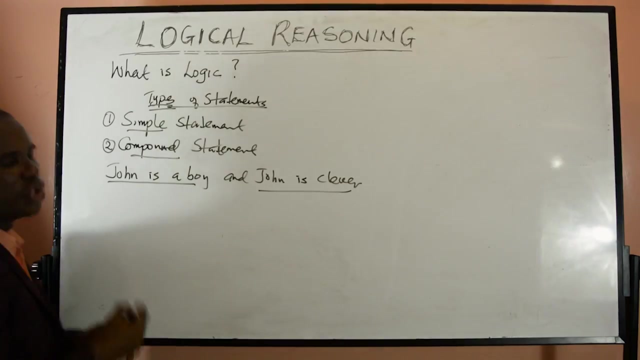 statement, because a statement is formed when two simple statements are joined together by a connective term, and this in this case. according to our example, our connective term is: and so let me just put it here you have: john is a boy, john is a boy and john is clever, john is clever, so in logic we can identify: 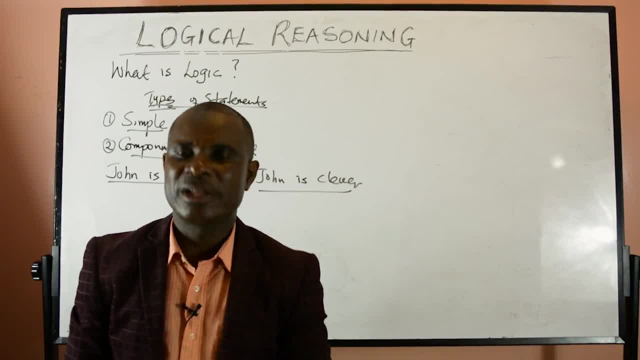 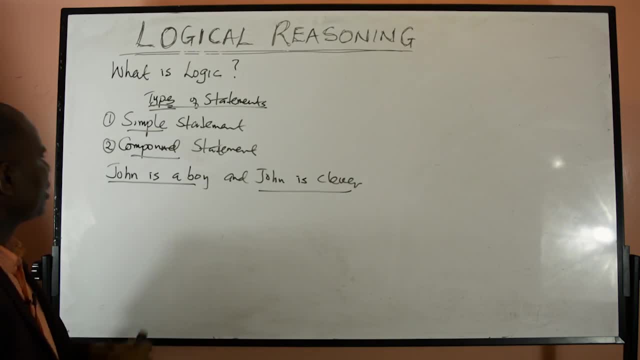 statements. we can represent six statements symbolically by letters. we normally use letters rsr, abusing pq and r here just to identify the statement. so let me call the statement p and i call the statement q. so these are two simple statements, one i can affirm whether this is true or 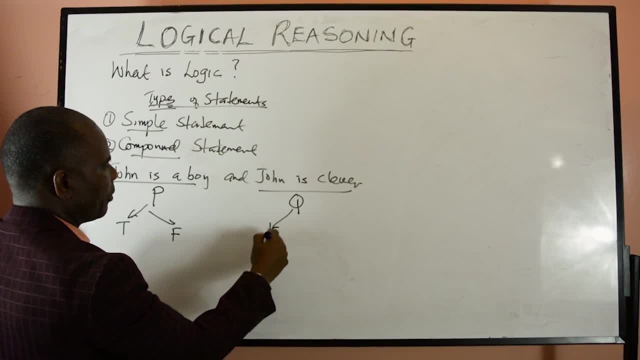 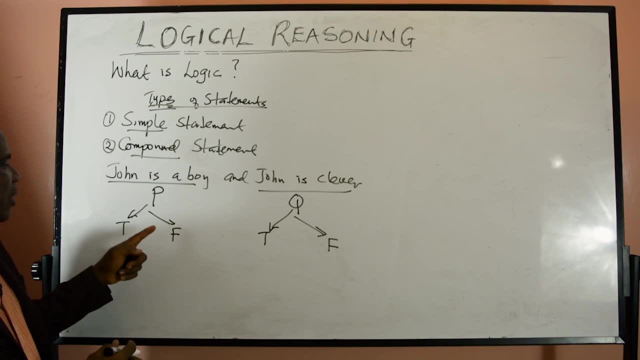 false. i can put true or false value here. here also i can put true or false value here. so, for as much as i can identify whether john is true, john is a boy by putting truth value. if john is actually a boy, then misstatement, which is a simple statement, is true. but if i look at john and john is not a boy, 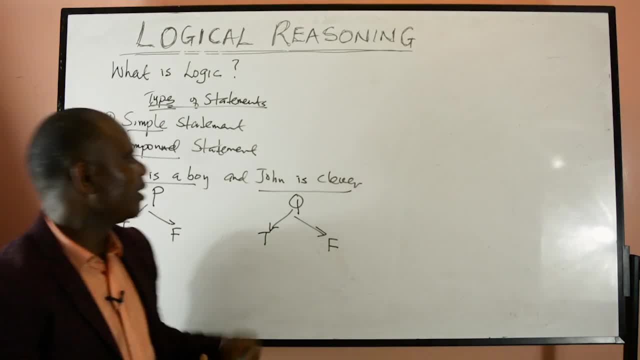 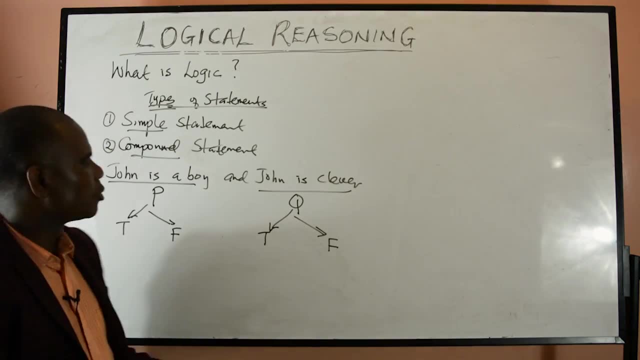 that statement is a false. now we look at the other part of this statement. if john is clever- actually know that, i prove that john is clever- then it's a truth statement. but if john is not clever, that becomes false. so this part of the statement i can put through to true there, or? 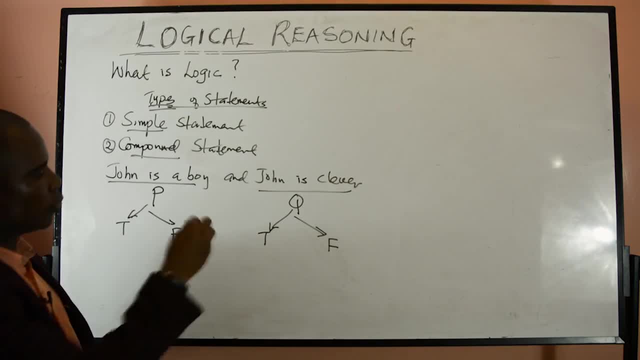 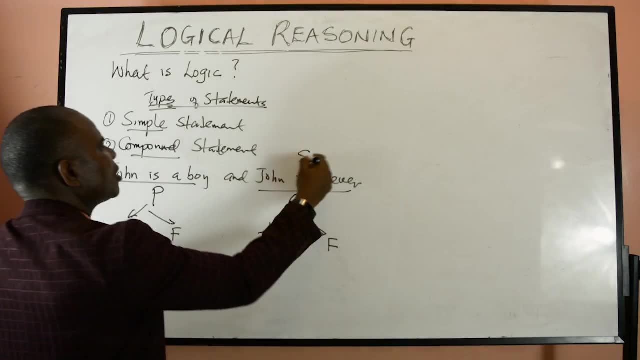 force. there i can identify the true. it true to value, which is true and false. here also i can identify a truth, value which is true and false. when, once i can put two simple statements, this is simple statement two and simple statement one, if you like. this is simple statement one. 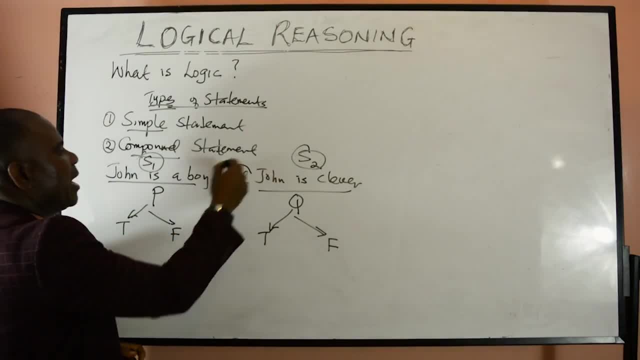 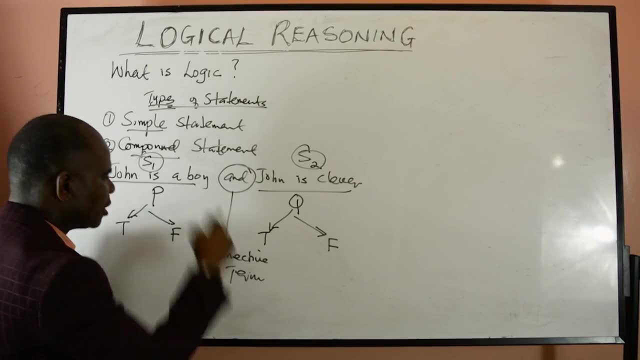 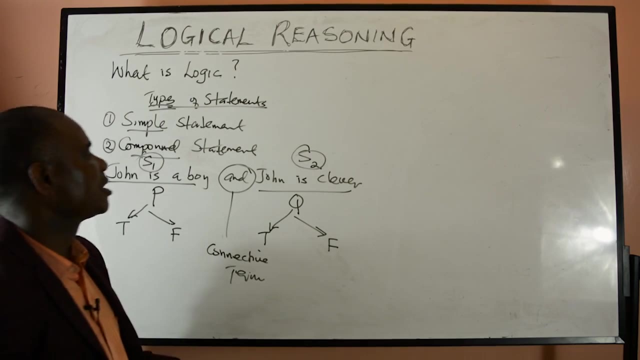 when i put two or more simple statements together by a connective term, this is a connective term. in that last thing this is a connective term. in this case it's, and for as much as i agree the two simple statement to give me a connect, a compound statement, then i can call this whole statement. 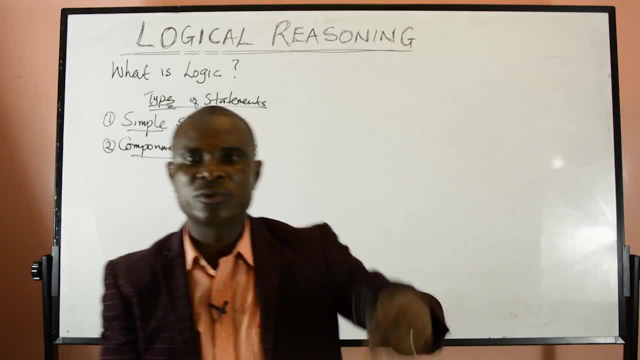 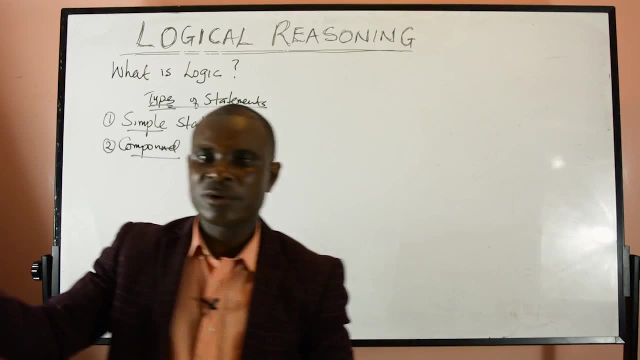 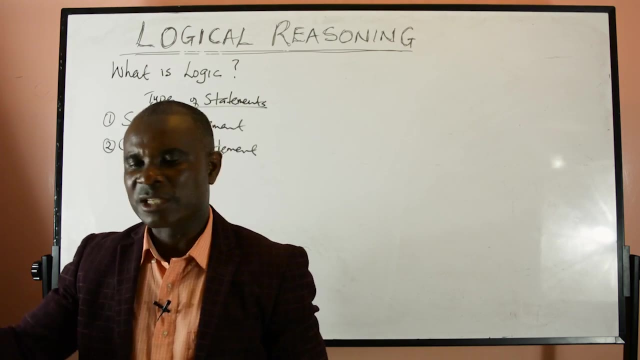 becomes a simple is a statement because i can put a truth value there and it is a single state. a simple statement because it's conveying only one idea: john is a boy and the other part of that statement is: and john is clever. john is clever is another simple statement. i can put a truth value on that. 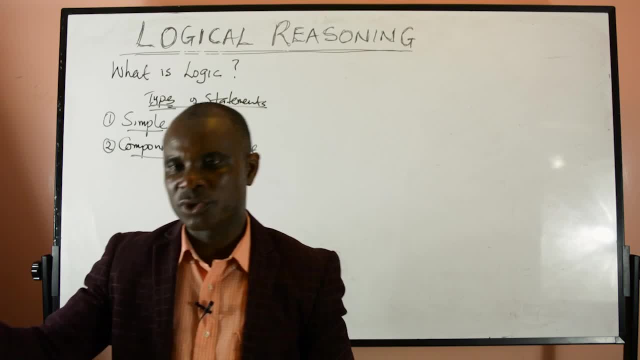 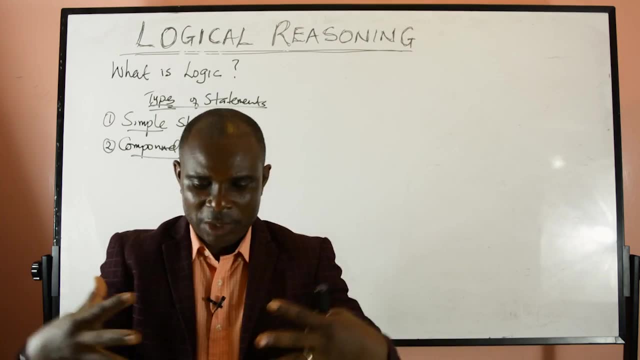 i can test whether john is clever or not, so i can put true or false there. but those two statements- simple statements- are joined together by a connective term, which is end. so because i'm joining them together with a connective term, it makes them a compound statement, because a 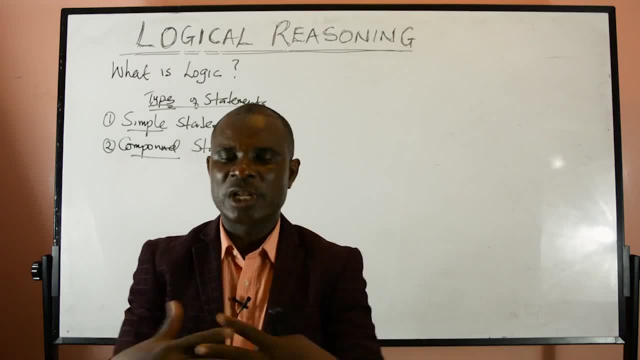 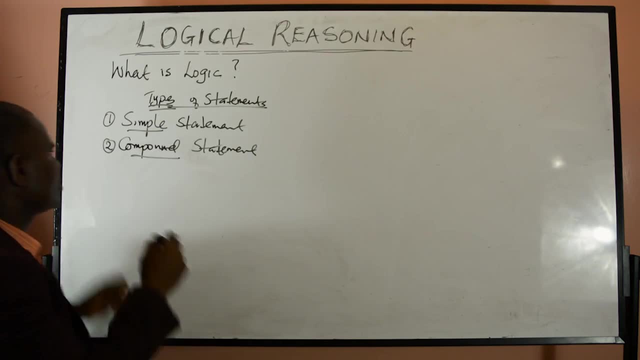 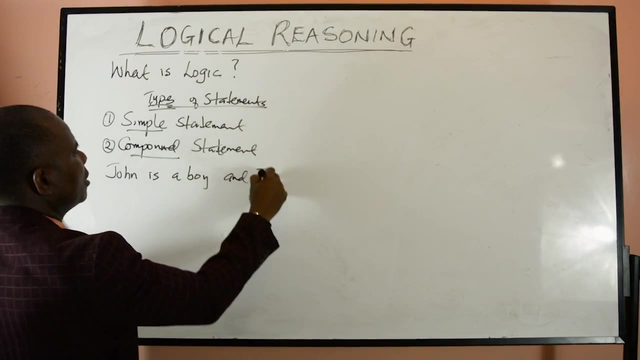 compound statement is formed when two simple statements are joined together by a connective term and in this case, according to our example, our connective term is: and so let me just put it here you have: john is a boy, john is a boy and john is clever. john is clever, so in logic we can: 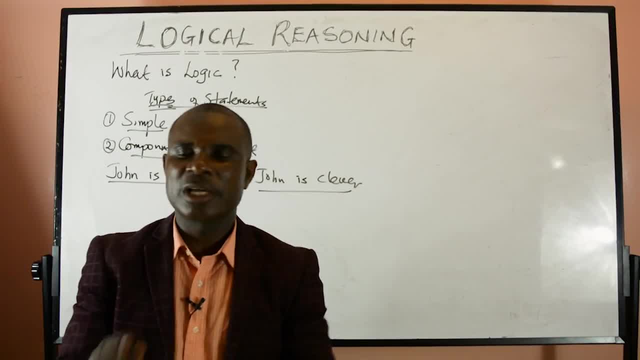 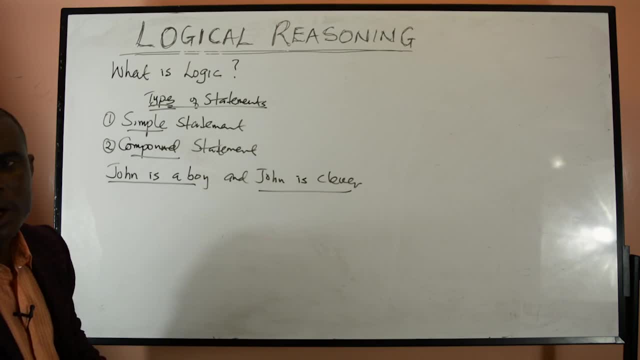 identify statements. we can represent six statements symbolically by letters. we normally use letters like p, p, p, qr, so i'll be using pq and r here just to identify the statement. so let me call this statement p and i call this statement q. so these are two simple statements, one i can affirm whether this 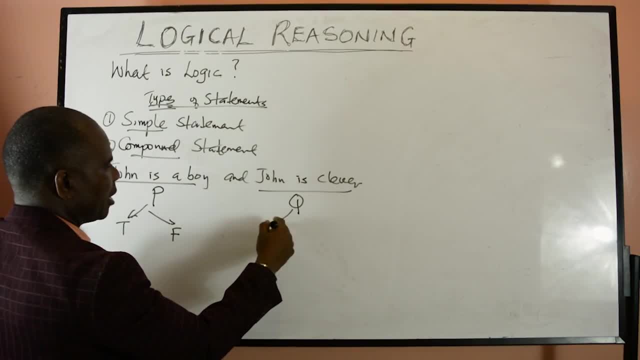 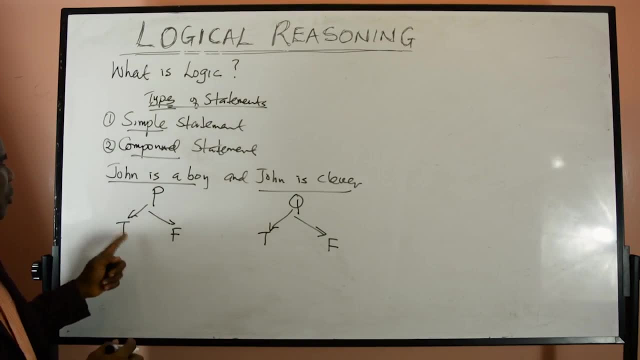 is true or false. i can put true or false value here. here also, i can put true or false value here. so, for as much as i can identify whether john is true, john is a boy by putting truth value. if john is actually a boy, then misstatement, which is a simple statement, is true. but if i look at john, 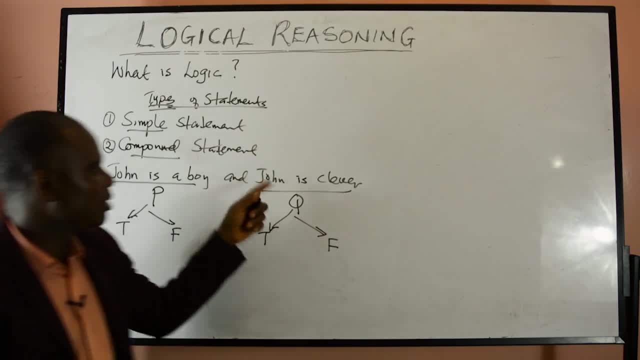 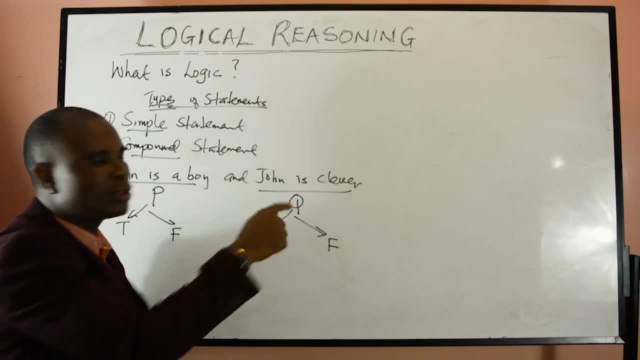 and john is not a boy, then that statement is a force. now we look at the other part of this statement. if john is clever- actually know that, i prove that john is clever- then it's a truth statement. but if john is not clever, that becomes false. so this part of the statement i can put. 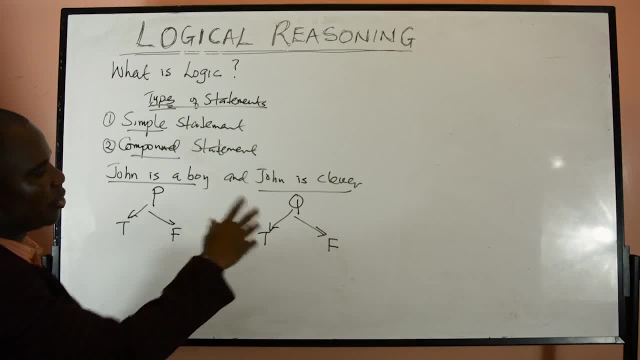 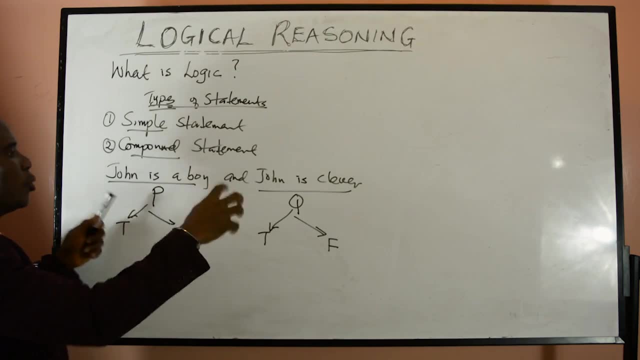 through two true, there are force. there i can identify the true truth value which is true and false. here also, i can identify a truth value which is true and false, when once i can put two simple statements. this is simple statement 2 and simple statement 1, if you like. this is simple statement. 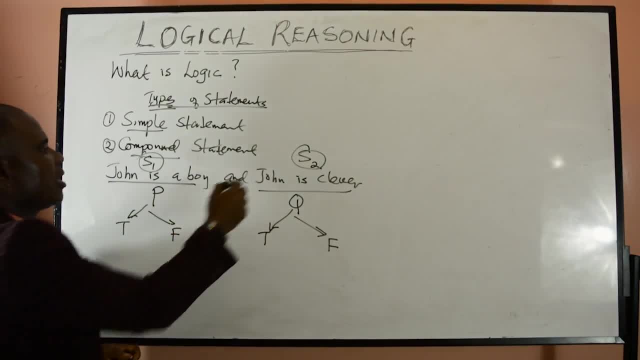 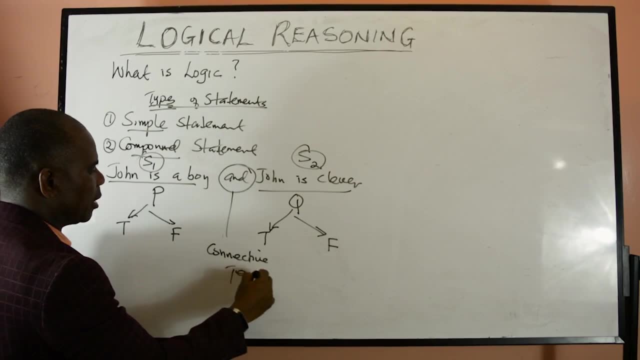 1. When I put two or more simple statements together by a connective term, this is a connective term in that thing. This is a connective term. In this case it's and, For as much as I can do, the two simple statements to give me a compound statement. 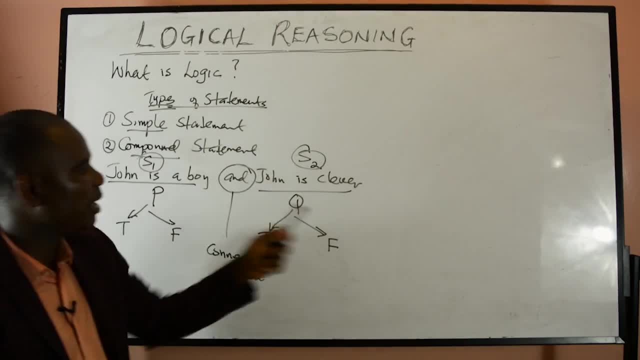 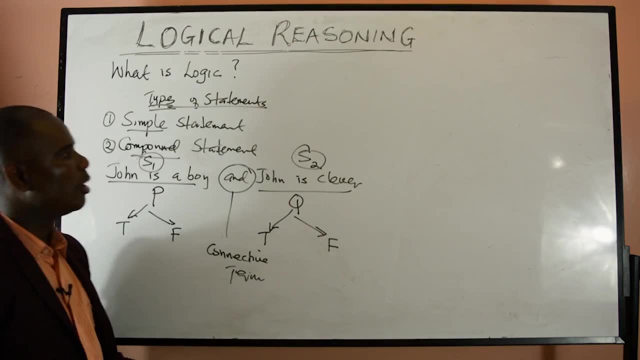 then I can call this whole statement from John here to Clever. It's called a compound statement because it's putting two simple statements together to form a compound statement, And I now know that you can distinguish between a simple statement and a compound statement. 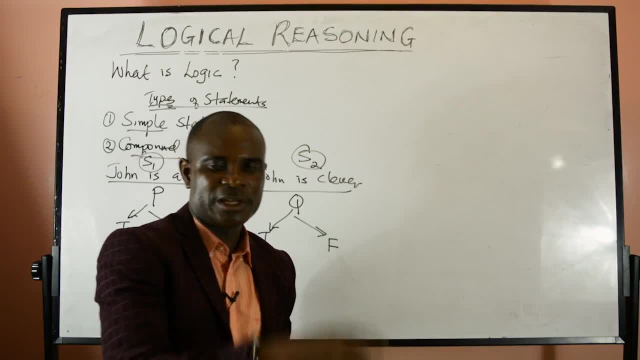 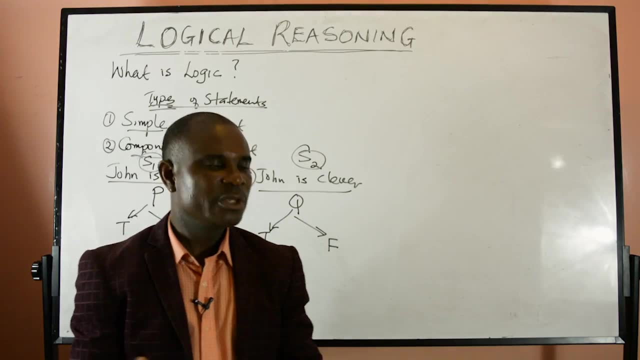 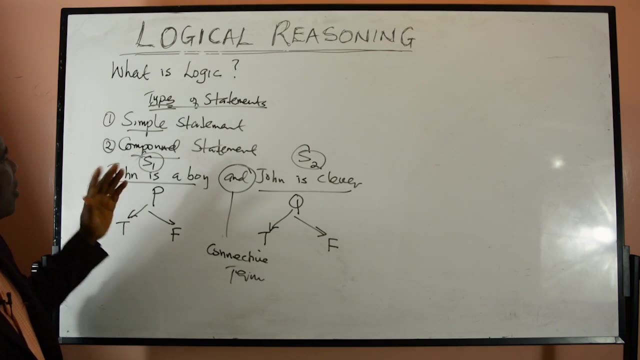 A simple statement conveys a single idea or one idea, and a compound statement is putting together a combination of two or more simple statements to form a compound statement, So we can attach truth values on each one of the simple statements. Now we can proceed with the types of compound statements. 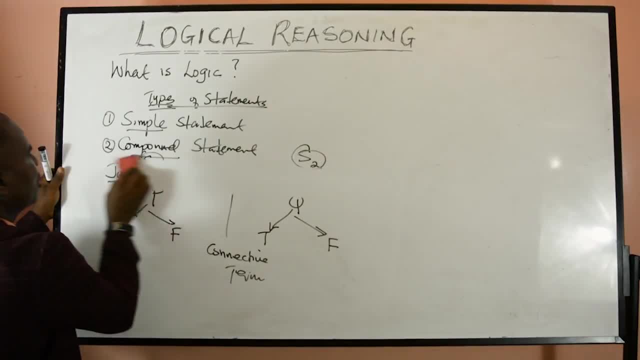 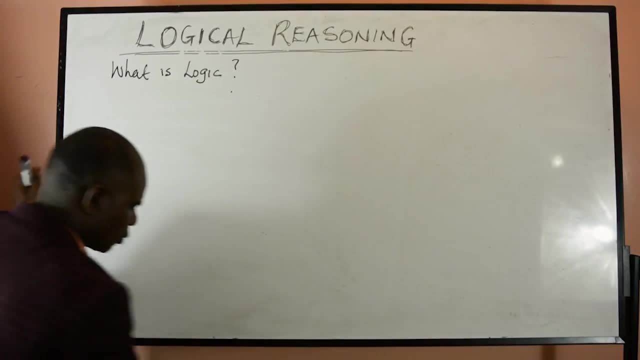 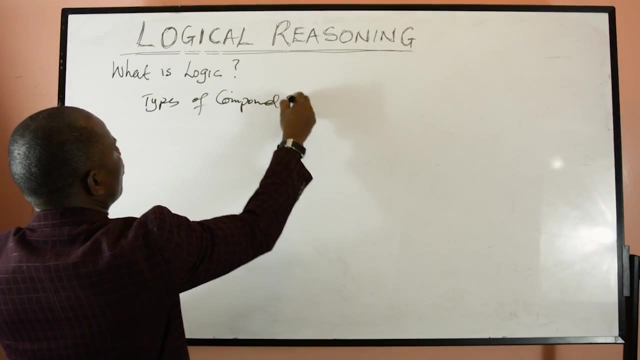 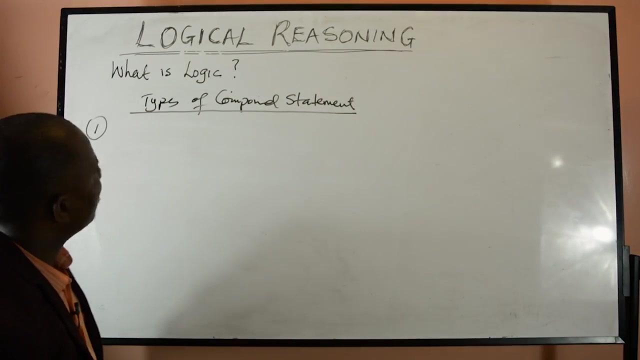 Let me just move with this. I have already established simple statements and compound statements. Now I want to look at compound statements in detail Here. So we look at what is the types of compound statements. Types of compound statements: Yes, we have first type of compound statement. 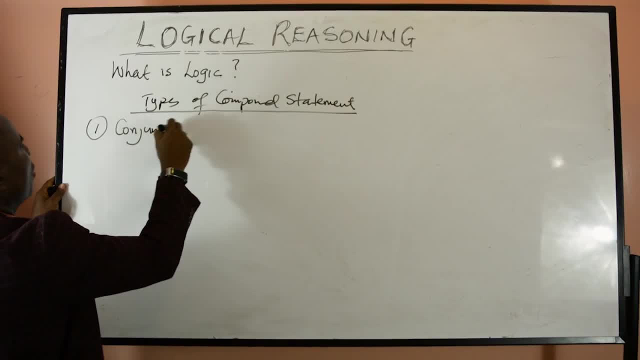 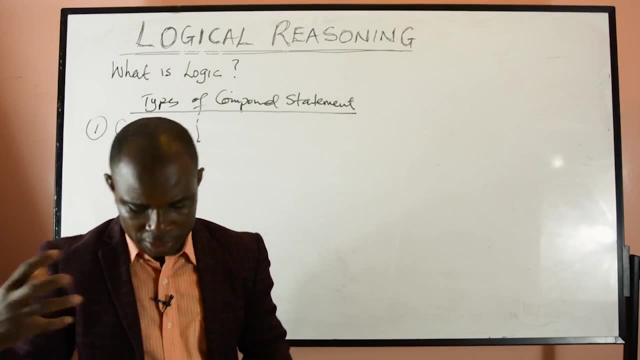 It's called a conjunction. What is a conjunction? A conjunction is a compound statement that is put together or joined together- simple statements joined together by a connective term. So If I'm forming a compound statement, I should put two or more simple statements. 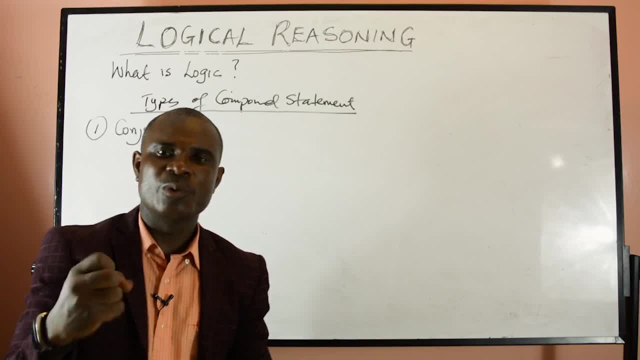 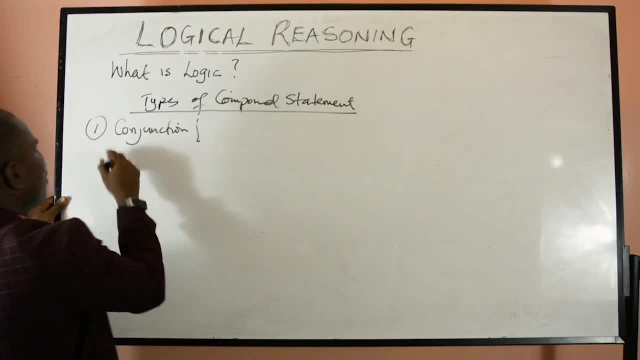 But in the process of putting a simple statement together, if I use the word and or but, then I'm looking at a conjunction. A conjunction is identified, let's say, from our previous example. Let me just write: say John is a boy. 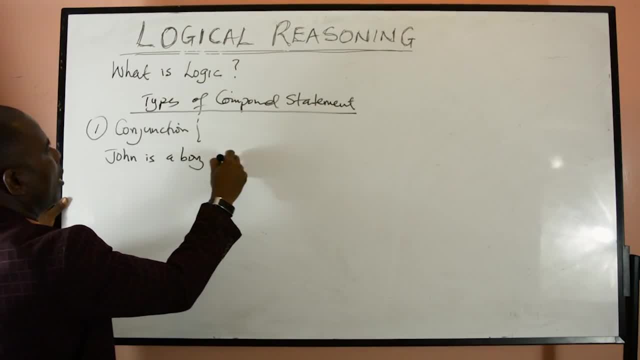 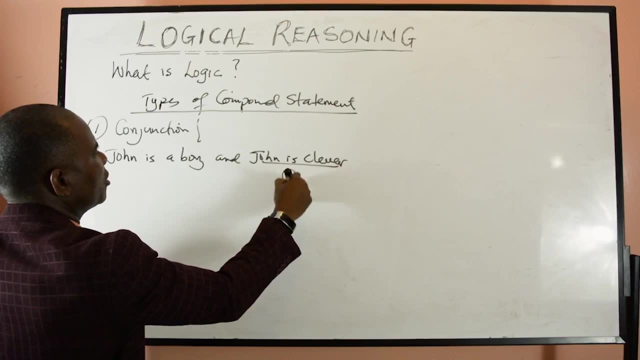 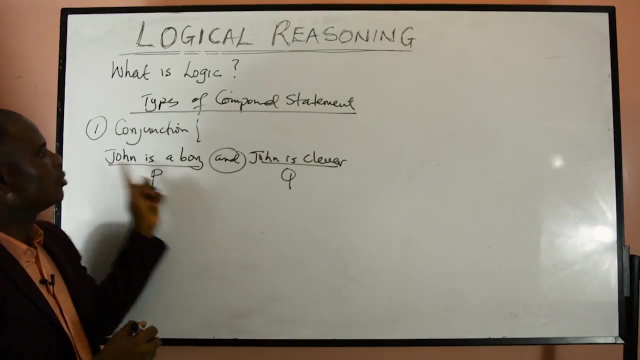 John is a boy And John is clever. So here I have the statement Q, I have the simple, I have the simple statement P, But it is joined together by and So, for as much as I'm connecting the two simple statements with the connective term and 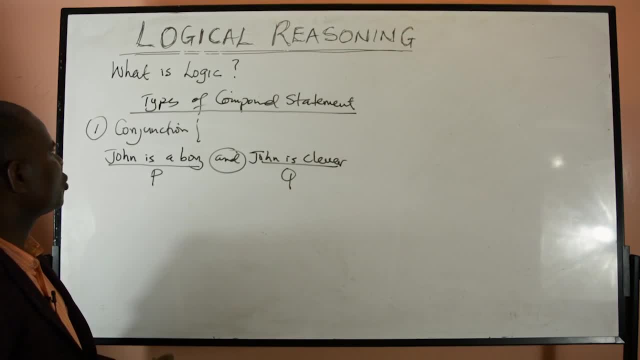 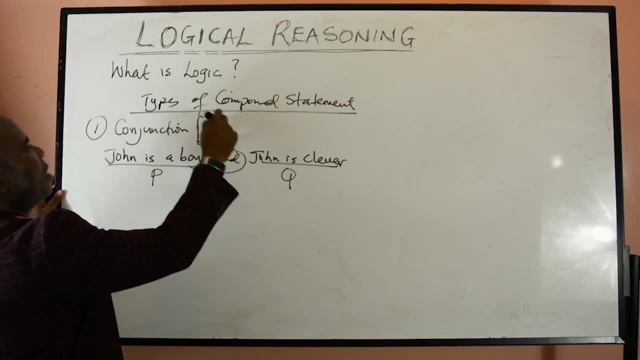 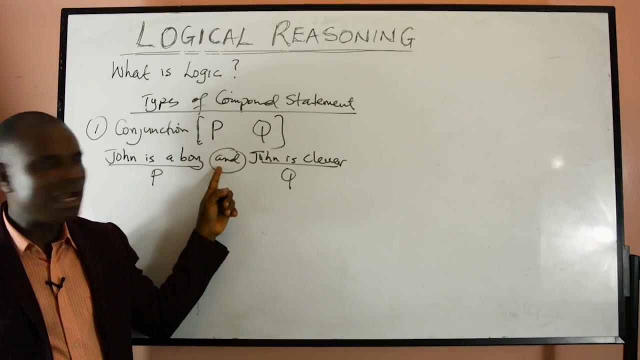 then it becomes a conjunction. That's a type of compound statement called a conjunction. So let me put them in symbolic terms. This statement is represented by P And this statement is represented by Q. So to represent it symbolically, I can represent and as obverse. 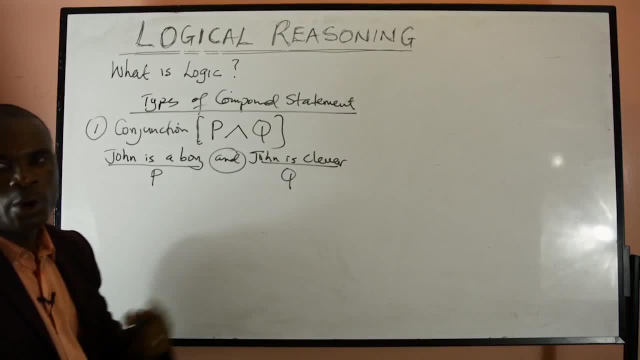 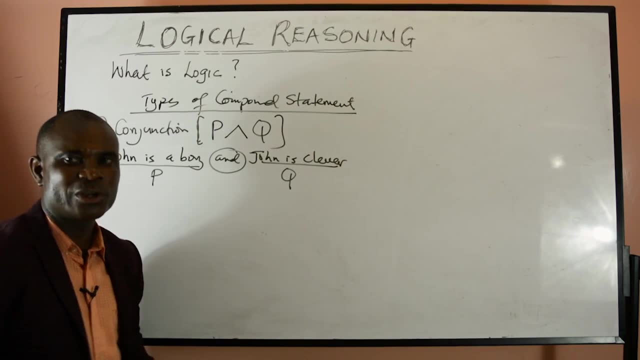 That is the inverse of V: V upside down, That is obverse, Obverse symbol, which is, and in terms of set theory, It's the same interpretation as set theory When we say A intersection B, That is A and B, Or P and Q. 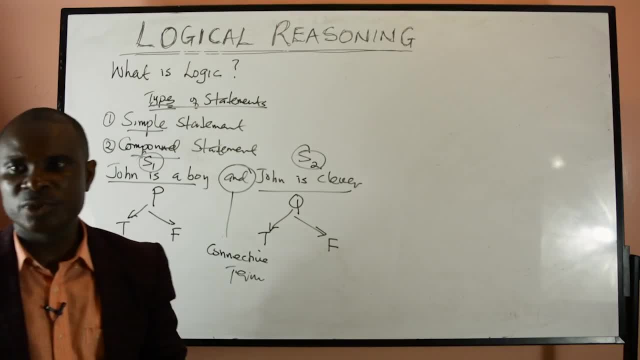 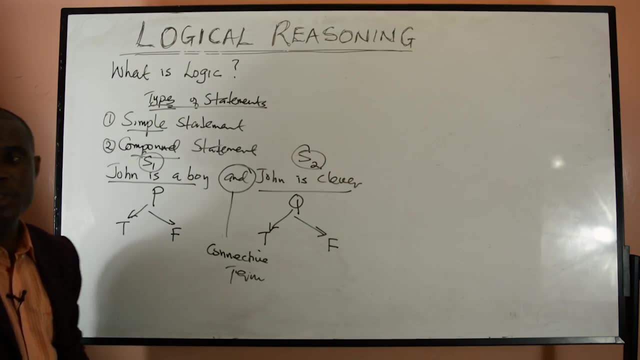 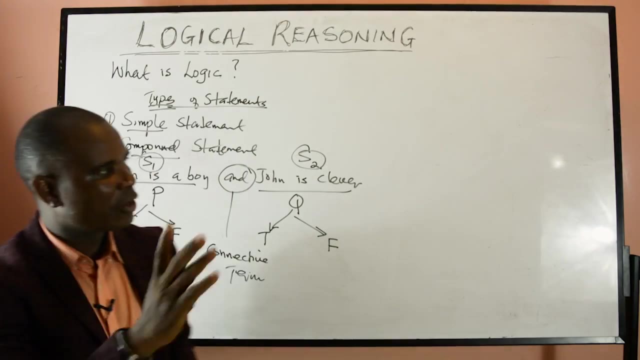 from john here to clever, it's called a compound statement because it's putting two simple statement together to form a compound statement, and i i now um know that you can distinguish between a simple statement and a compound statement. a simple statement convey a single idea, or one idea, and a compound statement. 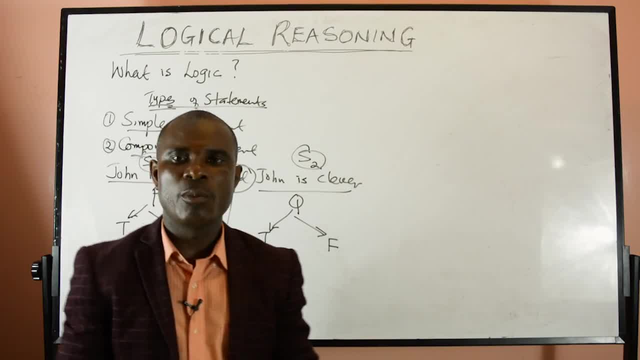 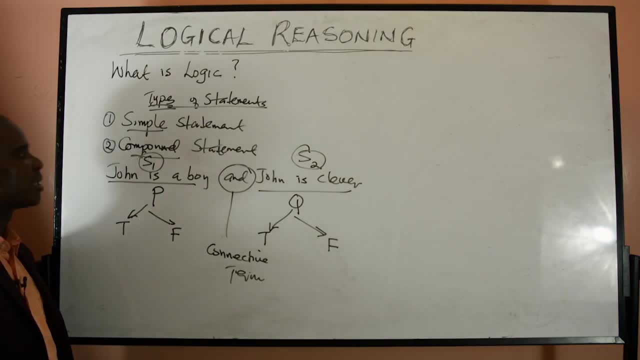 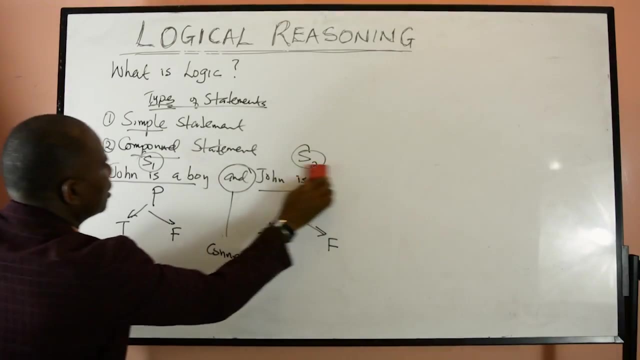 is a putting together or combination of two or more some simple statement to form a compound statement, so we can attach truth values on each one of the simple statements. now we can proceed with the types of compound statements, so let me just move with this. i have already established. 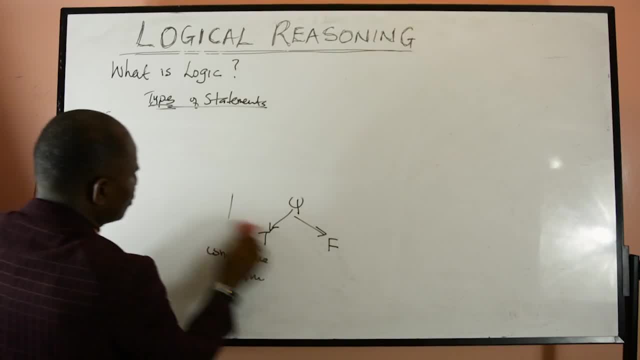 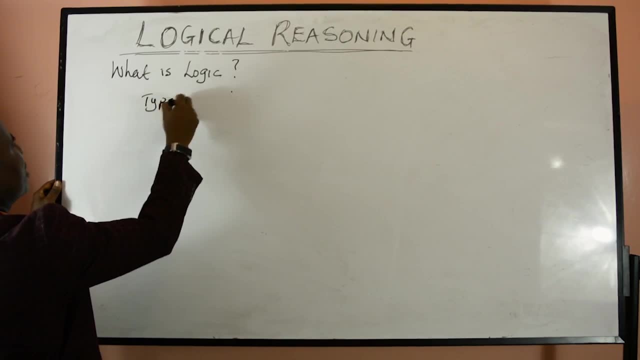 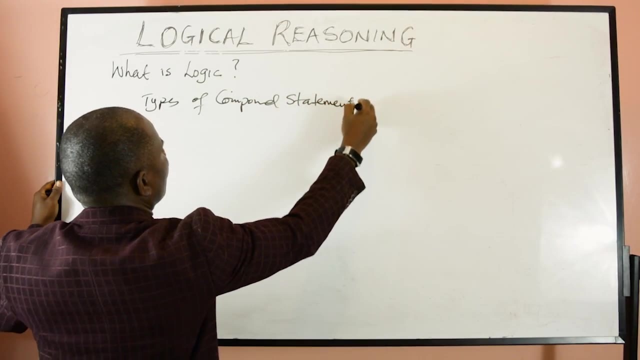 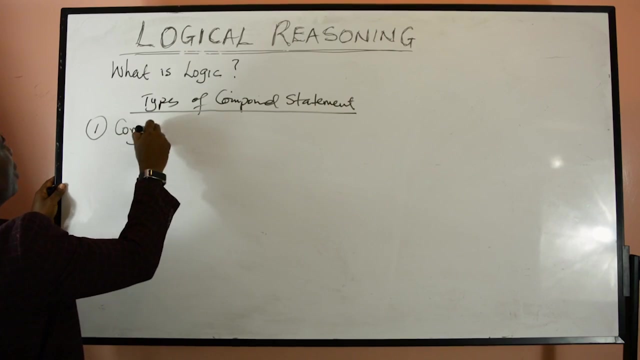 simple statements and compound statements. now i want to look at compound statements in details here. so we look at what is the types of compound statement. types of compound statements: yes, we have. first type of compound statement is called a conjunction. what is a conjunction? a conjunction is a compound statement. 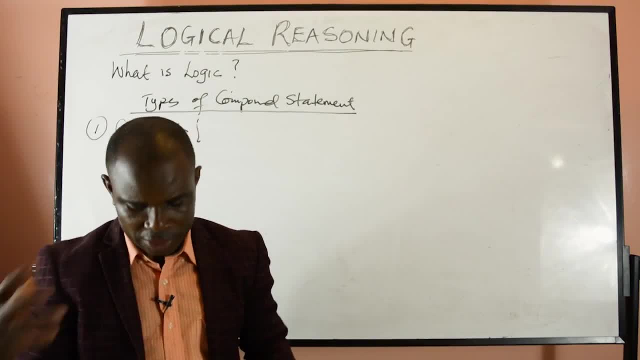 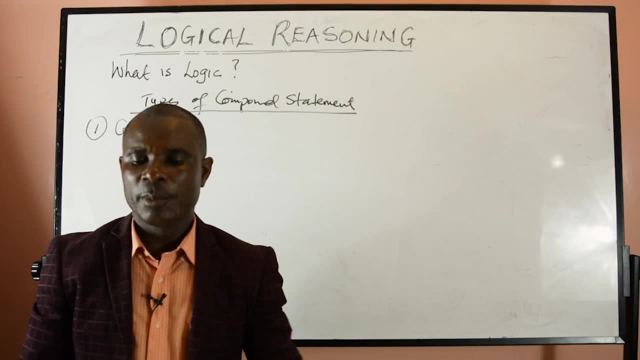 that is, put together or joined together. simple statements joined together by a connective term. so if i'm forming a compound statement, i should put two or more simple statements. but in the process of putting a simple statement together, if i use the word and or but, then i'm looking at a 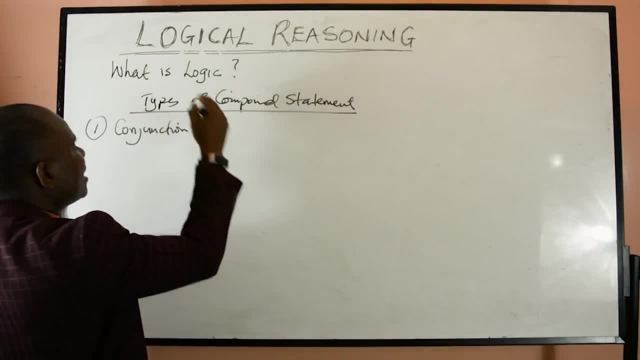 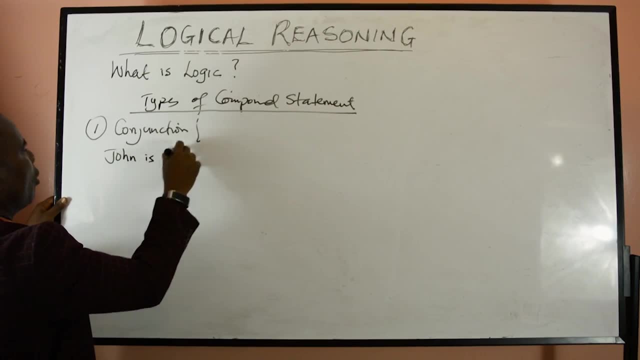 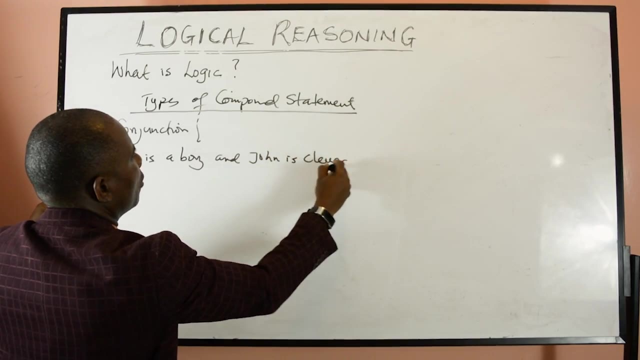 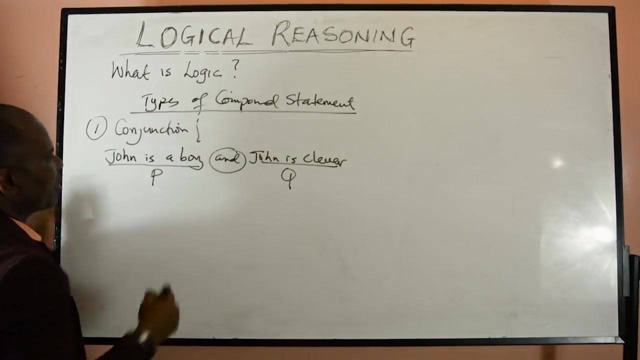 conjunction. a conjunction is is identified. let's say, from our previous example, let me just write: say: john is a boy, john is a boy and john is clever. so here i have the statement q, i have the simple statement p, but it is joined together by and so, for as much as i'm connecting the two, 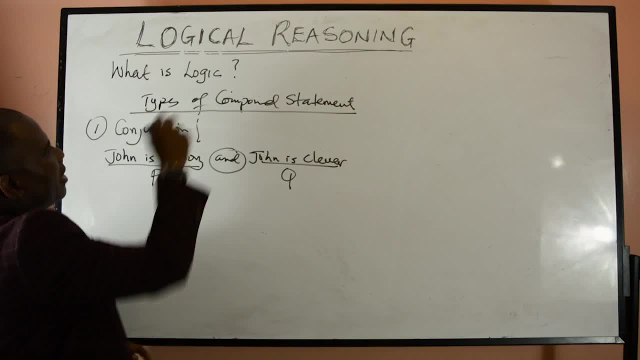 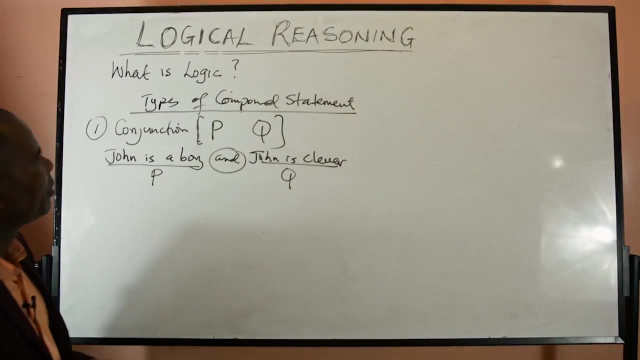 simple statements with the connective term and then it becomes a conjunct in your conjunction. that's the type of compound statement called a conjunction. so let me put them in symbolic term. this statement is represented by p and this statement is represented by q. so to represent it symbolically, i can represent: and as upward, that is the inverse of v. 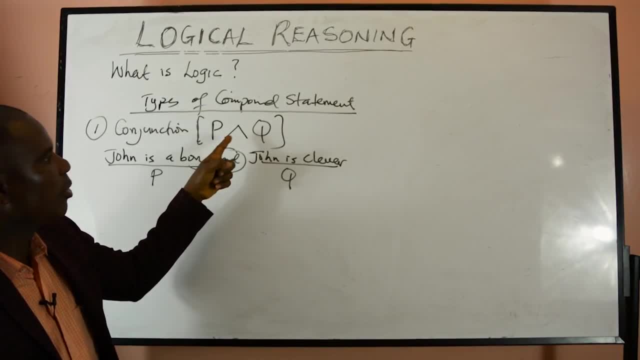 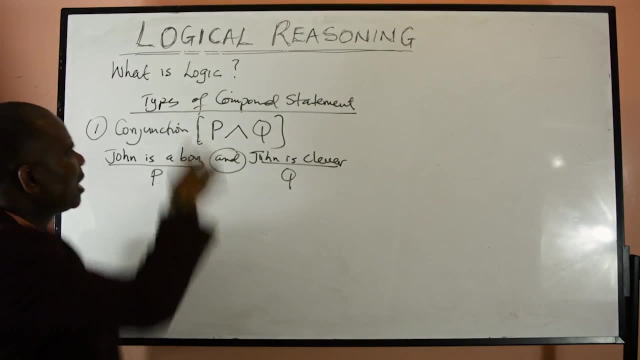 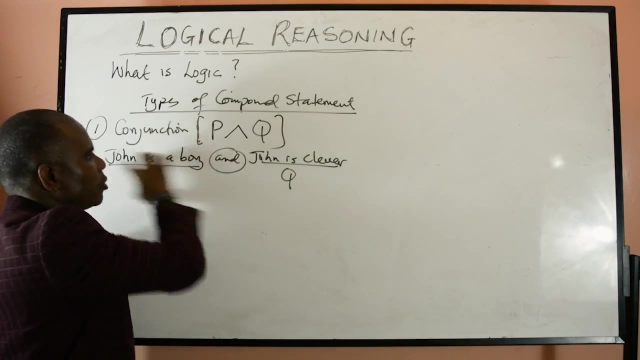 the opposite symbol, which is- and in terms of set theory it's the same interpretation as set theory. when we say a intersection b, that is a and b or p and q. so john is a boy is p and john is clever is q. so this whole sentence can be symbolically represented as p of vat, q. so that is the first type of compound. 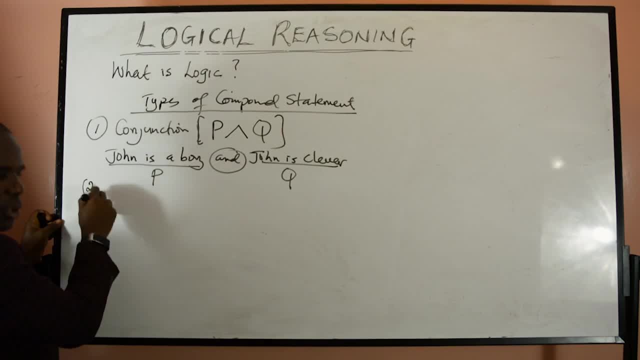 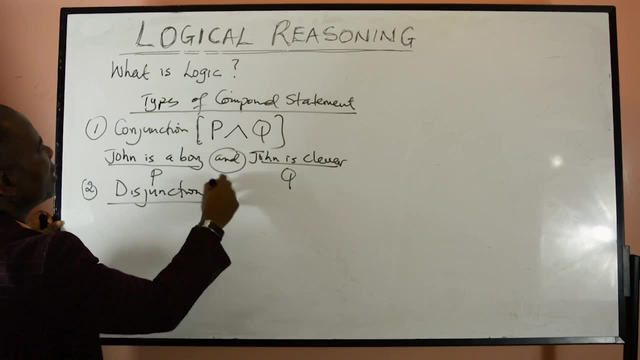 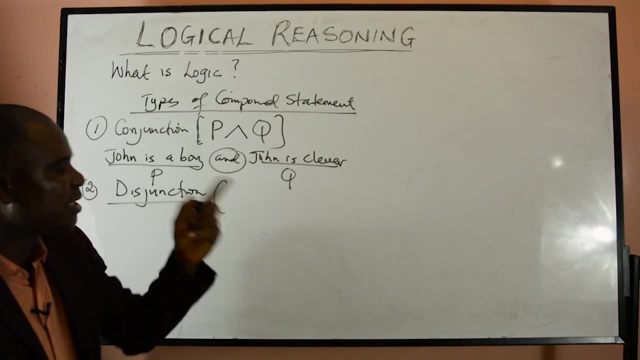 statement is called conjunction. so we go to the second time. the second type of statement is the disjunction. what is a disjunction? a disjunction is a compound statement that is also put together by it's two. it's two com- a simple statement put together to form a compound statement, but this time 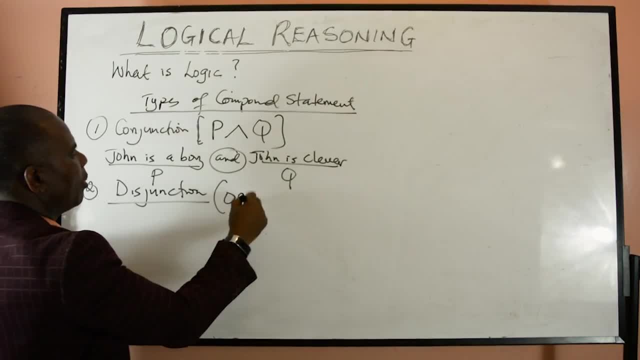 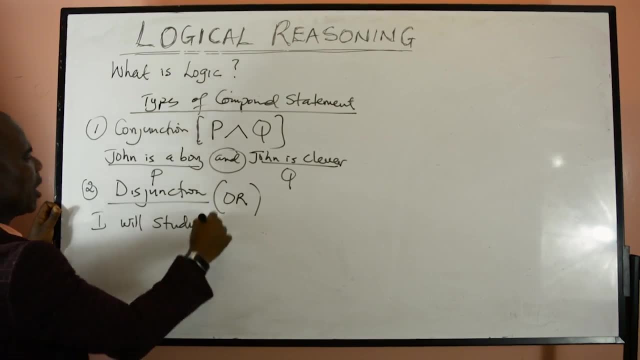 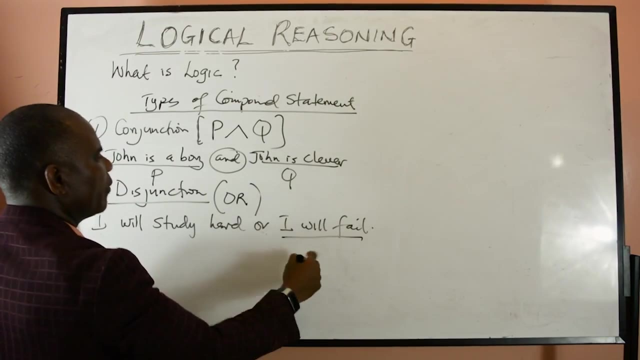 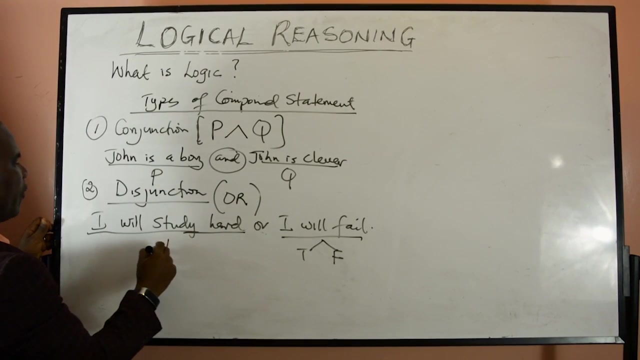 the connective term is all it is by connecting the time. oh so let's say: i will, i will study hard. i will study hard or i will feel so. here i will feel i can put true or false in that i will feel true of us. here i can also put: i will study hard through of us, true of us, but this time. 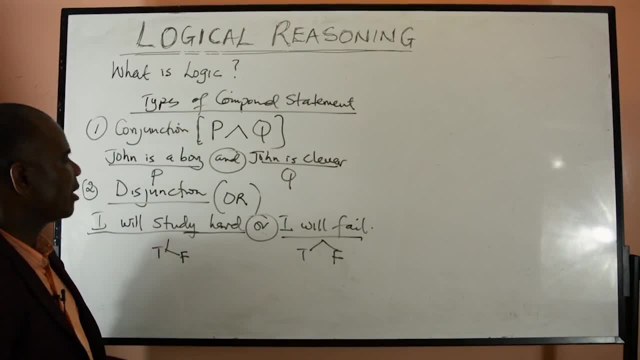 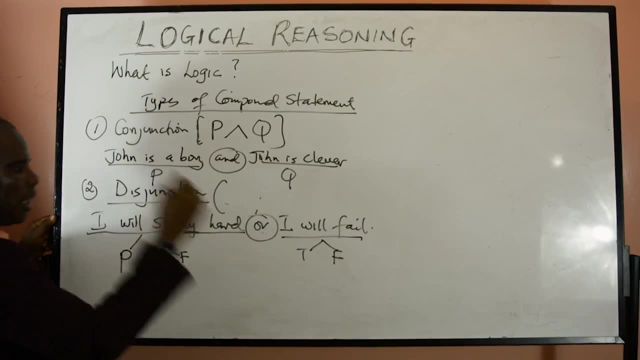 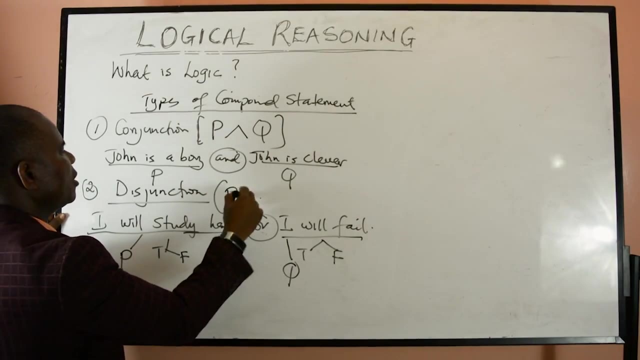 it is. this compound statement is put together by a connective term or so, or is this: if i can represent this statement as p and also represent this as q, then to represent the whole statement as a compound statement, disjunction is p invert q. this time it is inverse. this is like union in such 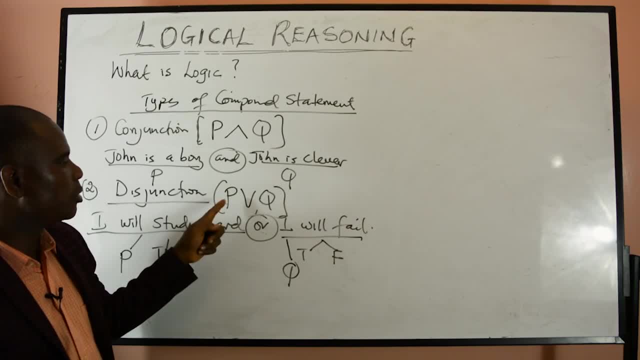 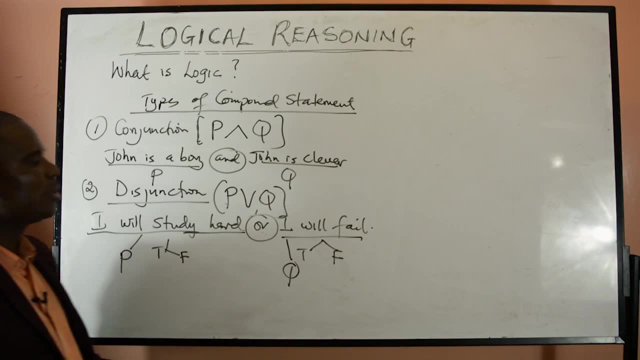 a is u or is p or q. in other words, p union q. this is invert. invert is the symbolic representation of disjunction. for disjunction, the, the compound statement, is put. the two simple statements are put together to form a compound statement by joining them with the word or when. i do that: 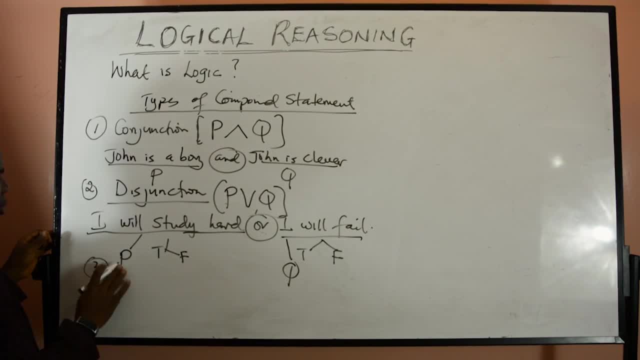 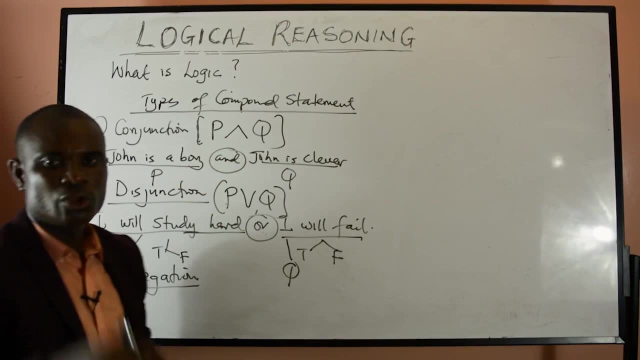 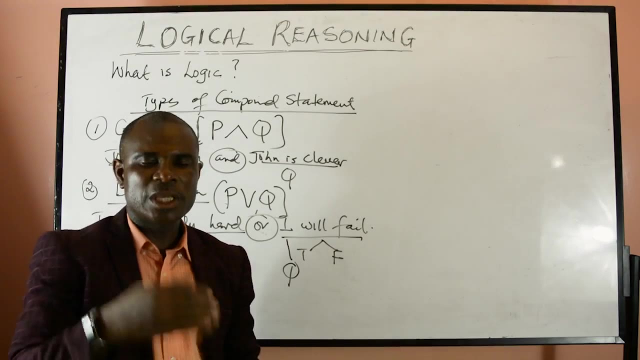 i'm forming a disjunction. let's go to the total type. the total type is negation. what is negation is from by inserting not inside for the principal statement. the first statement is if. if i insert not inside the statement, it means i'm negating the statement. for instance, if i say p is, 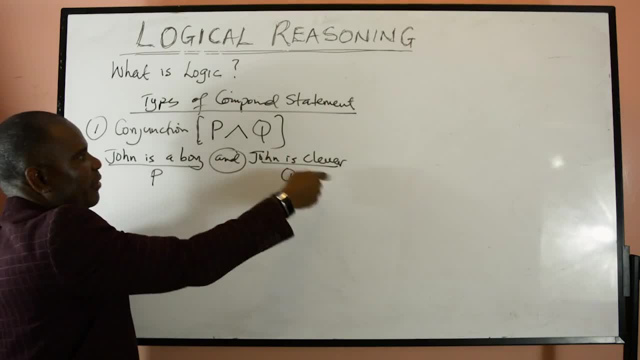 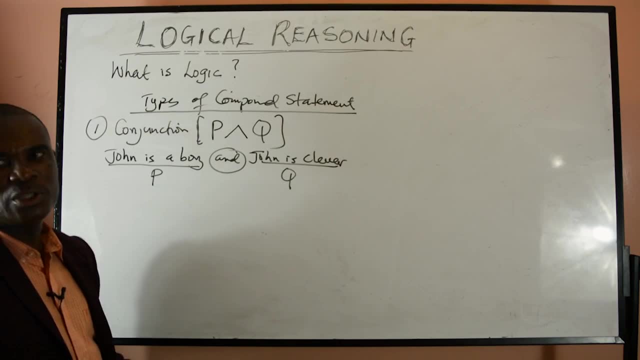 So John is a boy is P And John is clever is Q. So this whole sentence can be symbolically represented as P obverse Q. So that is the first type of compound statement. It's called conjunction. So we go to the second type. 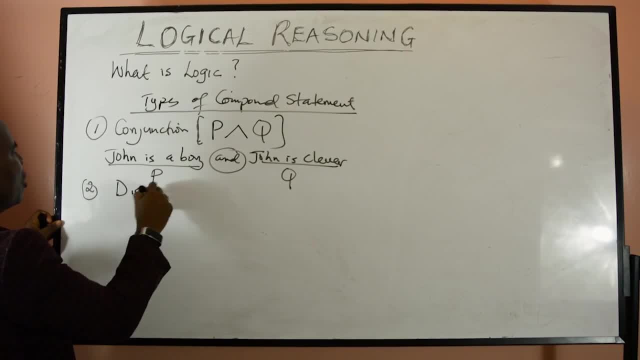 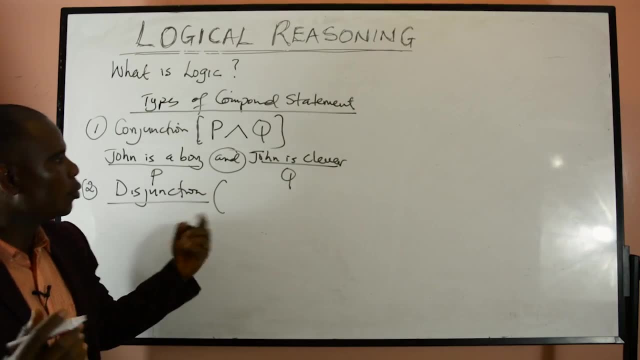 The second type of statement is the disjunction. What is a disjunction? A disjunction is a compound statement That is also put together. It's two simple statements put together to form a compound statement, But this time the connective term is O. 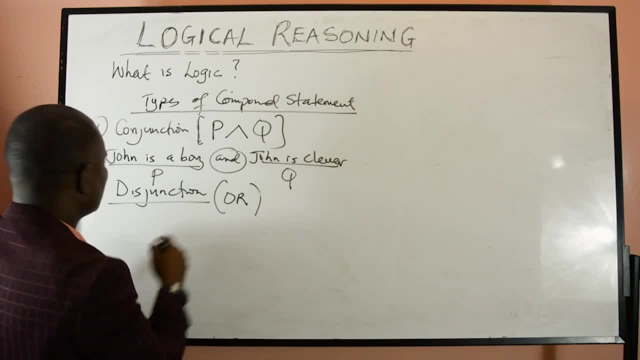 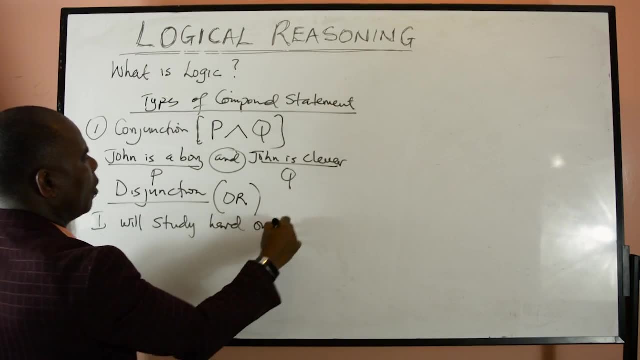 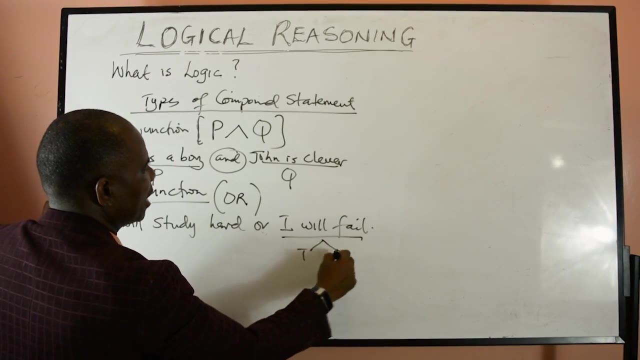 It is by connecting the term O. So let's say: I will study hard. I will study hard Or I will fail. So here I will fail. I can put true or false in that I will fail. True or false. Here I can also put: I will study hard. 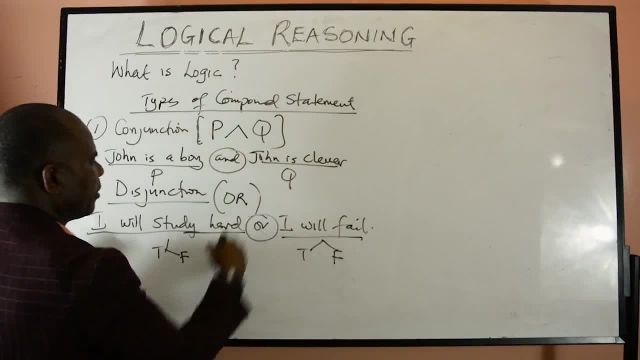 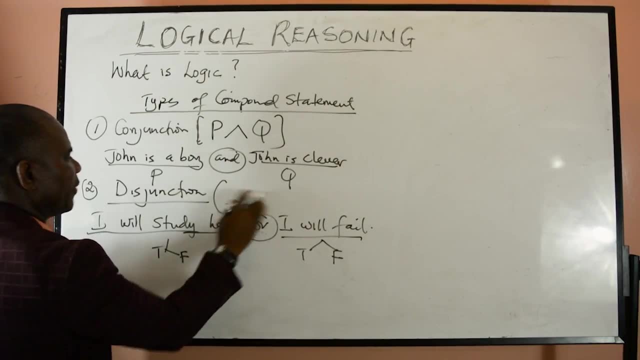 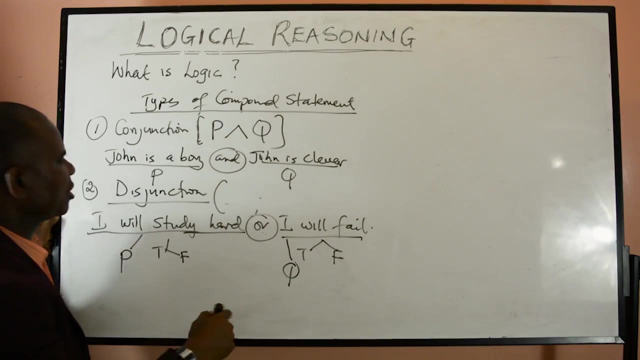 True or false, But this time it is. This compound statement is put together by a connective term, O. So O is, If I can represent this statement as P And also represent this as Q, Then to represent the whole statement as a compound statement. disjunction. 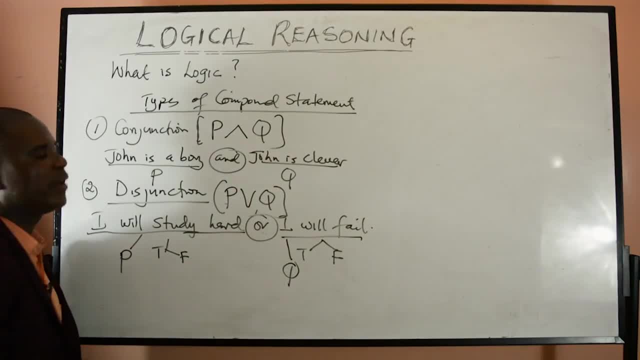 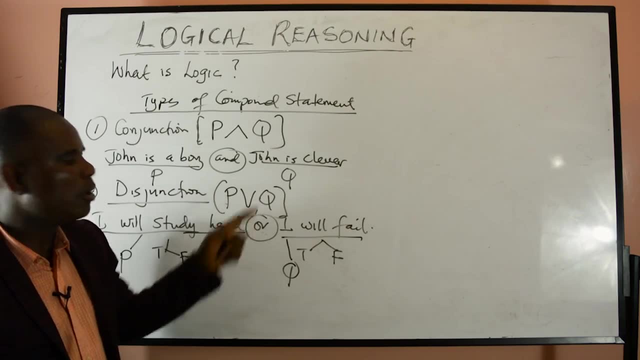 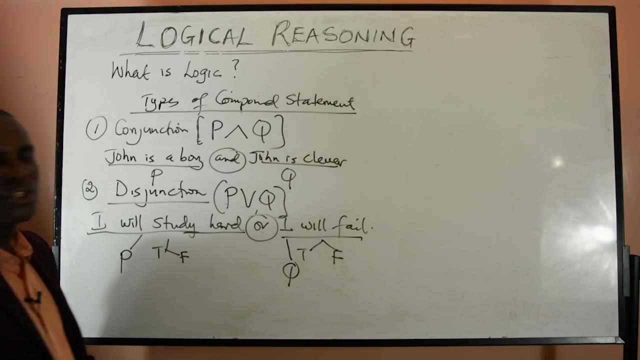 Is P inverse Q. This time it is inverse. This is like union in set theory: A is U or It's P or Q. In other words, P union Q. This is inverse. Inverse is the symbolic representation of disjunction. 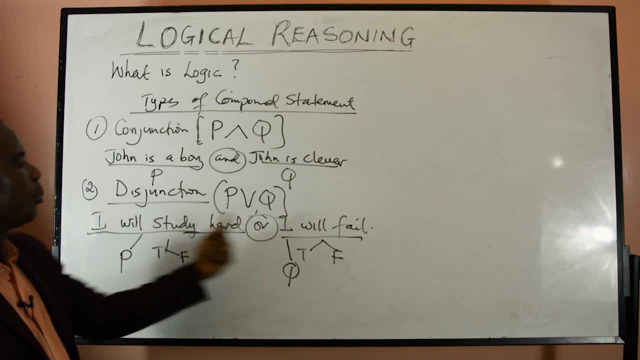 For disjunction, The compound statement is put. It's: two simple statements are put together To form a compound statement By joining them with the word O. When I do that, I am forming a disjunction. Let's go to the third type. 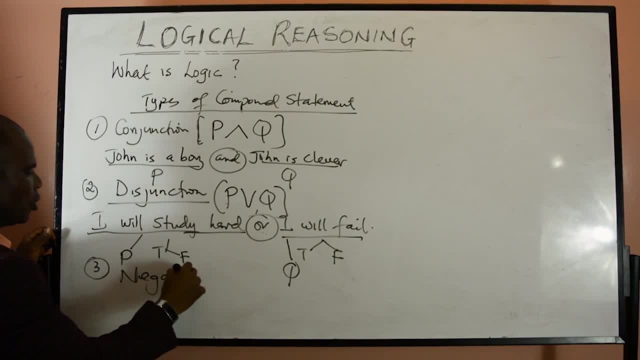 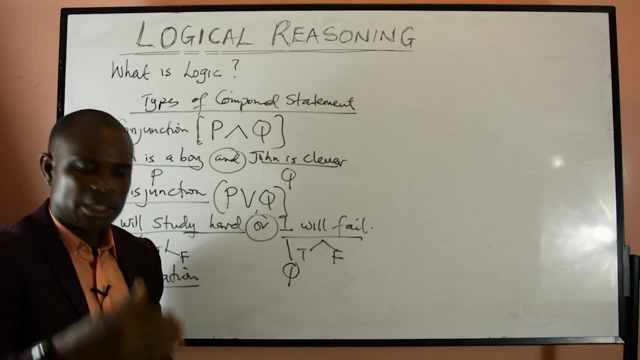 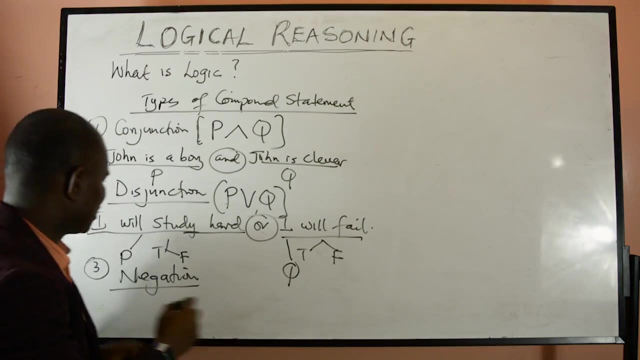 The third type is negation. What is negation? It is formed by Inserting not inside the principal statement. The first statement is: If I insert Not inside the statement, It means I am negating the statement. For instance: 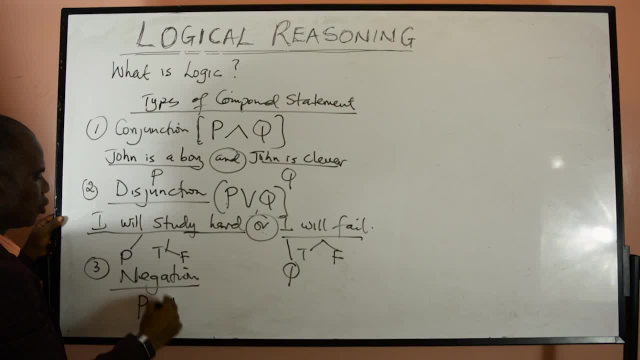 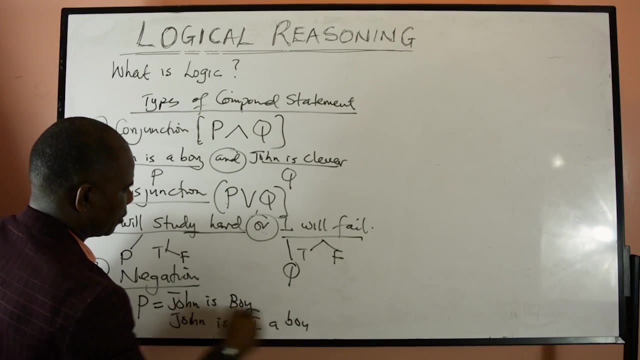 If I say P is From our statement here, John is a boy. Now I want to write: John is not a boy, John is not a boy. But because John is a boy, Is P. Now I want to negate the statement. 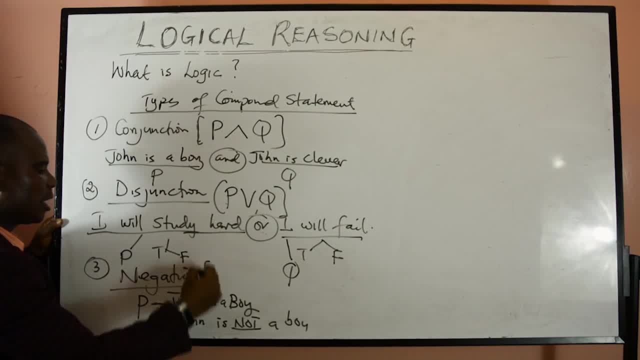 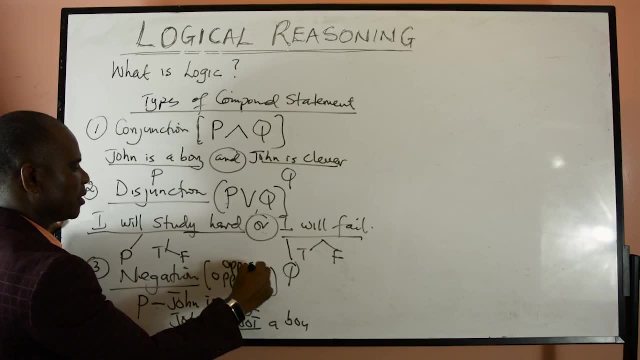 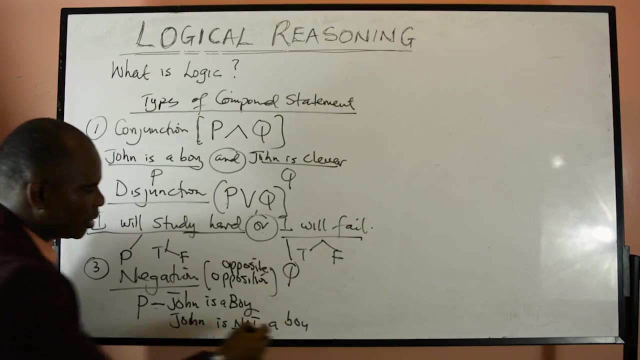 If I want to negate it, Meaning I want to oppose. That is opposition, Opposition or opposite. You can call it The opposite of the statement. Now, the opposite of the statement John is a boy Is John is not a boy. 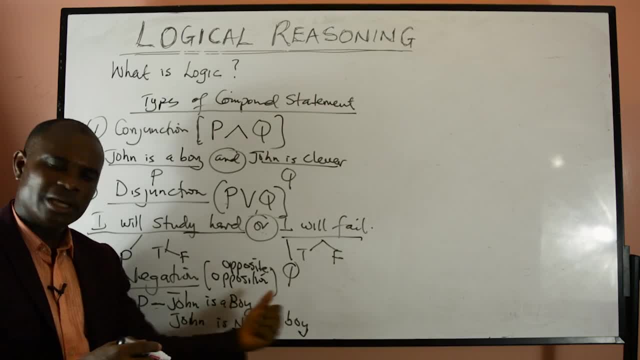 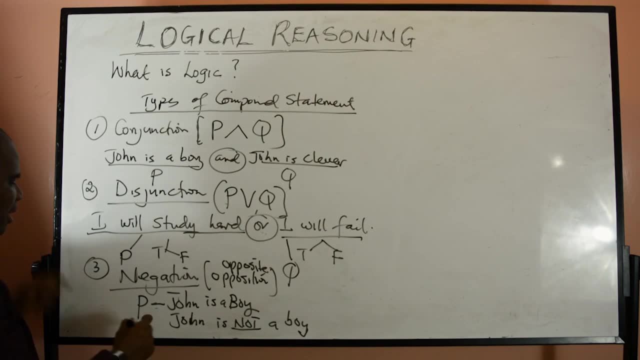 John is not a boy. I am inserting not inside the statement, For as much as I have Placed not inside the statement, I have already negated the statement And negating it is represented by Symbolic term. this: This is how negation is. 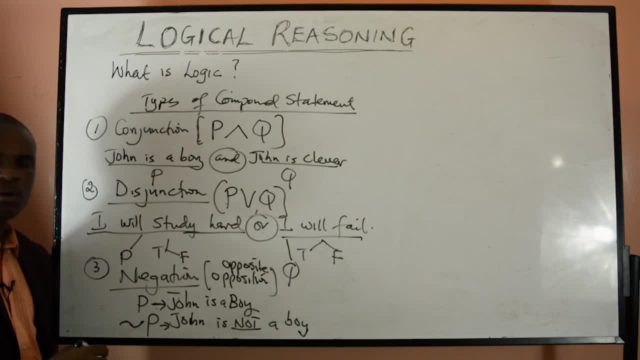 It is this tide which looks like a wave Or a sinusoidal curve. You have this. This is negation. Negation is the same as complement. in set theory. It is like, not A complement, A prime. That is the element in the universal set. 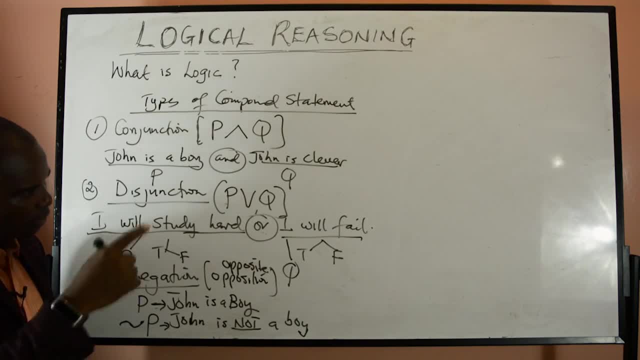 Or a complement of A. So we can say: Negation is the form. It is not in, It is formed by inserting in, Not inside the statement. When, once you can insert not inside the statement, Then you are negating the statement. 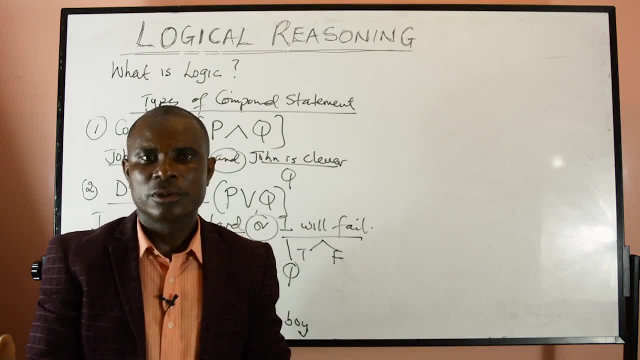 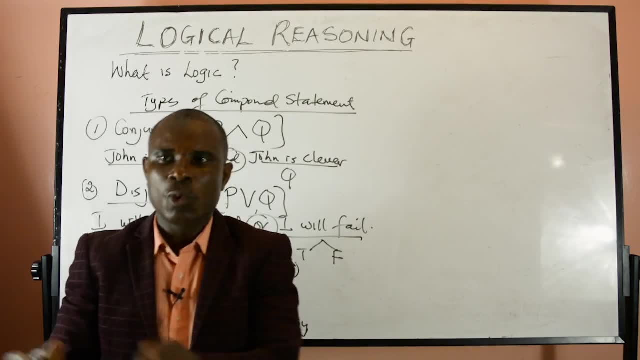 Like you can say I am happy, True or false. Then if I want to negate this statement, I can say I am not happy, So I have negated the statement. The opposite of the statement is Derived by putting not inside the original statement. 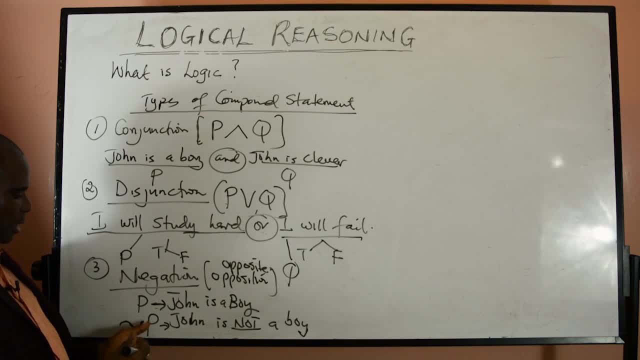 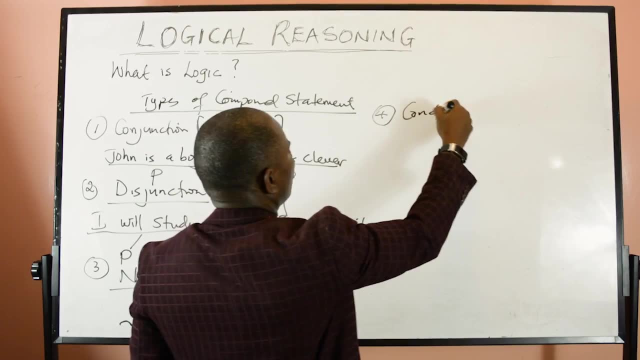 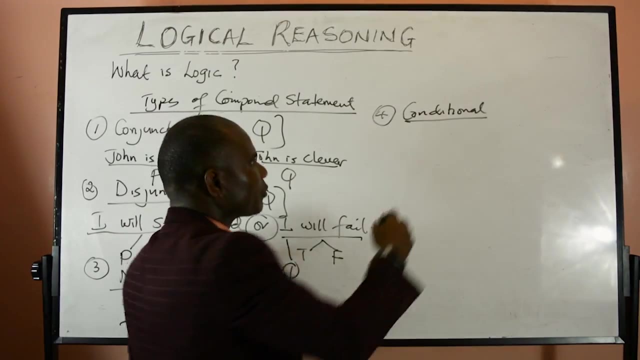 So this is written by Not. Not is inserted by this. This is the tall type of compound statement. What about the fourth type? The fourth type is called conditional. What is a conditional statement? Conditional statement is represented By the. Let's say: 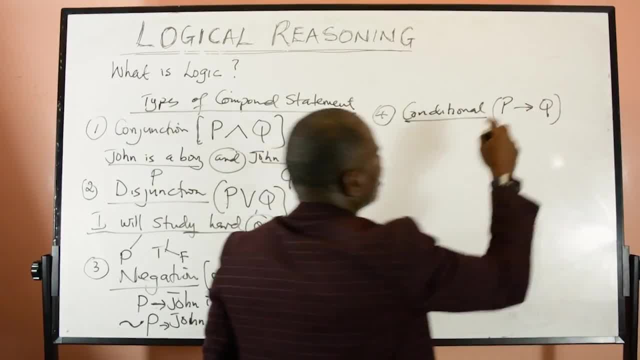 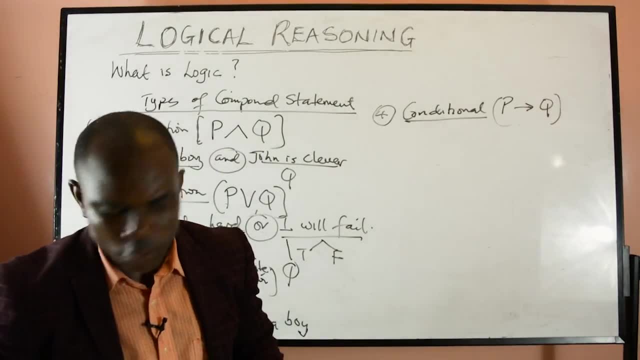 It is represented by that arrow. What is the meaning of this? Q will only happen Conditioned on the fact that P has taken place. What is a conditional statement? It is a statement in which The occurrence of one Is predetermined by 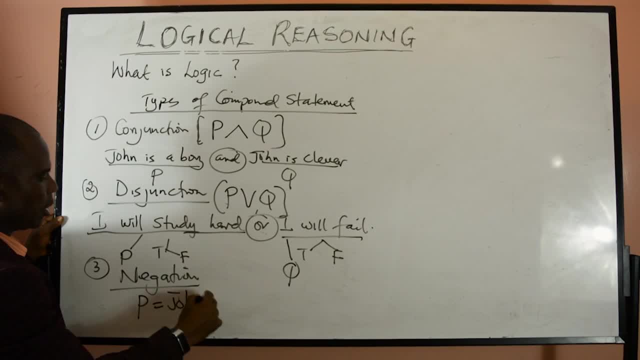 from our statement here: john is a boy. now i want to write: john is not a boy, john is not a boy. but because john is a boy, is p. now i want to negate the statement. if i want to negate it, meaning i want to oppose. that is opposition, if you like. opposition or opposites. 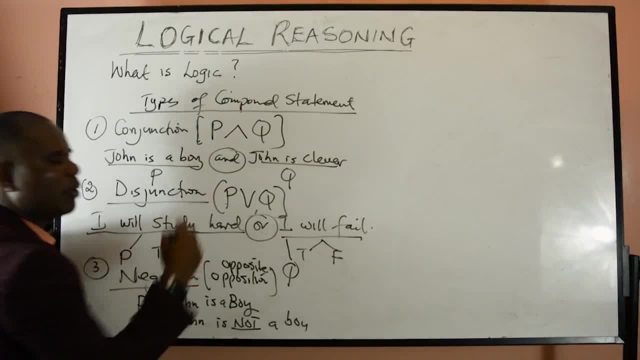 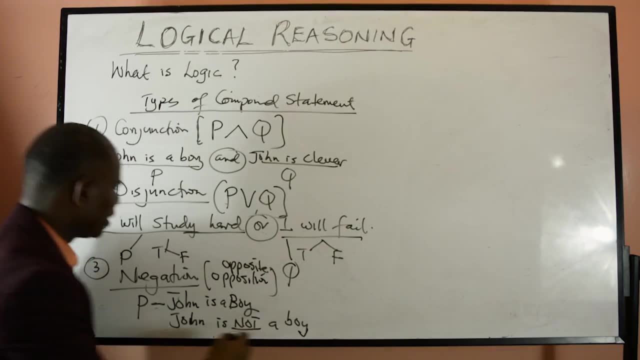 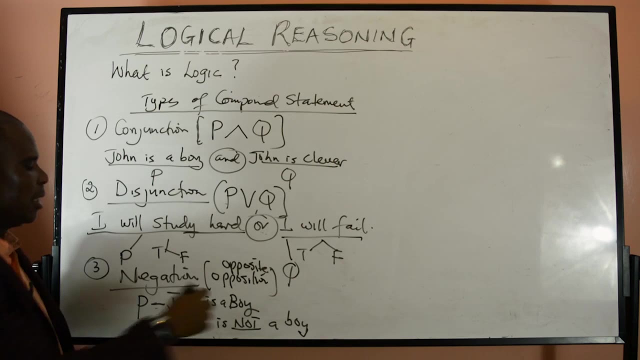 if you can call it the opposite of the statement. now, the opposite of the statement john is a boy is john is not a boy. john is not a boy. so a negation is formed by inserting not inside statement. for as much as i have placed not inside a statement, i have already negated that statement. 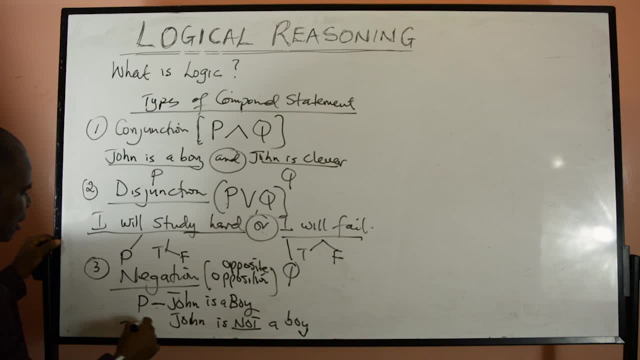 and negating. it is represented by symbolic term. this: this is how negation is. it is this tide which looks like a wave or a sinusoidal curve. you have this. this is negation. negation is the same as complement in set theory. it's like not a complement, a prime. that is the element in the universal set. 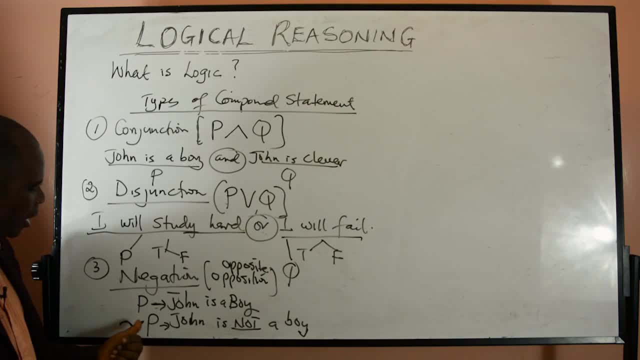 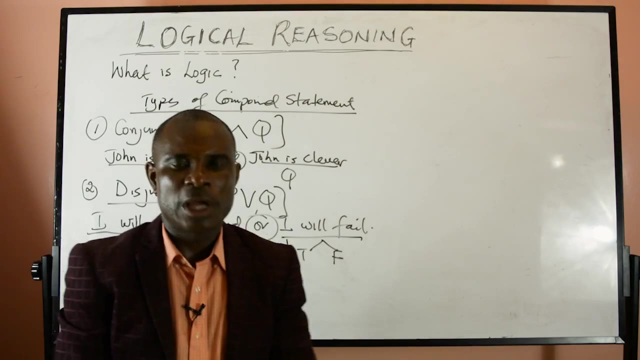 that are not found in a are all the complement of a. so we can say: negation is the form, it is not in, not it is formed by inserting n is a not inside the statement. when once you can insert not inside the statement, then you are negating the statement like you. you can see, i am happy. 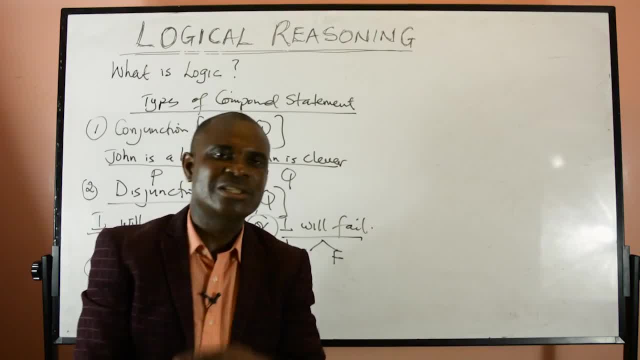 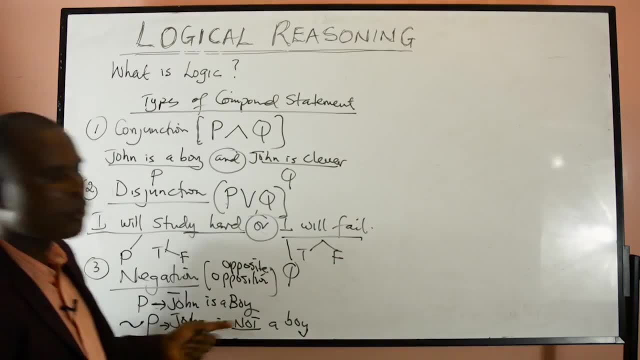 true or force, then if i, if i want to negate this, this statement, i can say i am not happy, so i have negated the statement by inserting not, which is not so. the opposite of the statement is derived by putting not inside the original statement. so this is written by: 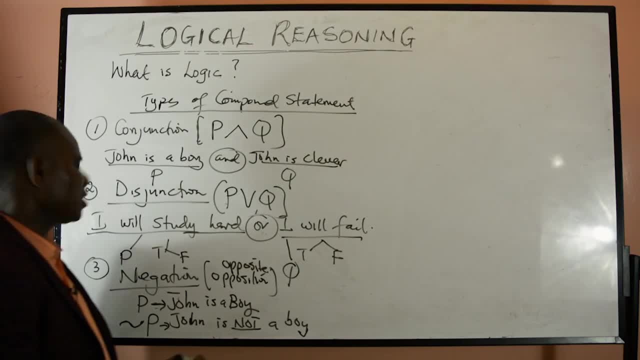 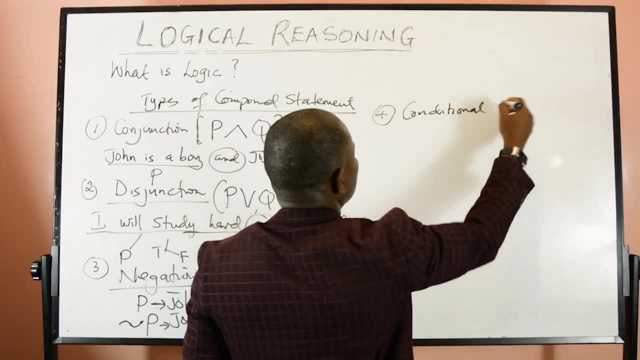 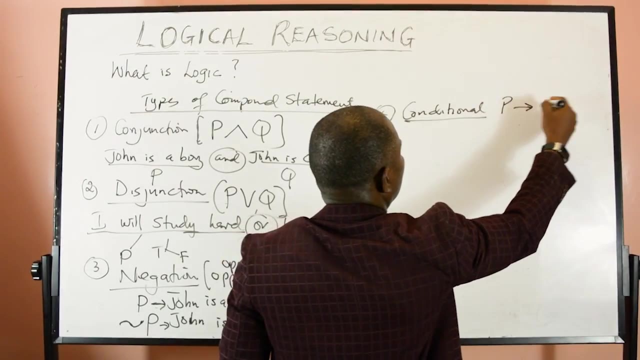 not, not is inserted by this. this is the tall type of compound statement. what about the fourth type? the fourth type is called conditional. what is a conditional statement? conditional statement is represented by the, let's say it's represented by that arrow. what's the meaning of this? it means 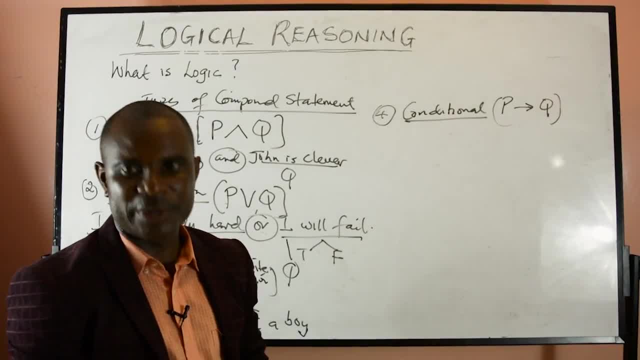 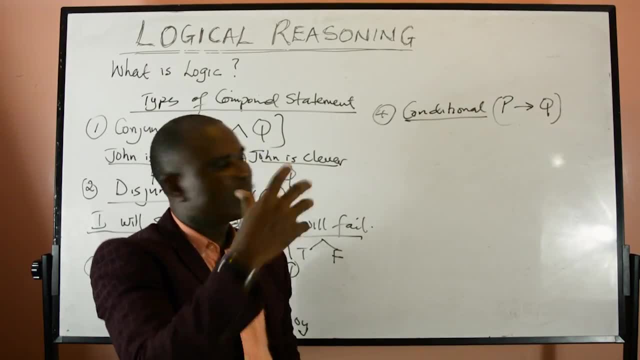 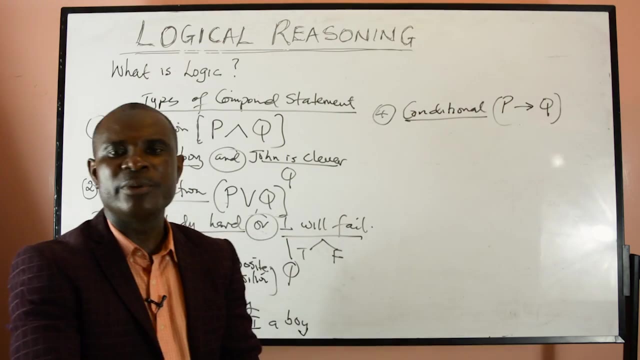 q will only happen, condition on the fact that p has taken place. what is a conditional statement? it's a statement in which the this occurrence of one is free, determined by the occurrence of the force. it is conditioned upon the fact that the false statement has taken place. the false event has taken place, and that's the, the. 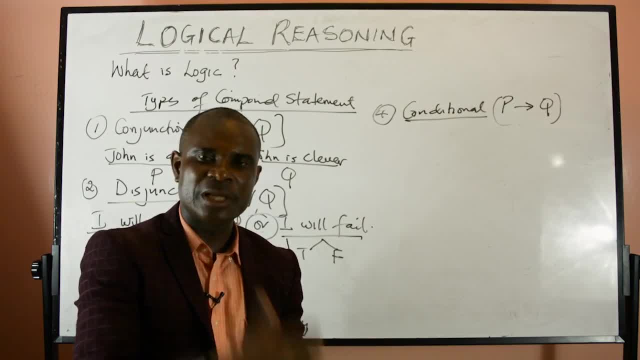 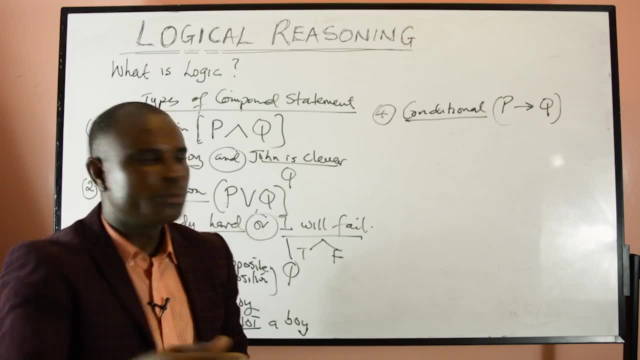 The occurrence of the first. It is conditioned upon the fact that The false statement has taken place. The false event has taken place. The occurrence of that false event Will now give you the occurrence of the other one. So for Q to happen, 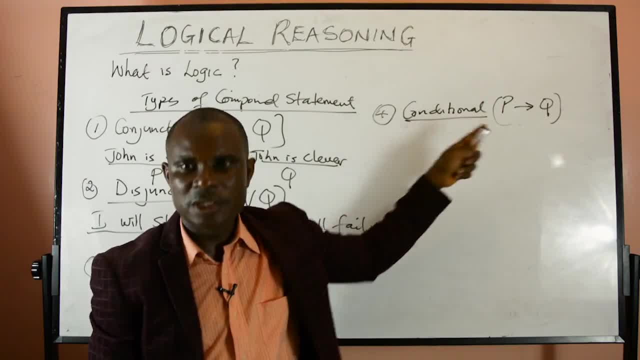 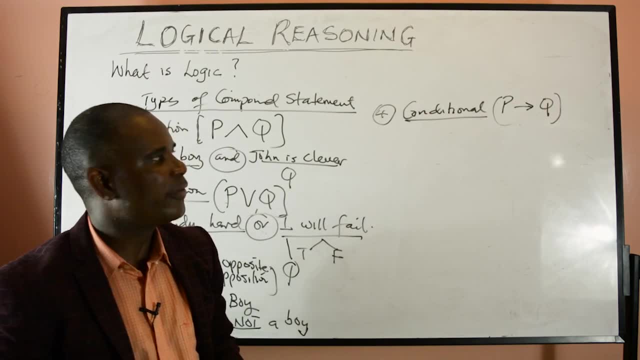 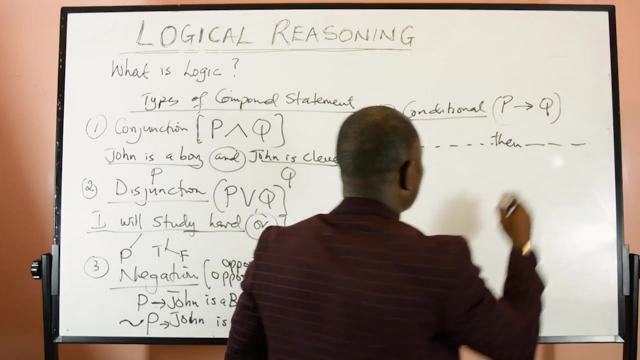 P must take place, So the condition for Q to happen Take place. So this is a conditional statement. And what is that conditional statement? How do we identify it in the question? It is identified by the word if, And then So. 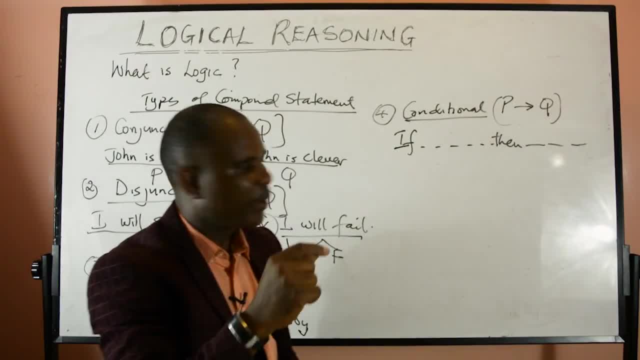 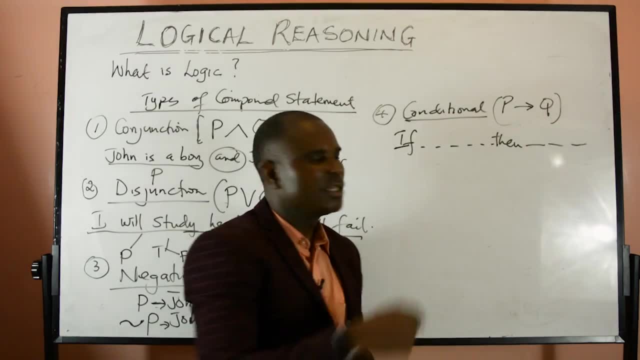 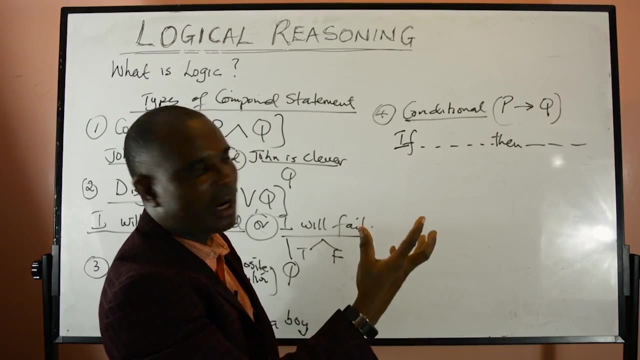 If I do not Use the pen, If I do not use A clear pen on this white board, Then the audience Will not see the writing. If I do not use A clear, white Or black marker, Clear one So that you can see. 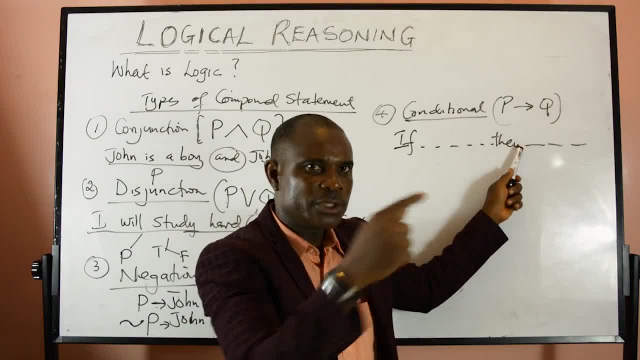 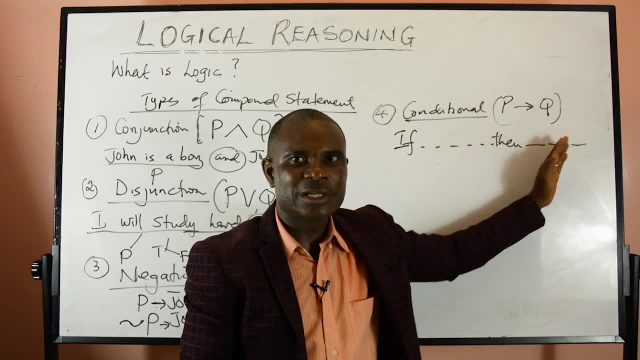 It means that if I do not use A clear marker, Then you will not see the writing on this white board. That is a conditional statement, Because if I have to see The writing clearly, Then I must use a clear Writing material. 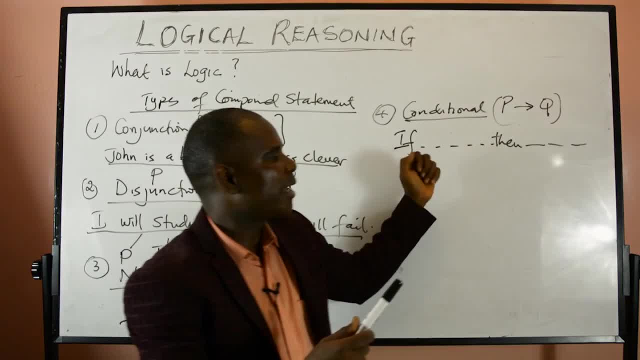 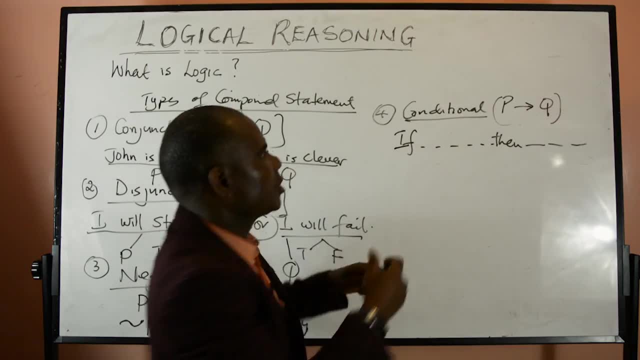 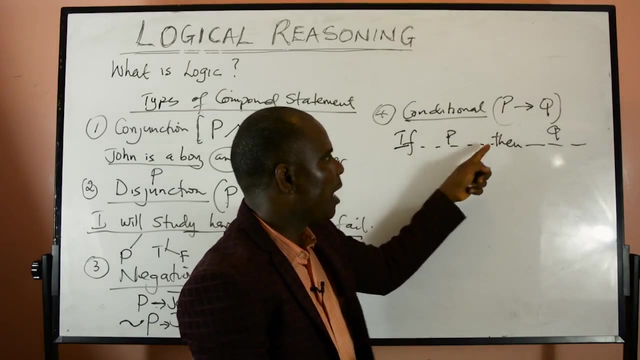 Which is the pen. I must use the marker here. That is clear Writing clearly. So if N, If the first statement takes place, Then Q will follow. It means If you want to be happy, Then you have to love people. 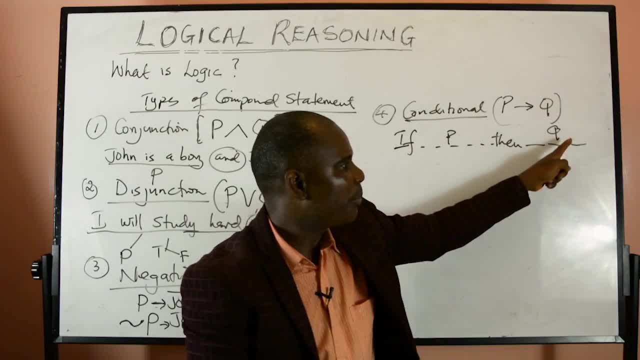 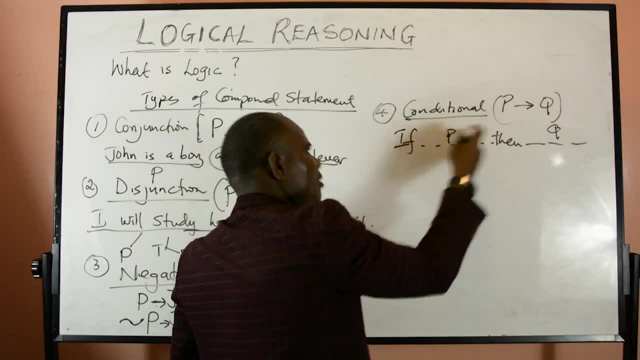 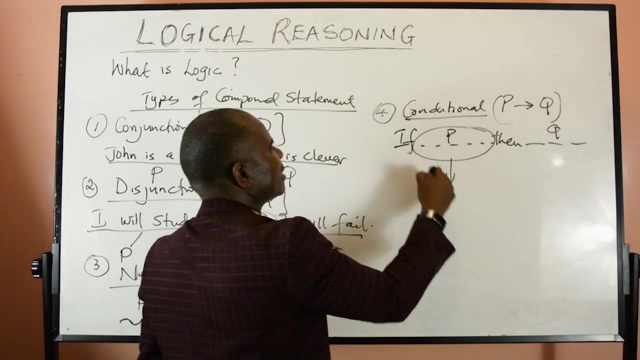 So now you look at, If I want to be happy, Meaning If I love people, Then I will be happy. So if I want to be happy, This first one must take place, This second statement That follows this if clause. 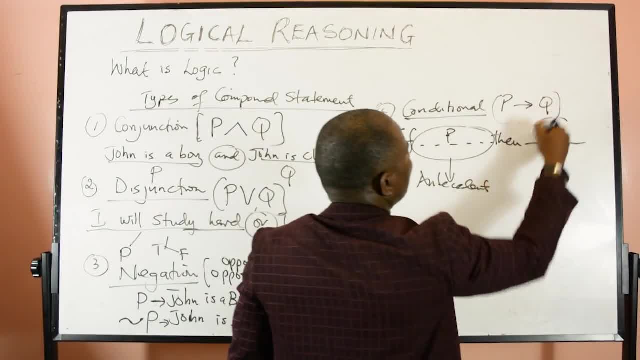 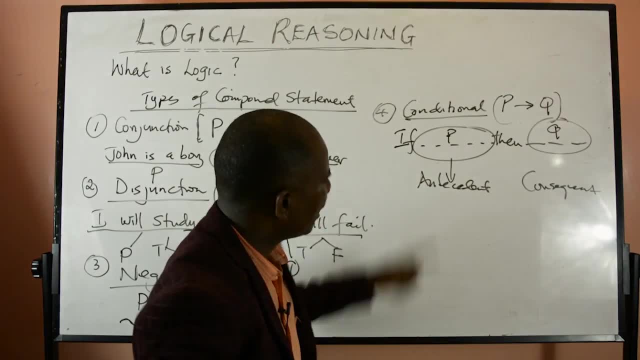 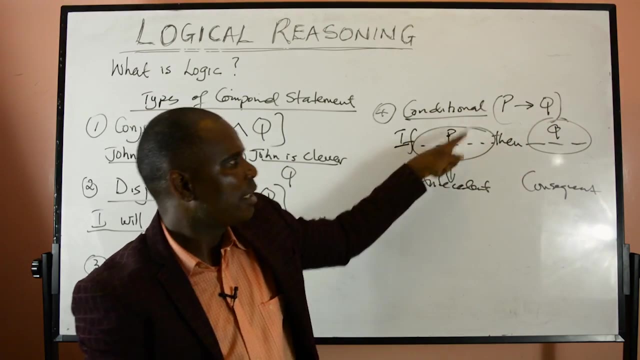 Are called the antecedent. We have the antecedent And all the statement that follows this then clause Are called the consequence. That is the result, The consequence thereof. So if this do not occur, Or if this occur, Then the order will occur. 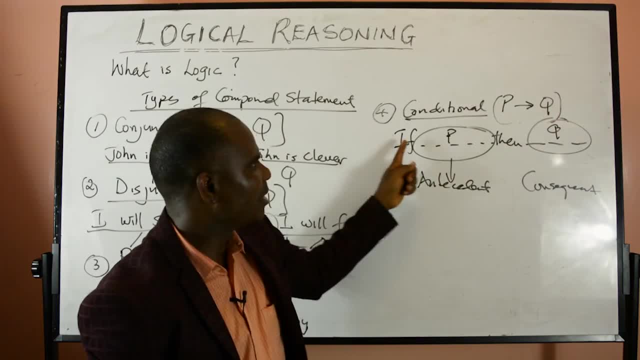 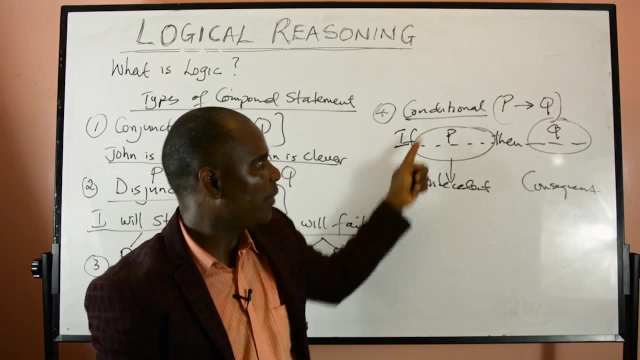 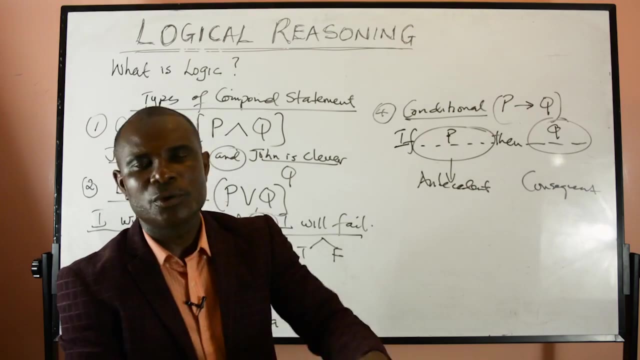 If you study hard, Then you will be happy The day of the result. So now this is the conditional: You have to study hard. So if I study hard, then I'll be happy the day of the result. So now this is antecedent, or the statement that follows the if clause is called. 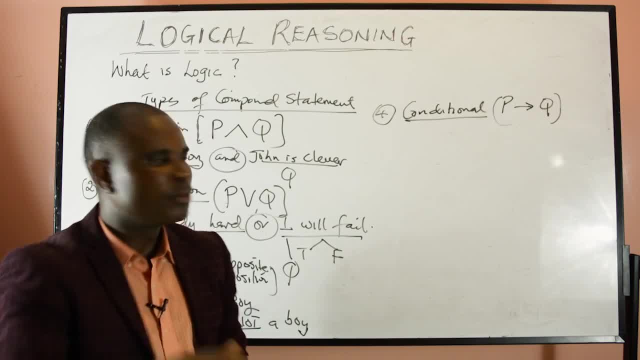 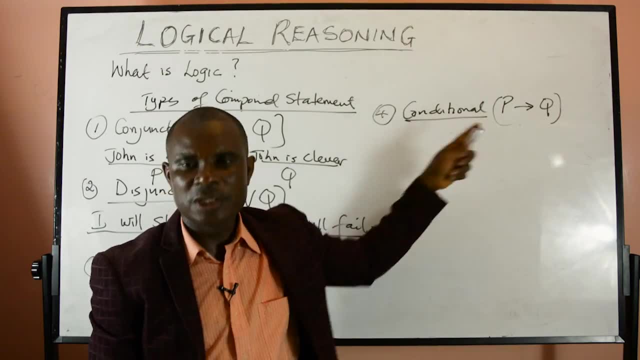 the occurrence of that false event will now prelude, will now give you the occurrence of the other one. so if for q to happen, p must take place. so the condition for q to happen it is when p takes place. so this is a conditional statement. and what? 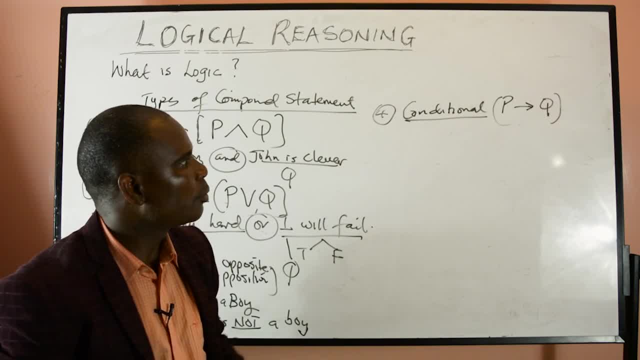 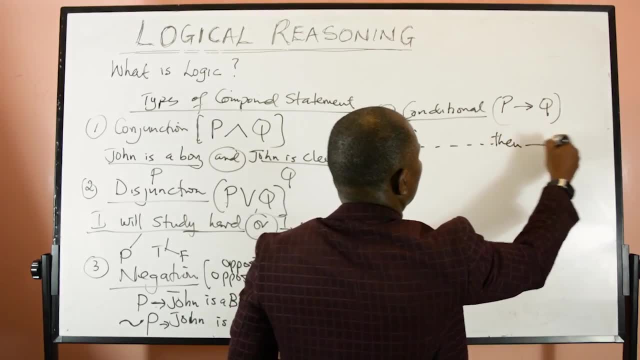 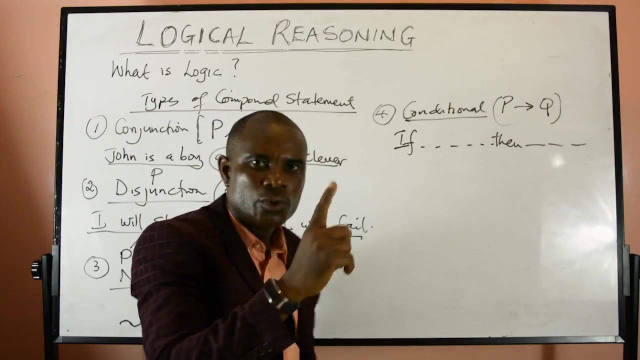 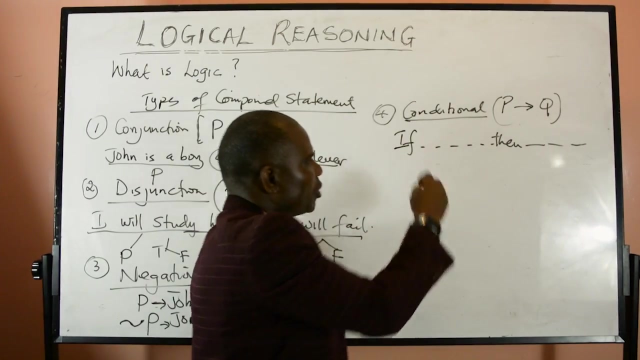 is that conditional? how do we identify it? in the question, it is identified by the word if and then. so if i do not, uh, use the pen, if i do not use a clear pen on this white board, then the audience will not see the writing. if i do not use a clean, a clear, white or black marker, clear one. 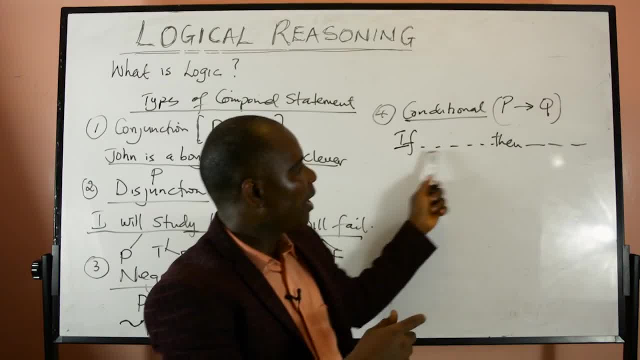 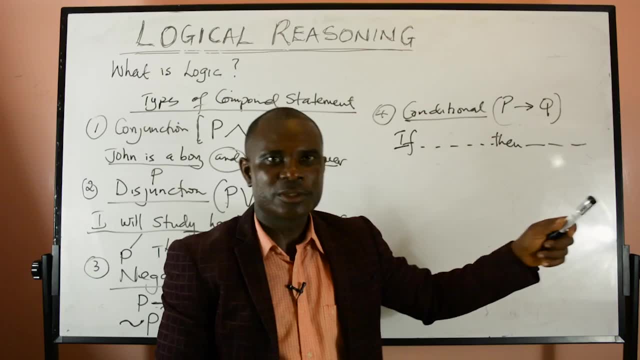 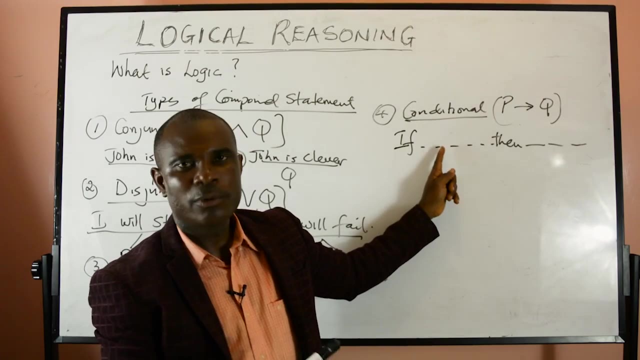 so that you can see. it means that if i do not use a clear marker, then you will not see the writing on this whiteboard. that is a conditional statement, because it if i have to see the writing clearly, then i must use a clear- uh right- writing material, which is the pen. i must use the marker here. 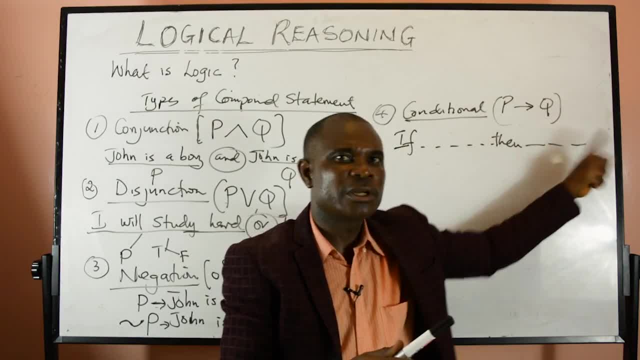 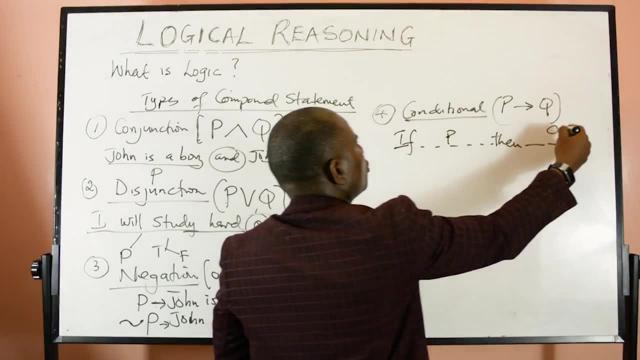 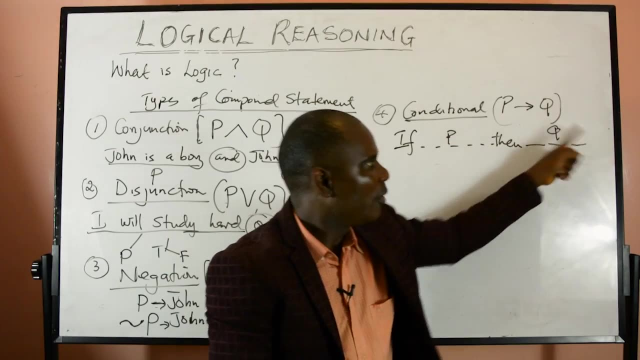 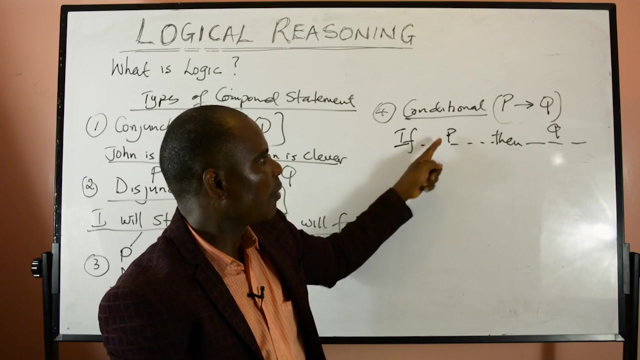 that is clear so that it can enable you to see the writings clearly. so if n, if the first statement takes place, then q will follow. it means if you want to be happy, then you have to love people. so now you look at, if i want to be happy, then for that say meaning, if i love people, then 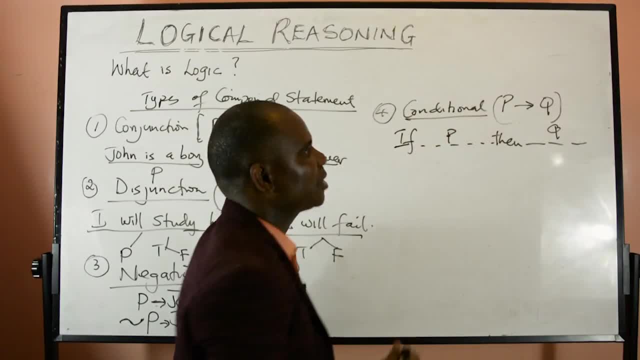 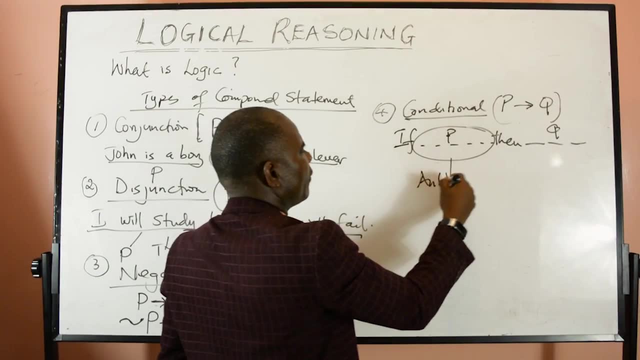 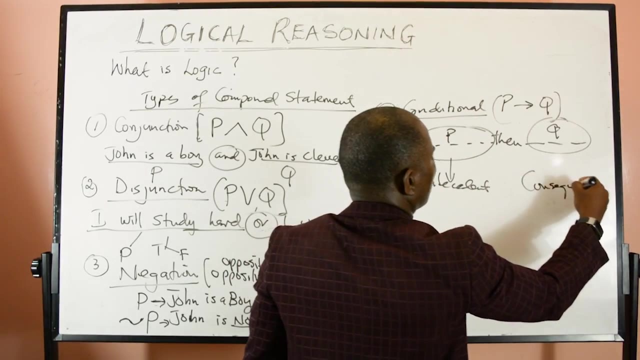 i'll be happy. so if i want to be happy, this first one must take place. so all these statements that follows this, if clause are called antecedents, we have the antecedent and all the statement that follows this. then clause are called the consequence. that is the. 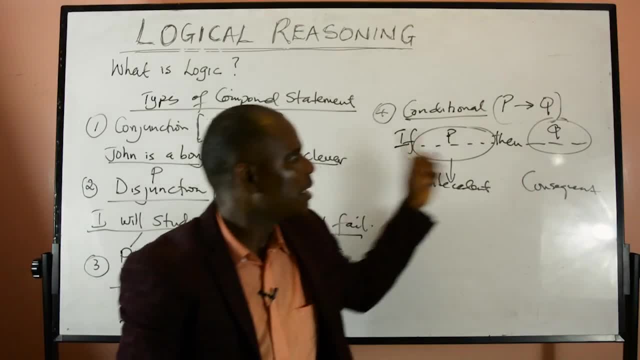 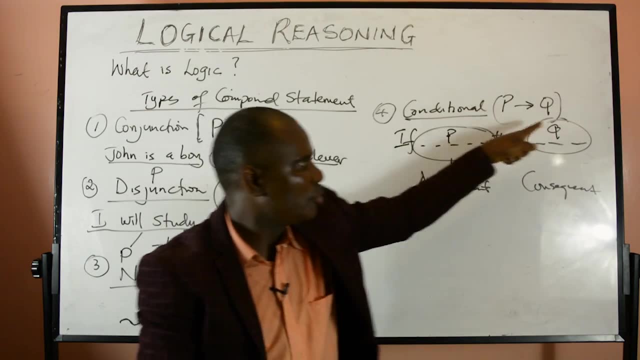 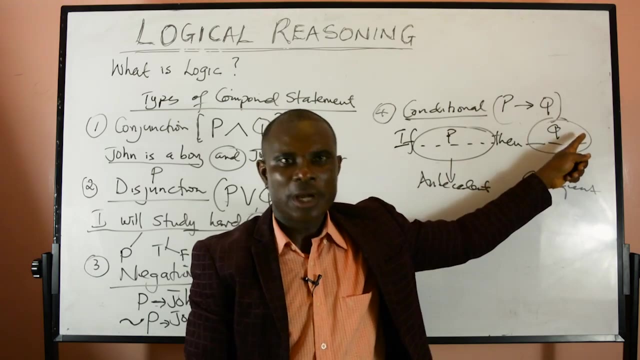 result, the consequence thereof. so it's this: do not occur, or if this occur, then the order will occur. if you study hard, then you will be happy the day of the result. so now, this is the conditional for you to be happy: you have to study hard. so if i study hard, then i'll be happy the day of the result. 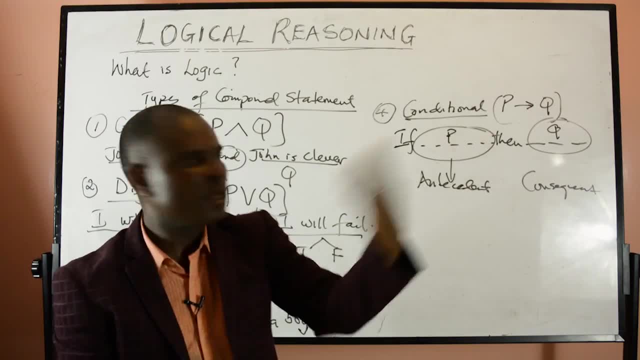 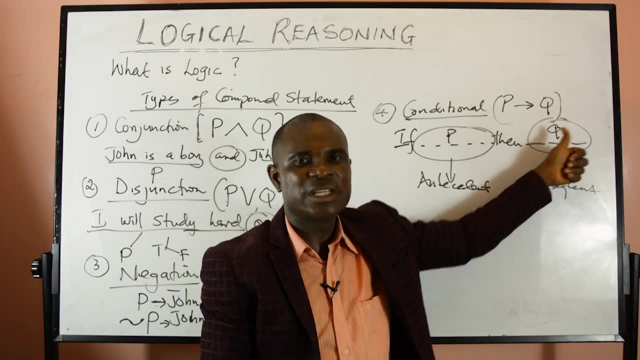 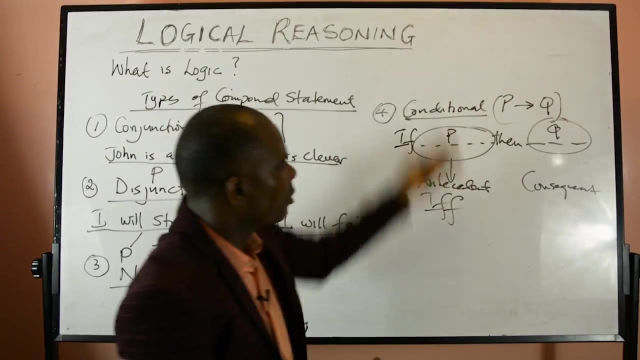 so now this is antecedent. all the statement that follows the if clause is called the statement that follows the if clause is called the antecedent, and the statements that follow the then clause is called the consequence. it can be summarized as if, and only if, this is a conditional statement. 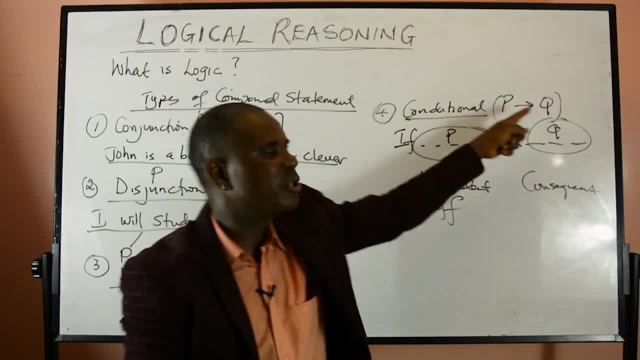 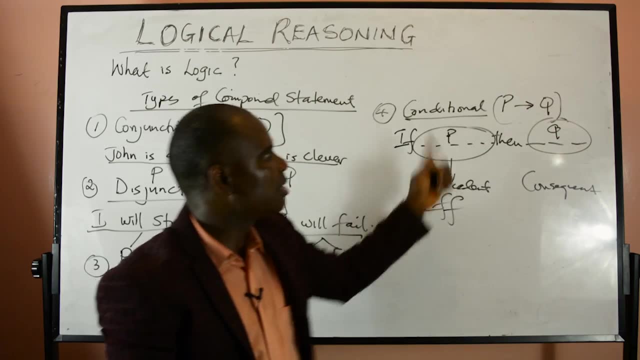 this symbol is if, and only if. so conditional statement is based on the fact that an event takes place before another event can also proceed from there. so it is because p takes place. that's how q will follow. that is what is called a conditional statement. so now, 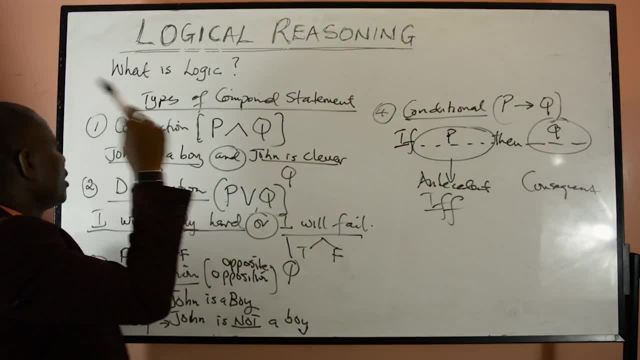 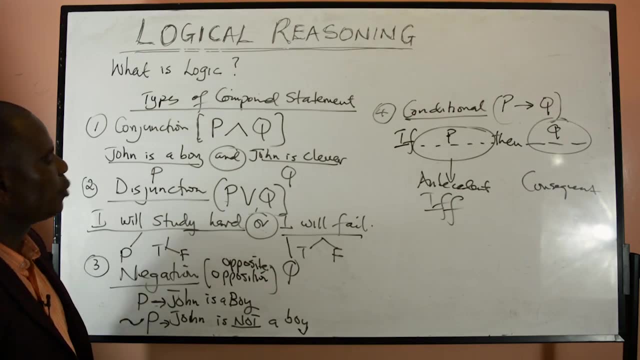 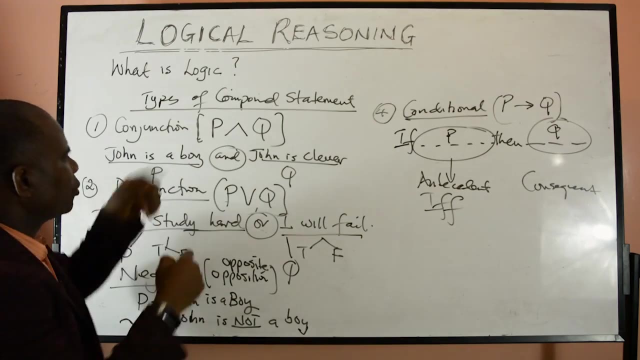 you have seen the four types of compound statements. you have a conjunction which is tied together by the, the word and, and we have this junction which is joined together by the word or. so the conjoints can be put together by the word or, and here also the conjoints are put together by the word n. 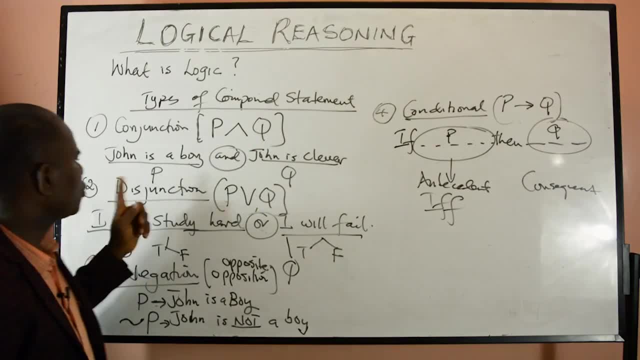 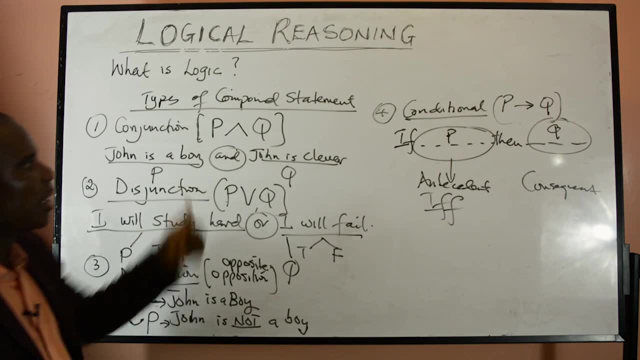 so when you use and we are forming a conjunction, when you use all your coming for me a disjunction and when you use not, you are negating the statement. it is also a compound statement which is negated and we have condition which is based on the fact that an event has taken before place. 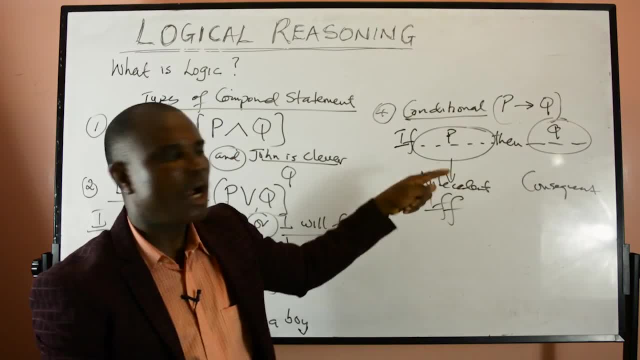 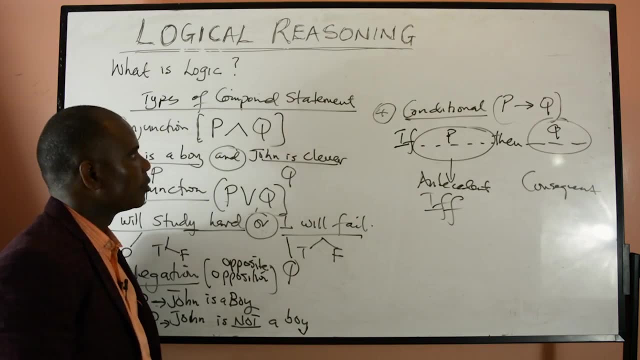 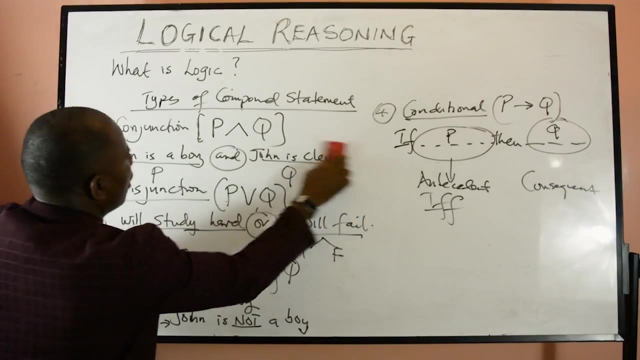 force before the next one takes place. so if this does not happen, then that will happen. that is a condition for that event to occur. so now we have the four types of statements. so now we can move a little bit and i can clean the board and we see how we can proceed with the very 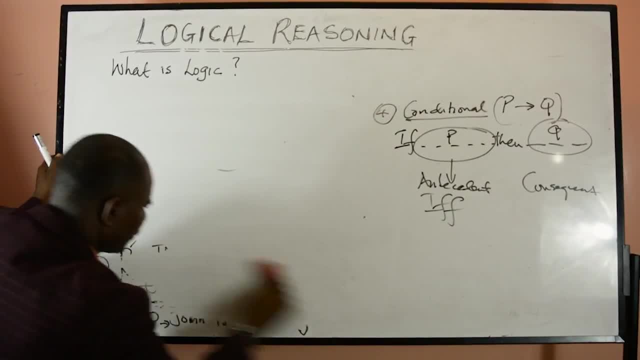 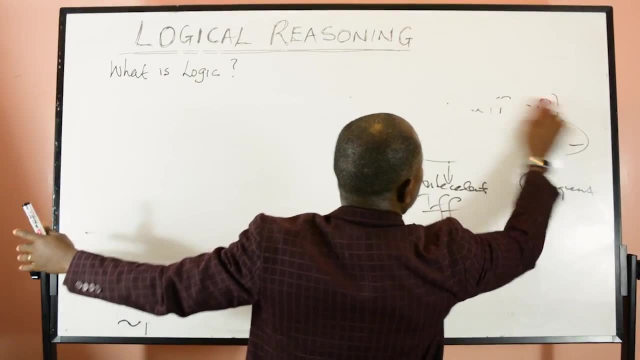 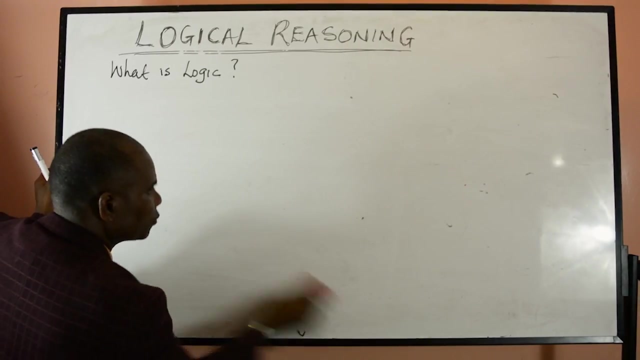 the very form of logic. so you have now seen the statement, the types of statements. we have simple statements and we have done the compound statements. so now we are going to move a little bit from the truth form of the statement and we move to the other part. so logic, logic and logical. 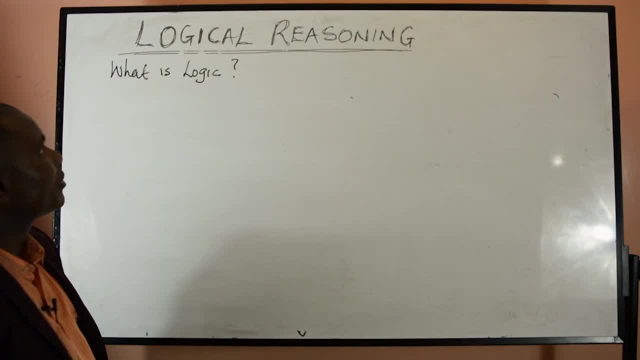 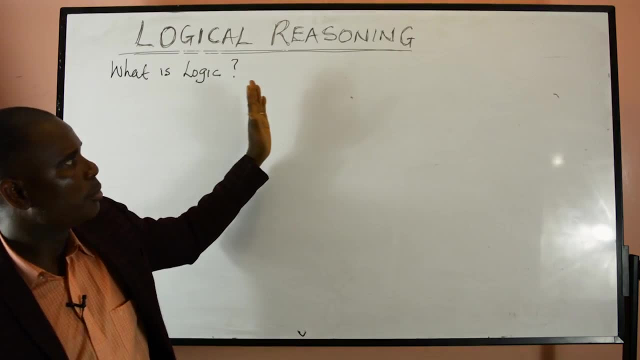 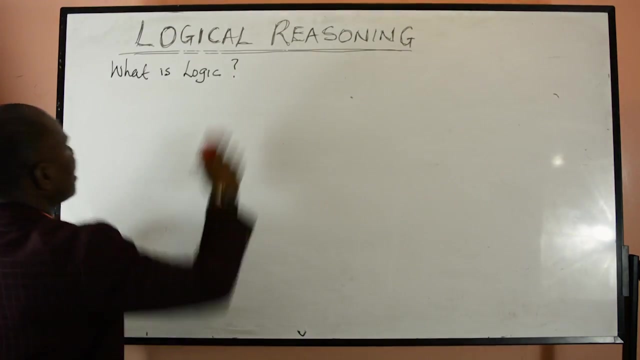 reasoning actually is based upon argument and truth. so now, once you have seen the statement table, so for for today, we're going to leave the truth table and we now go to the argument. so we have to look at the argument. so what is an argument? an argument, in other words, we call it syllogism. 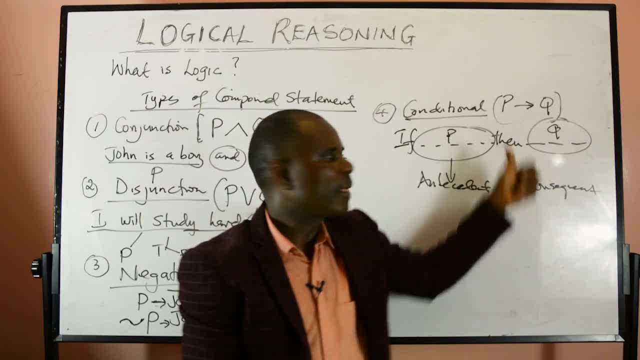 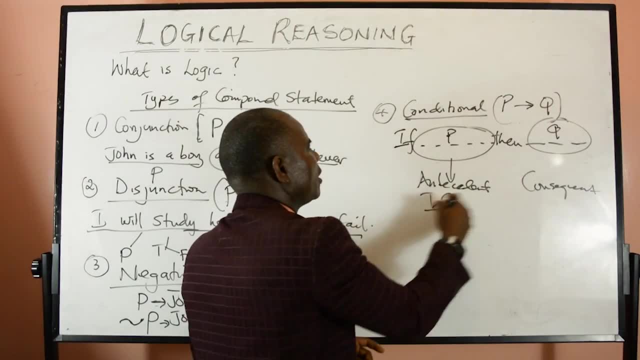 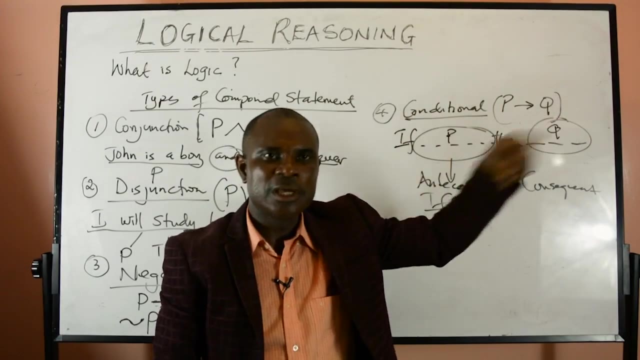 the statement that follows the if clause is called antecedent and the statements that follow the then clause is called a Consequence. it can be a sunrise, as if, and only if, This is a conditional statement is. this symbol is if, and only if. so conditional statement is based on the fact that an event 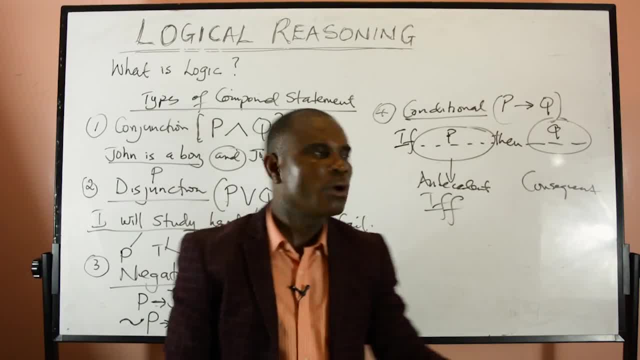 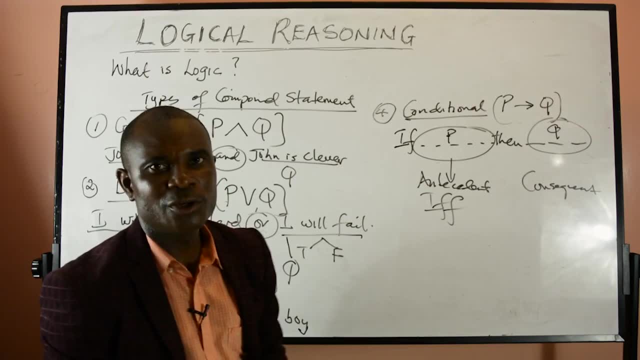 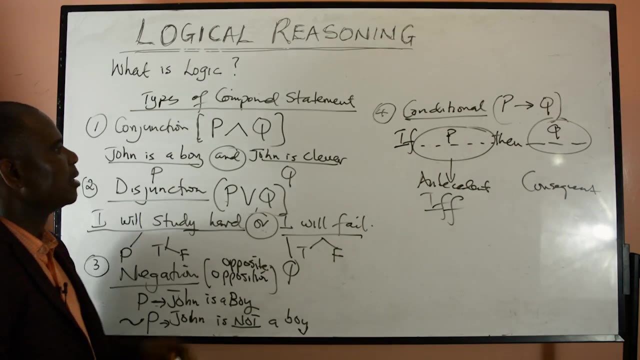 Takes place before another event can also proceed from there. So it is because P takes place. That's how Q follow. that is what is called a conditional statement. So now you have seen the four types of compound statements. you have a conjunction which is tied together by the. 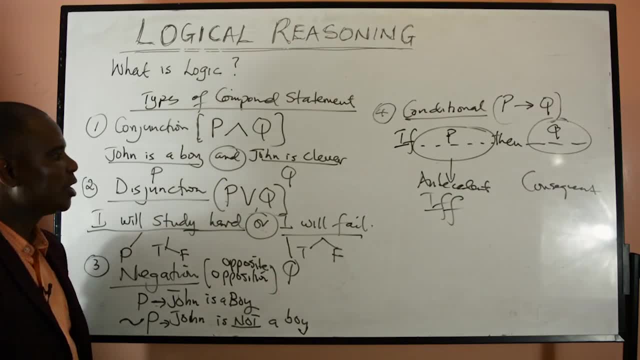 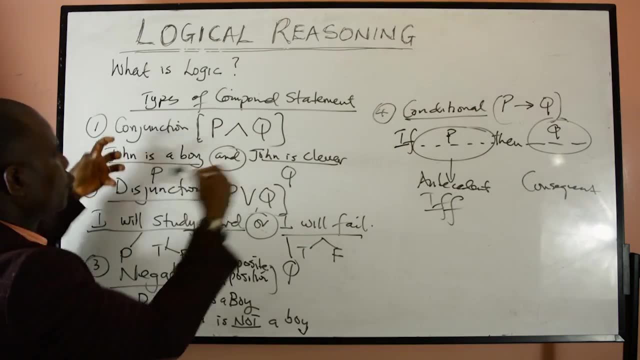 The word. and now we have this junction which is joined together by the word or. so the conjoints can be put together By the word or, and here also the conjoints are put together by the word end. and So when you use and we are forming a conjunction, 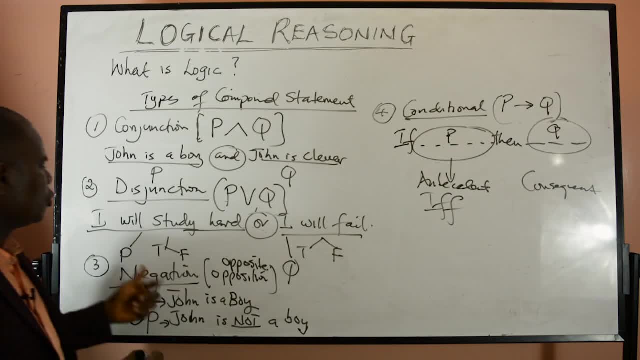 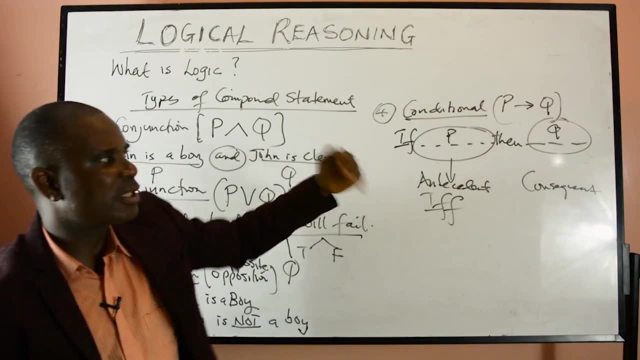 When you use all your coming for me a disjunction, and when you use not, you are negating the salt. this statement, It is also a composite which is negated, and we have condition which is based on the fact that an event has taken Place force before the next one takes place. 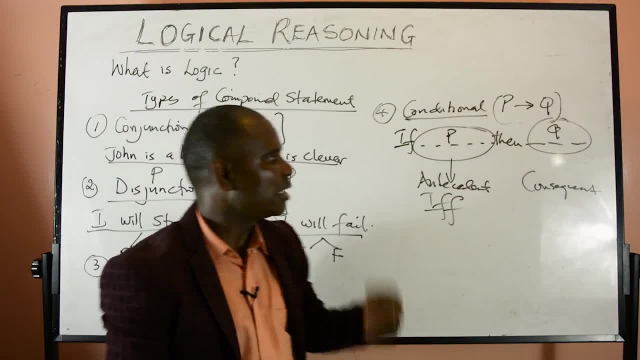 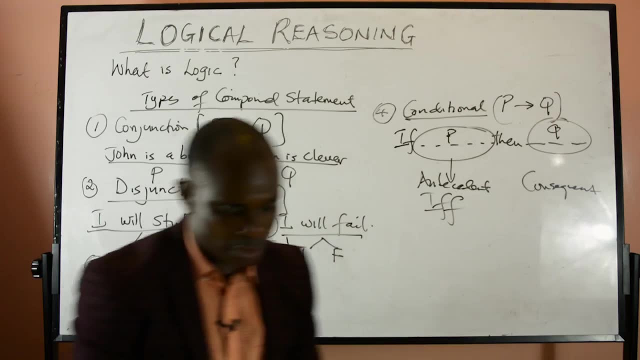 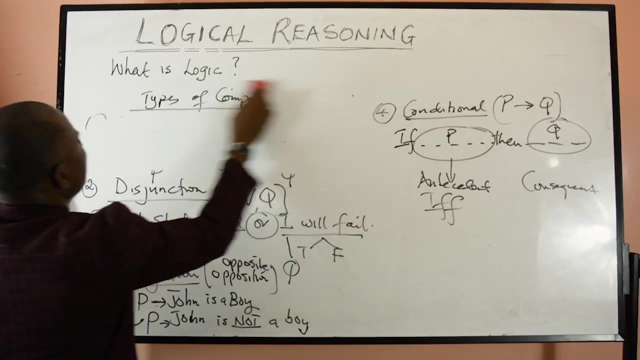 So if this does not happen, then that will happen. that is a condition for that event to occur. So now we have the four types of statements, So now we can move a little bit and I can Clean the board and we see how we can proceed with the very 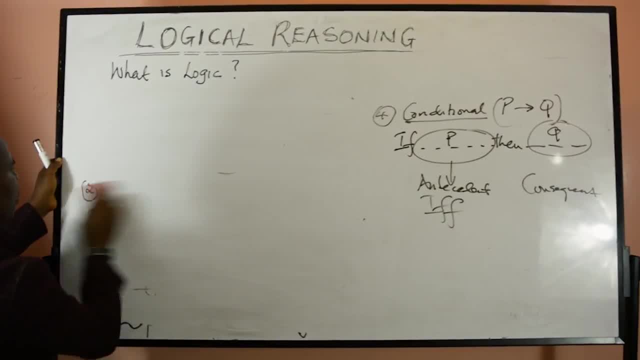 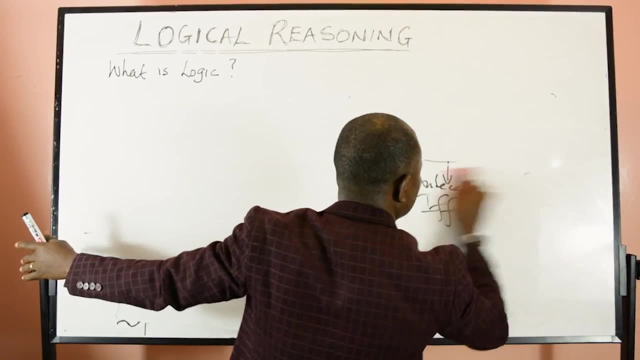 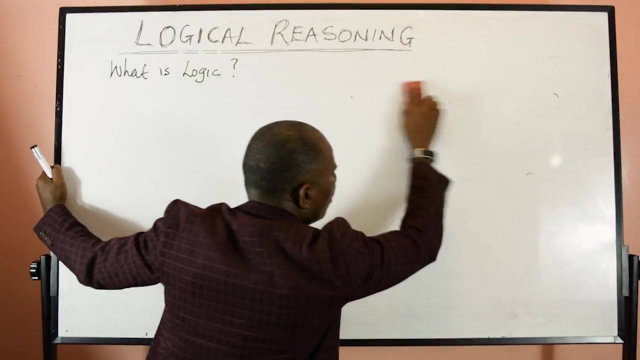 The very form of logic. so you have now seen the statements, The types of statements. we have simple statements and we have done the compound statements. so now we are going to move a little bit from The truth form of the statement and we move to the other part, logic, logic. 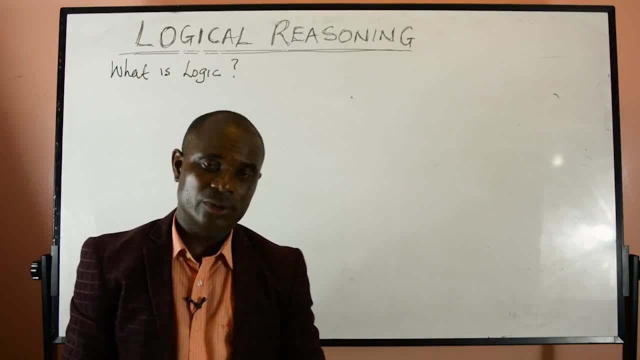 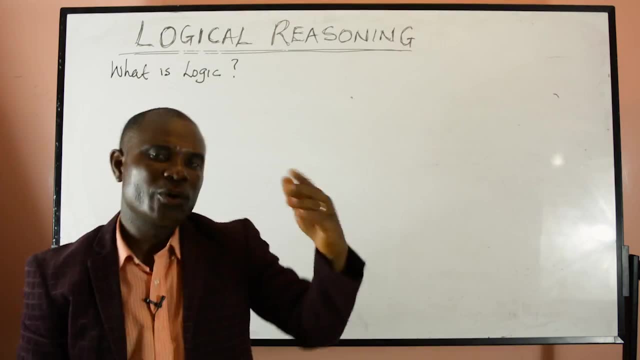 And logical reasoning actually is based upon argument and truth table. So for today, we're going to leave the truth table. I will now go to the argument. So we have to look at the argument. So what is an argument? and I give, there is not a wash. 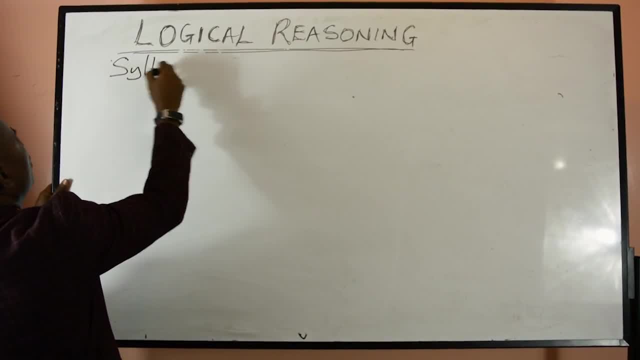 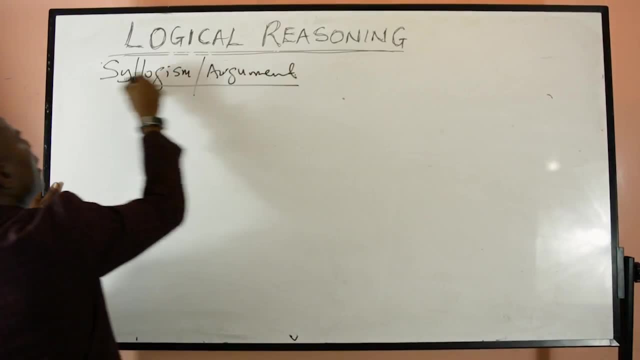 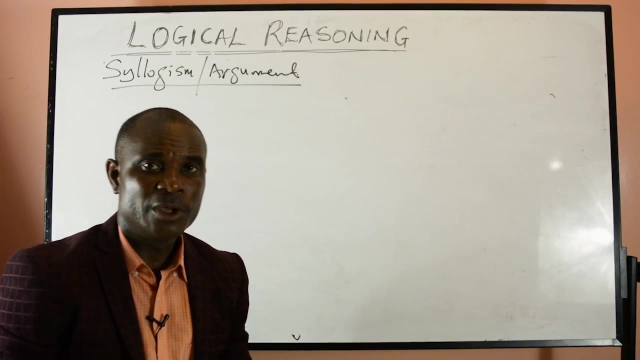 We call it syllogism, So let's call it syllogism. This is syllogism or arguments, was to look at that argument. So an argument or a syllogism is a Set of statements. you already know what the statements. now it is a set of statement that will. 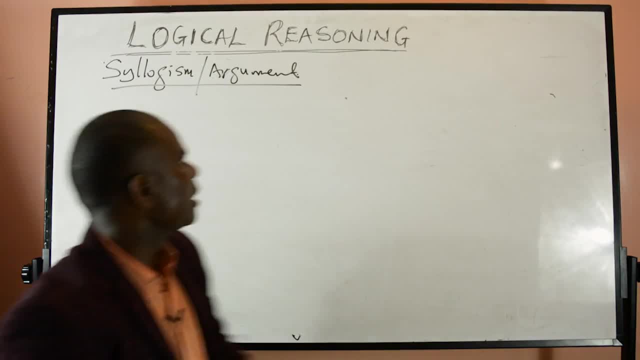 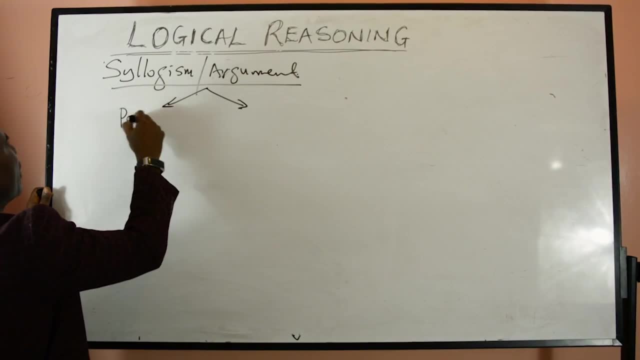 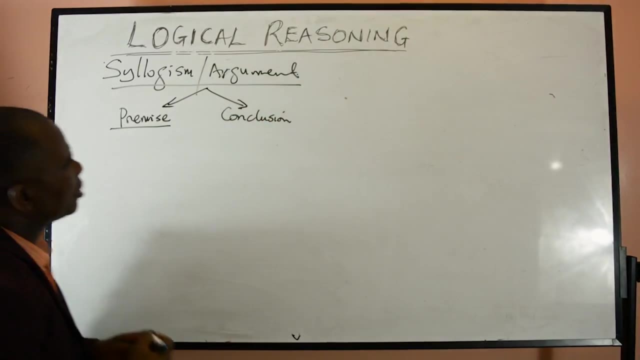 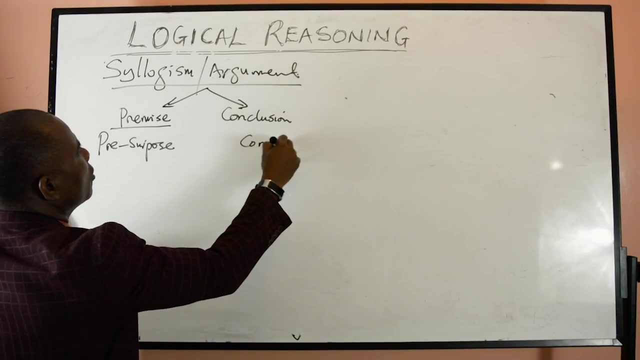 Conclude something. So what is that set of statement? It is divided into two. So an argument is this: divided into two, We have the premise, part of the argument, And you have the conclusion. The premise is: what will prescript suppose? This is what we are going to presuppose and this is what we conclude. We conclude with these. 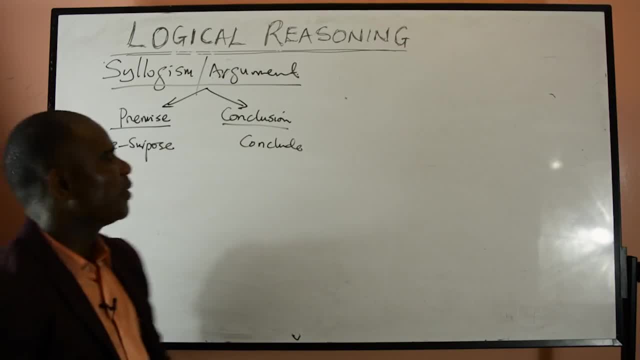 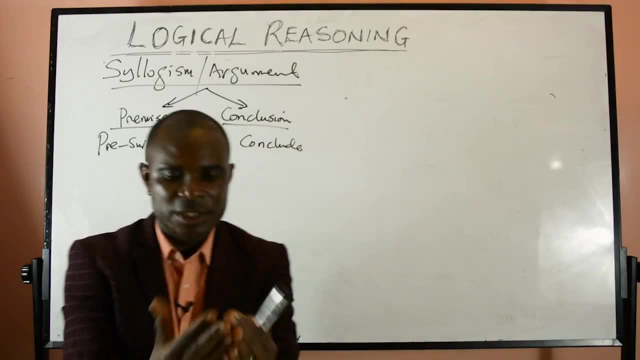 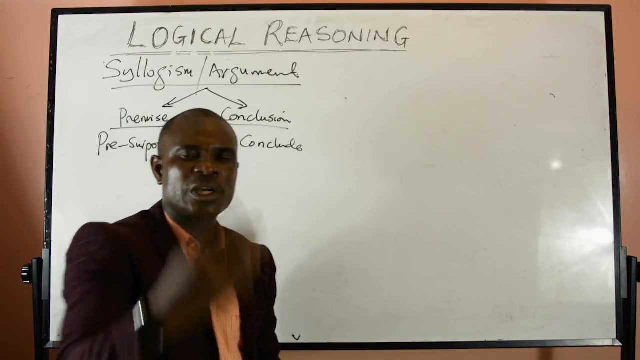 So we have to pack of an argument. We have the previous part of the argument. I'll have the conclusion part of the argument, and an argument or syllogism is a set of statements, one of which is a Conclusion which is drawn on the orders, on the basis of the orders, which I called the premise. 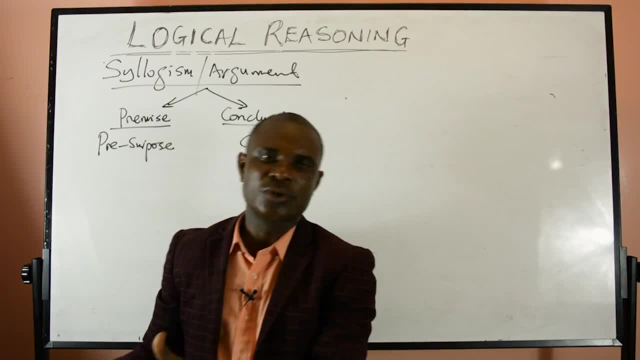 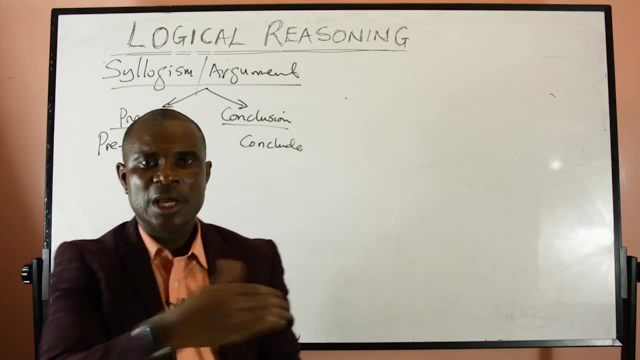 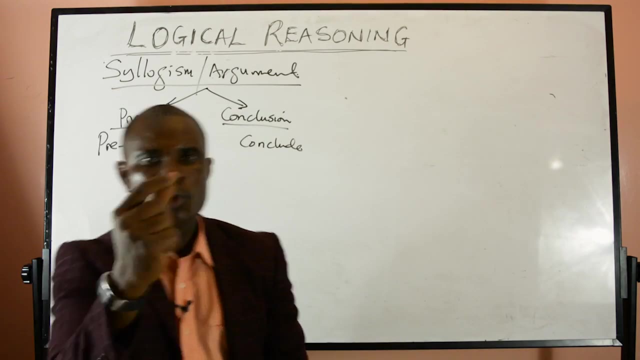 so now we have the premise part of the arguments and you have the conclusion part of the argument. so the argument is normally of three statements you have two of them are premises and the last one is the conclusion, and that conclusion is drawn from the premises. so the arguments can be divided into two. you have the presupposition, that is the 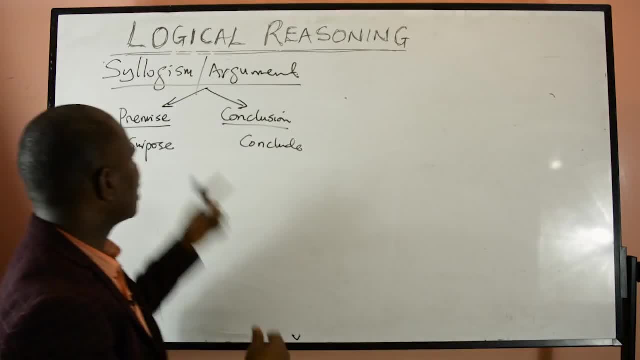 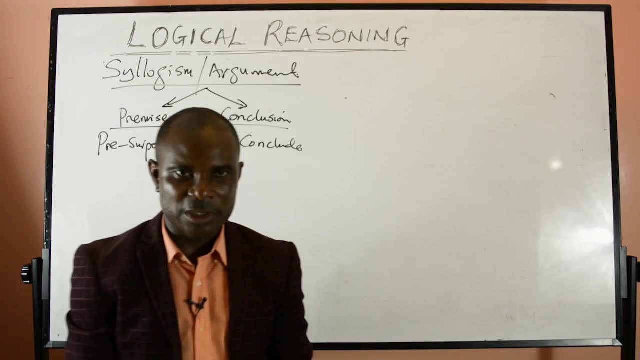 the premise part of it, the evidence is, and now we can use those evidences to draw conclusion. that's what makes up an argument. well, once this argument do have this part, there is not an argument. so an argument must have the following part: it must have two parts. first it must have a premise part, that is what you 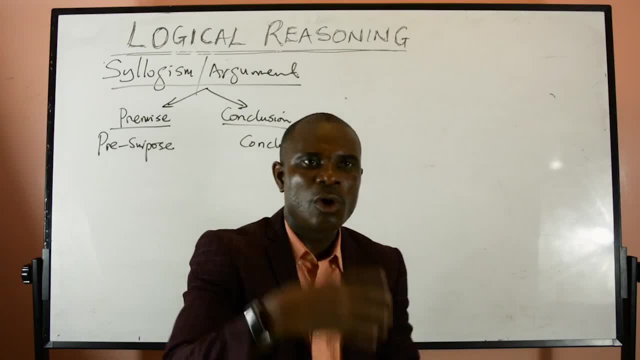 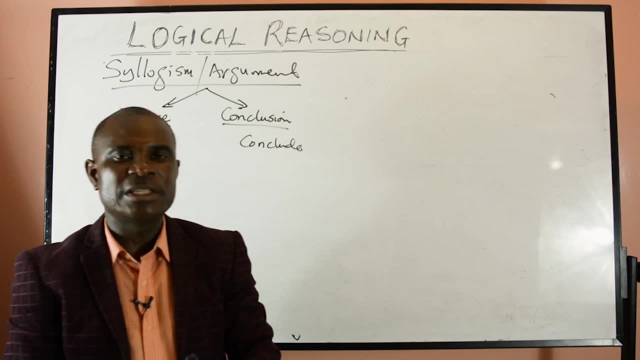 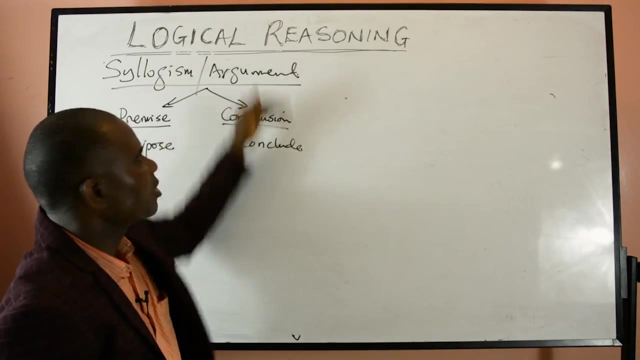 presuppose, or in other words the evidences or the premises. we call them and we have. it is from those premises that we can now conclude. the last one is normally what concludes, and that conclusion is drawn from the premises. so that kind that this set of statements put together is what you call. 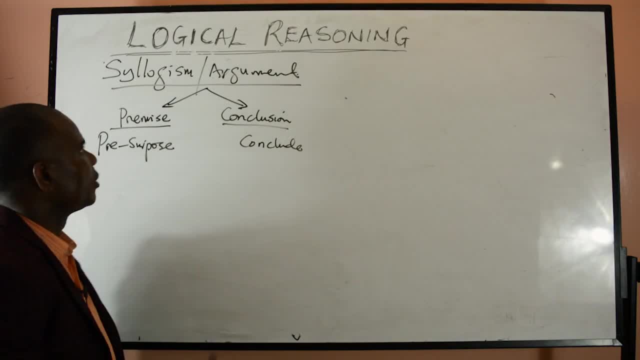 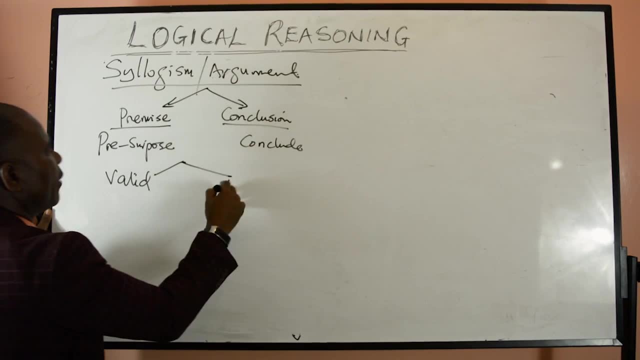 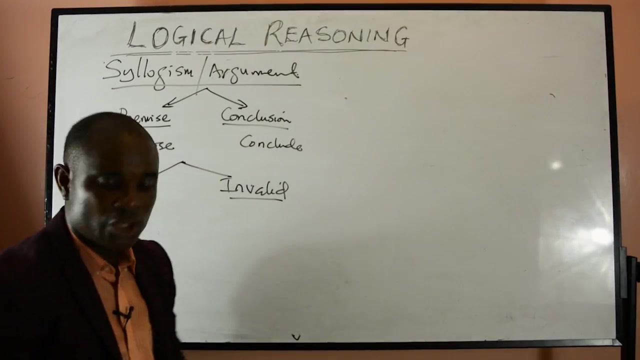 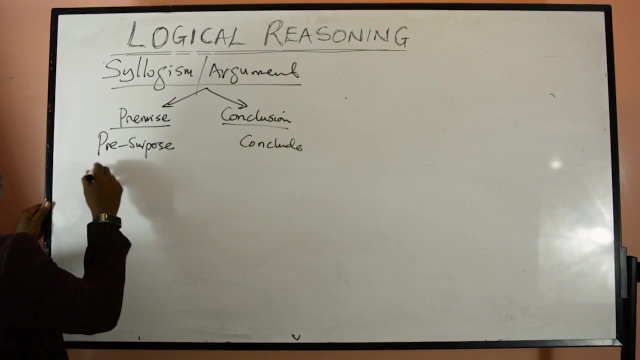 an argument. so we're going to look at the, the forms of argument. we have values, valid argument and you have invalid arguments. what is a valid argument? a valid argument, first, let me. let me give you an example of an argument. then we can know whether the argument is value or not. so, as I say all, all, all students are. 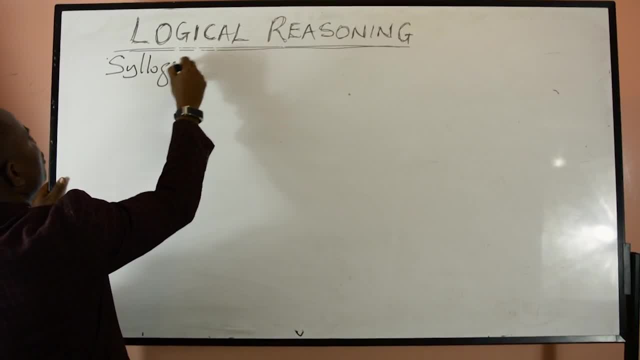 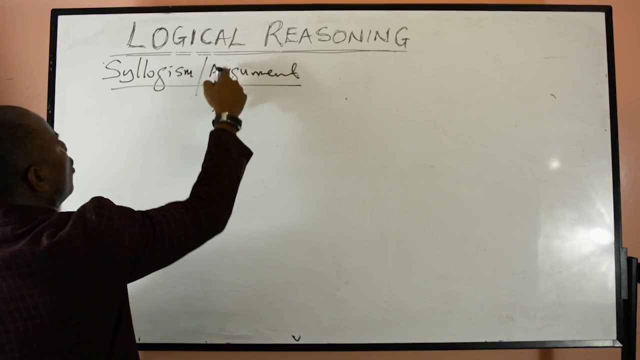 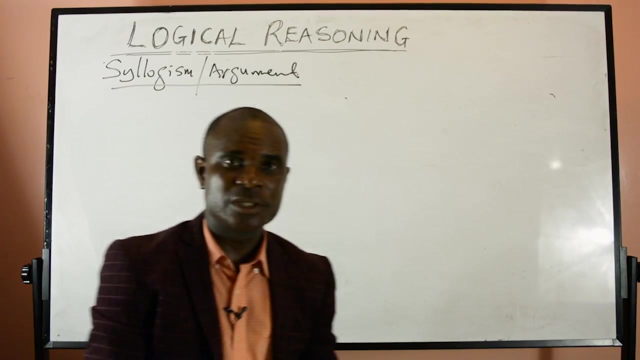 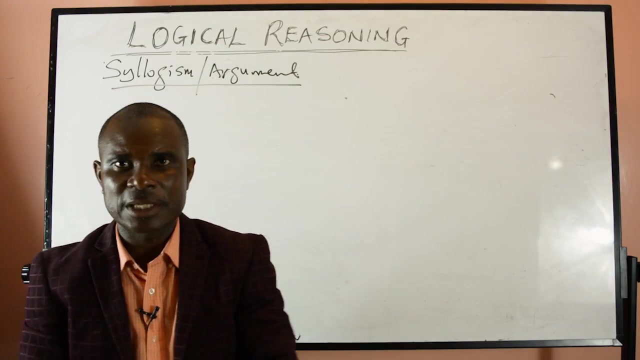 so let's call it syllogism. this is syllogism or arguments. we have to look at that argument. so an argument or a syllogism is a set of statements. you already know what a statement now. it is a set of statement that will, uh, conclude something. so what is that state of? 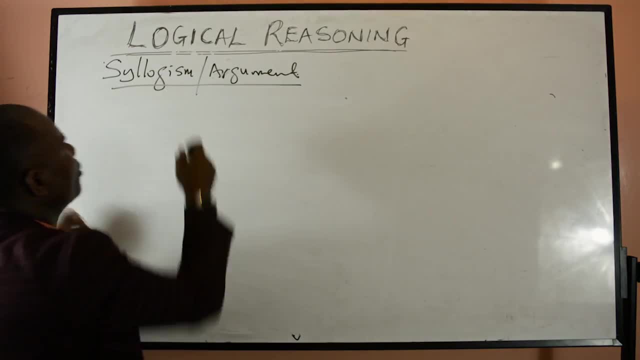 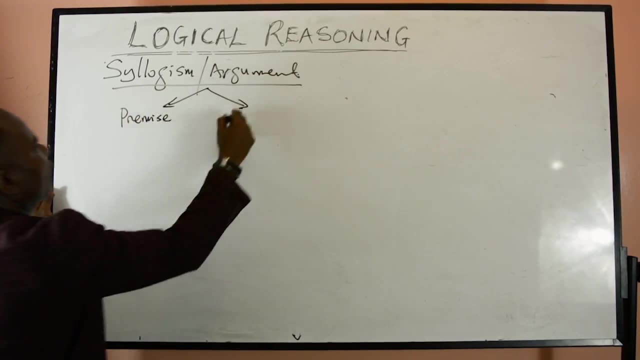 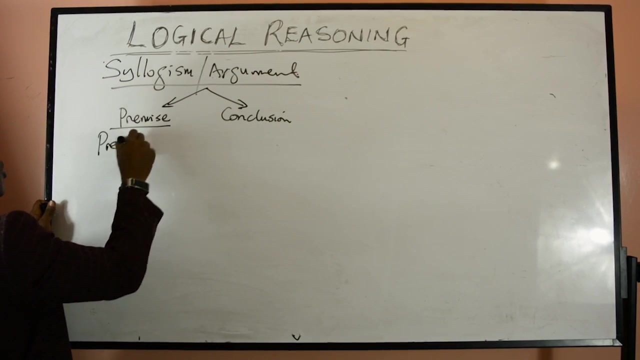 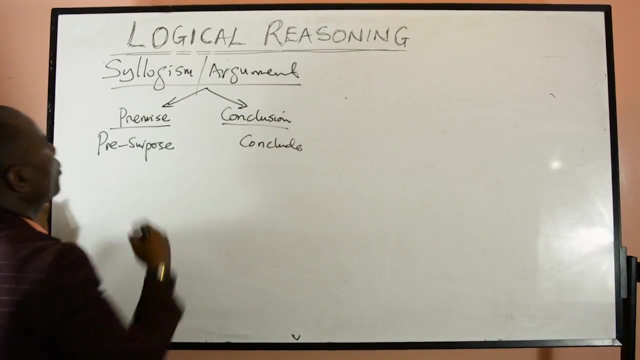 statement. it is divided into two. so an argument is divided into two. we have the premise part of the argument and you have the conclusion. the premise is what will presuppose, this is what we are going to presuppose and this is what we conclude. we conclude with this. so we have two parts of an argument. we have the premise part. 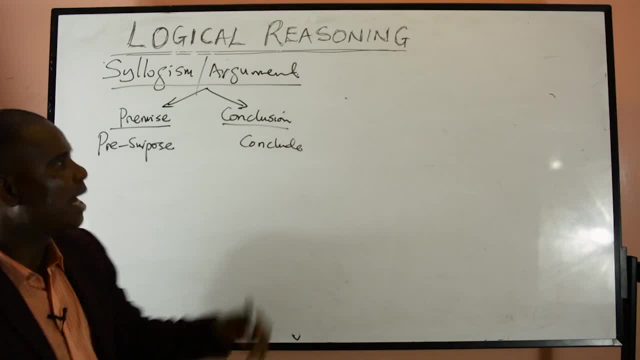 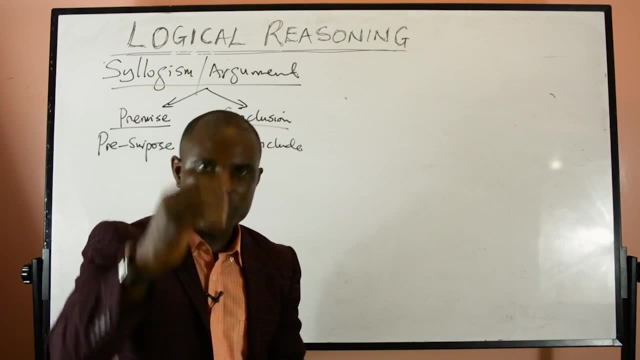 of the argument. i'll have the conclusion part of the argument, and a. an argument or syllogism is a set of statements, one of which is a conclusion which is drawn on the orders, on the basis of the orders, which are called the premise. so now we have the premise, part of the argument. 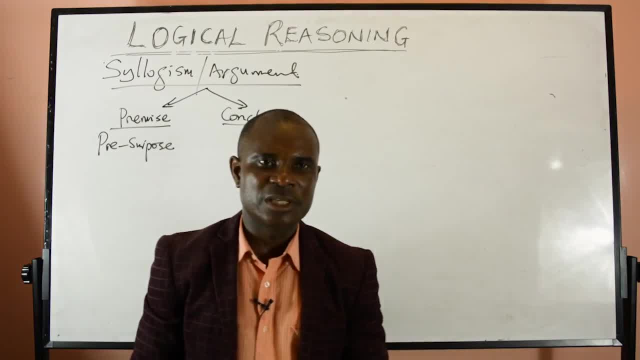 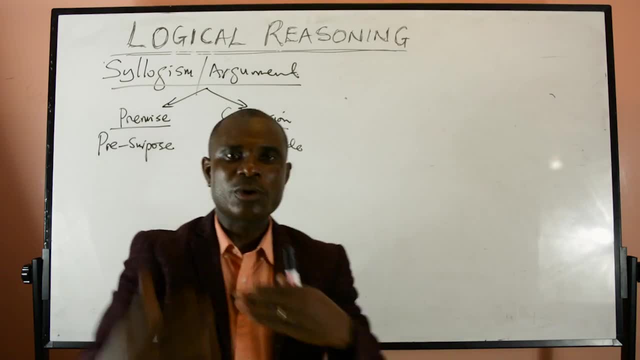 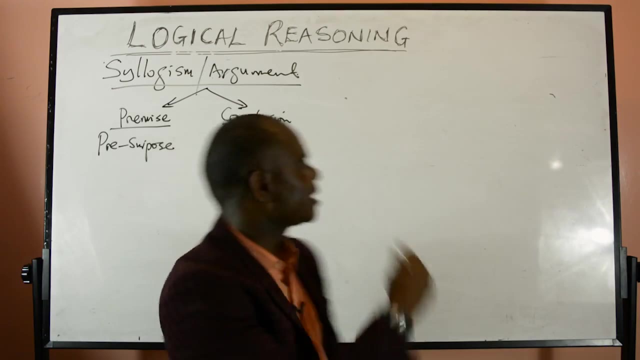 and you have the conclusion part of the argument. so the argument is normally of three statements. you have two of them are premises and the last one is the conclusion, and that conclusion is drawn from the premises. so the arguments can be divided into two. you have the presupposition, that is the 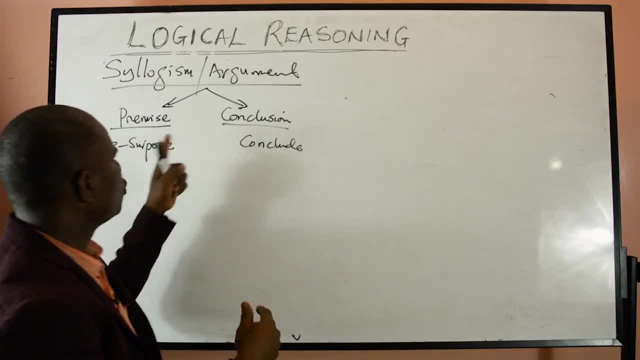 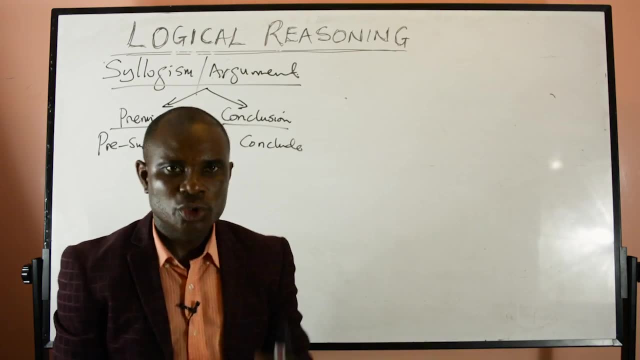 the premise, part of it the evidences, and now we can use those evidences to draw conclusion. that's what makes up an argument. well, once this argument don't have this part, there is not an argument. so an argument must have the following part: it must have two parts. first it must have 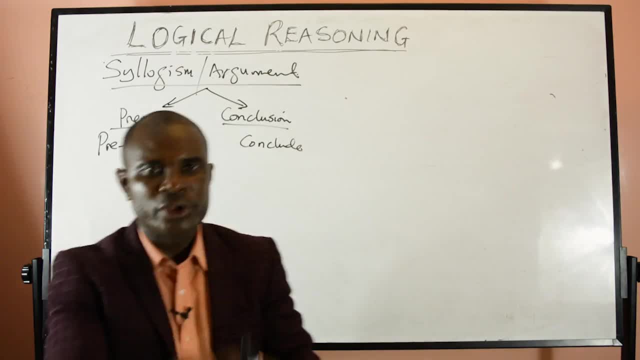 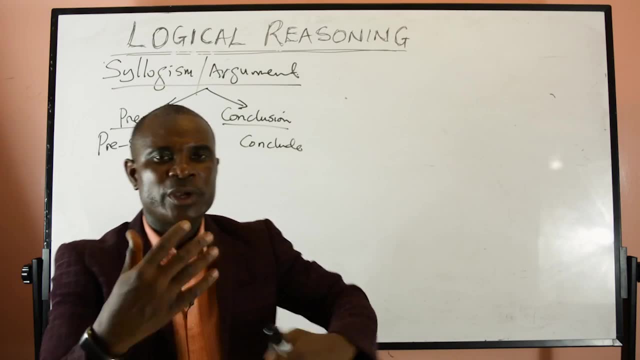 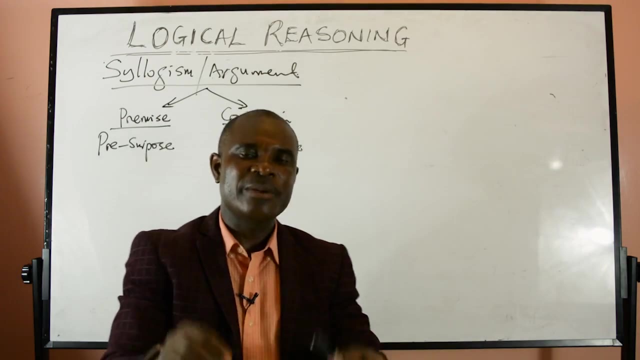 a premise part, that is what you please presuppose. oh, in other words the evidences or the, the, the premises we call them and we have. it is from those premises that we cannot conclude. the last one is normally what concludes and that conclusion is drawn from the premises. so that kind that this set of uh statements put together is what 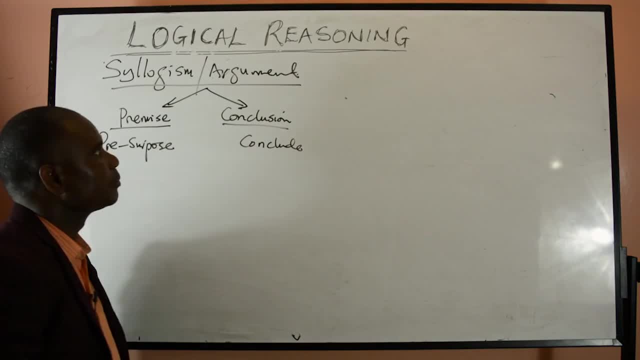 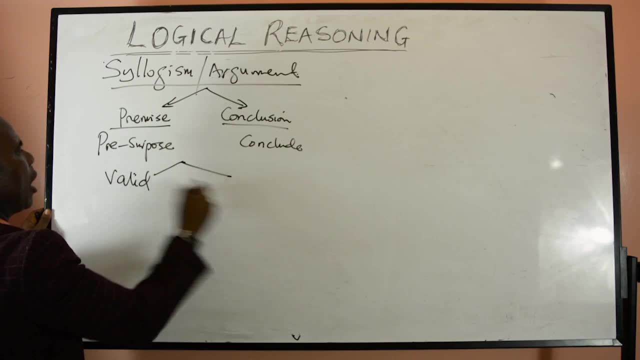 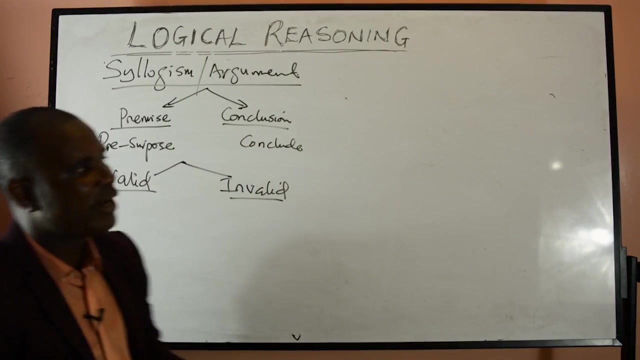 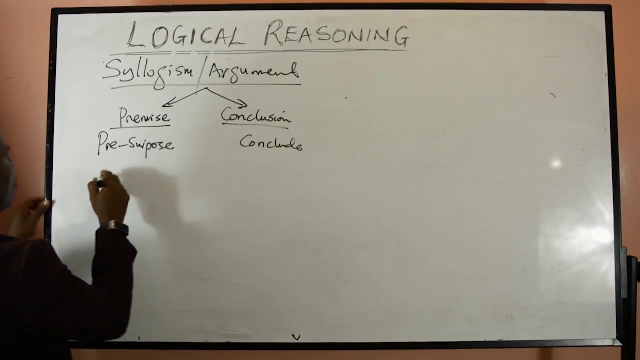 you call an argument. so we're going to look at the, the forms of arguments. we have valid argument and you have invalid arguments and you have valid arguments. what is a valid argument? a valid argument? first, let me let me give you an example of an argument. then we can know whether the argument is value or not. so i 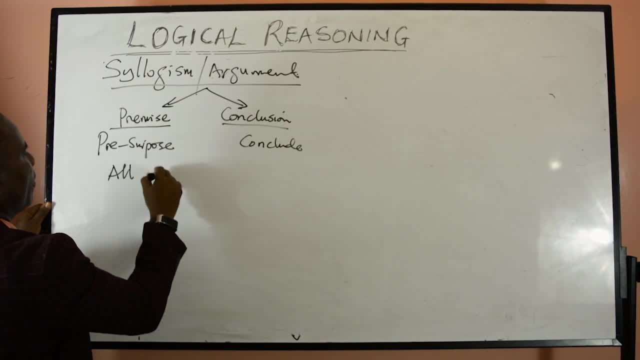 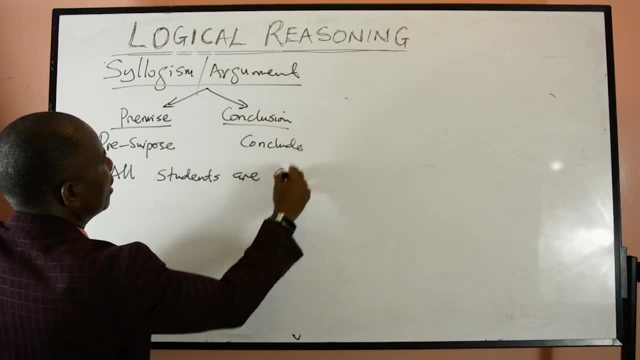 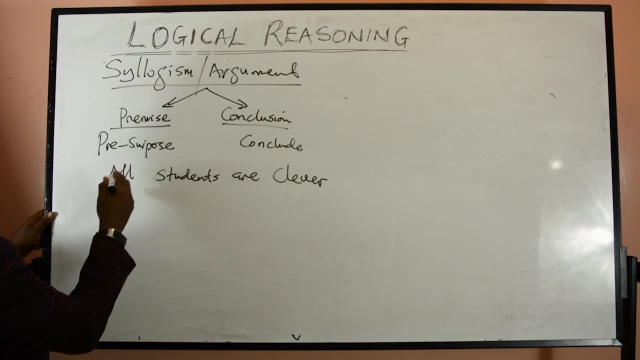 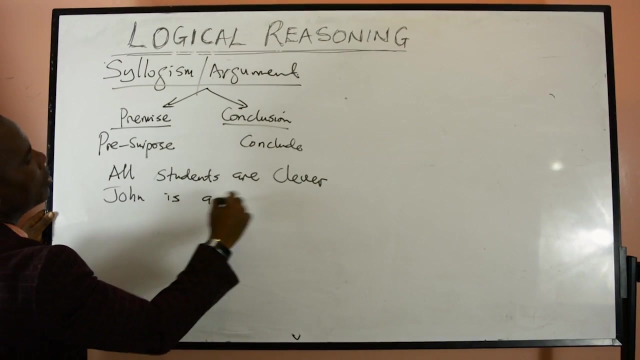 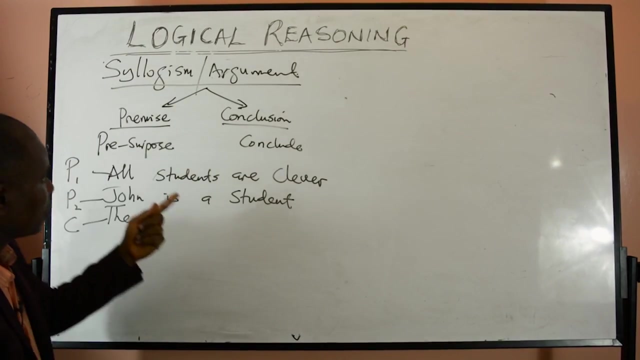 if i say all, all, all students are clever, then see, then some, okay, let's say, uh, john, i'm say after: john, john is a student, therefore also. so we have got one part. this is premise one. we have premise two. now we have the conclusion. so you can conclude from here that all students are clever and john is a student. so you. 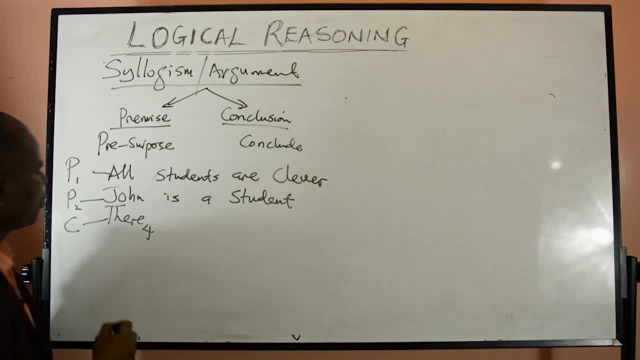 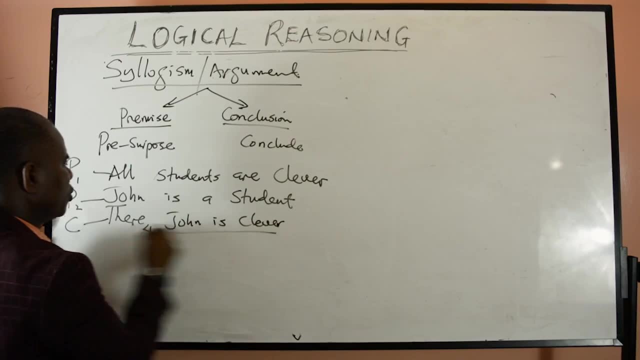 can therefore conclude that all students are clever and john is a student. so you can therefore conclude that all students are clever and john is a student. so you can therefore conclude that john, therefore john is clever. why did you conclude that john is clever? because there is a statement here that supports, or there. 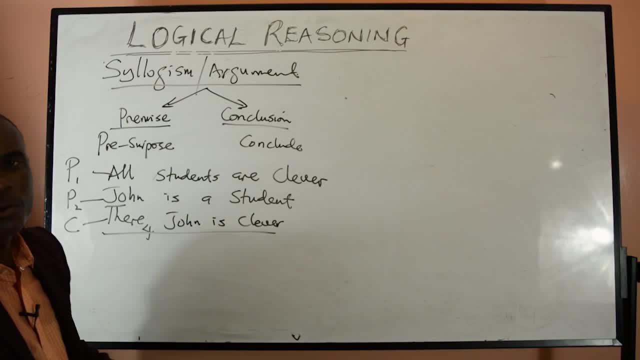 are statements here which are the premises which are supporting the conclusion. so this is an argument. an argument is having two parts. we have the premise part of it. this is the first premise. i will have the second premise. then you have the conclusion drawn from the premises there. this is a 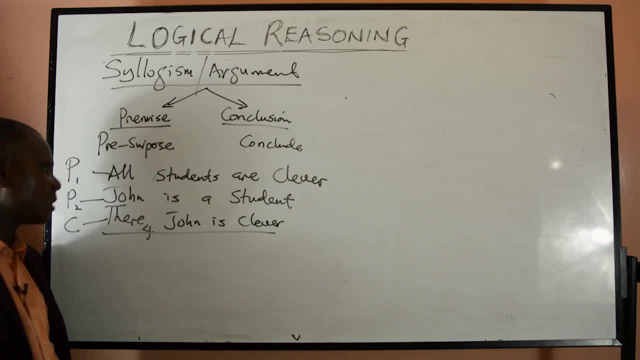 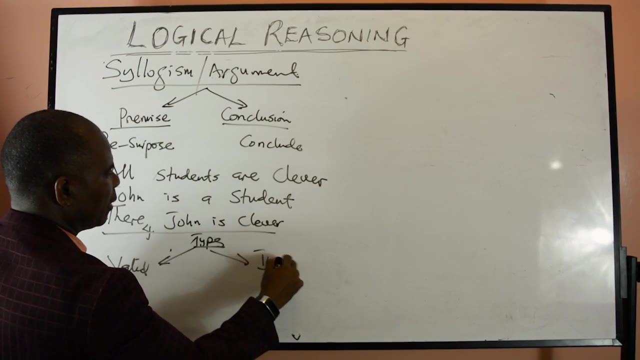 an argument. this is a set of statements put together to form an argument, and you don't know a typical example of an argument, so we can look at the, the types of arguments. we have types of arguments, we have a valid argument- valid argument- and you have an invalid argument- invalid. 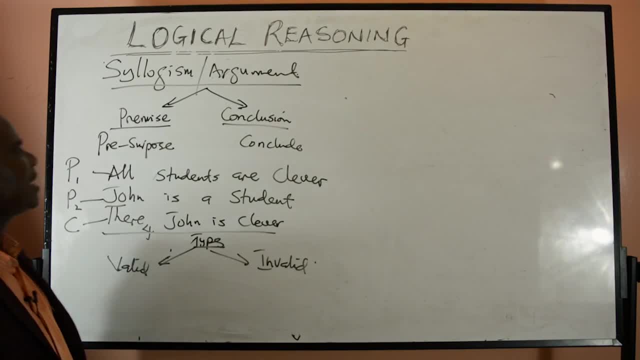 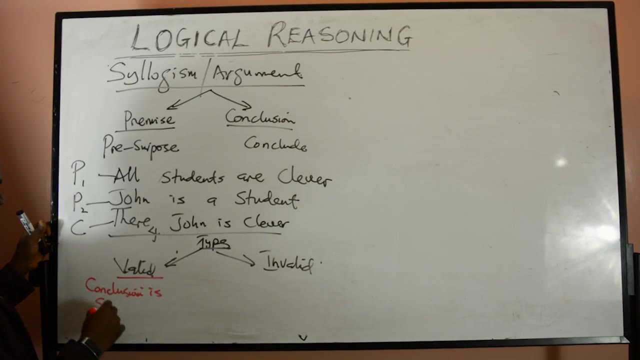 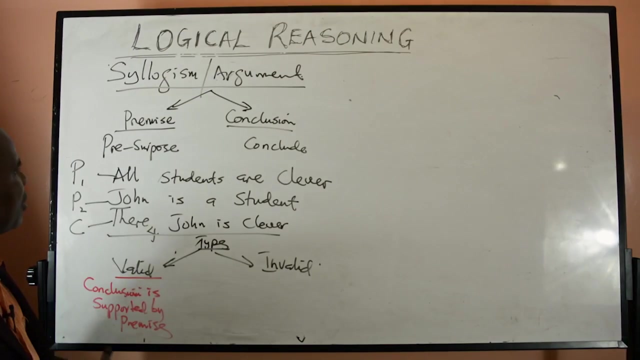 so what is a valid argument? a valid argument is that arguments, that is, each conclusion, is drawn from the premises. so if i draw the conclusion from the premises, conclusion is supported by the premises, supported by premises or evidences or the presuppositions here, and it is a kind of proposition. so in an argument you 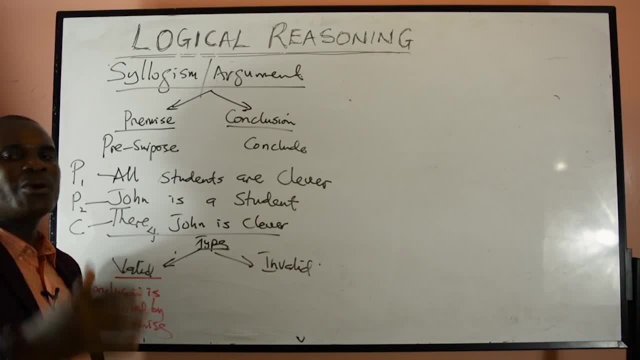 actually have three propositions. the first two propositions are called the premises and the last proposition is what is called the conclusion. so the first proposition is what is called the first premise and the second proposition is what is called the second premise and the stored proposition, which is normally the conclusion. so the the argument contains these three parts. it. 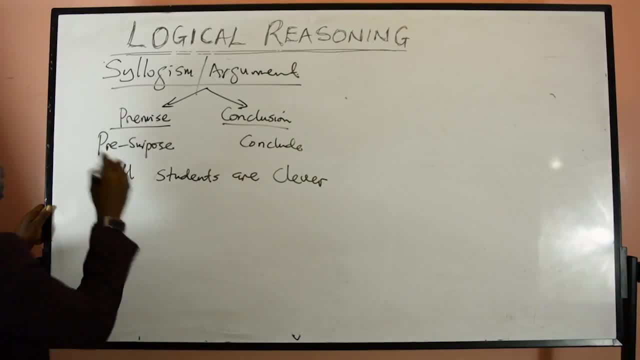 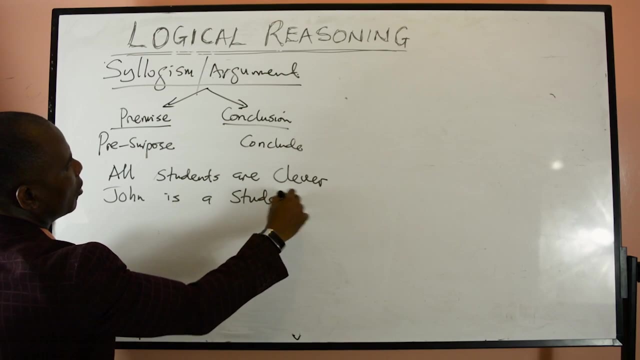 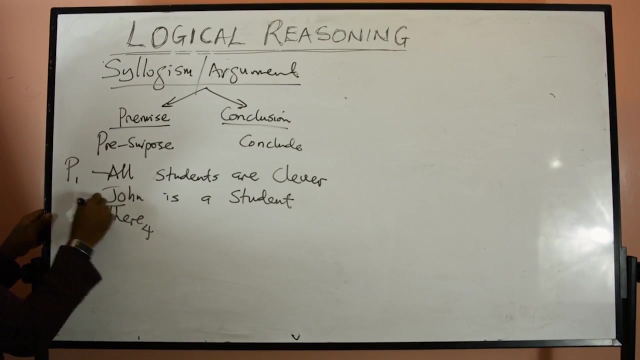 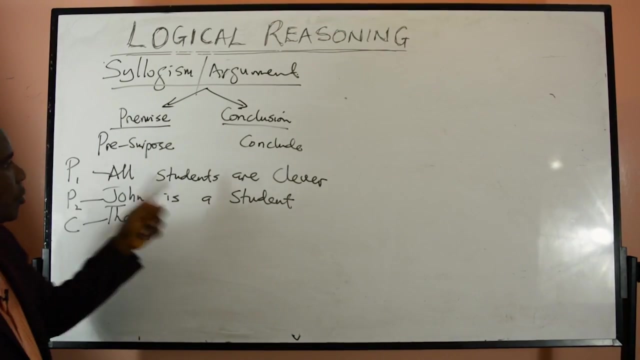 clever then see then. so okay, let's say John, I'm C after John, John is a student, therefore also. so we have got one part. this is premise one. we have premise two. now we have the conclusion. so you can conclude from here that all students are clever. I. 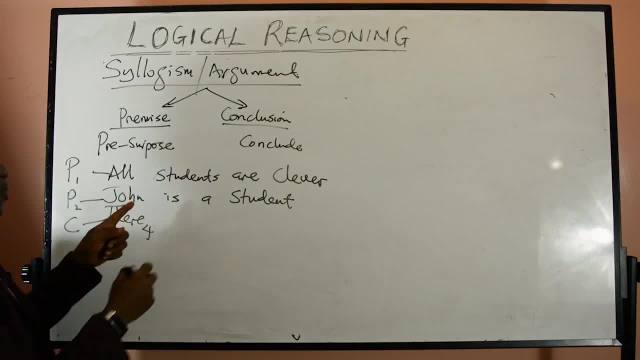 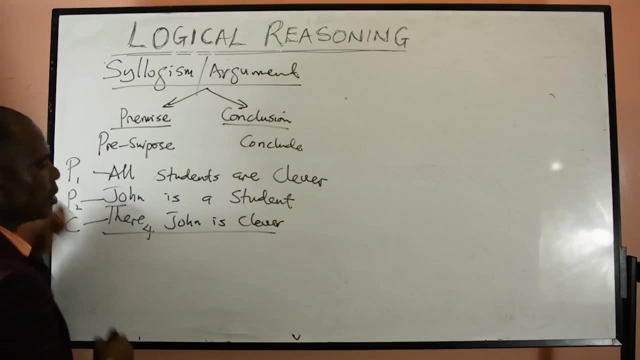 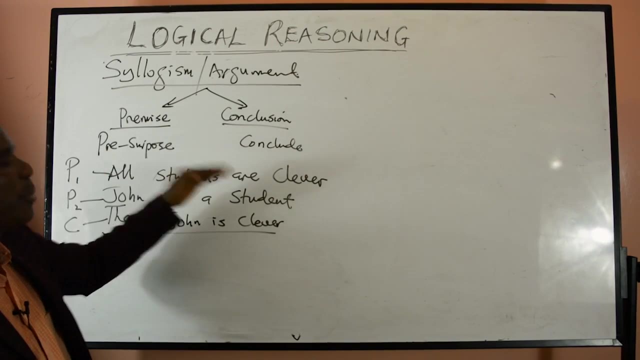 and John is a student. so you can therefore conclude that John, therefore John is clever. why did you conclude that John is clever? because there is a statement here that supports, or their statements here, which are the premises which are supporting the conclusion. so this is an argument. an argument is: 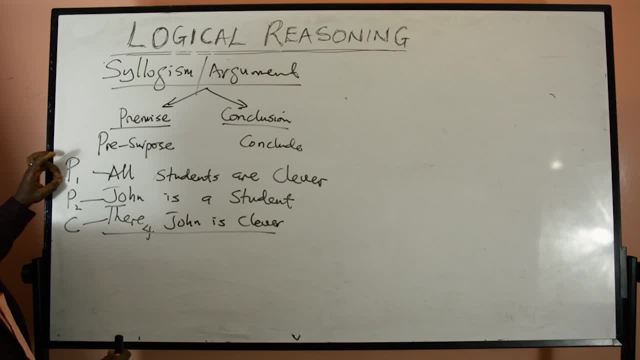 having two parts. we have the premise part of it. this is the first premise. I will have the second premise. then you have the conclusion drawn from the premises there. this is a an argument. this is a set of statements put together to form an argument, and you don't know a typical example of an argument, so we can look at the, the types of 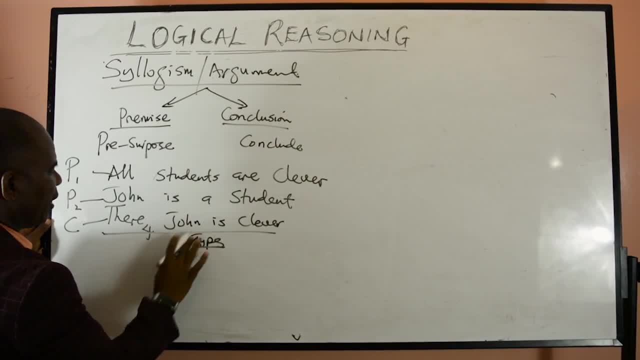 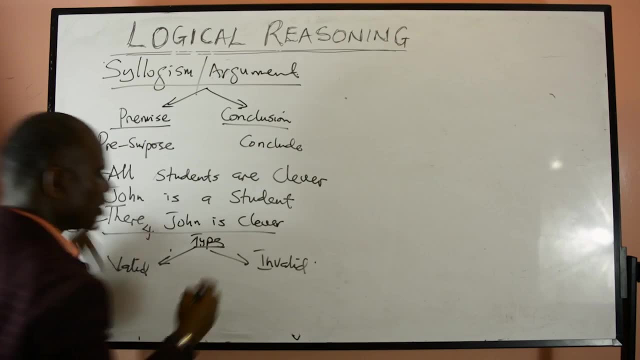 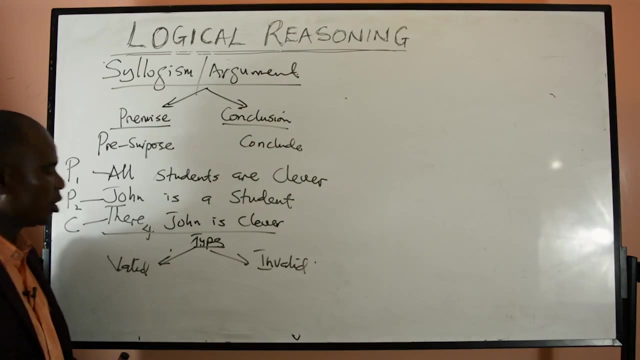 arguments. we have types of argument. we have a valid argument, valid argument. now you have an invalid argument, invalid. so what is a valid argument? a valid argument is that argument, that is, each conclusion is drawn from the premises. so if i draw the conclusion from the premises, conclusion is supported by the premises. supported by premises. 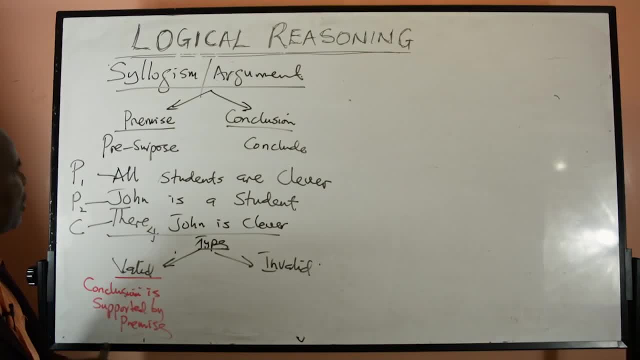 or evidences or the presuppositions here, and it is a kind of proposition. so in an argument you actually have three propositions. the first two propositions are called the premises and the last proposition is what is called the conclusion. so the first proposition is what is called the first premise and the second proposition is what is called the second premise and the 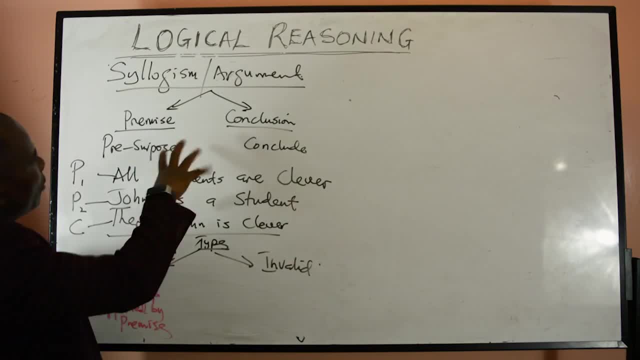 third proposition, which is normally the conclusion. so the, the, the argument contains these three parts: it must have a premise, it must have two premises and the last statement must be that conclusion. so this, when we are not looking at the types of arguments, so if the, the valid arguments and 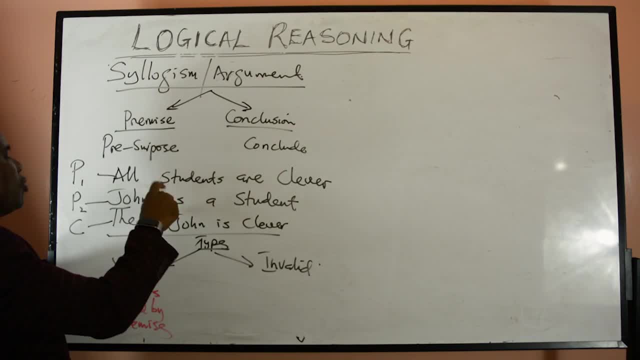 must have a premise, it must have two premises and the last statement must be that conclusion. so this, when we are not looking at the types of arguments. so if the the valid argument and invalid argument, you want to differentiate between the two. so a valid argument is a kind of argument. 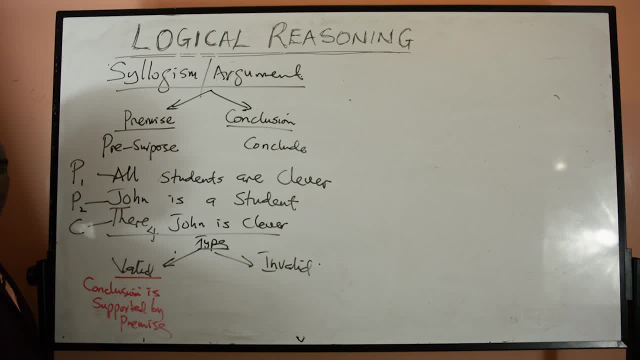 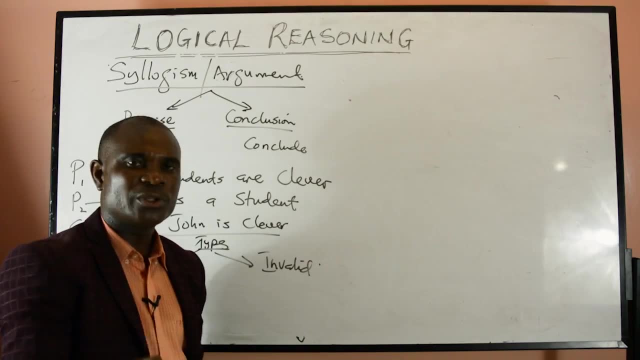 in which the argument is completely different. the argument is quiet. eat the argument so that the conclusion is supported by the premise. In other words, the conclusion is drawn from the support of the evidences. If the evidences are supporting, the conclusion, is supported by the evidences. 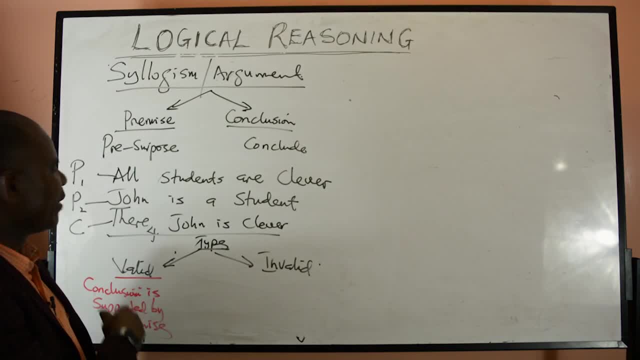 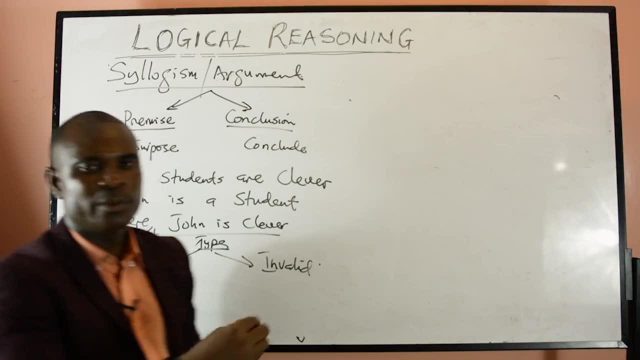 then we can say: or the premises. we can say the argument is already valid. When the conclusion is drawn on the basis of the premises, then we can now say that argument is valid. But if I draw a conclusion which is not supported by the evidences, 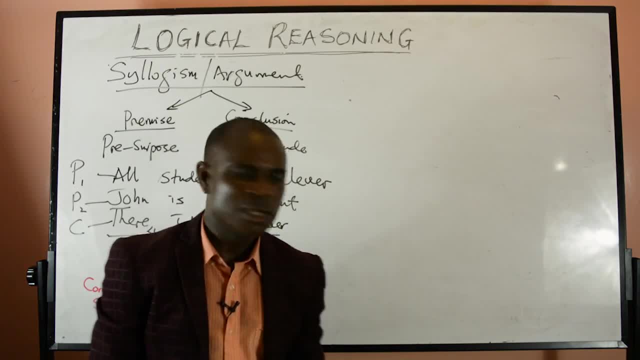 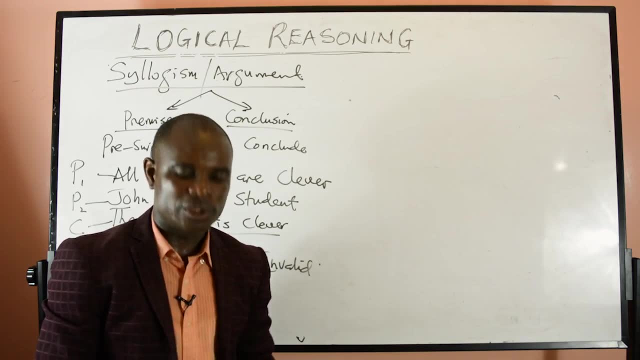 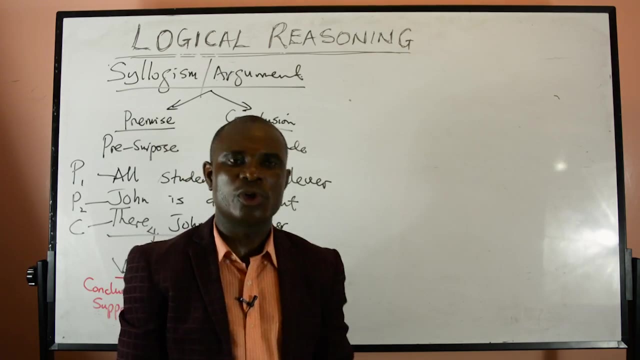 then that concluded argument is going to be an invalid argument. so we can distribute between valid arguments and invalid argument based upon the way the premise behave with the conclusion. if the premise supports the conclusion, then we can say that that argument is valid. it means that the conclusion has been drawn on the basis of the premise. but if the conclusion is drawn, 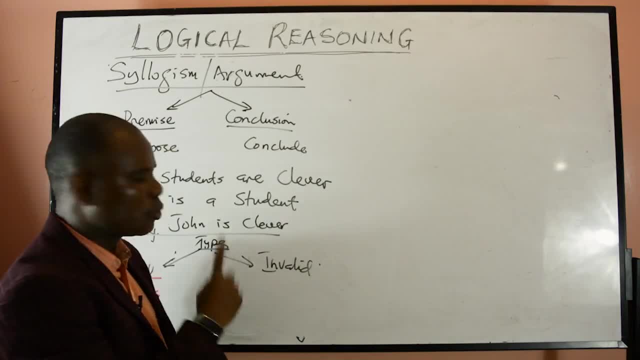 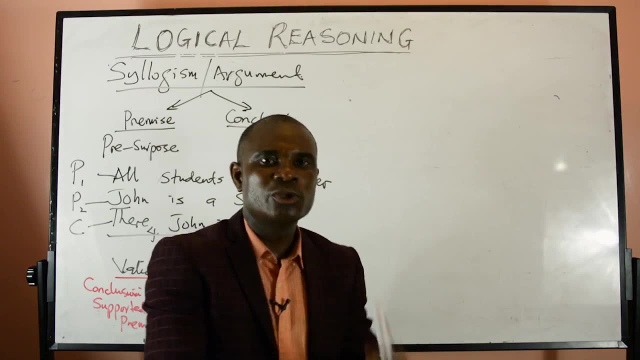 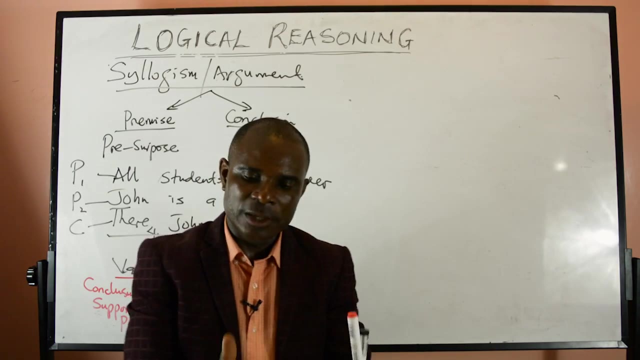 not on the basis of the premise, then we can conclude that that particular argument is invalid. so an invalid argument is the one whose assertion, which, whose conclusion, is drawn on the basis that the premises they do not support that argument do not support the conclusion. if the the the conclusion is in deviant with the premises, then we can conclude that this: 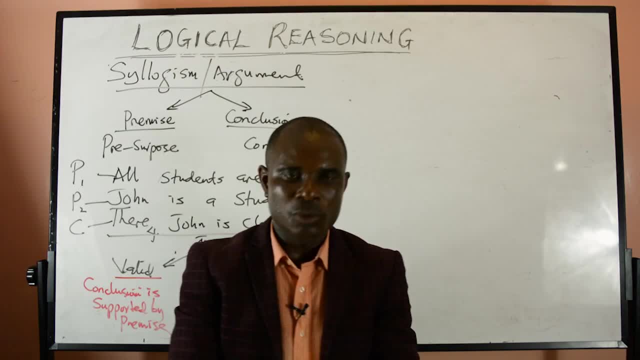 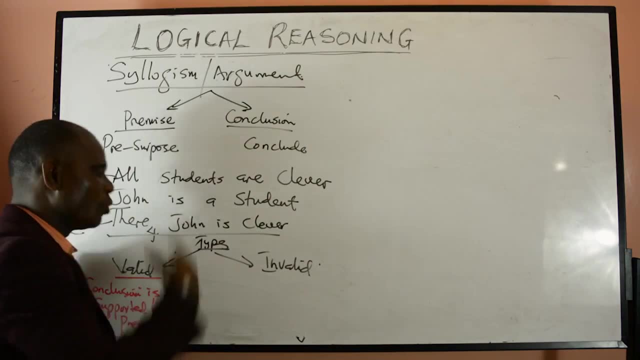 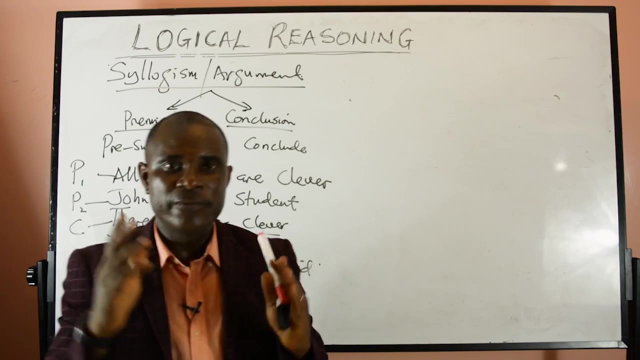 particular argument is invalid. but if the the premise, the conclusion is drawn on the support given by the premise, then we can say the argument is valid. now you know the difference between the two. now it doesn't matter whether the argument, whether the premises are true or not. the fact here is that 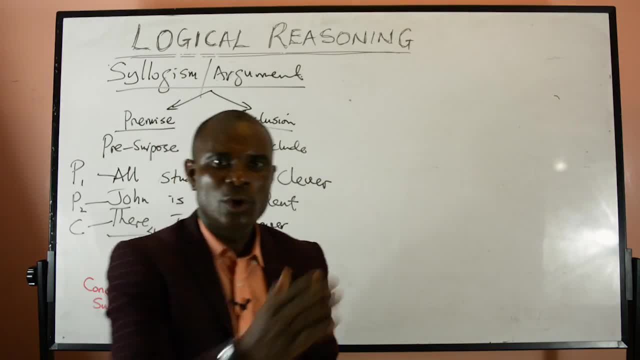 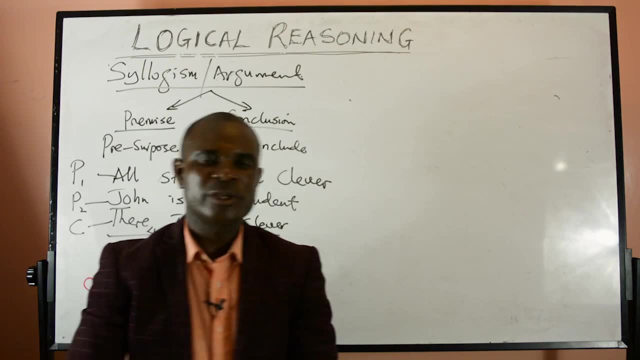 for as much as the premises support the argument, then we can see the conclusion. if the conclusion is drawn from those premises, then we can see the argument is uh valid, irrespective of the fact that the the premises are not true, but for as much as those premises are supporting the conclusion. 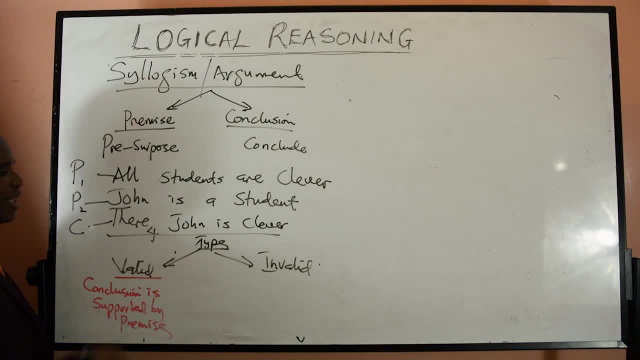 arguments are valid arguments and the valid arguments are valid arguments and the valid invalid argument. We want to differentiate between the two. So a valid argument is a kind of argument in which the conclusion is supported by the premise, In other words, the conclusion is drawn. 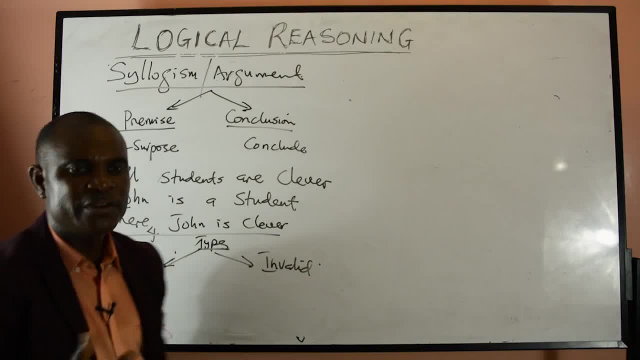 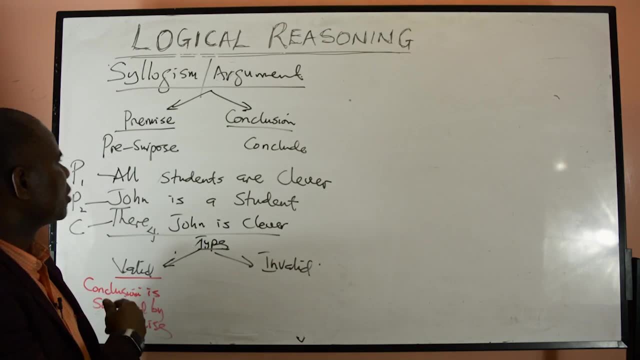 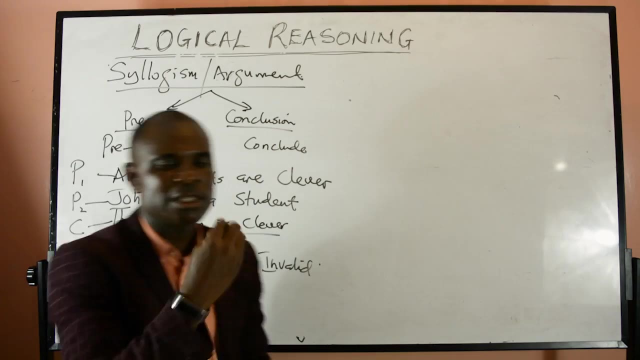 from the support of the evidences. If the evidences are supporting the conclusion is supported by the evidences, then we can say: or the premises. we can say the argument is already valid. When the conclusion is drawn on the basis of the premises, then we can now say that argument is. 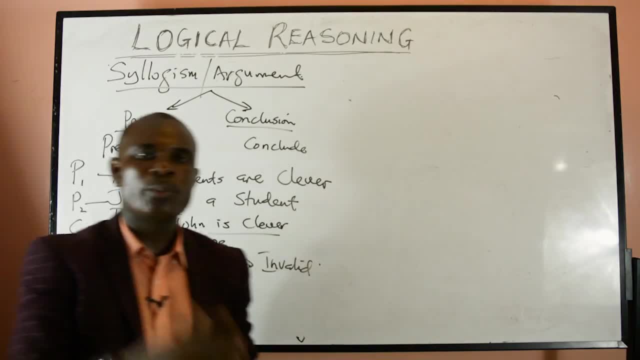 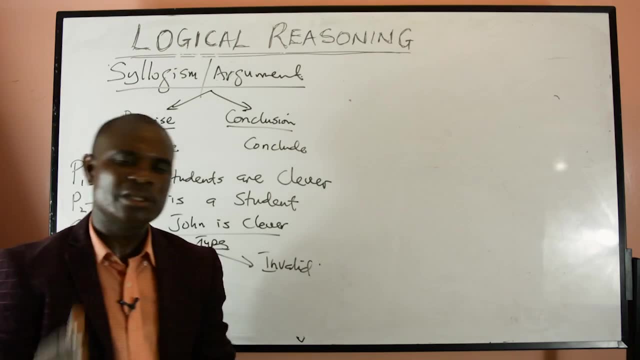 valid. But if I draw a conclusion which is not supported by the evidences, then that argument is going to be an invalid argument. So we can distinguish between valid arguments and invalid arguments based upon the way the premise behaves with the conclusion. If the premise supports the 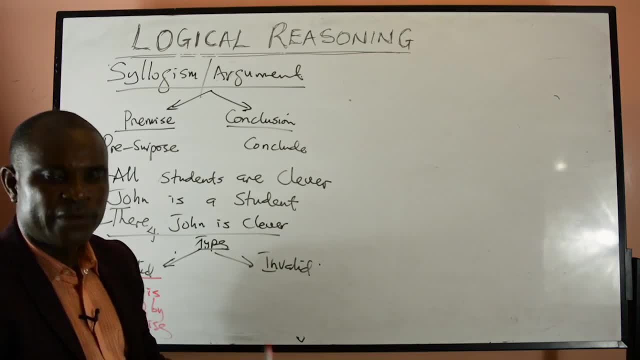 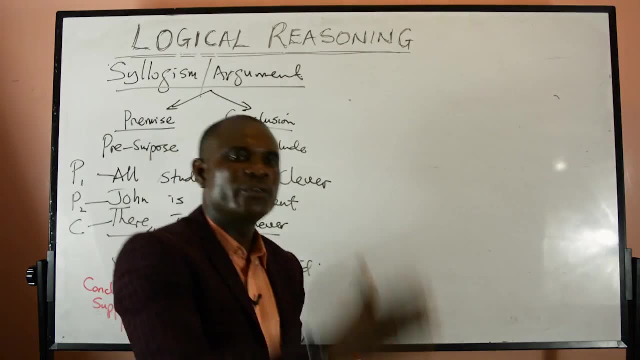 conclusion, then we can say that that argument is valid. It means that the conclusion has been drawn on the basis of the premise. But if the conclusion is drawn not on the basis of the premise, then we can conclude that that particular argument is valid. 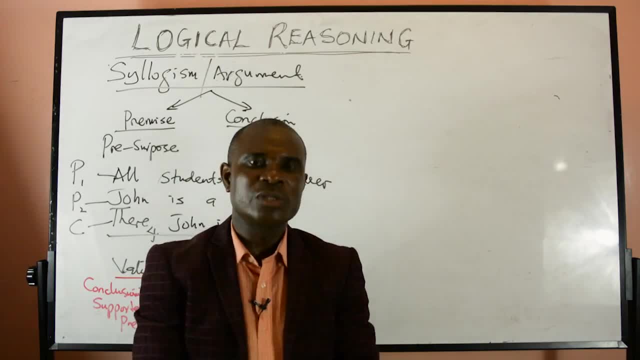 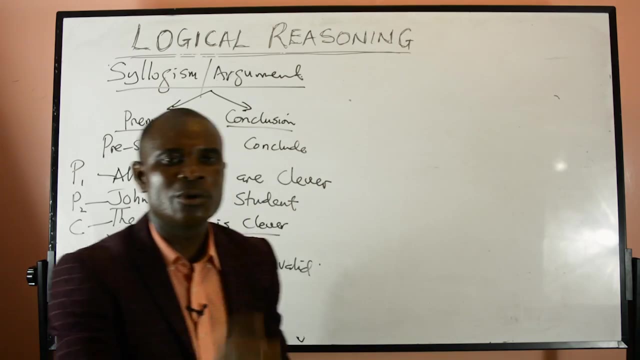 So an invalid argument is the one whose assertion, whose conclusion, is drawn on the basis that the premises do not support that argument, do not support the conclusion. If the conclusion is indiviant with the premises, then we can conclude that this particular argument is invalid. But if 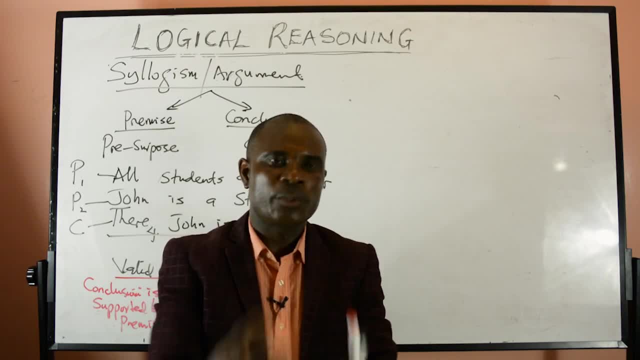 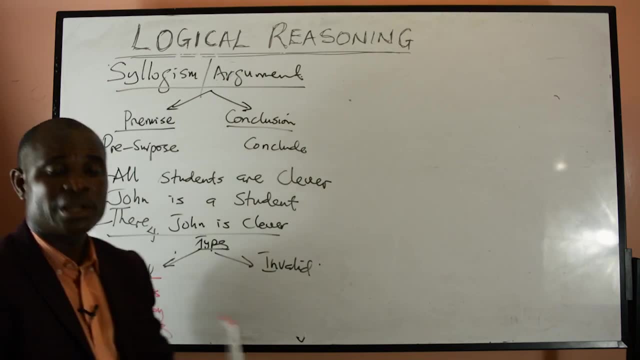 the premise. the conclusion is drawn on the support given by the premise. then we can say: the argument is valid. Now you know the difference between the two. Now it doesn't matter whether the argument, whether the premises, are true or not. The fact here is that 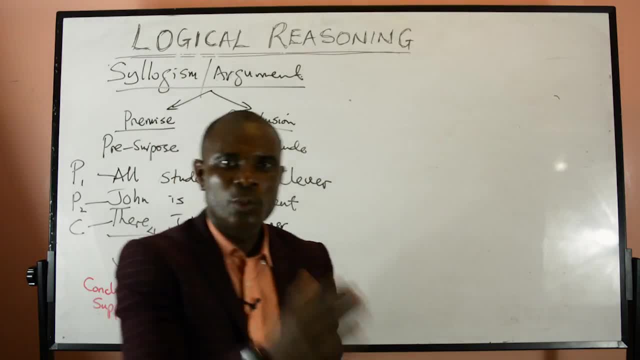 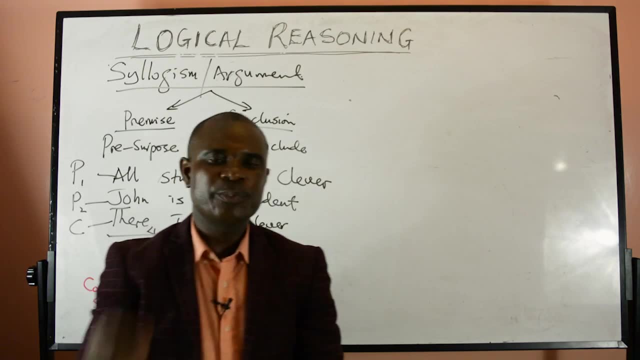 for as much as the premises support the argument, then we can say the conclusion. if the conclusion is drawn from those premises, then we can say the argument is valid Irrespective of the fact that the premises are not true, But for as much as those premises are supporting the conclusion. 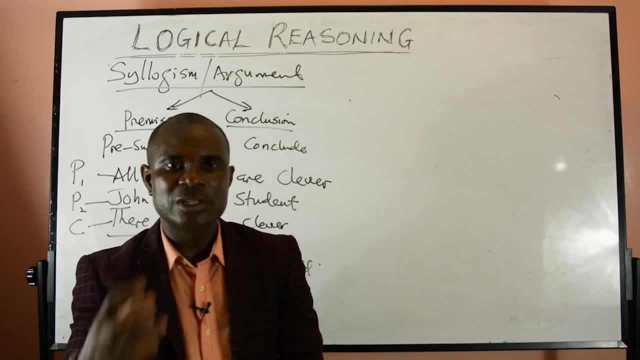 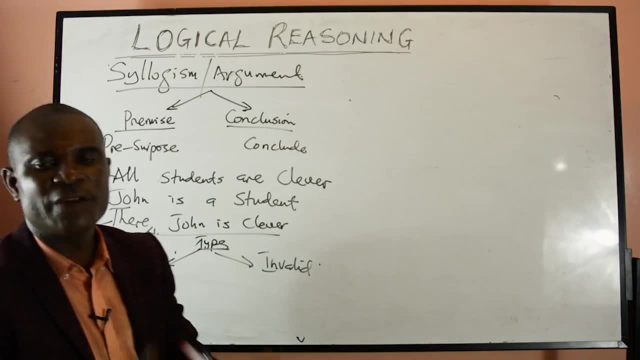 then that valid conclusion can be a valid argument, Meaning the conclusion is now supported by the premises. It doesn't mean that the premises have to be true or not, But for as much as the premises support the conclusion, then we can say the argument is valid. 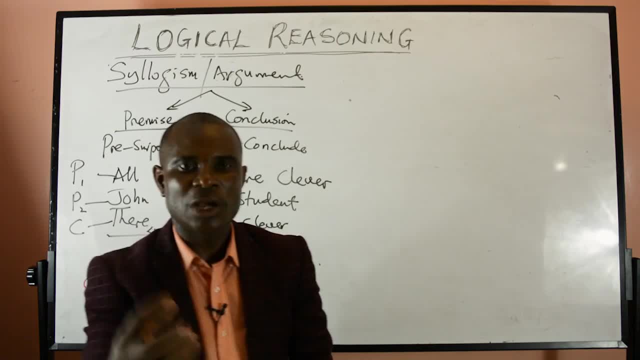 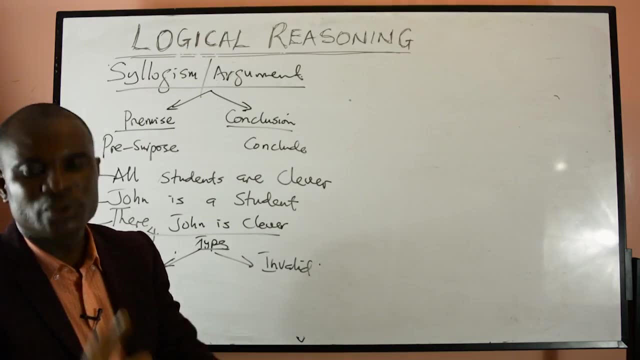 then that valid conclusion can be a valid argument, meaning the the conclusion is now supported by the premises. it doesn't mean that the premises have to be true or not, but for as much as the premises supports the conclusion, then we can say the argument is valid. yeah, so now we have this. we 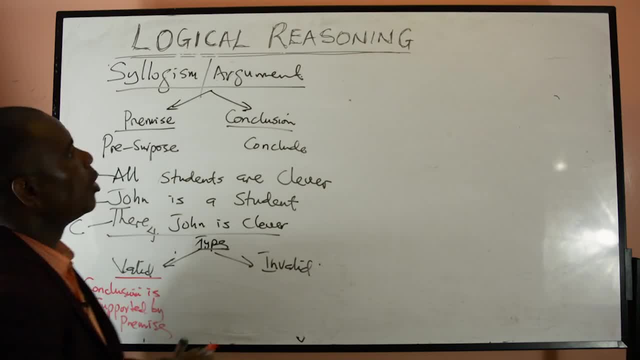 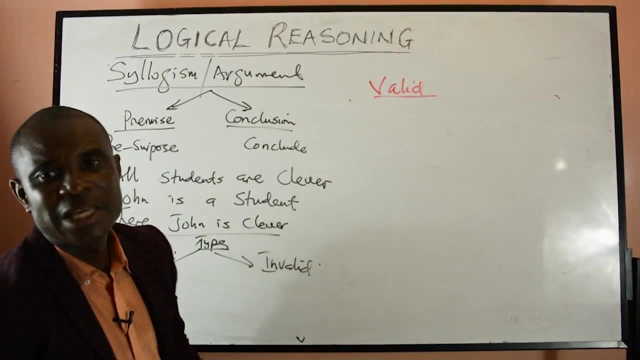 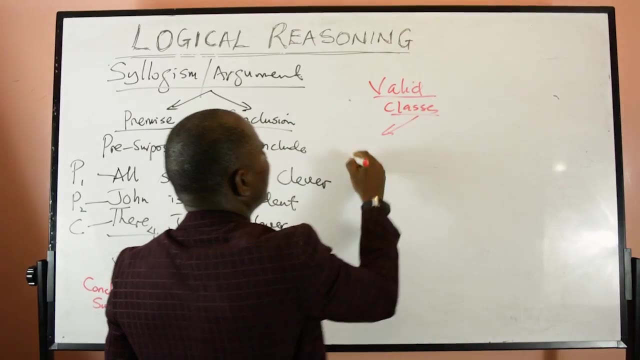 have this there. we have the distinction between the two. now let's look at the form of what we are going to do: much more of validity. we are going to dwell much more on valid arguments. now a valid argument can be further classified into the classes. we look at it. we have deductive argument. 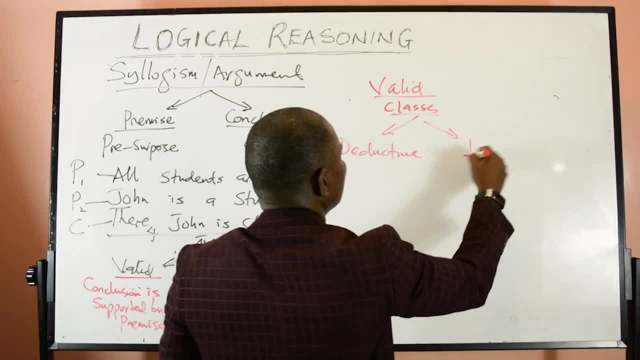 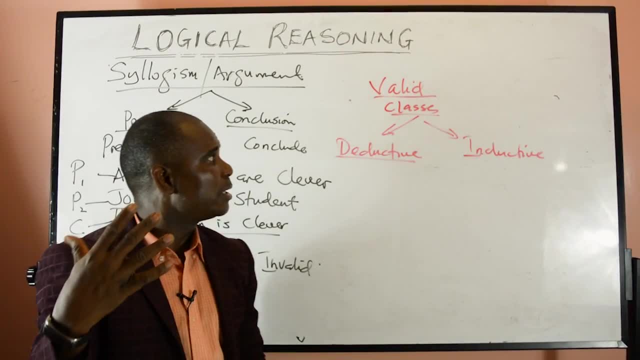 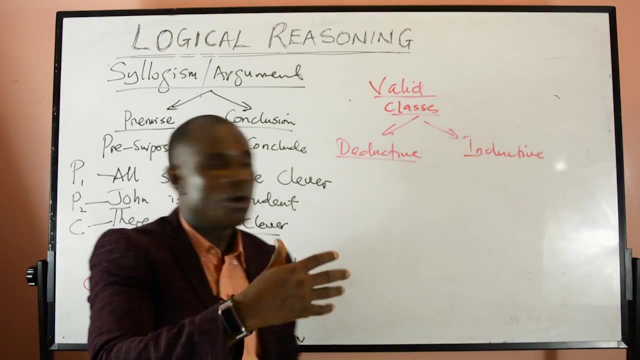 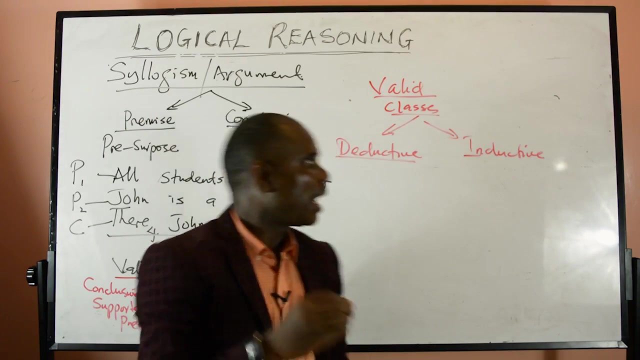 deductive argument and also inductive argument. you have inductive and deductive argument now it it is actually a valid argument. but if the valid argument through a situation in which the validity of that argument is based upon the fact that the truth of the premises are absolutely drawn from the truth or the truth of the conclusion, 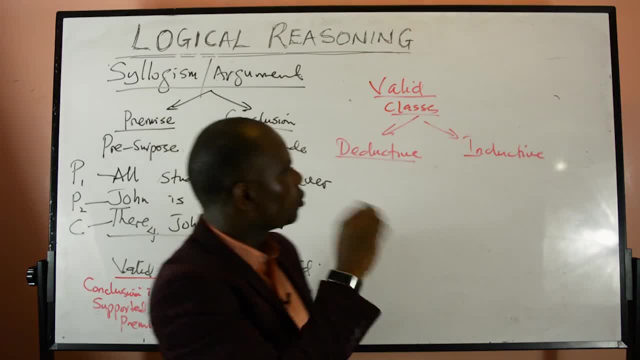 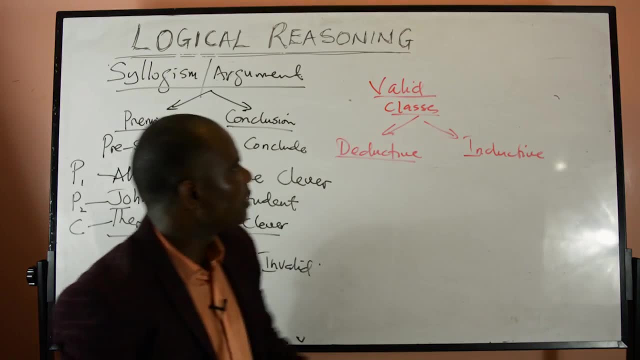 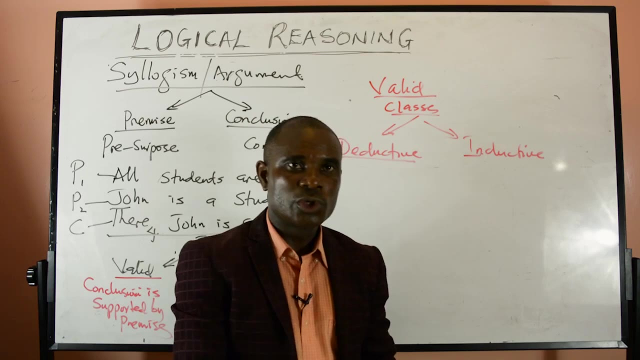 is absolutely dependent upon the truth of the, the truth, the true nature of the premise that we can say is a deductive conclusion. so what's that it means, if it's a valid statement? first of all, its validity is based upon the fact that its truth values, its premises, are going to be given based 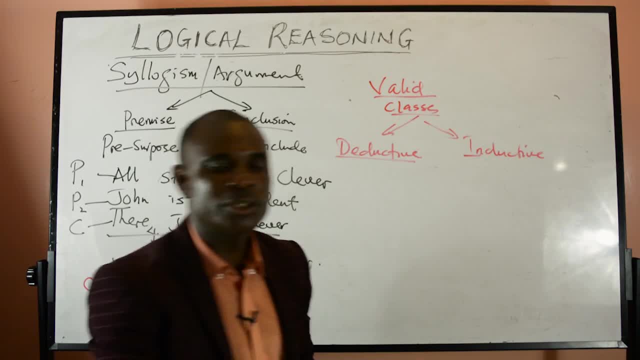 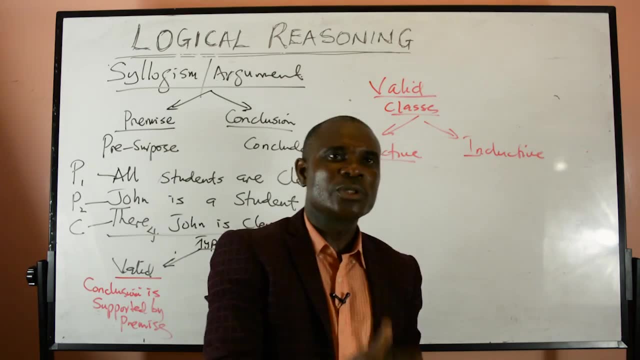 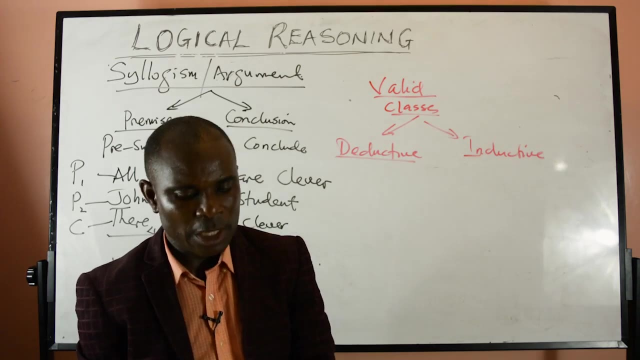 upon the truth nature of the conclusion. you cannot say: the conclusion is valid and when the premises are absolutely going to be valid, then if the the premises are absolutely valid, then the conclusion are also, with the conclusion also going to be valid, absolutely. so that is what we, we we conclude. 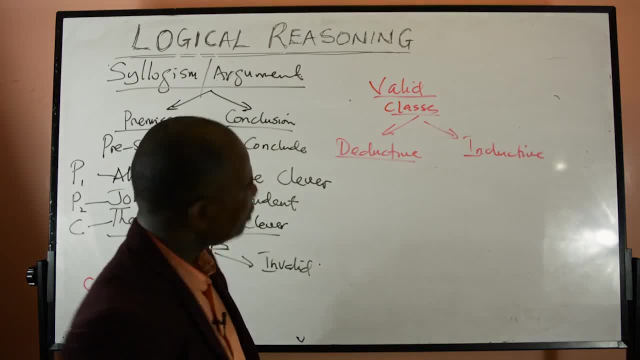 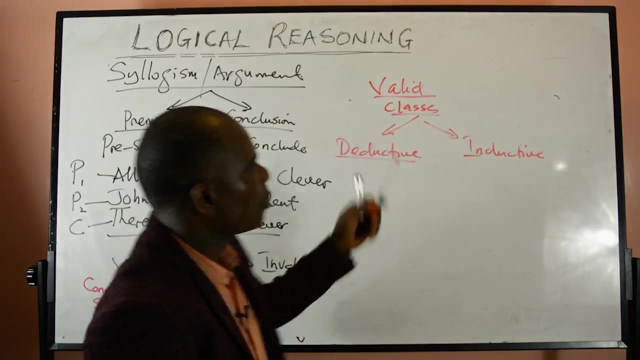 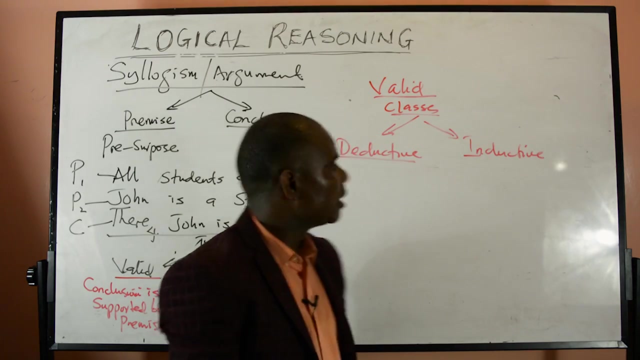 and we put together as a deductive argument, is the kind of argument in which the truth of the premises is absolutely guaranteed by the truth of the conclusion. so if the truth of the premises of the conclusion, that we can call it an inductive of argument, this one, the truth. 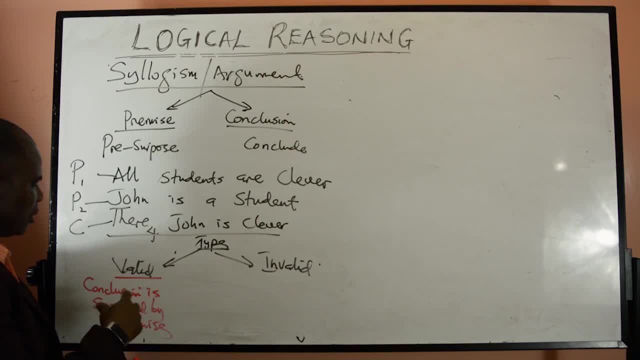 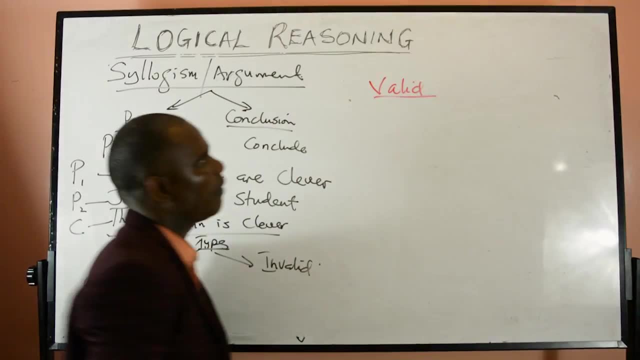 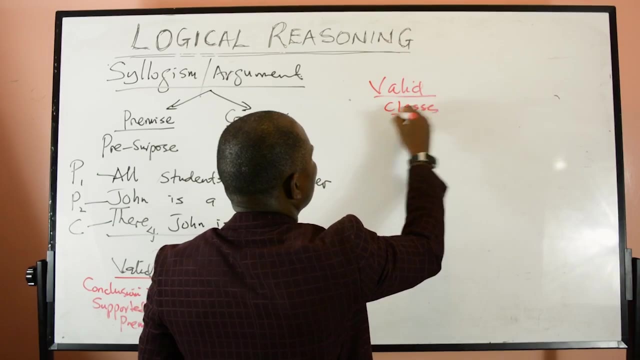 So now we have the distinction between the two. Now let's look at the form of. we are going to dwell much more on validity. We are going to dwell much more on valid arguments. Now a valid argument can be further classified into the classes. We look at it. We have deductive 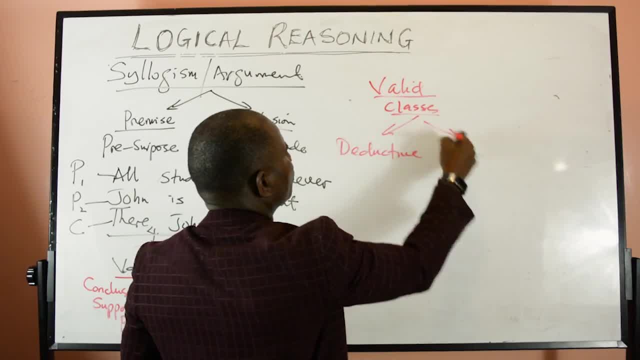 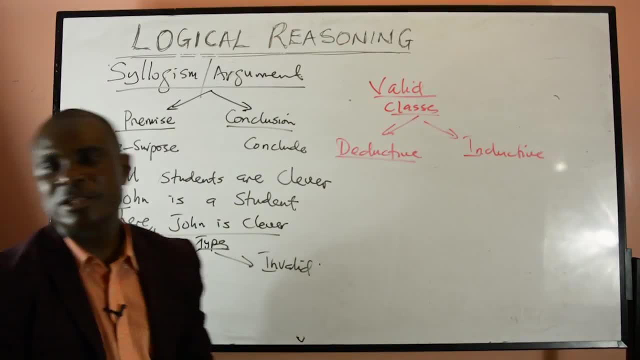 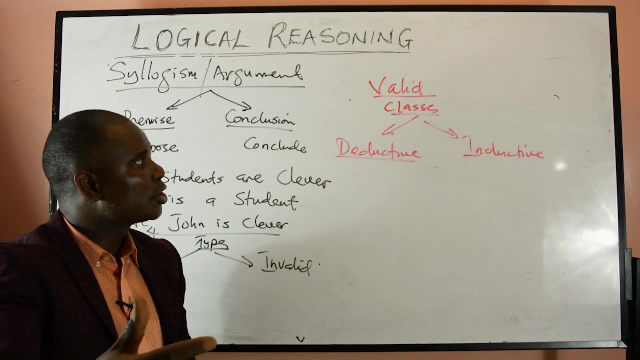 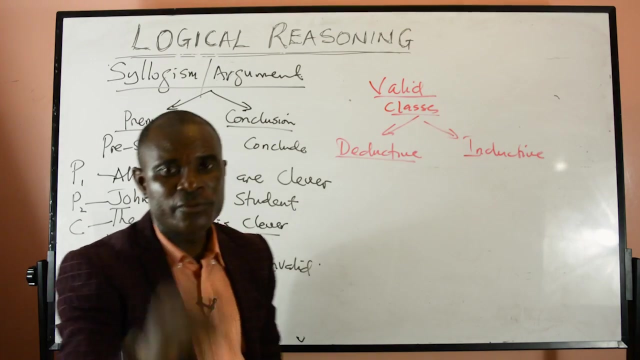 argument. We have deductive argument and also inductive argument. We have inductive and deductive argument. Now it is actually a valid argument. But if the valid argument through a situation in which the validity of that argument is based upon the fact that the truth of the 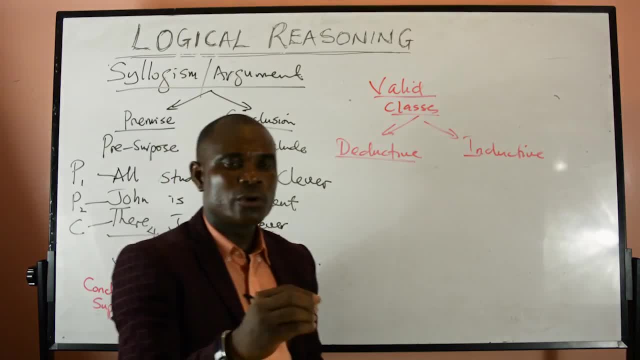 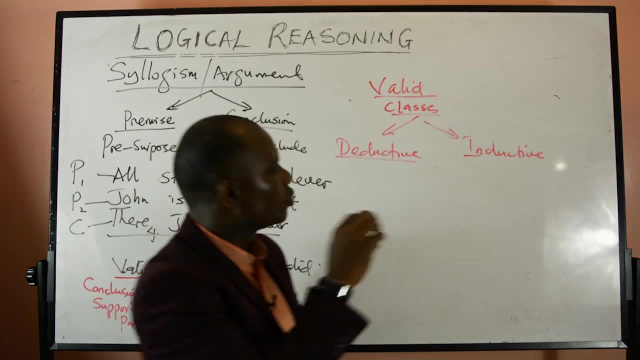 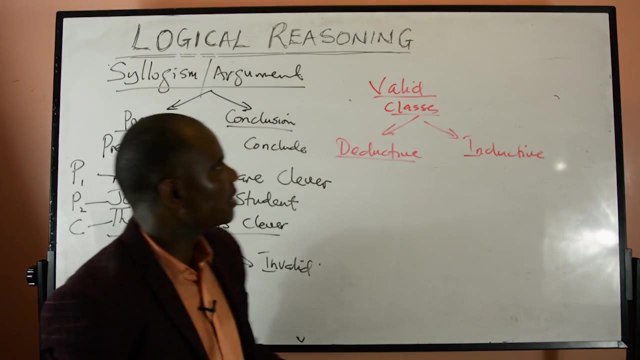 premises are absolutely drawn from the truth or the truth of the conclusion, then the argument of the conclusion is absolutely dependent upon the truth of the, the true, the true nature of the premise that we can say is a deductive conclusion. So what's that It means, if it's? 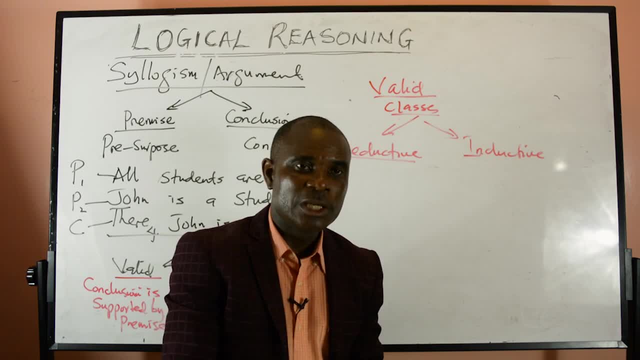 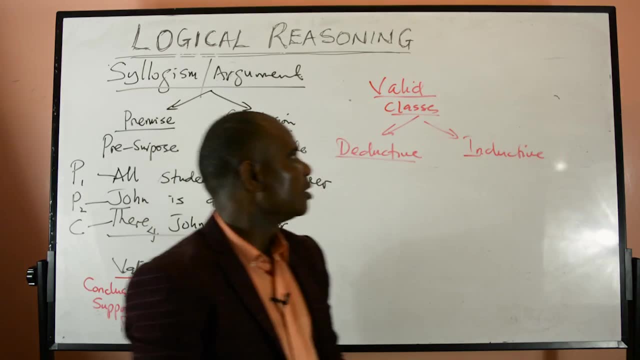 a valid statement. first of all, its validity is based upon the fact that its truth values, its premises, are going to be given based upon the truth nature of the conclusion, You cannot say the conclusion is valid And when the, The, The, 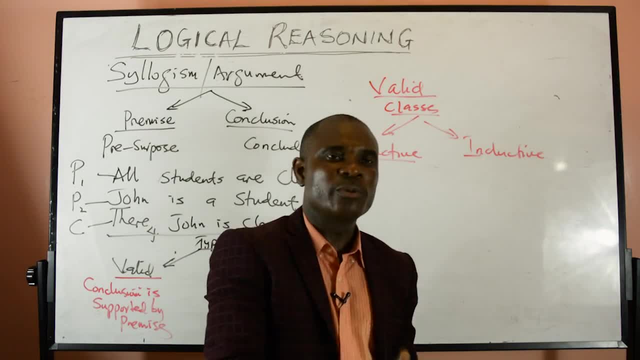 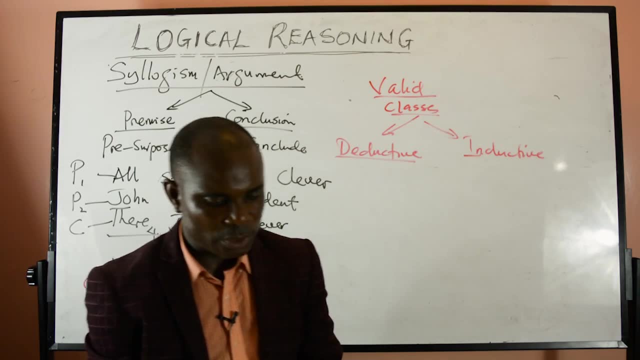 The. The premises are not valid, The premises are absolutely going to be valid. Then if the premises are absolutely valid, then the conclusion are also. the conclusion is also going to be valid Absolutely. So that is what we, we, we conclude and we put together as a deductive. 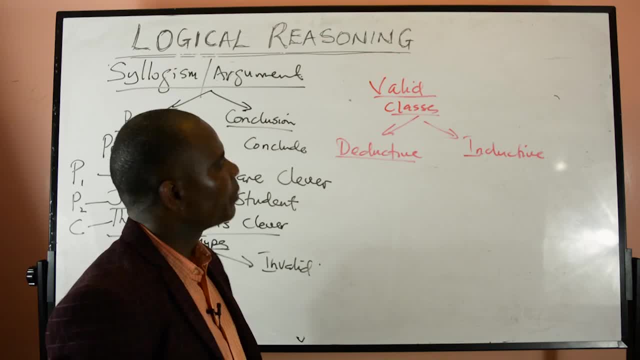 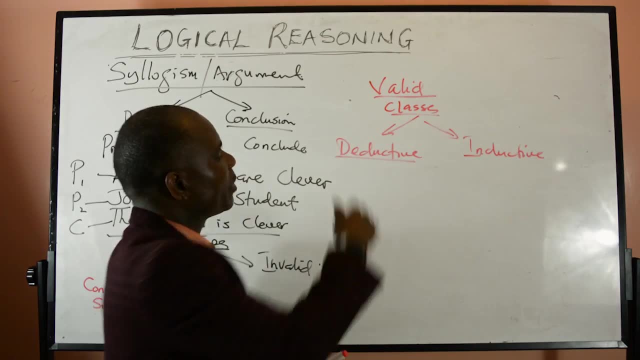 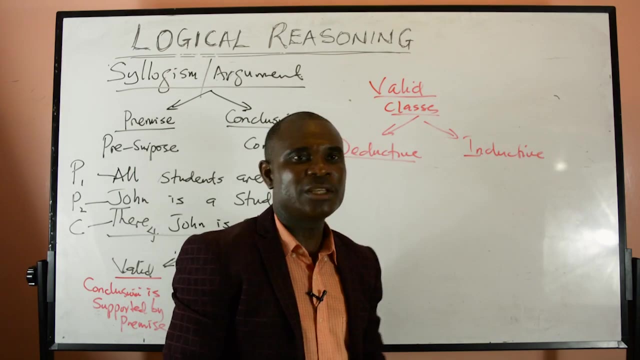 argument. It's the kind of argument in which the truth of the premises is absolutely guaranteed by the truth of the conclusion. So if the truth of the premises do not guarantee the truth of the conclusion, the validity of the conclusion, then we can call it an inductive. 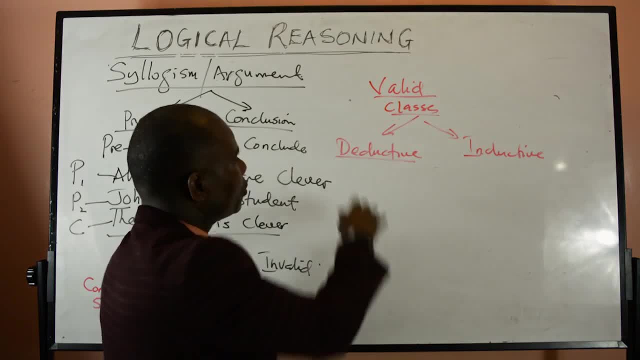 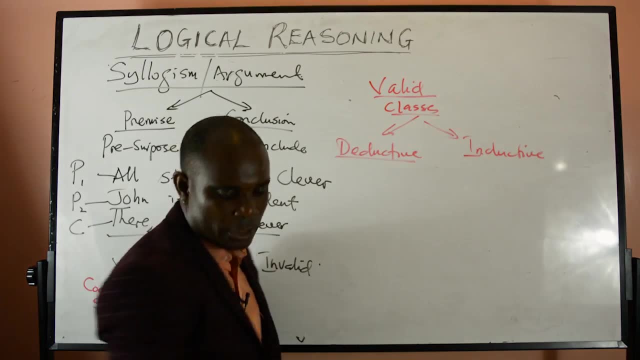 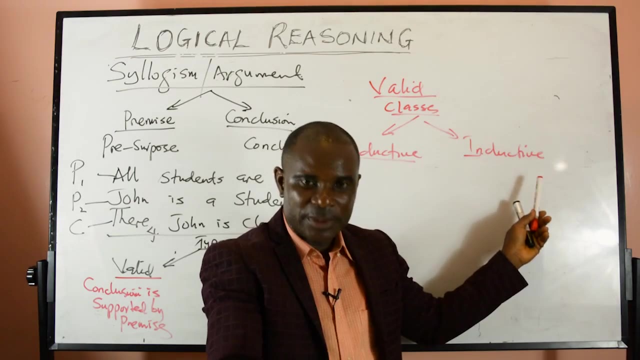 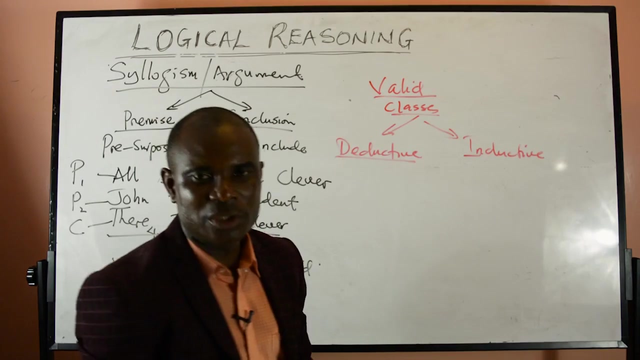 argument, This one, the truth of the premises absolutely guarantees the truth of the conclusion, Then we can now say the, we can now say it is deductive. But if the truth of the premises do not absolutely guarantee the truth of the conclusion, then that argument is called inductive. 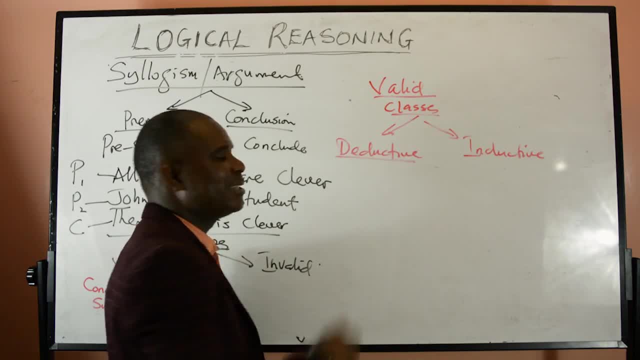 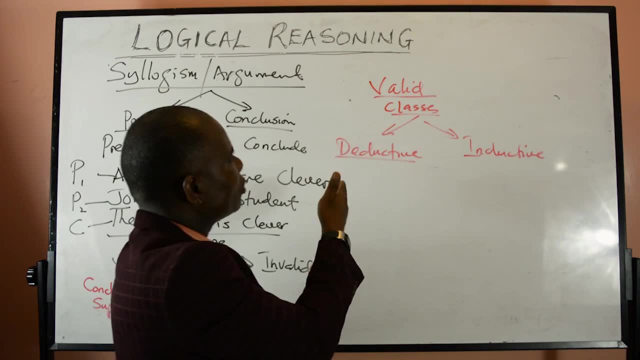 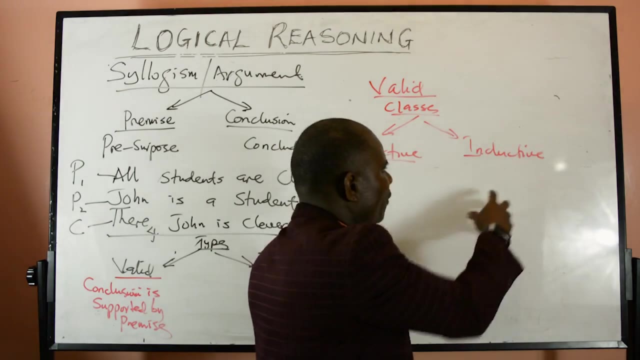 of the premises absolutely guarantees the truth of the conclusion, then we can now say the we can now say it is deductive. but if the truth of the premises do not absolutely guarantee the truth of the conclusion, then that argument is called inductive argument. so now we want to distinguish between the 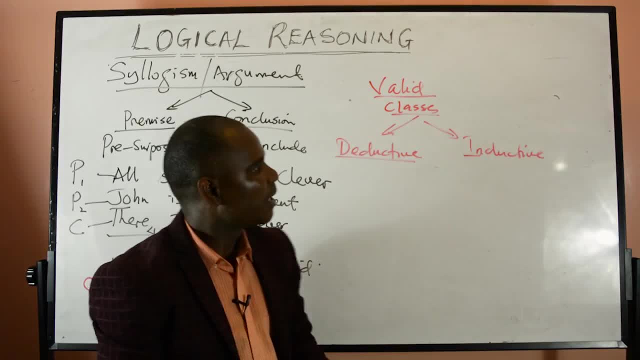 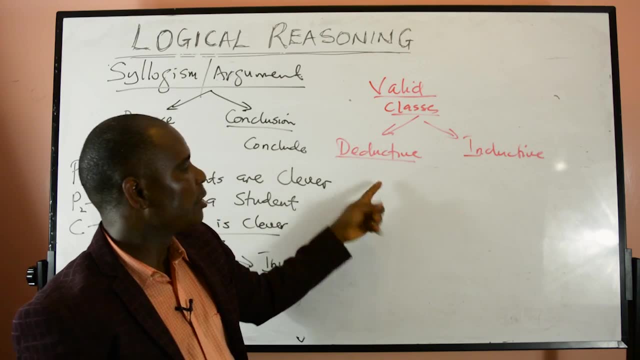 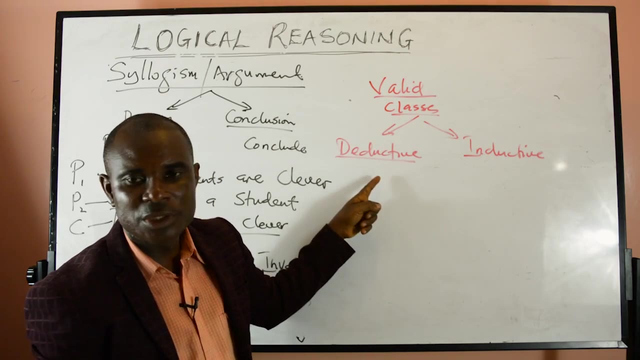 two, as I've already said. so what was that in? in in deductive argument, we said that it is first of all good to be valid and the truth of the premises is absolutely going to determine. it's absolutely good to determine the truth nature of the conclusion, but if the truth of the premise do not absolutely. 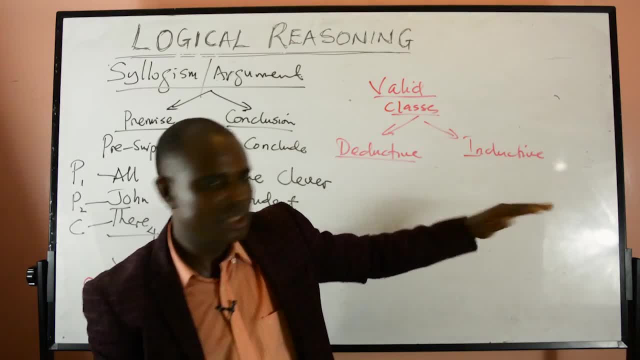 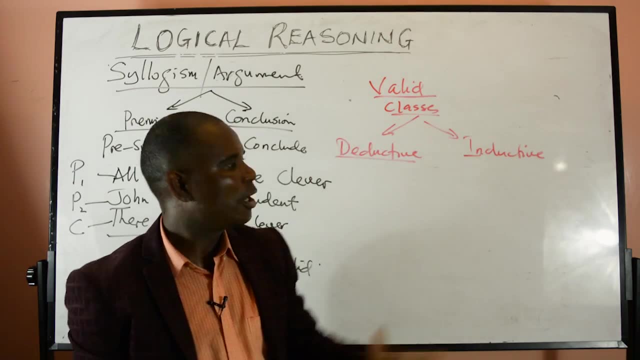 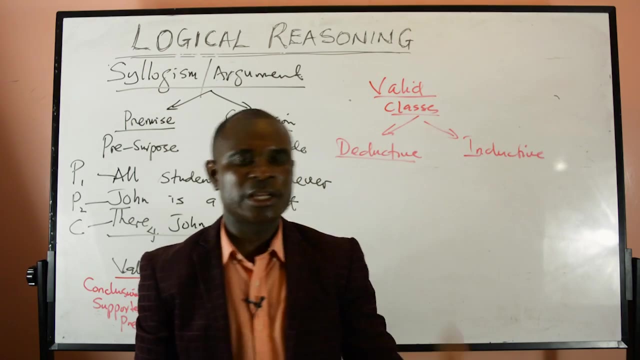 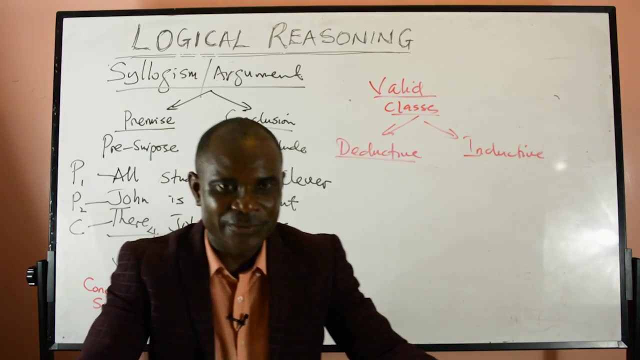 guarantee the truth nature of that conclusion, then that particular argument is called inductive argument, an inductive argument and that those inductive argument we normally commit those in our discussions, like if I see you just did an experiment on books, books that have hard covers are interesting, let's see. for instance, I 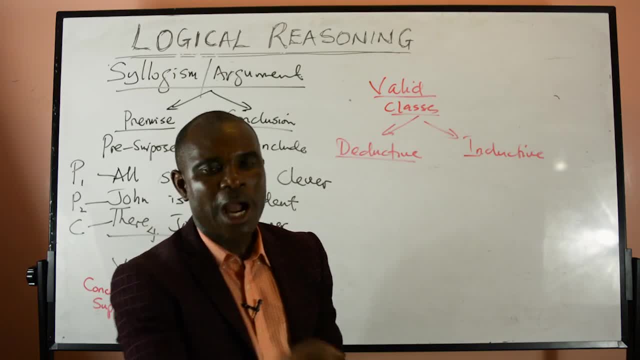 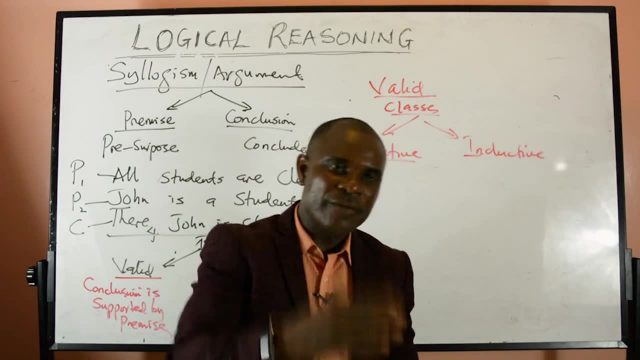 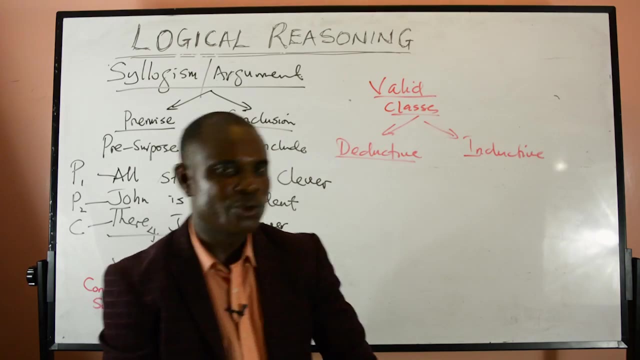 have no verse, no verse which had cover. I interesting, let's see- this guy brought up this conclusion by just reading a couple of movies that are having hard covers. but because the noves are having hard covers, and he read just a couple of their blessed 2025 and he was able to conclude: this is a kind of 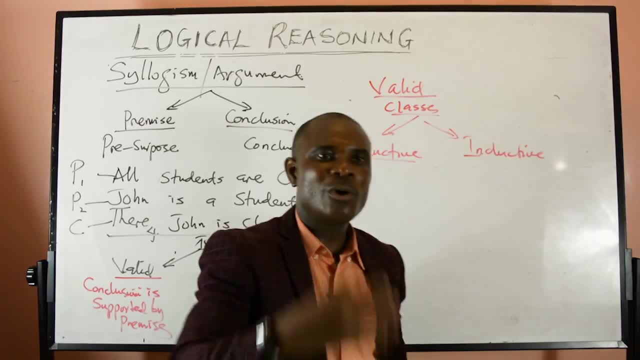 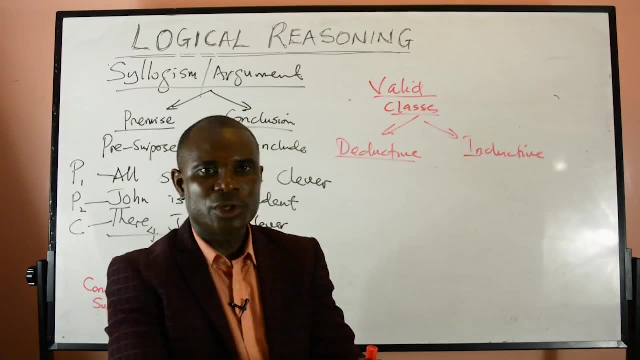 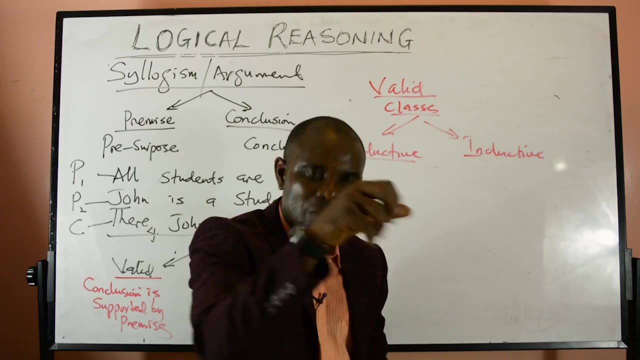 argument where you make generalization it is called HD January's, like the fallacy. when we make history generalization, just a few research or a few claims, there you know generalize it like you do a research on a couple of event and you know take that if that conclusion from those couple of events. 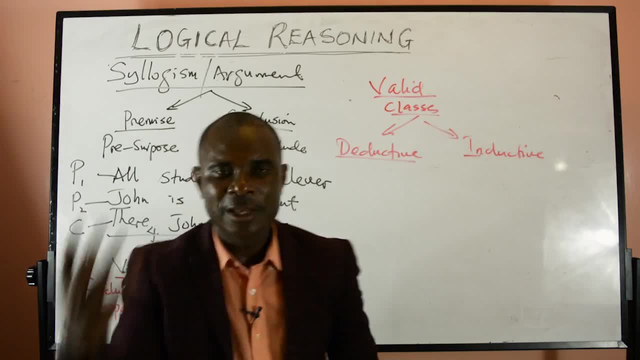 not even watch me, because at least we have a few reports that you do. you know, generalize it like you do a research on a couple of events and you not take that if that conclusion from those couple of events- not even much, maybe not inclusivity, 100 or more, then you now generalize and say that concept is generally now accepted. that is a true. 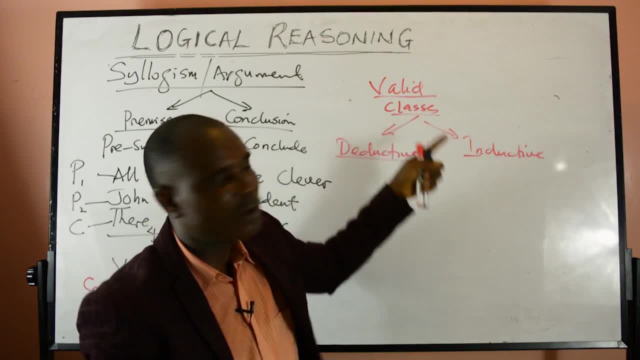 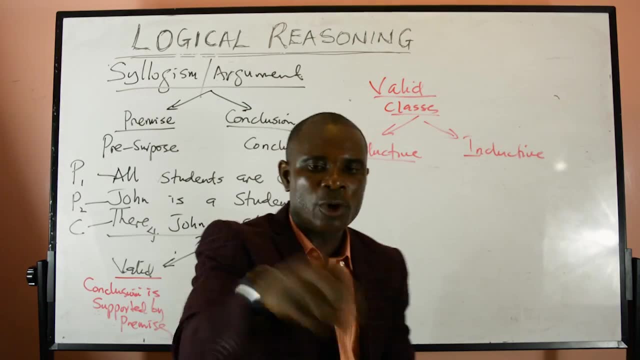 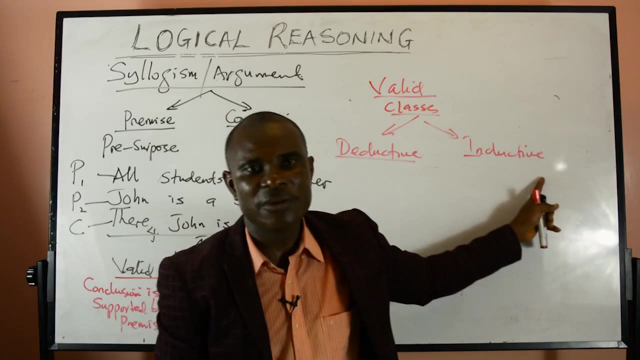 statement. so that kind of induction is that kind of validity, is what is called inductive conclusion. when you conclude on the basis of the fact that you just took a couple of investigations and you generalize that result on all other cases, then you are doing an inductive uh. 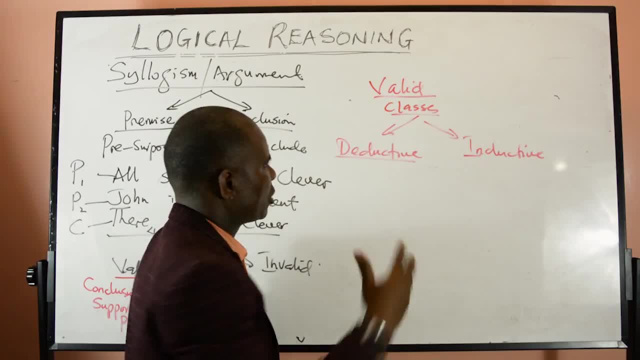 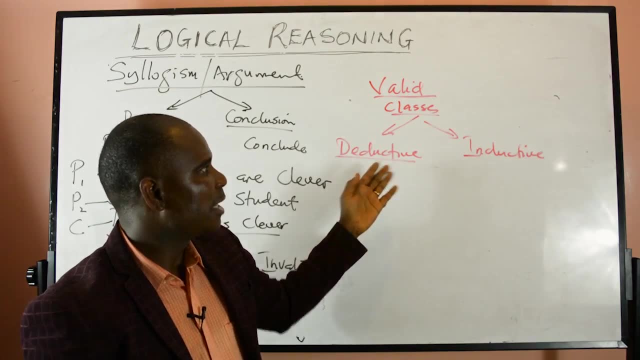 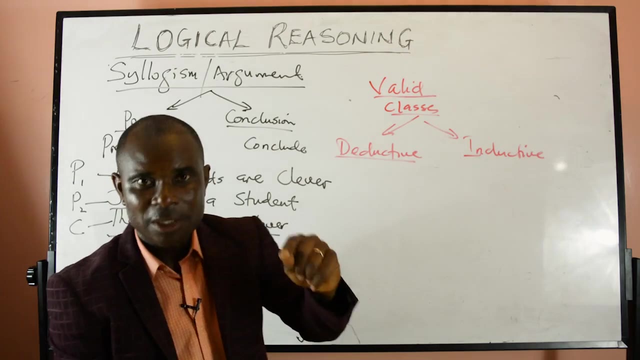 argument. So we want to distinguish between the two, as as I've already said. So what was that? in? in in deductive argument, we said that it is first of all going to be valid and the truth of the premises is absolutely going to determine. is absolutely going to determine. 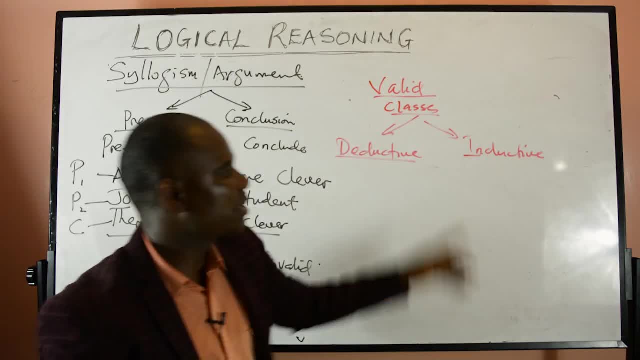 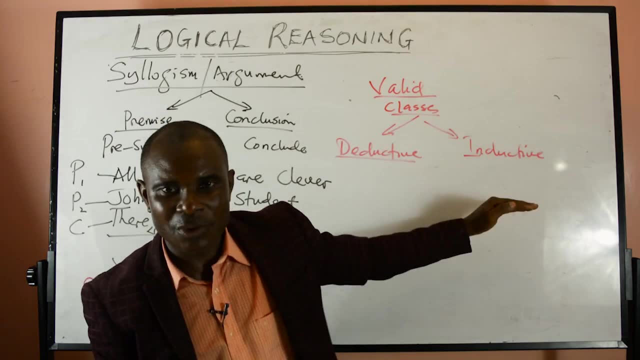 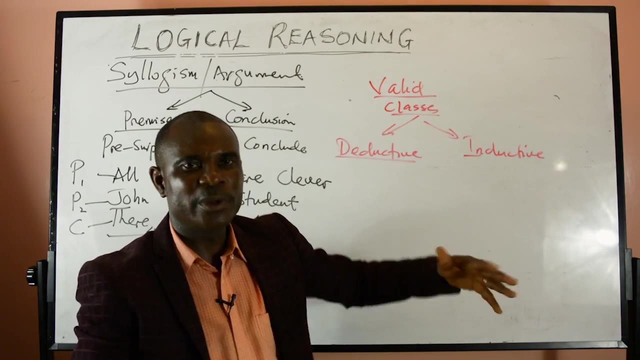 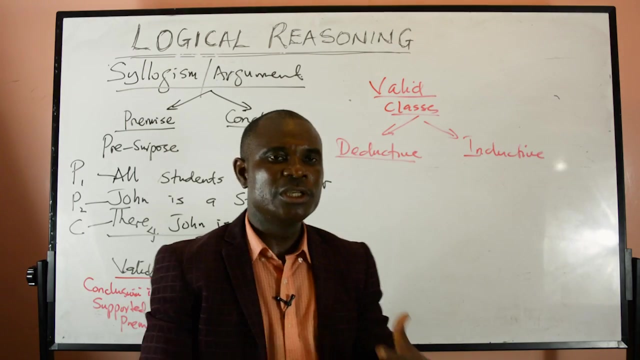 the truth nature of the conclusion. But if the truth of the premise do not absolutely guarantee the truth nature of that conclusion, then that That particular argument is an inductive argument And that those inductive argument we normally commit, those in our discussions, Like if I see you just did an experiment on books. 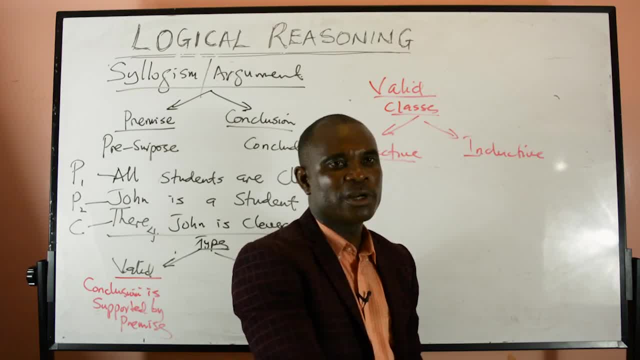 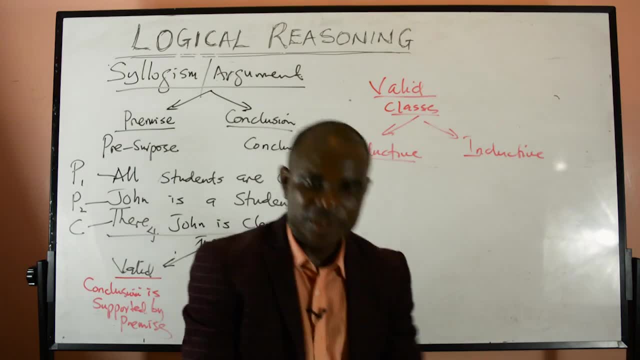 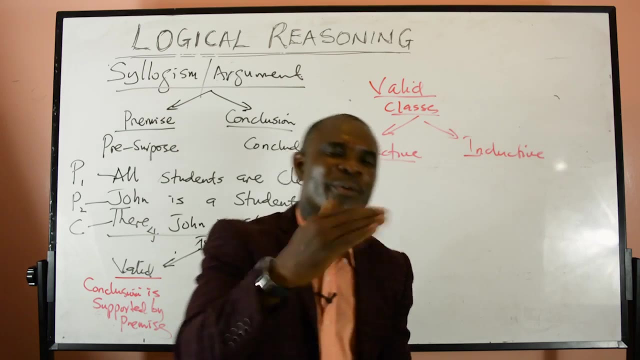 books that have hard covers are interesting. Let's say, for instance, I have novels. novels with hard cover are interesting. Let's say, this guy brought up this conclusion by just reading a couple of books, couple of novels that are having hard covers. but because 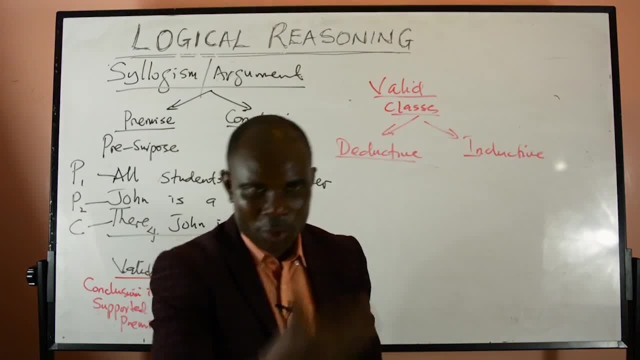 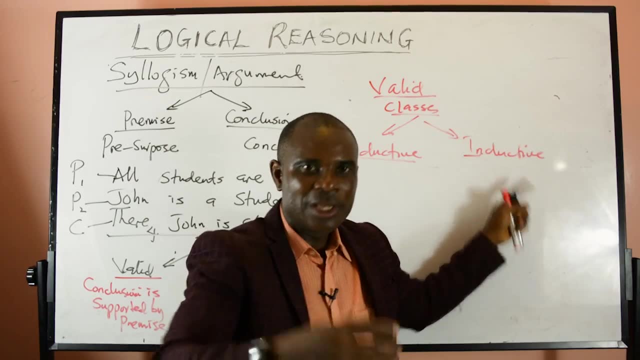 the novels are having hard covers, and he read just a couple of them, let's say 20-25, and he was able to conclude: this is a kind of argument where you make generalization, it is called a fallacy. when we make generalization just a. 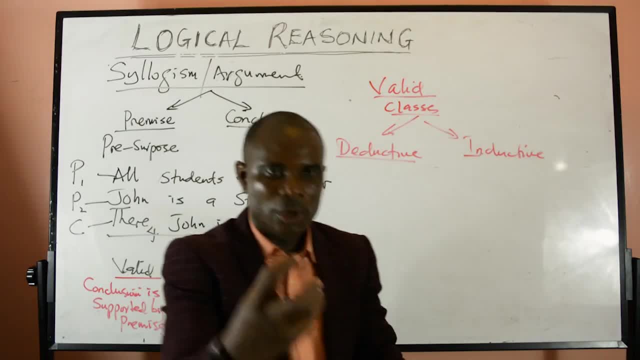 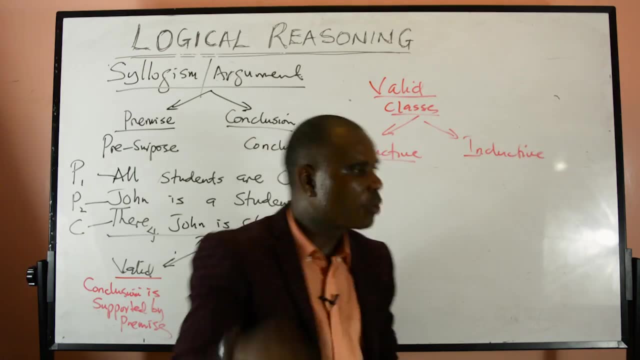 few research or a few claims, that you now generalize it like you do a research on a couple of events and you now take that if that conclusion from those couple of events not even much, maybe 100 or more- then you now generalize and say that concept is: 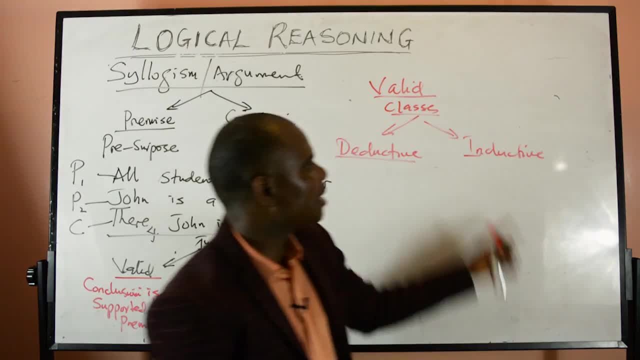 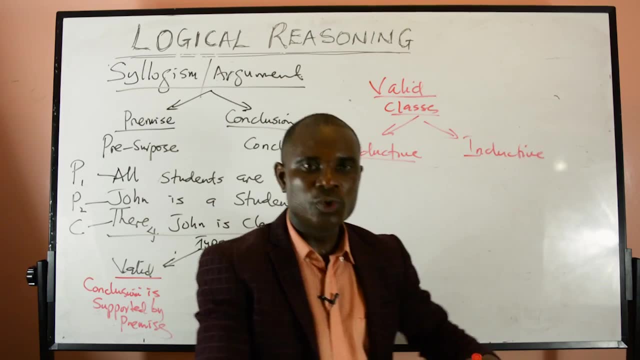 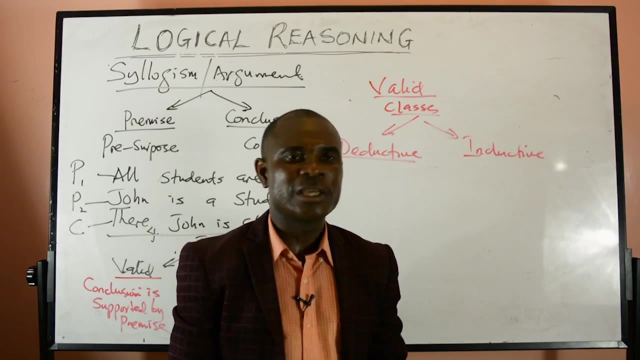 generally now accepted. that is a true statement. so that kind of induction is, that kind of validity, is what is called inductive conclusion, when you conclude on the basis of the fact that you just took a couple of investigations and you generalize that result on all other cases. 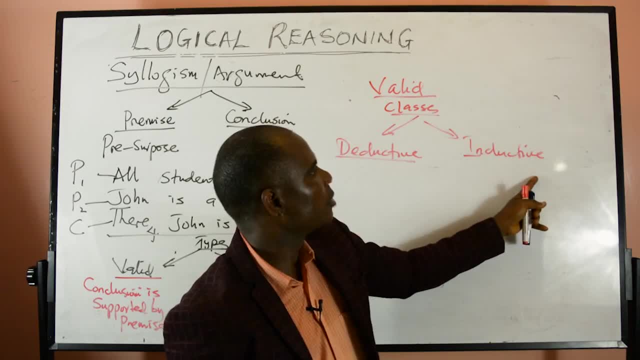 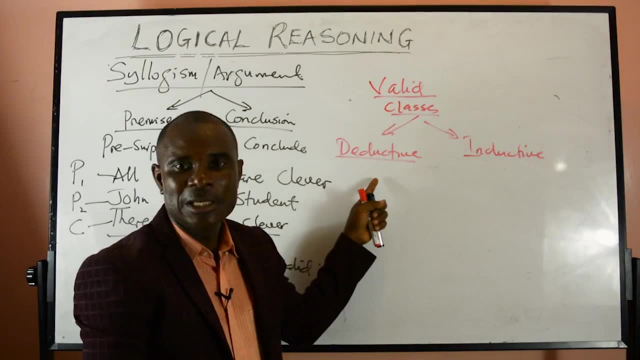 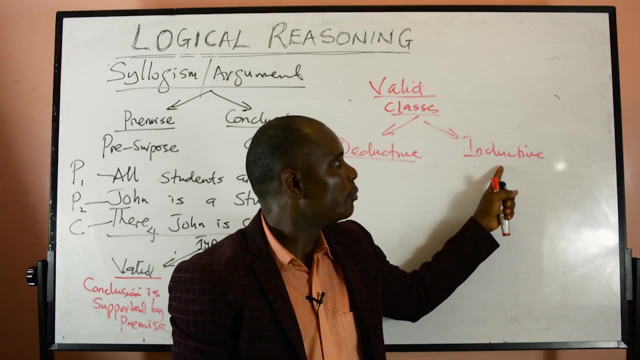 then you are doing an inductive argument, so we have seen the validity. but when, once, the validity is absolutely guaranteed by the absolute truth of the premise, then we talk about deductive argument, when the truth of the premise do not absolutely guarantee the validity of that conclusion. 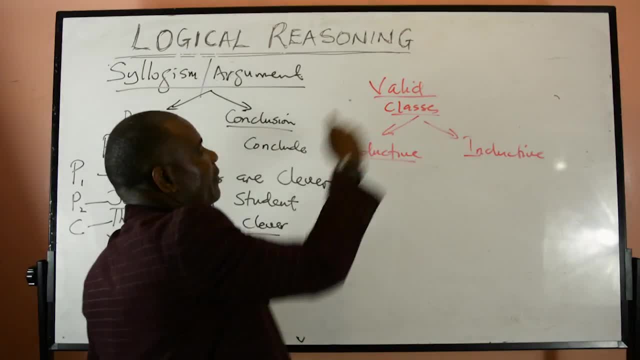 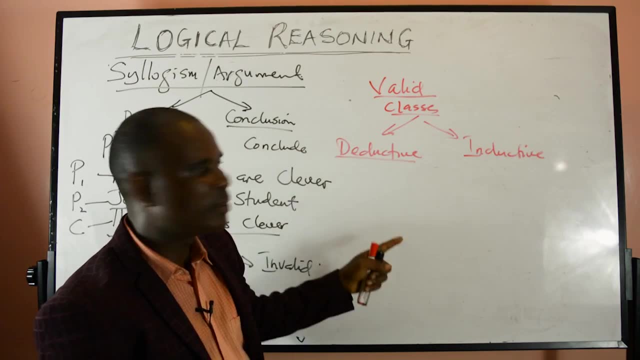 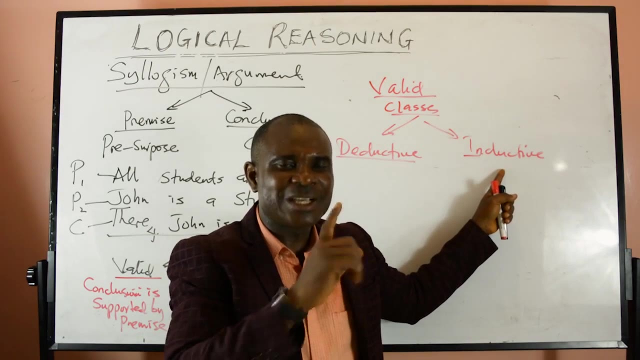 uh, inductive argument. so we have seen the validity. but when, once the validity is absolutely guaranteed by the absolute truth of the premise, then we talk about deductive arguments. when the the the truth of the premise do not absolutely guarantee the validity of that conclusion, then we were talking about an inductive argument. so now, 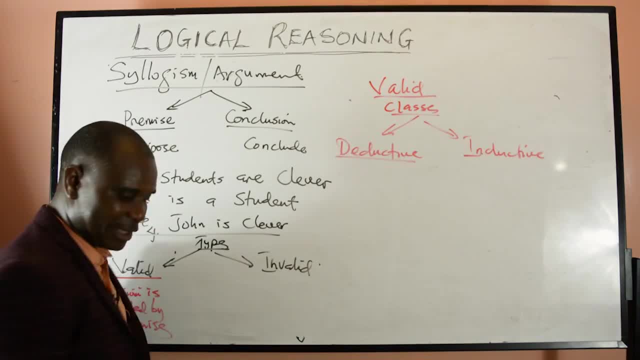 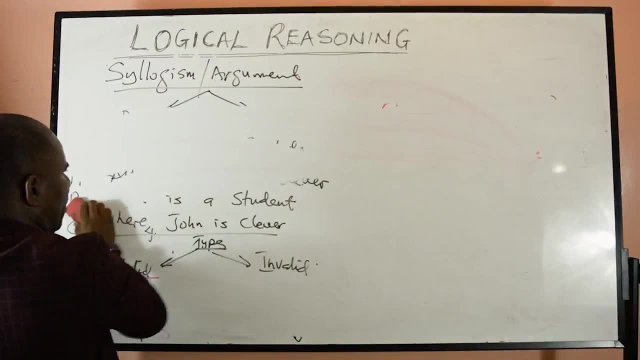 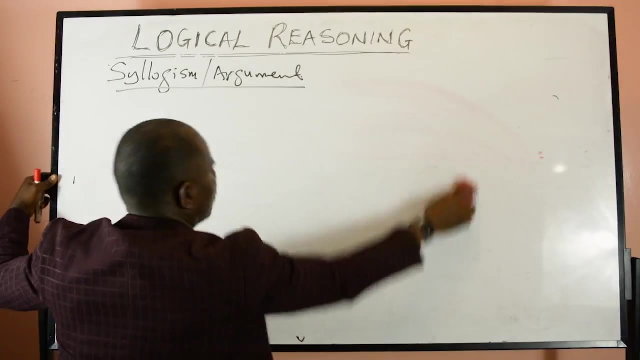 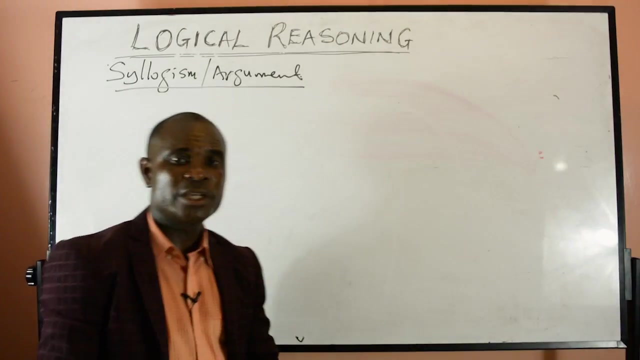 we have distinguished the two classes of validity. so our target is to really proceed with. so i come back here. let me clean here, then we'll look at the a simple example. so we want to look at. you are still under syllogism or argument. we now want to take an example. we now know what is a valid argument, what is an invalid argument. 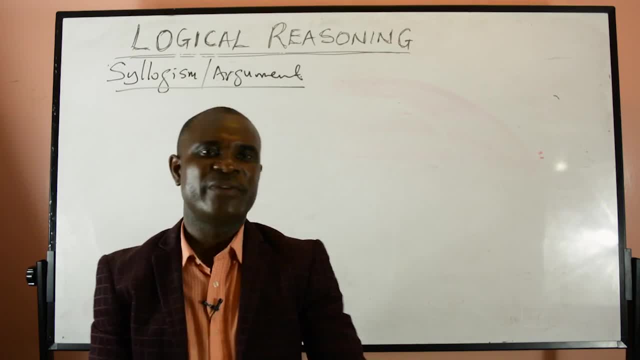 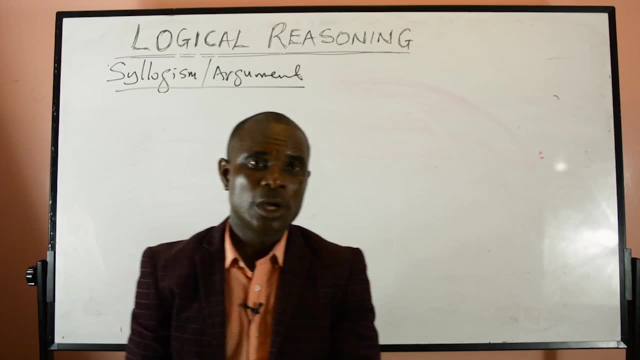 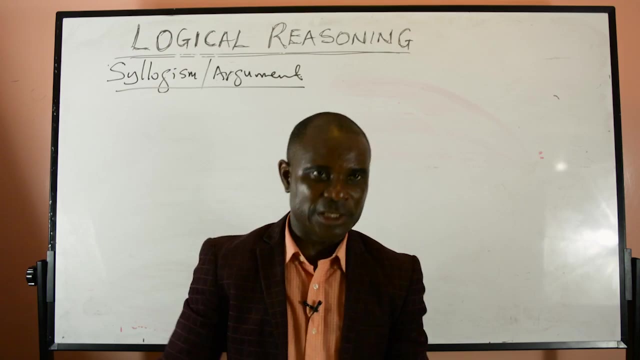 and we can also go by extension. the argument can be valid but sound as well. if the premises of that argument is all, they are all true and the argument is valid, then we can say that argument is also sound. so you can have a sound argument. that is it. first of all has to be valid when it all the 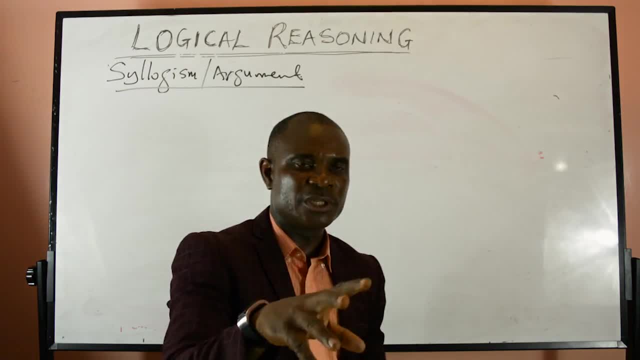 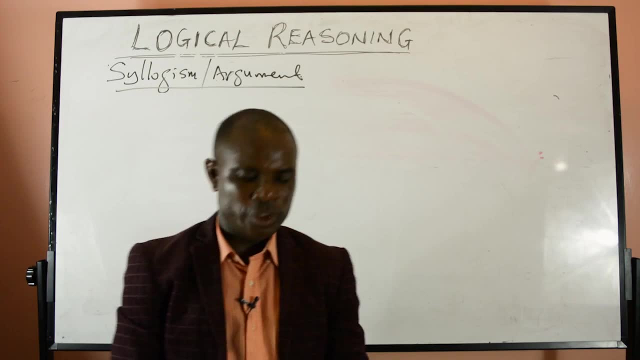 premises, all the the conclusion is supported by the premises, then we call it a valid argument. and if you look at the premises as well- and those premises are all true- then we can see it is a sound argument. so a sound argument has to be valid first of all. and when you are valid, 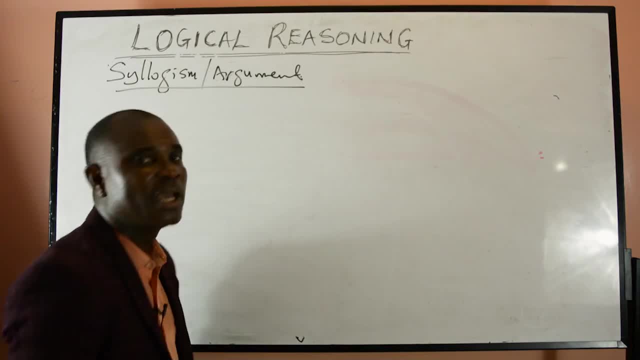 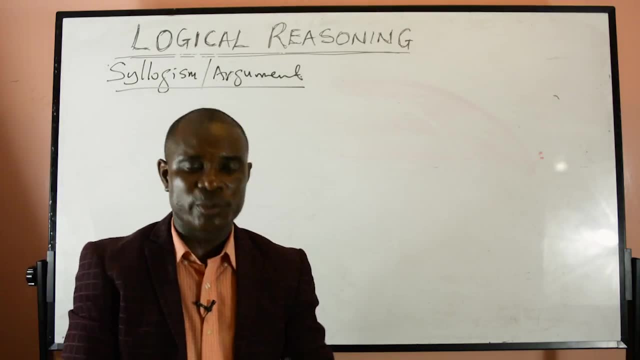 then all the premises become true. they will call it a sound argument. now let's come to the examples now. so i'll look at an example of the validity. so how do we find the validity of an argument? we can find the validity of an argument in two ways. first, we can find it not. 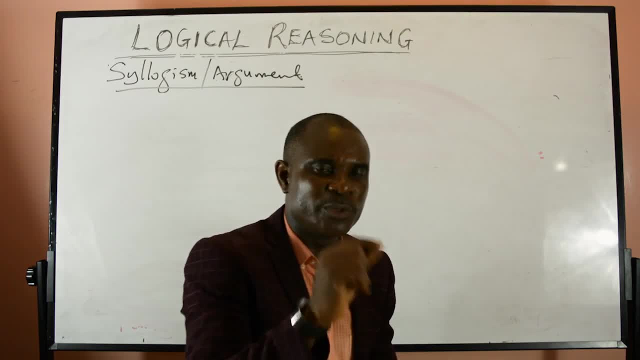 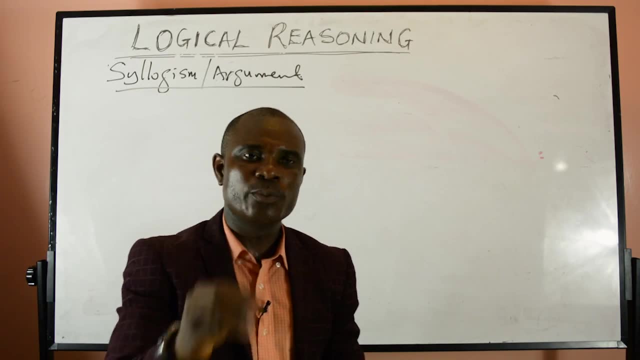 not even two ways. we have more ways, but for this course we just want to limit ourselves to two. now, the first way we can find the validity of an argument is when we include the solution based upon the venn diagram. so i'm going to use the venn diagram, so finding validity of an argument, finding. 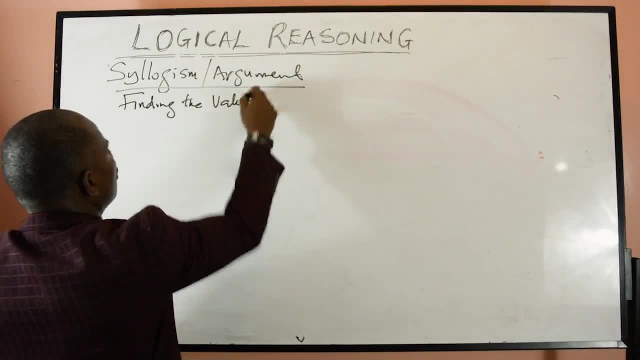 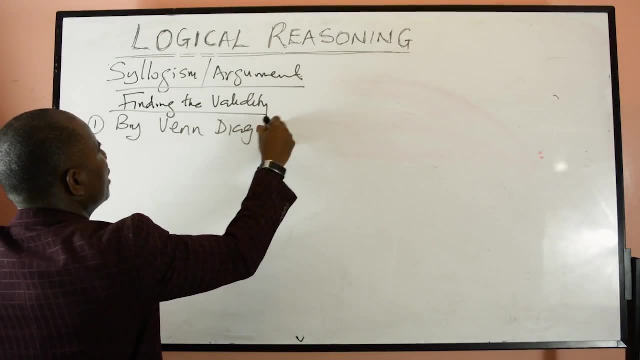 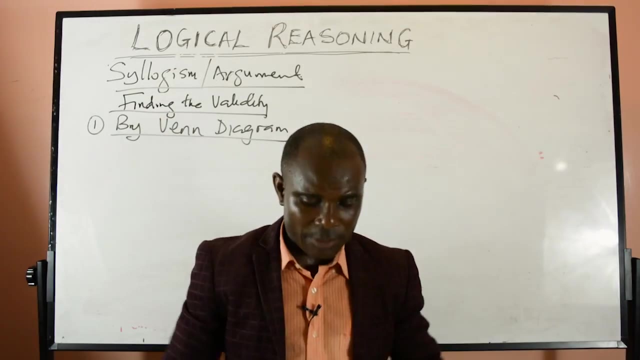 the validity of an argument, validity. so one way we can find the validity is by venn diagram, venn diagram. so how do we find the validity? by venn diagram? first you have to see, uh, what are. what is the venn diagram? it's a rectangular, it's a regular structure that has overs inside, and overs are those right side or 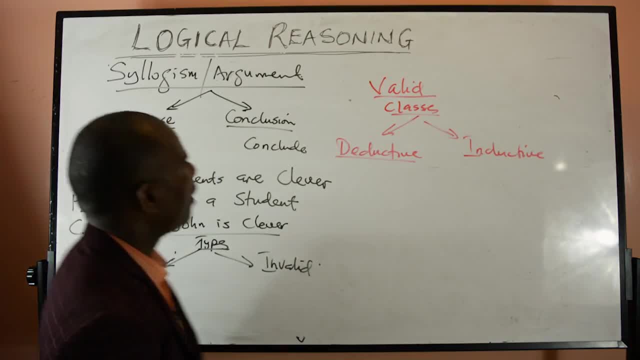 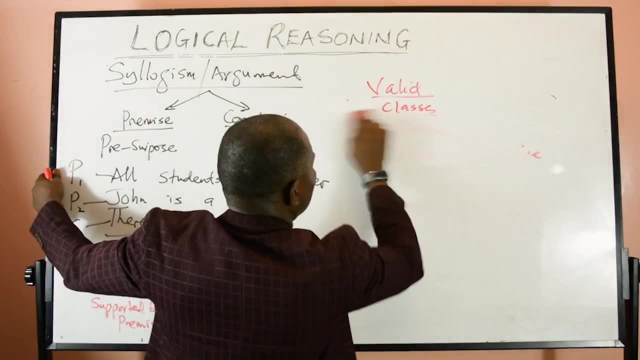 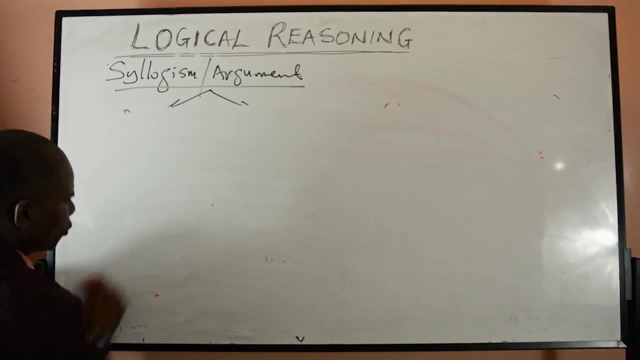 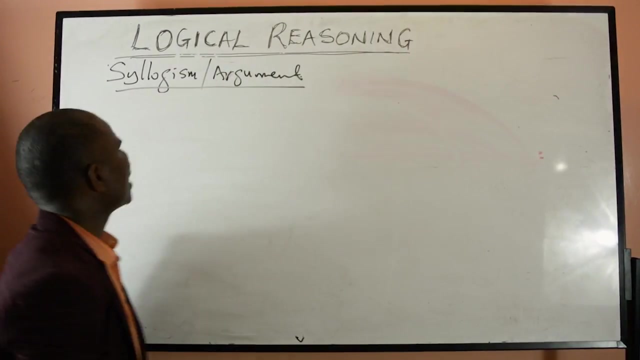 then we were talking about an inductive argument. so now we have distinguished the two classes of validity. so our target is to really proceed with so I come back here, so let me clean here. then we'll look at the simple example so we want to look at. 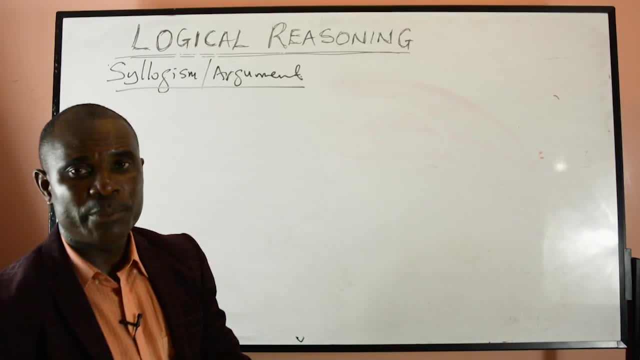 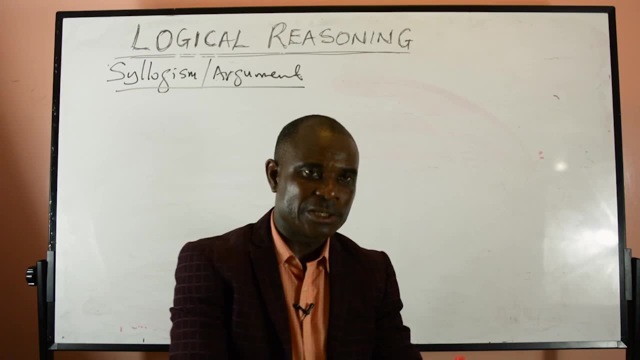 we're still under syllogism or argument. we now want to take an example. we now know what is a valid argument, what is an invalid argument, and we can also go by extension. the argument can be valid but sound as well, if the premises of that 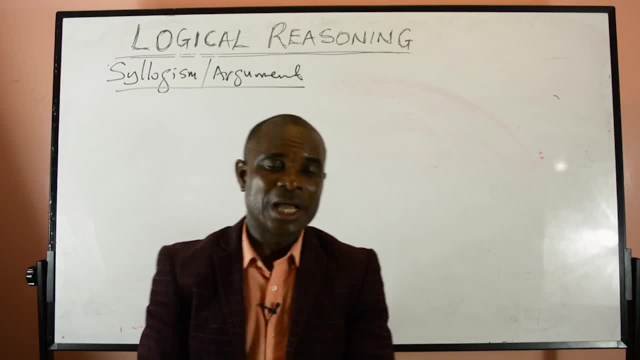 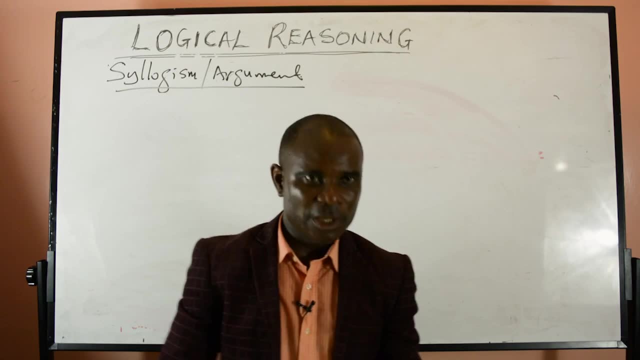 argument is all, they are all true and the argument is valid, then we can say that argument is also sound. so you can have a sound argument, that is, it first of all has to be valid when all the premises, all the, the conclusion is supported by the premises. 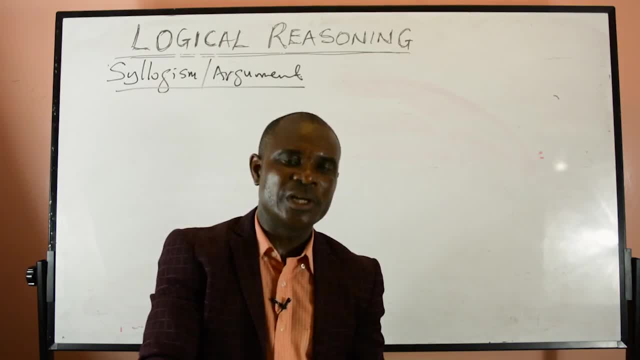 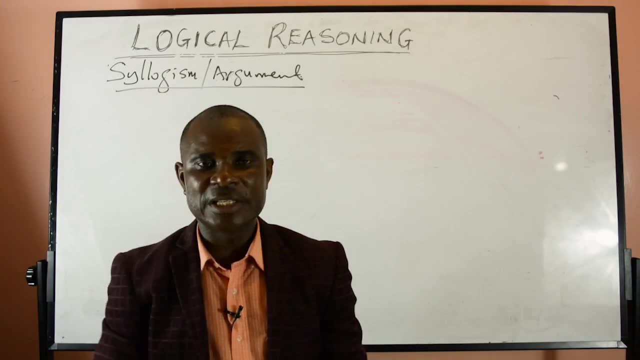 then we call it a valid argument. and if you look at the premises as well, and those premises are all true, then we can say it is a sound argument. so a sound argument has to be valid first of all, and when you are valid, then all the premises. 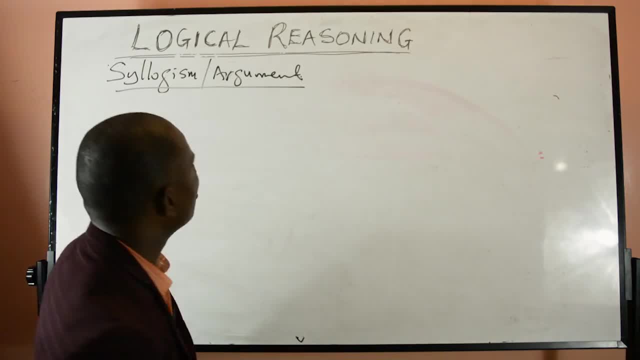 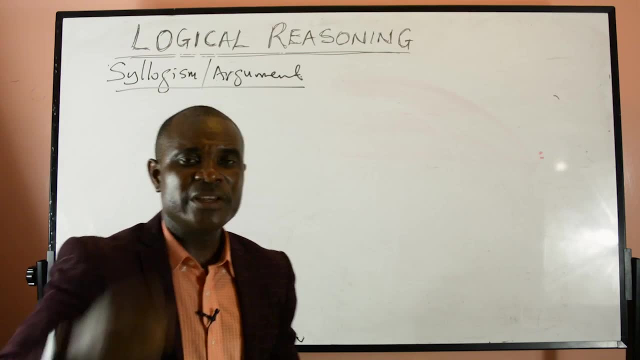 become true, they will call it a sound argument. now let's come to the examples now. so i'll look at an example of the validity. so how do we find the validity of an argument? we can find the validity of an argument in two ways. first, we can find it not, not even two ways, we have more ways. but for this course, 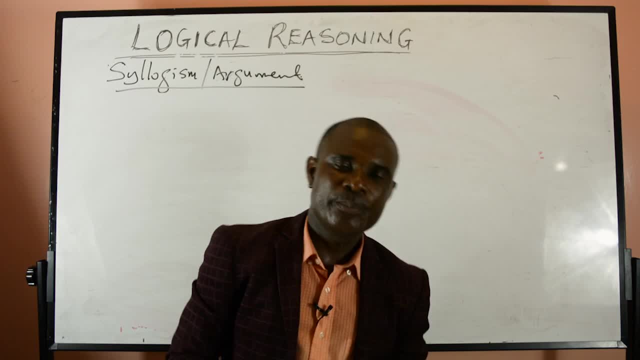 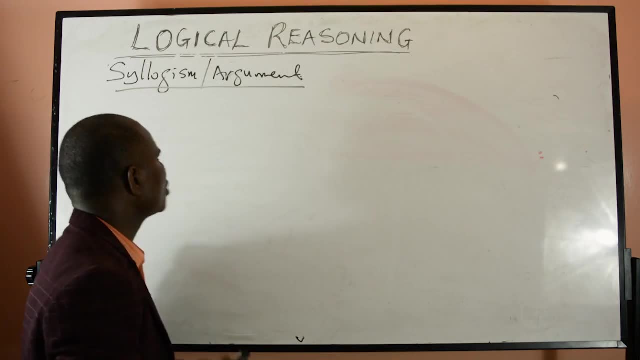 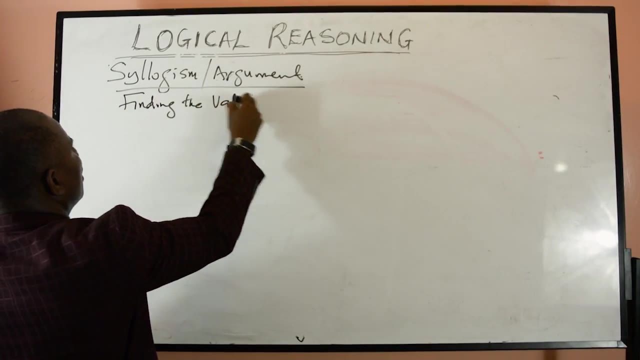 we just want to limit ourselves to two now. the first way we can find the validity of an argument is when we include the solution based upon the venn diagram. so i'm going to use the venn diagram. so finding validity of an argument, finding the validity of an argument, validity. so one way we 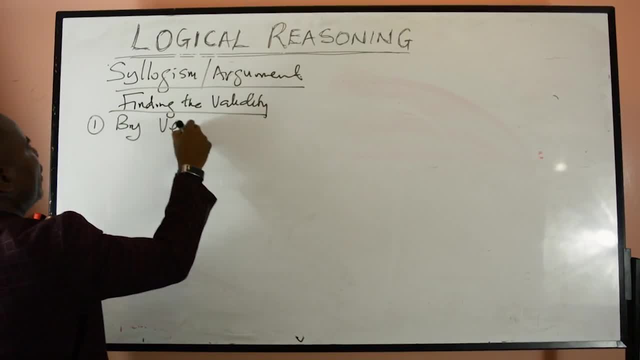 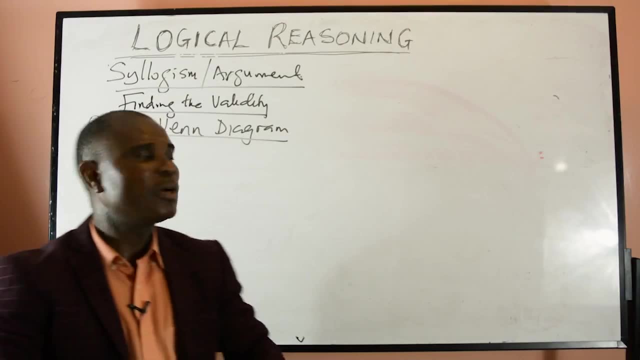 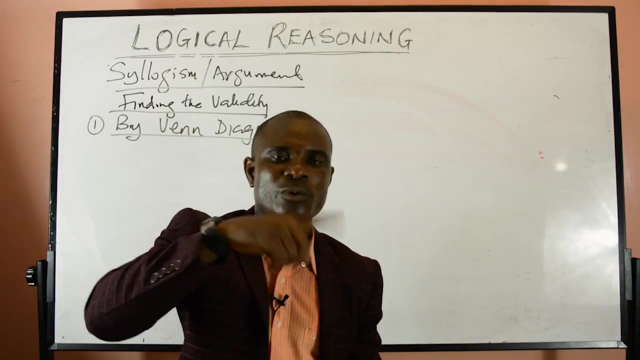 can find the validity is by venn diagram, venn diagram. so how do we find the validity by venn diagram? first you have to see: uh, what are. what is the venn diagram? it's a rectangular. it's a rectangular structure that has overs inside, and overs are those right side or round circles, those 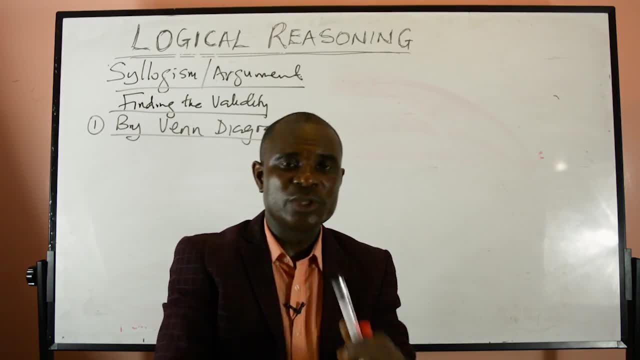 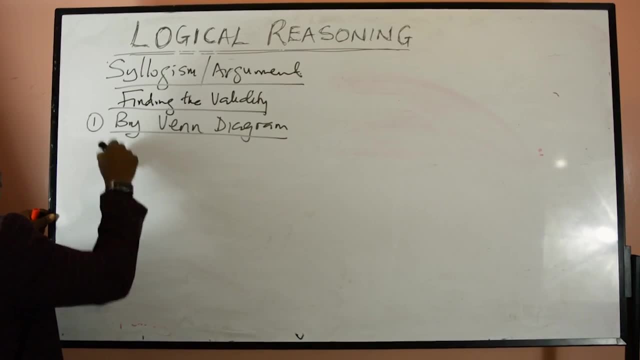 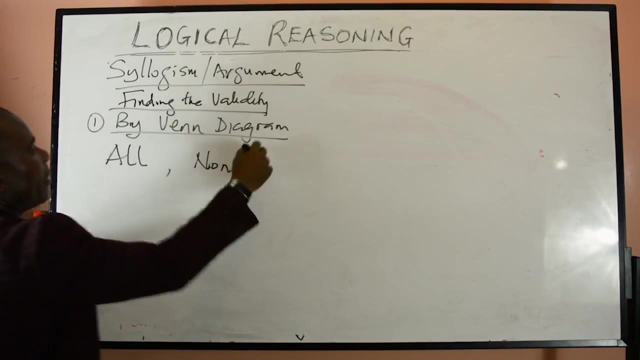 overs are showing you the relationship between the, the, the, the statements you are coming to as such. so now those statements can be: first, i can say: i can define words like all. i can also define as none i can. none is the same as no. i can have all. 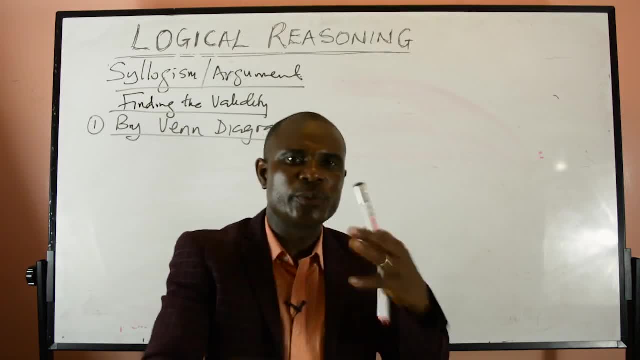 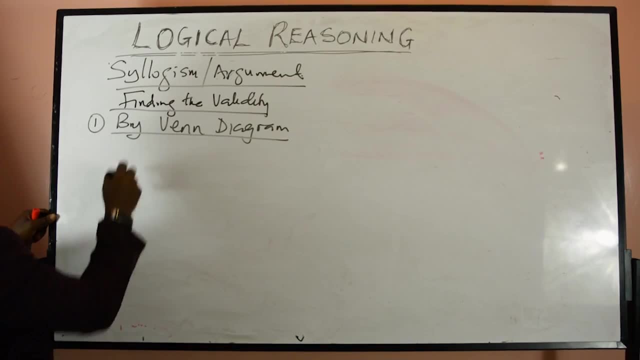 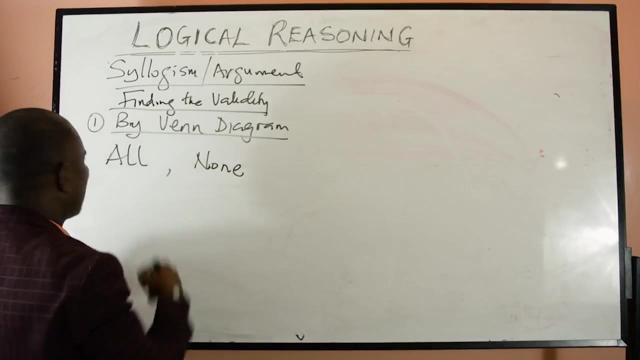 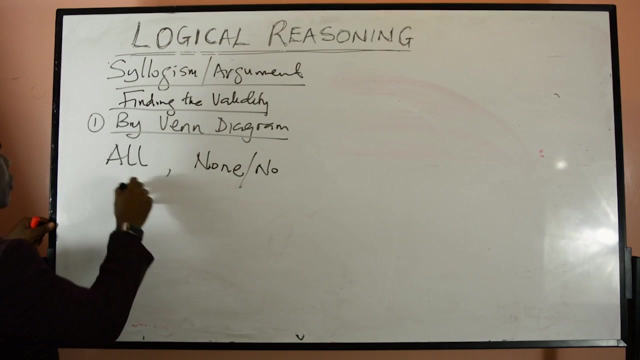 round circles. those overs are showing you the relationship between the, the statements you are coming to as such. so now those statements can be. first i can say i can define words like all i can also define as none i can. none is the same as no. i have all i can have. no i can. i can also have some. so i'll define some, most if you many. 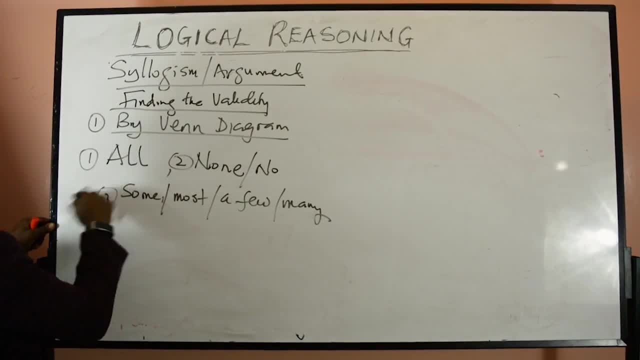 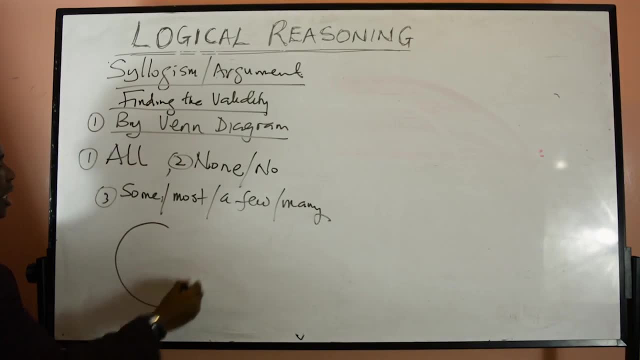 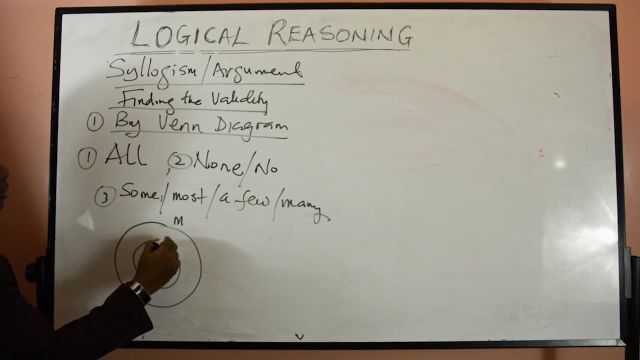 so these three terminologies must be able to understand that properly. when i say, when i use all in the venn diagram, if i say, for instance, all math teachers are tall, all math teachers are tall, this is, all math teachers are tall. so now we have tall and you have math teachers, all the math teachers are tall. 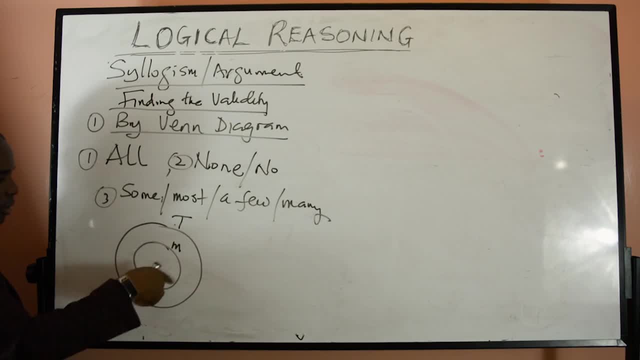 so i've used all. it means that all the math teachers are inside the top circle. in other words, all the variables inside the math over, the math over is going to be swallowed by the tall circle circle. so that is the meaning of all. all math teachers are tall: m for math and t for tall. that 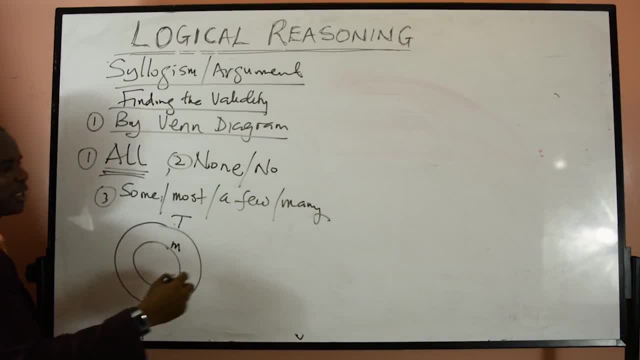 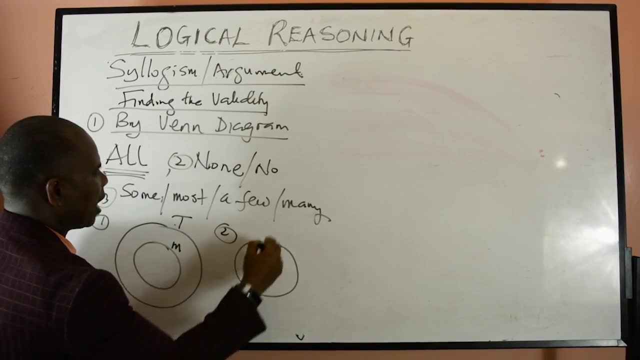 is an example of using the word all. what about the second one? the second one is: no math teacher is tall. this is number one. number two: no math teacher is tall. so i have tall here, then i have math there. no math teacher is tall. it means there is no intersection, there's no way. these two 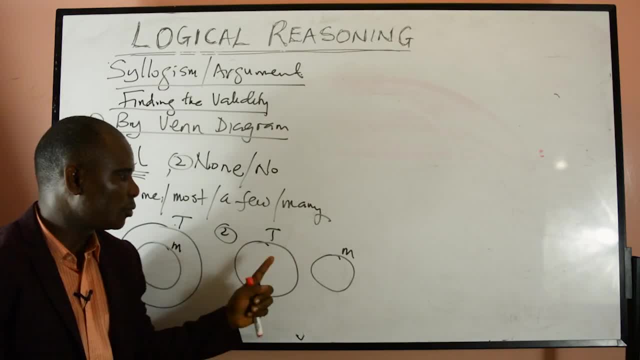 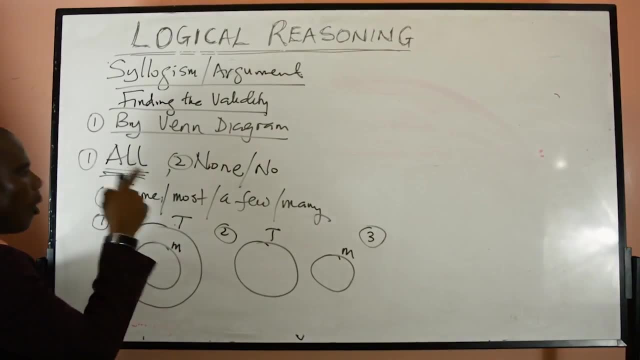 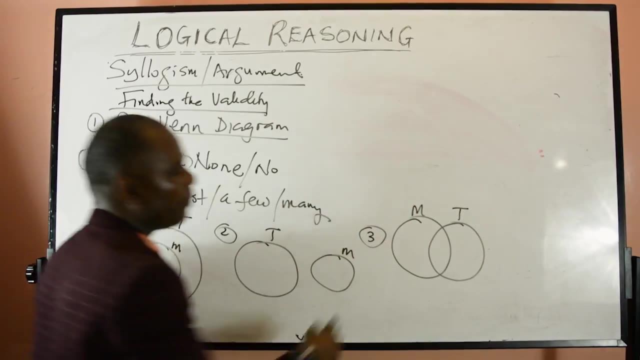 circles can meet. this is there's no connection between the two. no, math teacher is tall. now we'll have the thought. the third part of it- when i see some or most math teachers at all, so i can say most math teachers at all, so i have math teachers at all, some math teachers at all, means that there 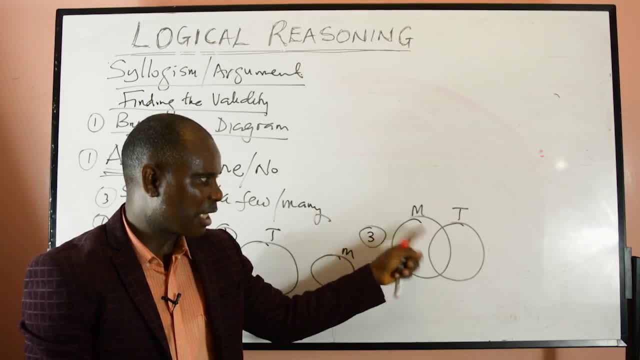 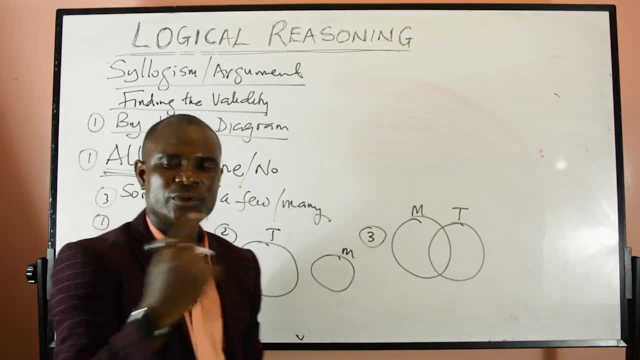 is an intersection, then more: some math teachers at all, most math teachers at all, many math teachers at all. all of them give you the intersection. so there are three words you have to understand before we actually look at these questions as we go. first, you must know what is all, all means. 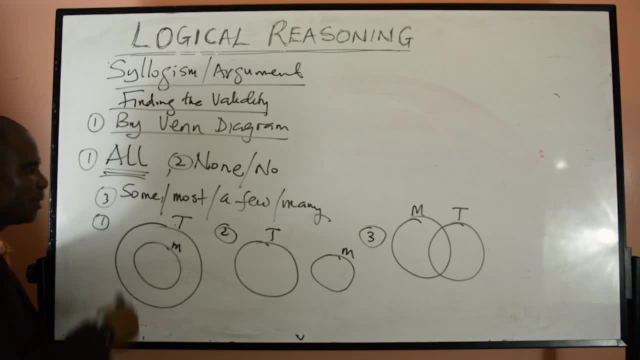 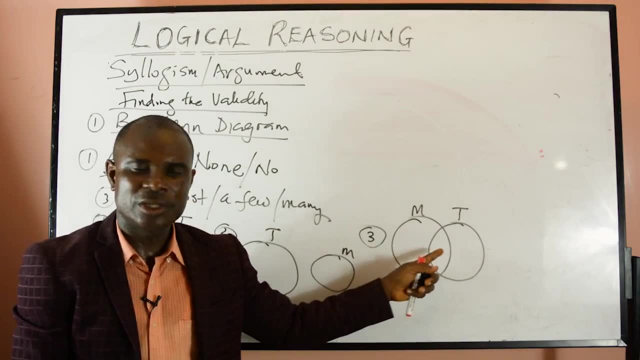 all, all the circle are embedded in that particular circle. so we now look at this one. they don't have any connection. this is what we call it century as this joint set. now we have what is called intercession here some the word, some, most a few, many, all of them are inside the intersection. now. 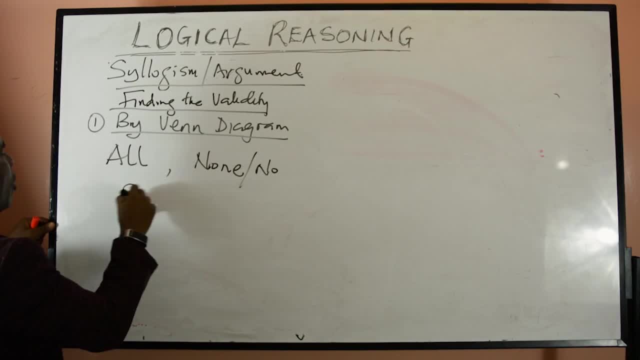 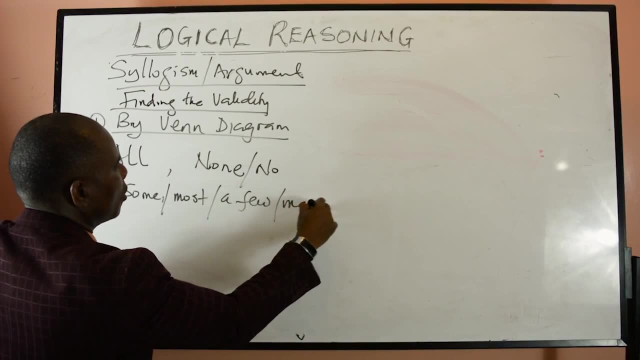 i can have. no, i can, i can also have some, so i'll define some most a few many. so these three, some most a few many. so these three terminologies must be able to understand. terminologies must be able to understand. terminologies must be able to understand that properly, when i say, when i use all, 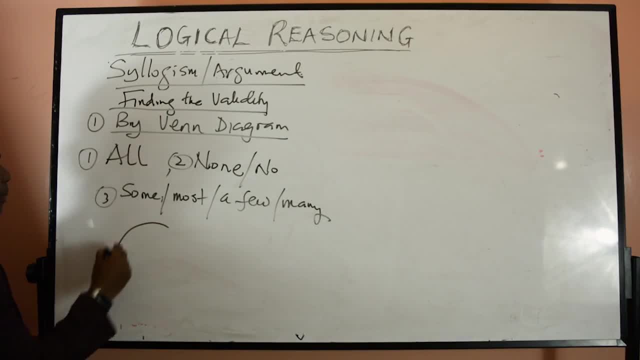 that properly when i say when i use all that properly, when i say when i use all in the venn diagram, if i say, for instance, in the venn diagram, if i say, for instance, in the venn diagram, if i say, for instance, all my teachers are tall, all my teachers. 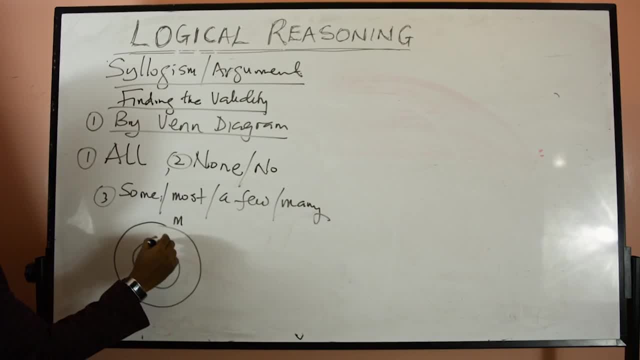 all my teachers are tall. all my teachers, all my teachers are tall. all my teachers are tall. this is all my teachers are tall, are tall. this is all my teachers are tall, are tall. this is all my teachers are tall. so now we have tall and you have mass. 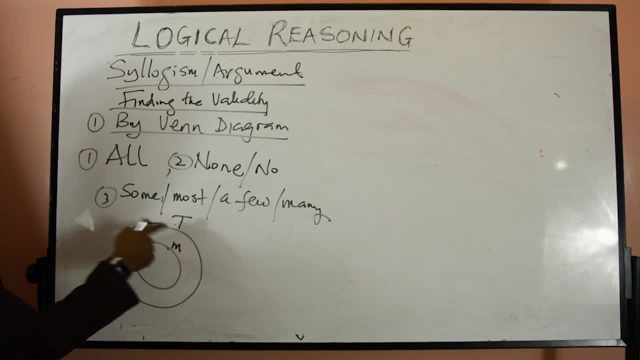 so now we have tall and you have mass. so now we have tall and you have mass teachers. all the mass teachers are tall teachers. all the mass teachers are tall. so i've used all it means that all the mass teachers are inside the tall circle. in other, 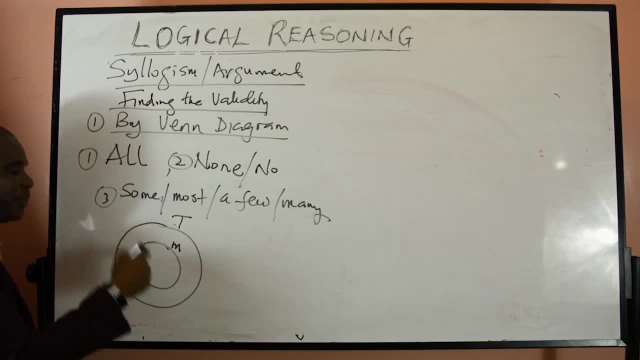 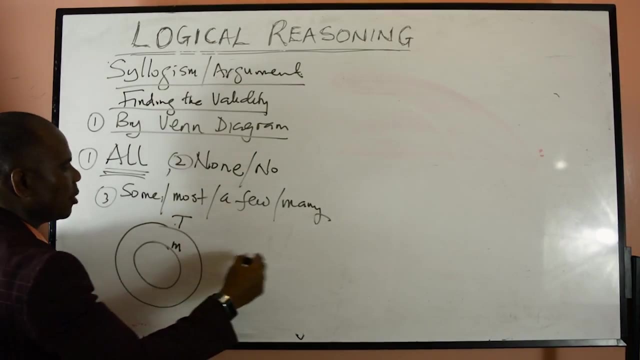 words all the variables inside the math over. the math over is going to be swallowed by the tall circle. so that is the meaning of all. all mass teachers are tall: m for math and t for tall. that is an example of using the word all. what about the second one? the second one is: 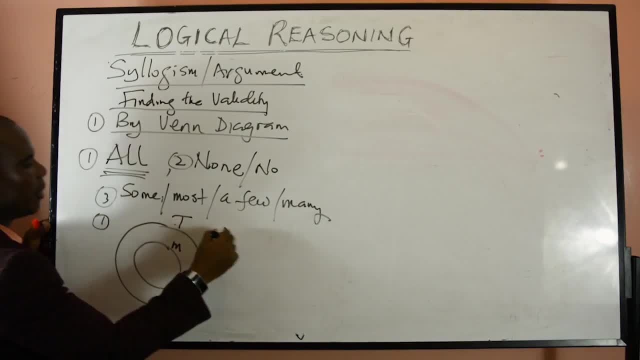 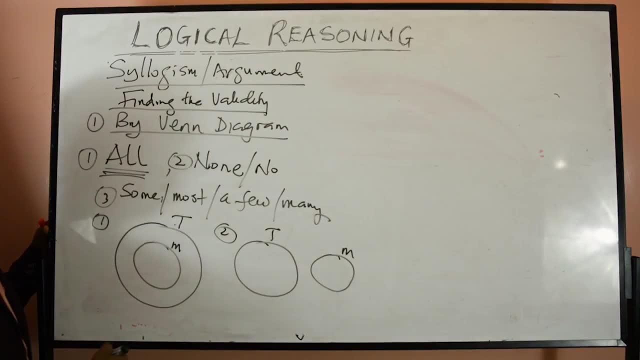 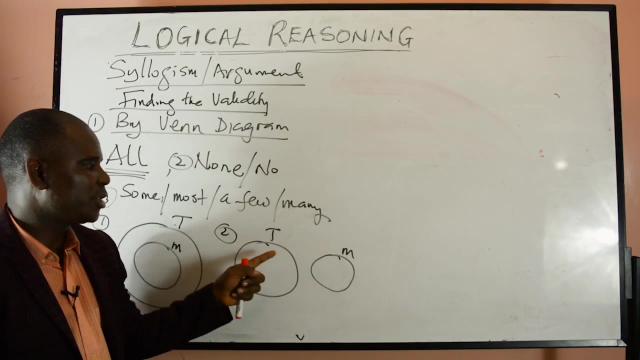 no master has told this is number one, number two: no master is thought. so i have thought here, then i have mass here. no master is thought. it means there is no intersection. there's no way the two circles commit. this is there's no connection between the two. no birth teacher. 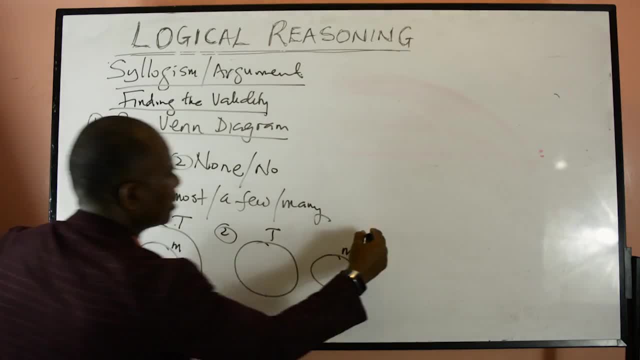 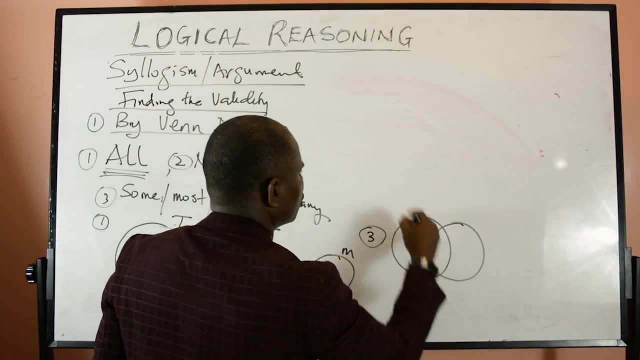 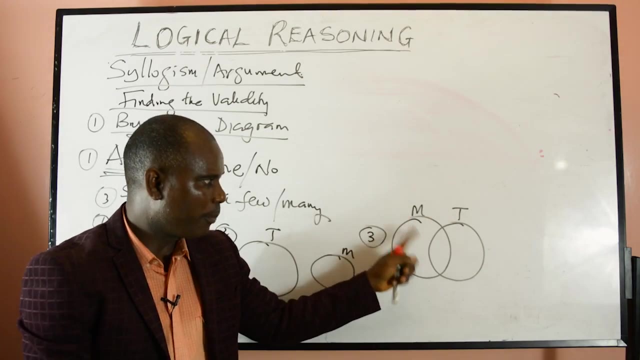 is tall. now we have the thought, the third part of it, when i say some of most mass teachers are tall- most mass teachers, after all. so i have my situation. Some mass teachers are tall means that there is an intersection. Then some mass teachers are tall. 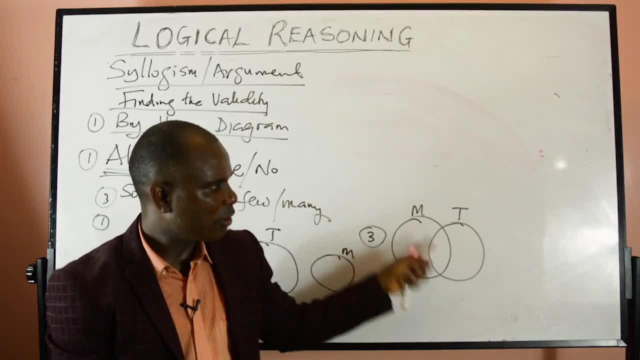 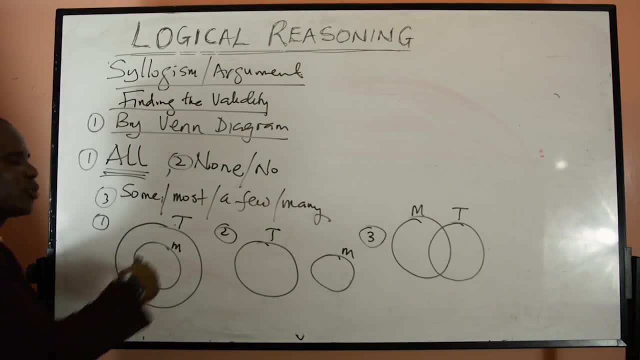 Most mass teachers are tall. Many mass teachers are tall. All of them give you the intersection. So there are three words you have to understand before we actually look at these questions as we go. First, you must know what is all. All means all. 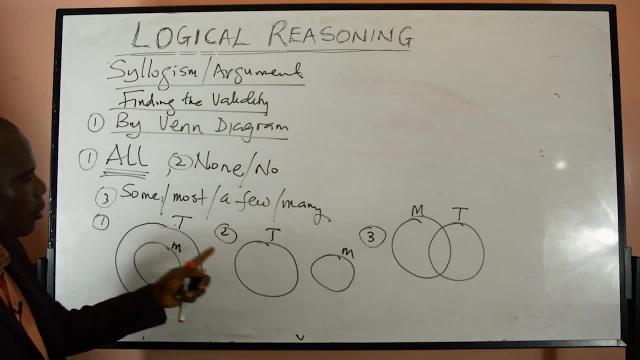 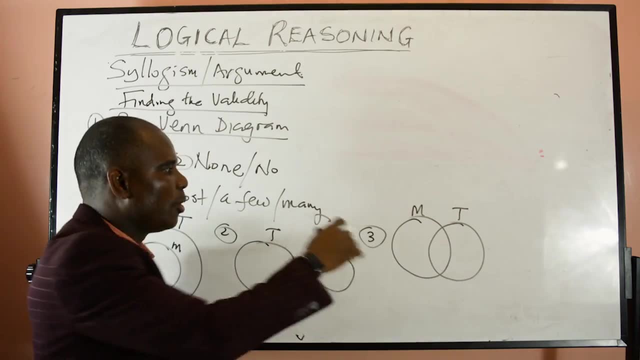 All the circles are embedded in that particular circle. So we now look at this one. They don't have any connection. This is what we call in set theory as disjoint set. Now we have what is called intersection. here. Some the word, some, most a few, many, all of them are inside the intersection. 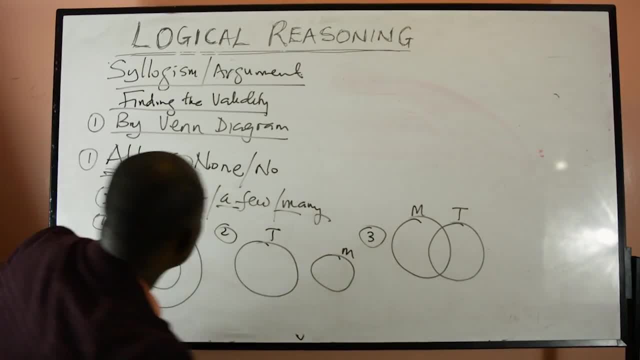 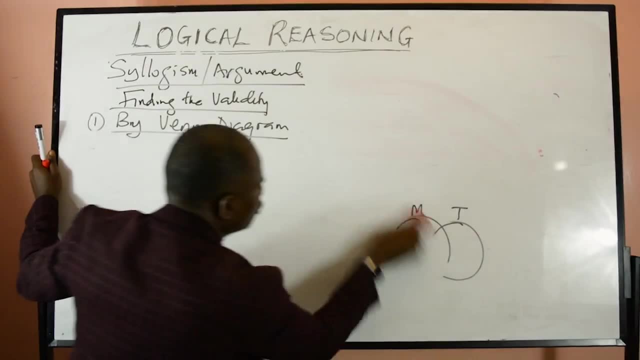 i now know the meaning of those overs as i move. now let me go to the questions proper. now we have to find the validity of the statements based upon its venn diagram. so we use the venn diagram to determine the validity. so let's say, for instance, i'll develop an 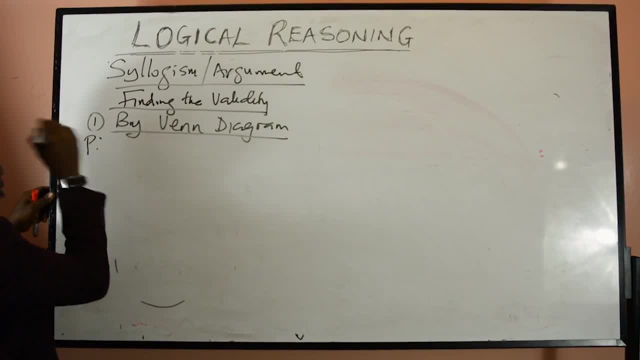 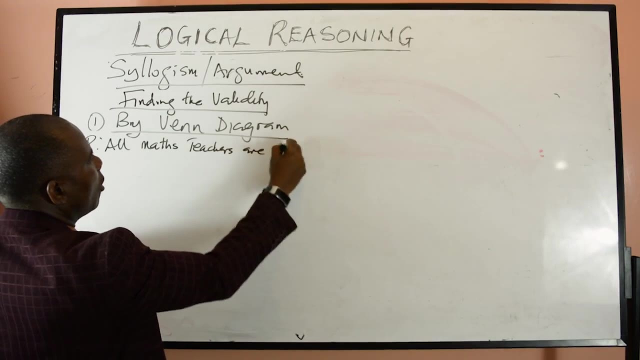 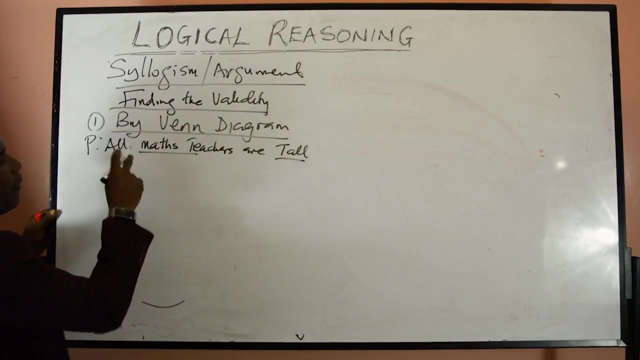 argument here. so let's say p, since it is symbolic. we want to represent the statement, not based upon the letter. so we say: all mass teachers, all math, all mars teachers are tall. so here so let's say math, m for math and t for tall, m for mass teachers and t for tall. and 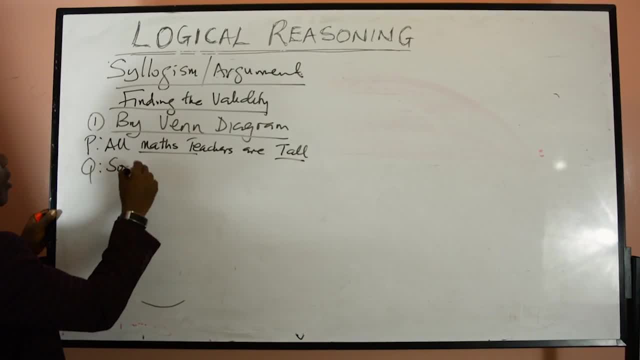 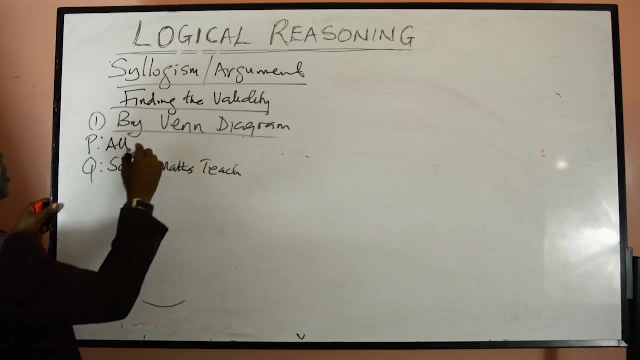 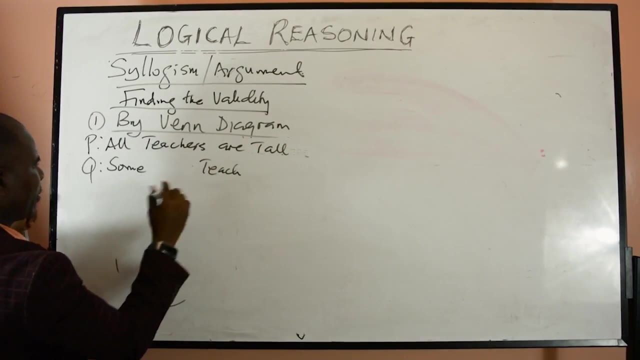 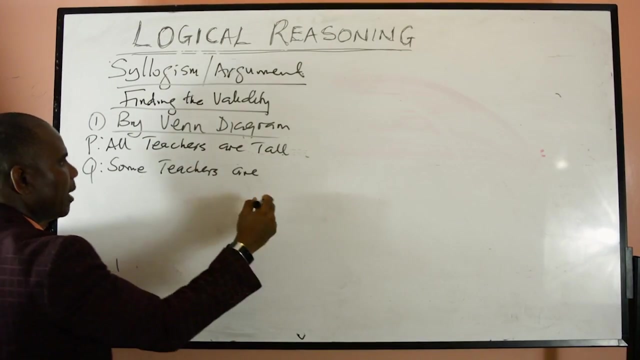 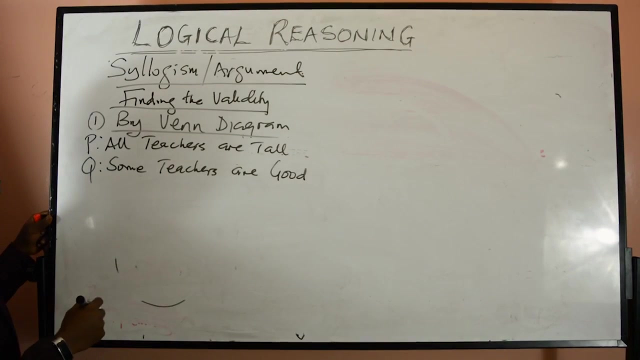 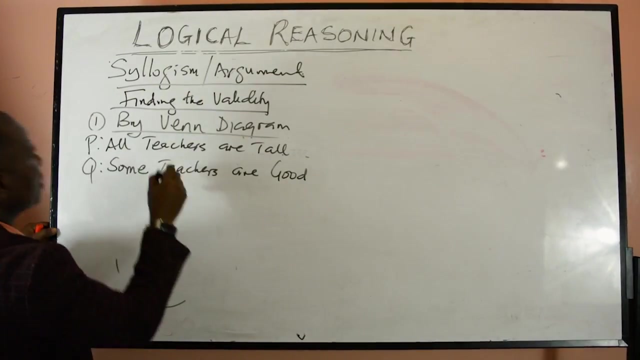 q. we can say some some maths teachers, let's say all teachers at all. so i can shorten this: some teachers are good, some teachers are good, so now we have some. so we can look at the first premise. it has two characters in there. we have teachers and tall. 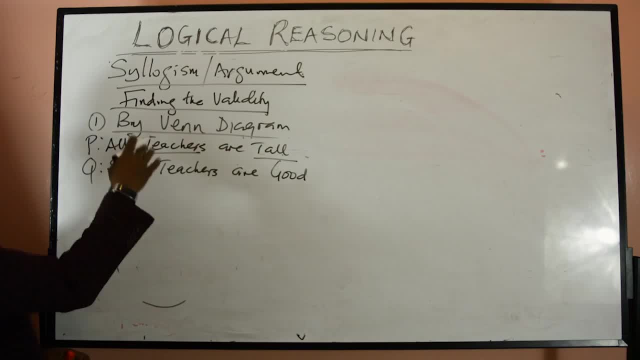 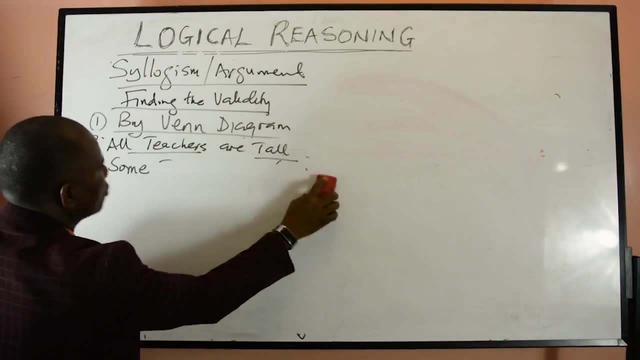 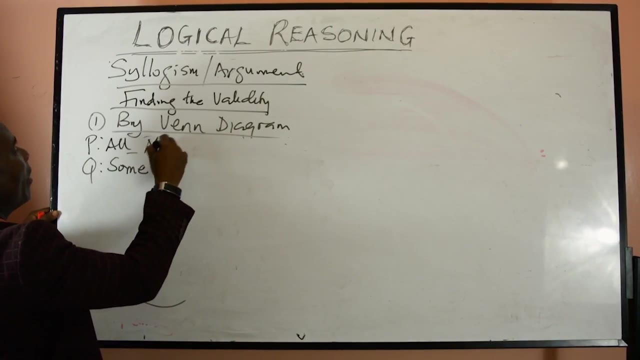 oh, okay, i, i, i better change this tall so that we don't mix the two t's together, so let me still use the the, the mass teachers there it can help us with that. so now we have, because i'm trying to simplify so that we have different letters. so, okay, let me use men. all men are tall. 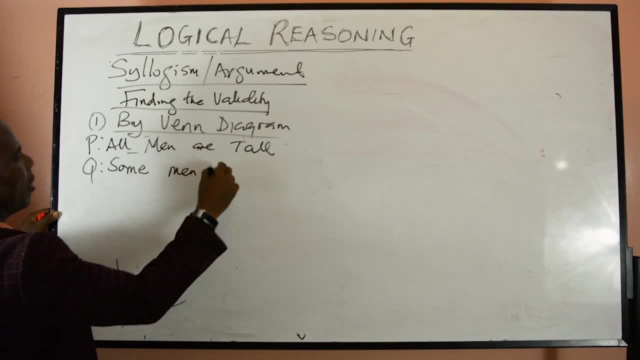 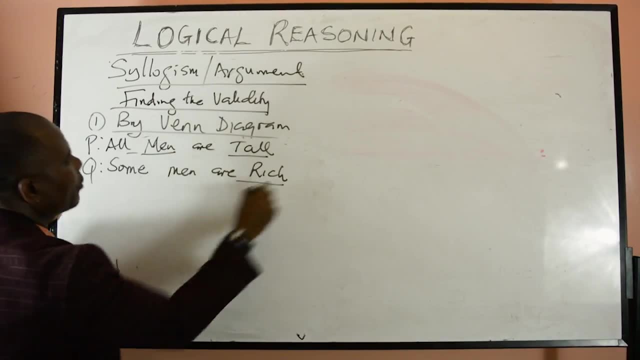 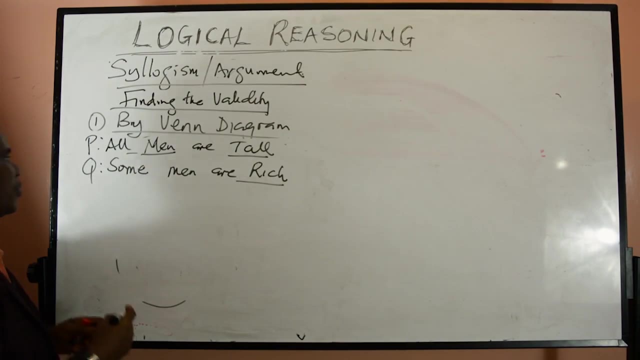 some men are rich, so let me use that so tall and unreached. so we have that now. i just change the sentence because i want to have different letters so i don't keep confusing you. so look at it. this is: they say: represent this. i want to represent this information on on event diagram. so let's say the. 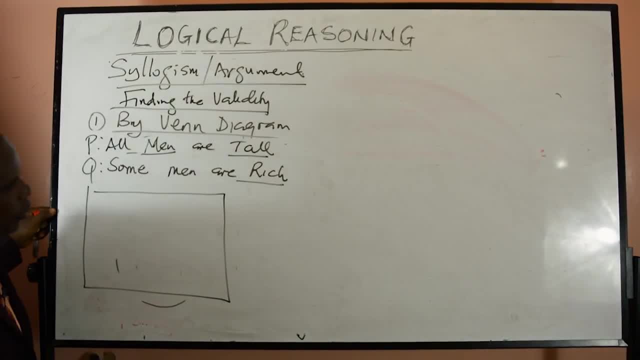 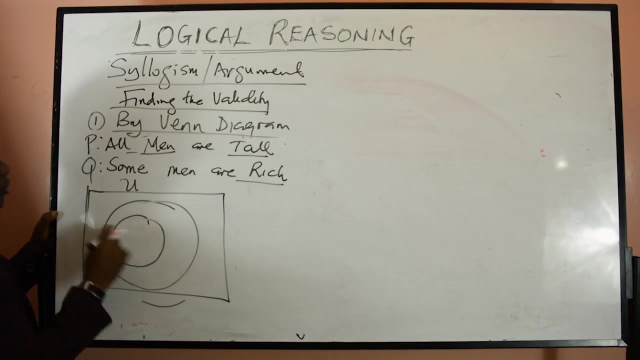 venn diagram. so we have venn diagram represented by this venn diagram. so we have the venn diagram represents men, but this all men, as the universal set says. yes, now, we now have all men at all. so we can have the two circles together and you can help me out with this- you also move together. so 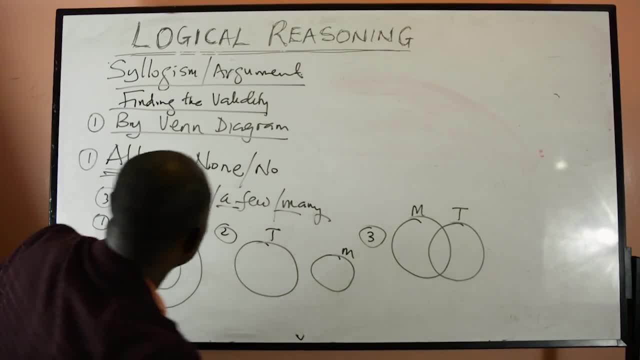 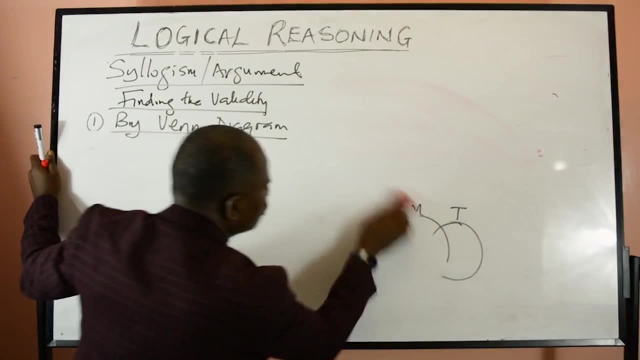 Now, you now know the meaning of those overs as I move. Now let me go to the questions proper. Now we have to find the validity of the statement based upon its Venn diagram. So we use the Venn diagram to determine the validity. 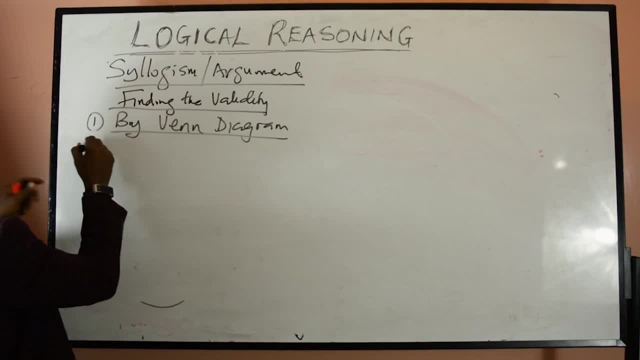 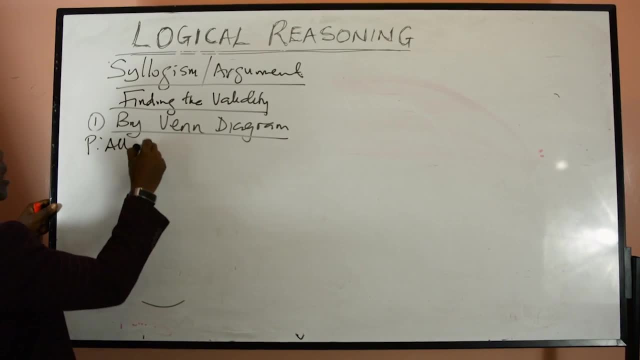 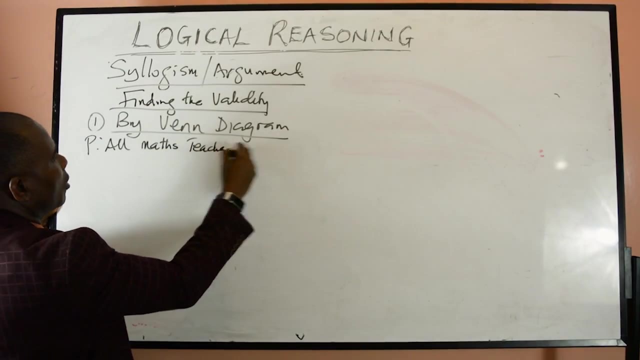 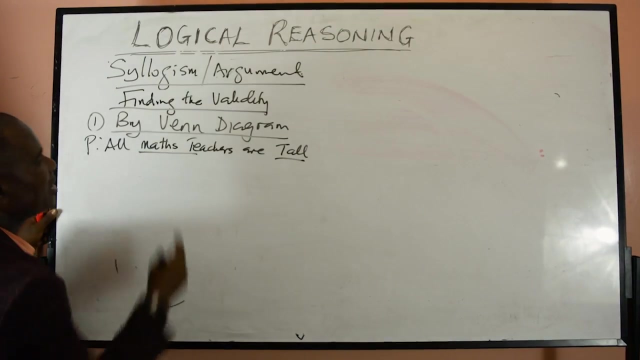 So let's say, for instance: I will develop an argument here. So let's say P. Since it is symbolic, we want to represent the statement based upon the letter. So we say: all mass teachers, All mass teachers are tall, So here. so let's say math, M for math and T for tall. 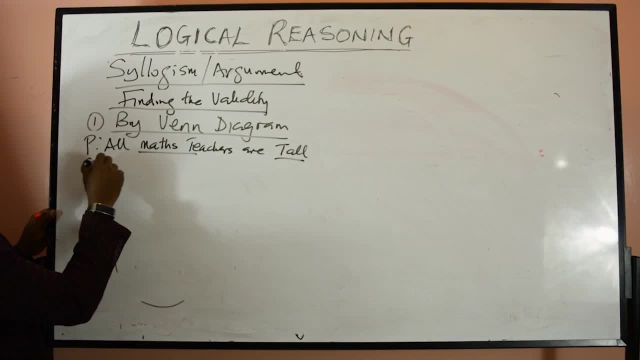 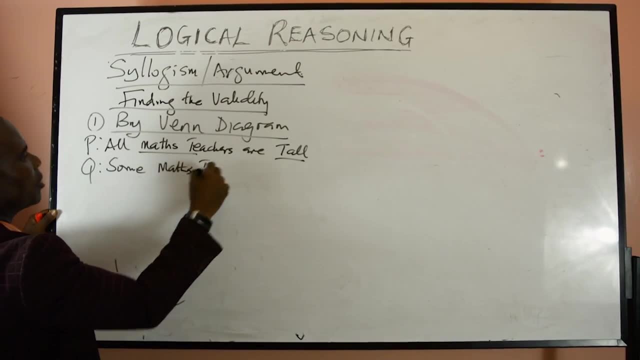 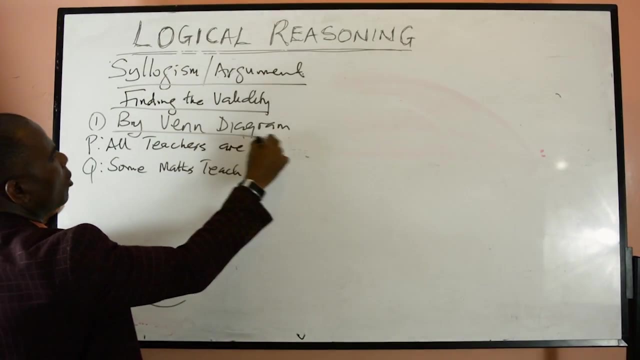 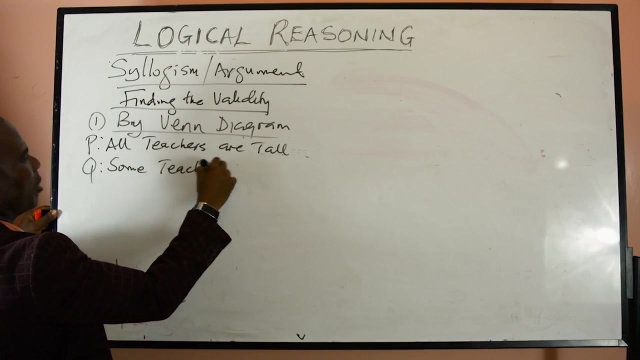 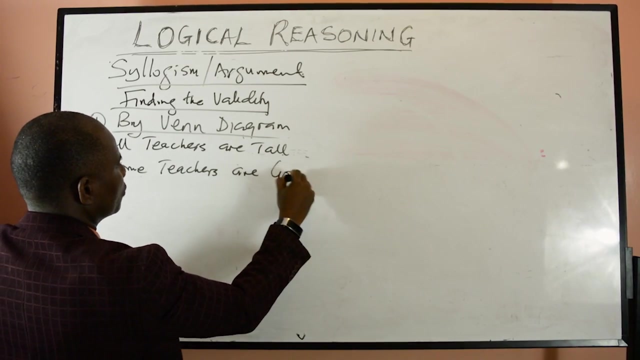 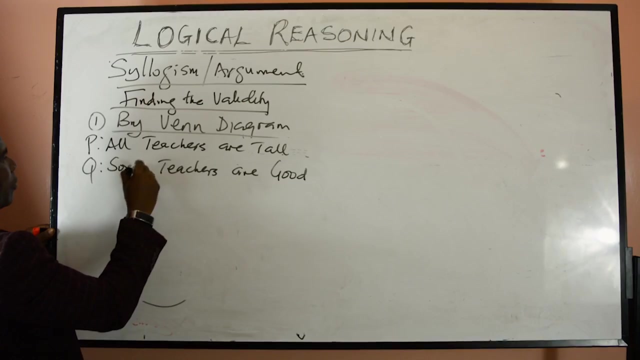 M for mass teachers and T for tall And Q. we can say some mass teachers. Let's say all teachers Are tall. So I can shorten this: Some teachers are good, Some teachers are good. So now we have some. So we can look at the first premise. 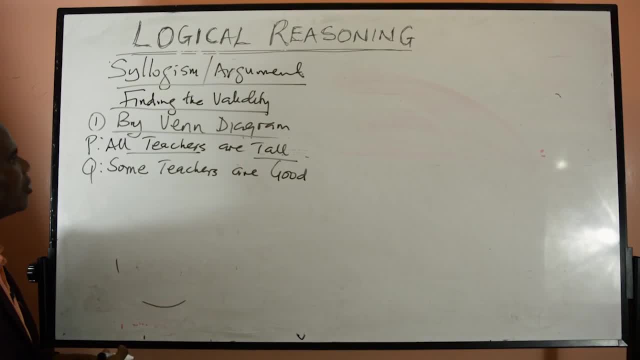 It has two characters in there. We have teachers and tall Or tall. Okay, I better change this tall so that we don't mix the two T's together. So let me still use the mass teachers there. It can help us with that. 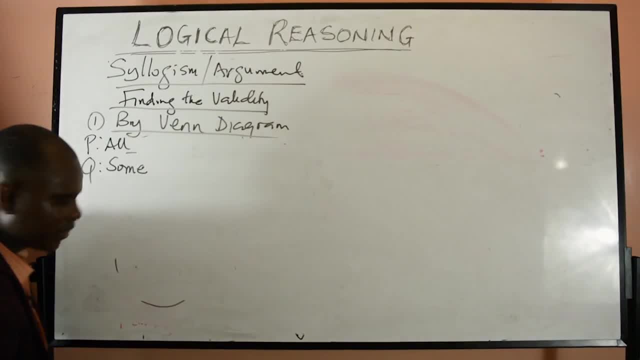 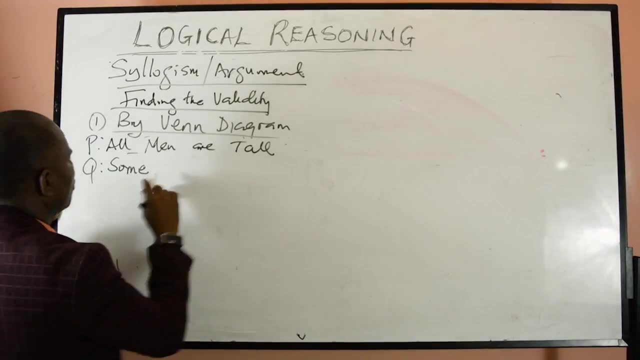 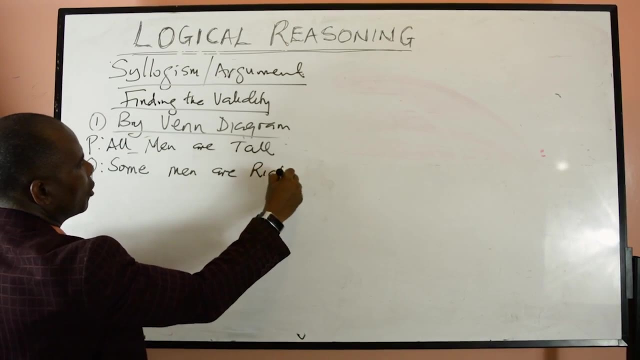 So now we have- because I'm trying to simplify so that we have different letters. So, okay, let me use men. All men are tall, Some men are rich, So let me use that. So tall and unreached. So we have that. 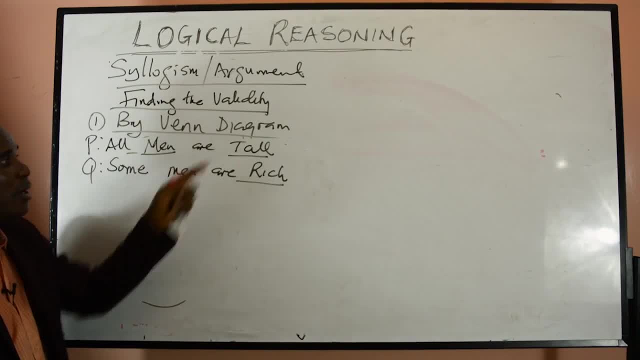 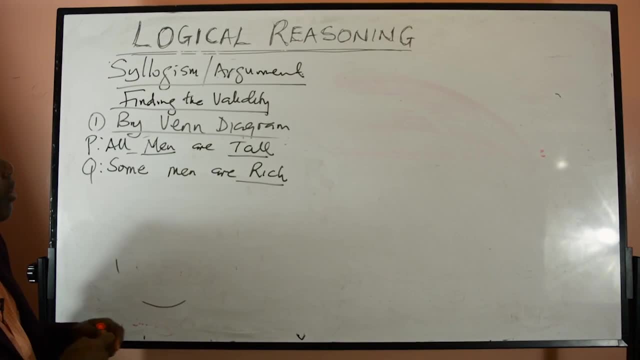 Now I just changed the sentence because I want to have different letters so I don't keep confusing you. So look at it. This is, let's say, represent this. I want to represent this information on a Venn diagram. So let's see the Venn diagram. 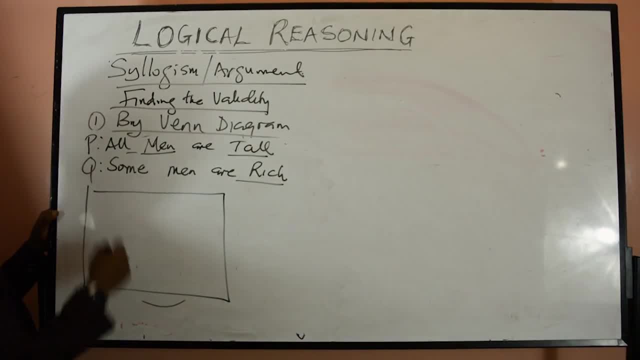 So we have Venn diagram represents men, But this, all men, that's the universal set Let's get Now. we now have all men at all, So we can have This is all men, The two circles together, and you can help me out with this. 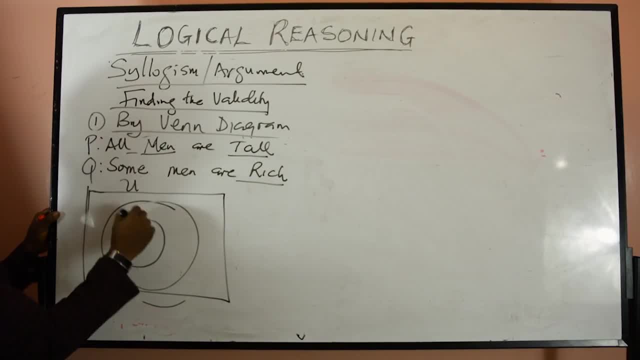 You also move together. So we have tall all men at all. So all the men are inside the tall circle. That's the meaning of the first statement. And now some men are rich, So I can put here rich, So I can put the rich circle somewhere here. 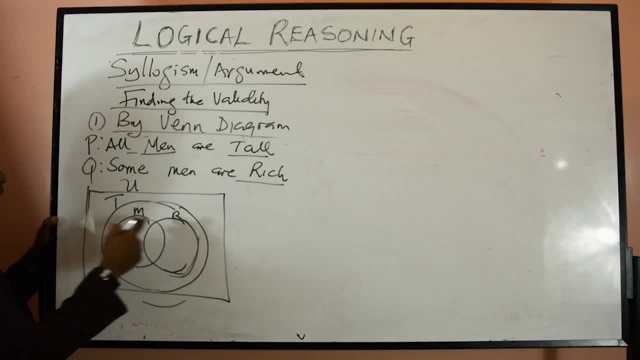 Some men are rich, So not all the men are rich, but some men are rich. Some is intersection. So this, this diagram represent this statement here: This is rich. There is no link between tall and there is no link between tall and rich. 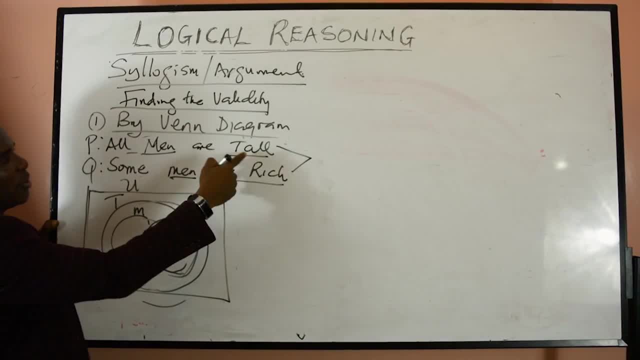 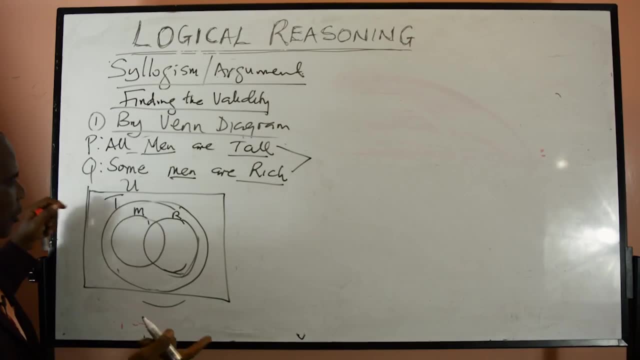 The link here is men- Men is linking tall and men is linking rich. but there is no link between tall and rich. And because there is no link between tall and rich, so I have right to assume here- I'm assuming- that all the rich men at all and we just not indicating the question. but 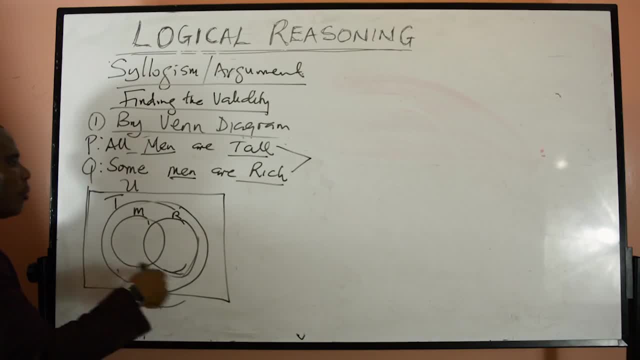 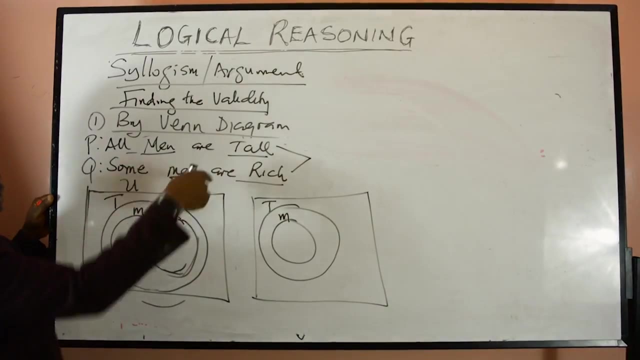 because I want to solve, I'm going to assume that all rich men at all. I can as well draw this Venn diagram. I can say in another form, which is also logically correct: So I have all men at all. I can say all men at all. this is tall, all men at all. 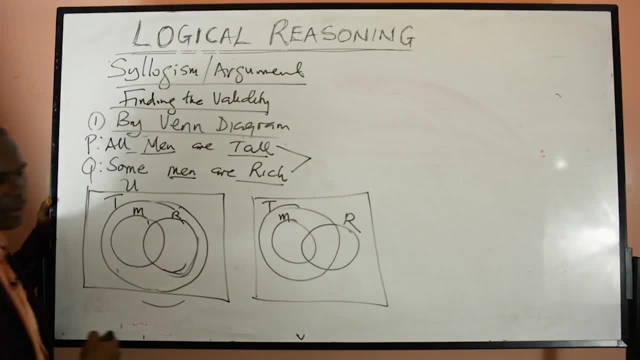 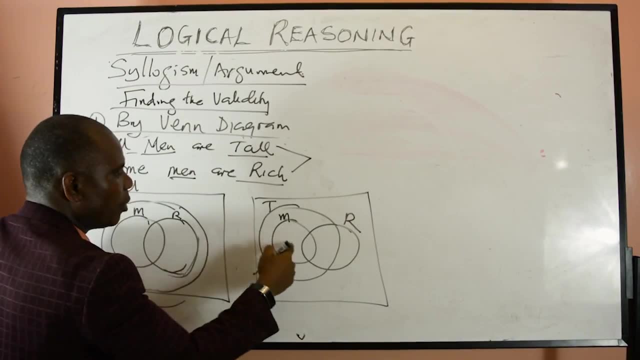 Now, some men are rich, some men are rich. So here I have assumed that not all the rich people at all, and here also not all the rich people are men. So I have this statement also interpret this. This is another form of this statement here. 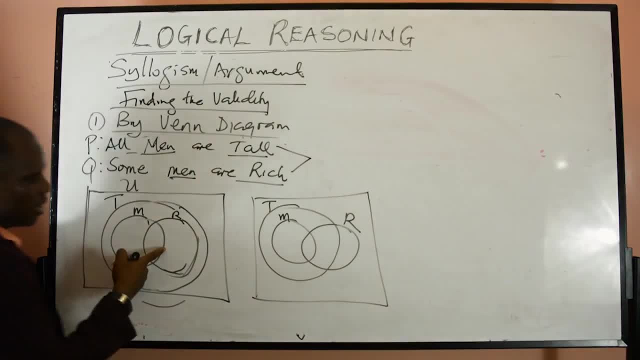 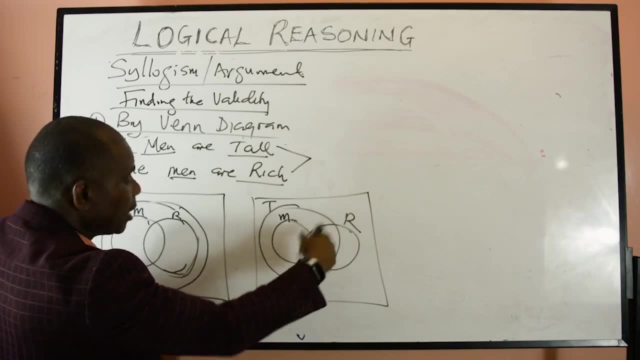 The assumption is that not all the rich people are tall. Here I have assumed that all the rich people are tall, so I put it right inside the tall circle. Here I have taken the rich circle out of this, some of the rich circle out of the tall circle. 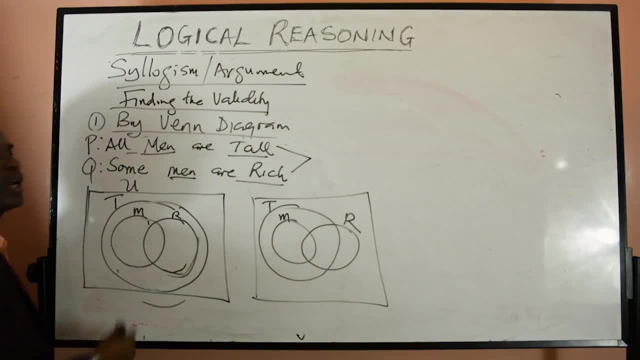 because there is no link between tall and rich. So I can assume here. I can assume here as well. So now I am going to show you a technique of solving this. That is my own technique that I developed so that you can actually see the simplicity. 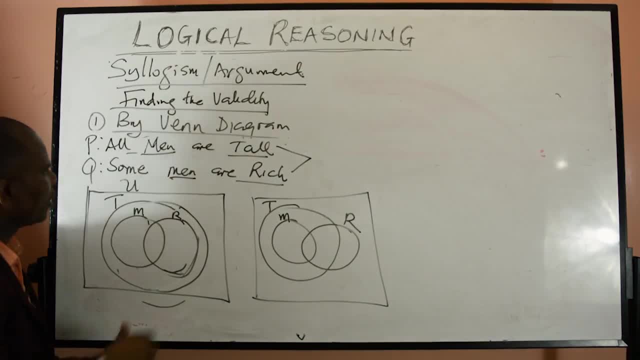 of this First, how do we find the validity now? So if you now have this statement and you are able to form the Venn diagram, then I'm coming to my own procedure. This is my own way of solving it. You can have multiple ways of solving it, but I just want to give you a simple way of. 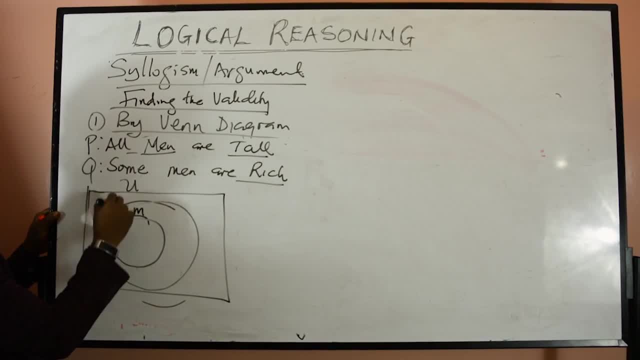 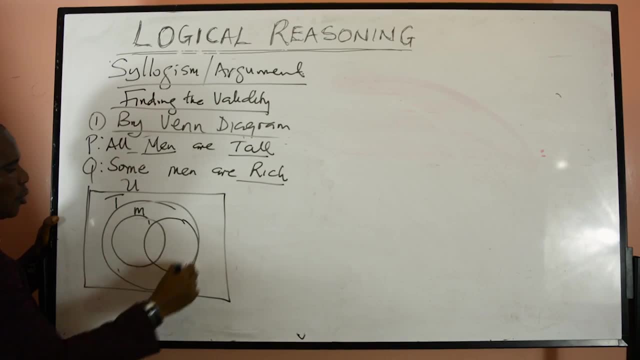 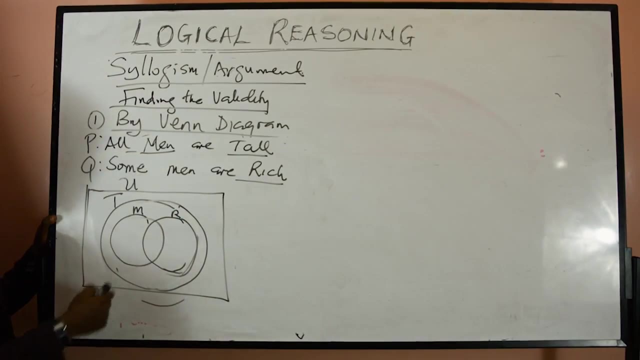 we have tall, all men at all, so all the men are inside the tall circle. that's the meaning of that first statement. and now, some men are rich, so i can put here rich, so i can put the rich sacrosanct here. some men are rich, so not all the men are rich, but some men are rich, some is. 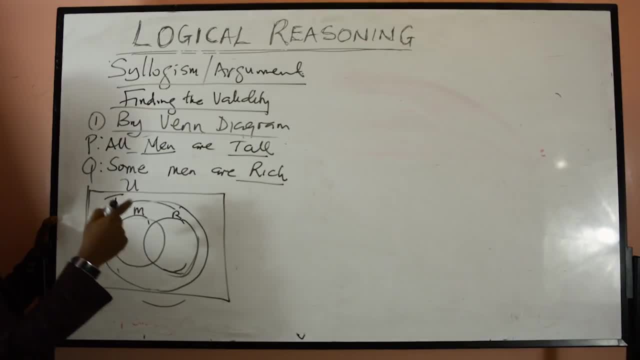 intercession. so this, this diagram represents this statement here. this is rich. there is no link between tall and there is no link between tall and rich. the link here is men- men is linking tall and men is leaking rich. but there is no link between tall and rich. and because there is no, 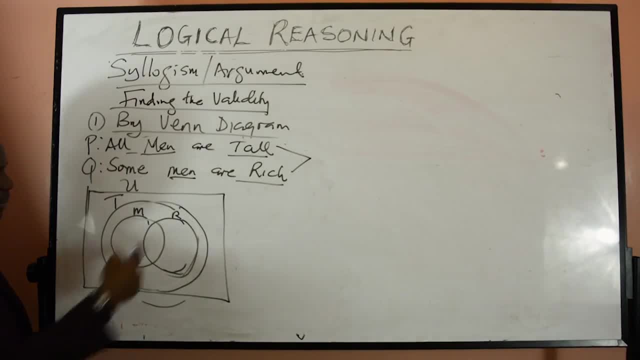 link between tall and rich. so i have right to assume here i'm assuming that all the rich men at all, and we just not indicating the question, but because i want to solve, i'm going to assume that all rich men at all. i can as well draw this vein in another form, which is also logically. 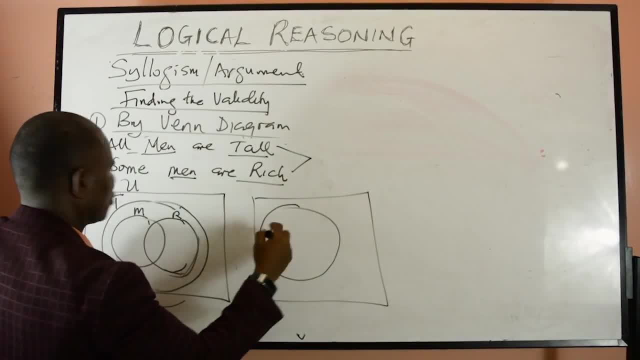 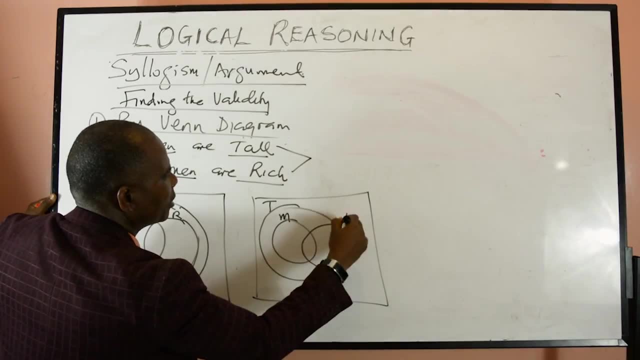 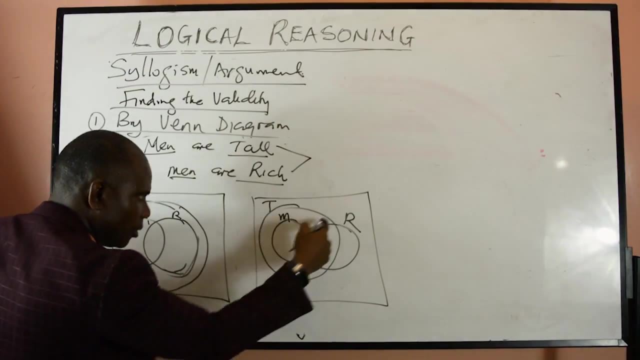 correct. so i have all men at all. i can say all men at all. this is tall, all men at all. now some men are rich, some men are rich. so here i have assumed that not all the rich people at all, and here also all the rich people are men. so i have this statement also interpreted this. this is another. 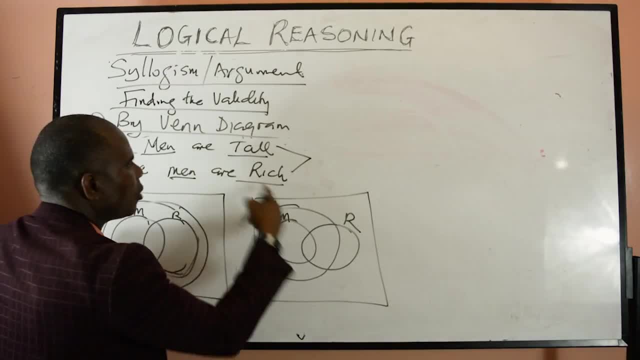 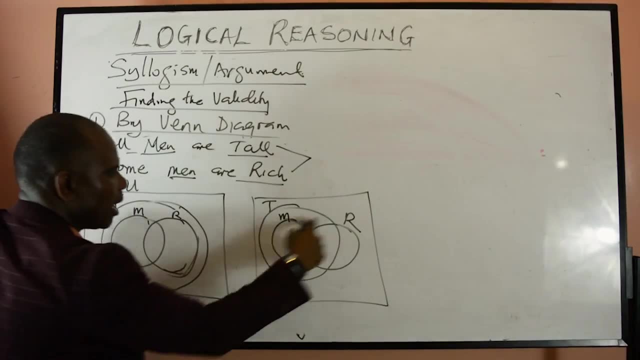 form of this statement. here the assumption is that not all the rich people at all here i have assumed that all the rich people are taught, so i put it right inside the thought cycle here. i have taken this rich circle out of this, some of the rich circle out of the thought cycle, because there's 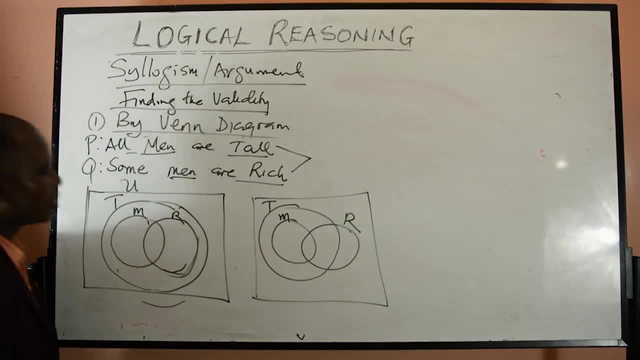 no link between tall and rich. i can assume here. i can assume here as well. so now i am going to show you a technique of solving this. that is my own technique, that i didn't know how to solve it, but i am going to show you a technique that i didn't know how to solve it, but i have developed so that you can. 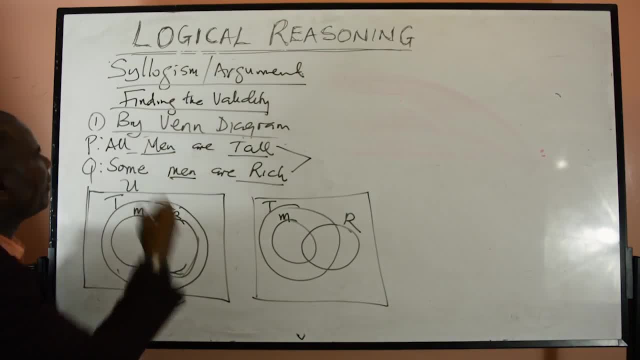 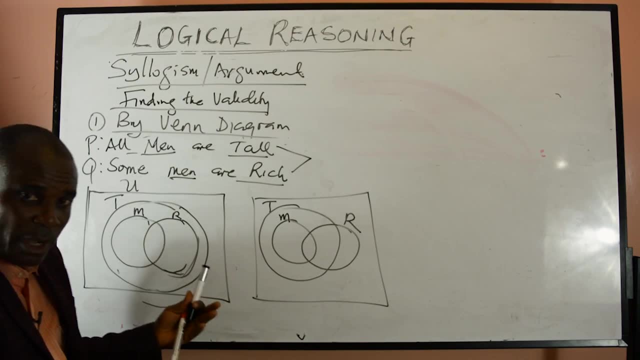 actually see the simplicity of this first. how do we find the validity now? so if you now have this statement and you're able to form the venn diagram, then according to my own procedure, this is my own way of solving it. you can have multiple ways of solving it, but i would just want to give 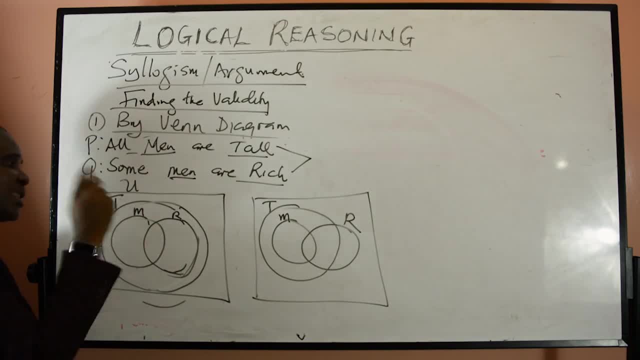 a simple way of understanding this concept, for as much as it has a lot of grammar inside, here you have to find shortcuts to make the student understand. so i've designed a way for the student to understand this. this is my own opinion, so let's look at it and it is logically correct. 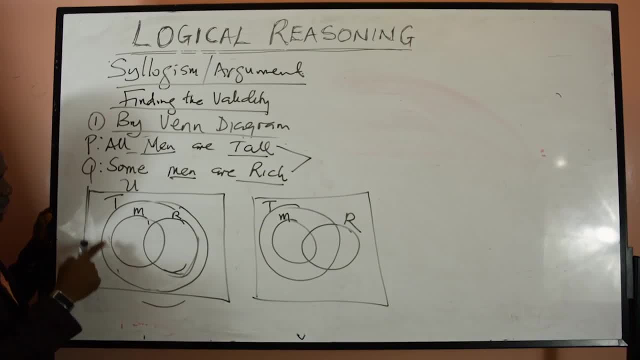 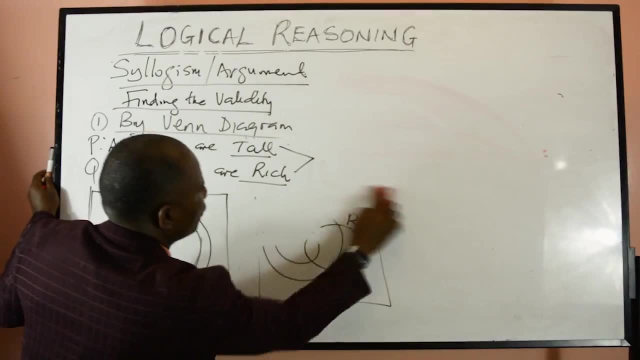 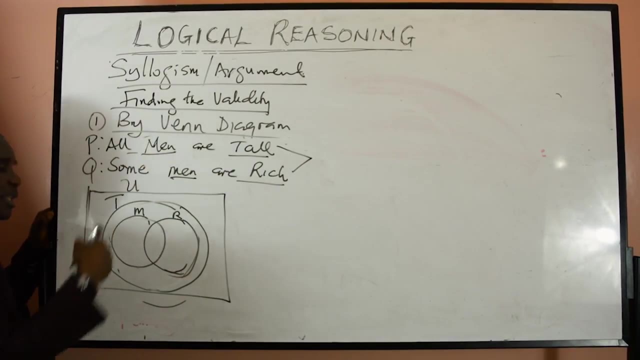 so so we have a. i'm going to find i'm going to leave this component in this, so let's just concentrate on this one first and leave that, so that i don't get to confuse you more. so we get this out. so i have already represented these two statements in there, so if i now write the 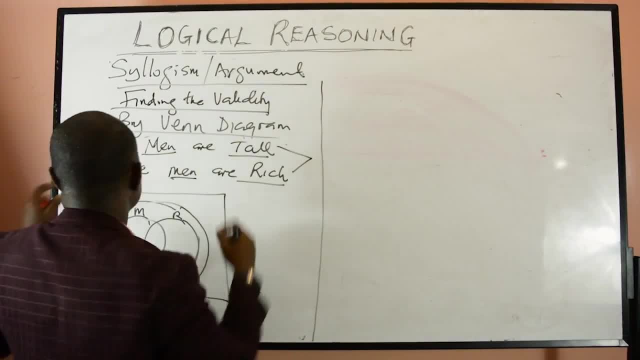 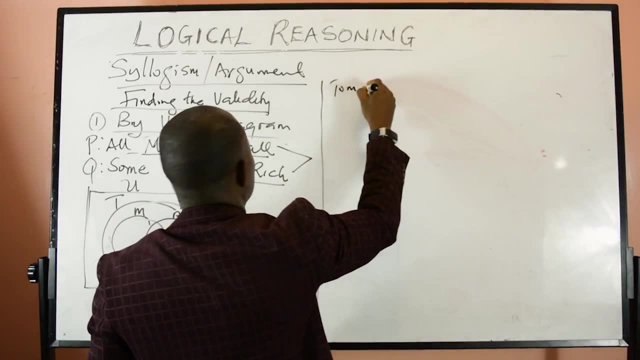 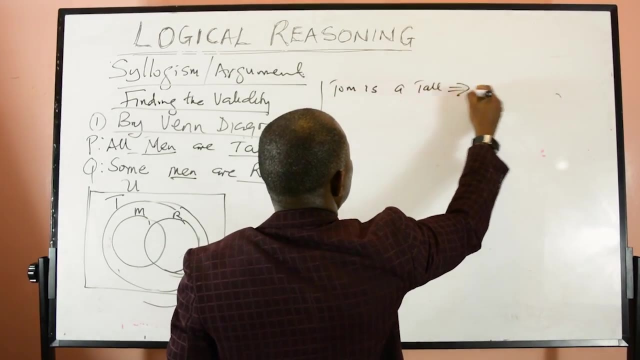 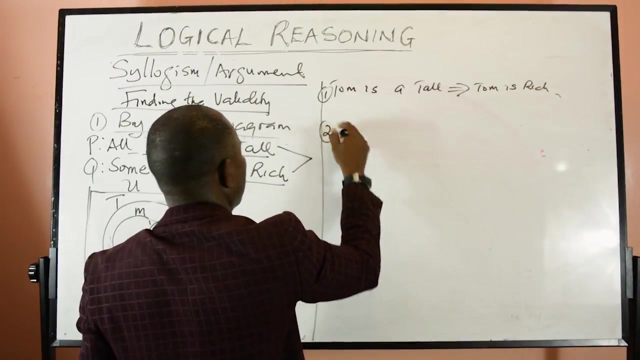 questions. let's say i want to find the validity of the first question. let's say: use your venn diagram now to illustrate to find the validity of the following statement. let's say: first: tom. tom is a store implies tom is rich. so i can also write: say fat matter, fat matter is. 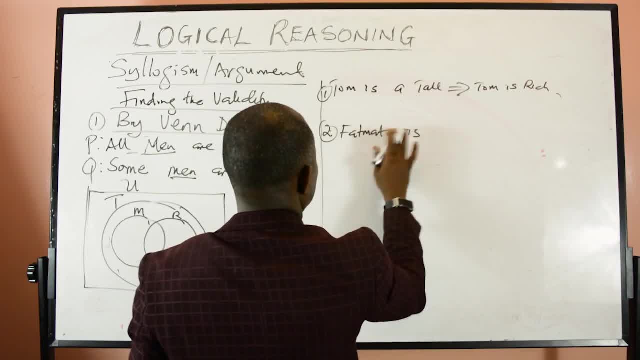 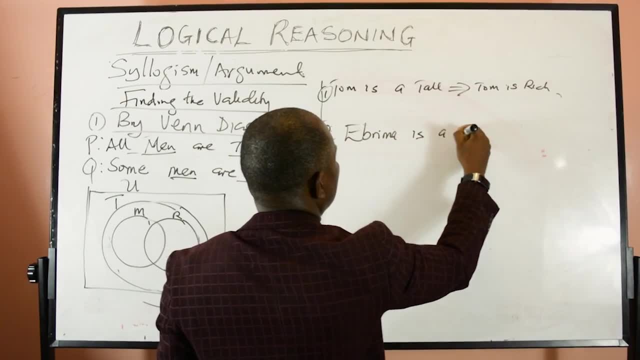 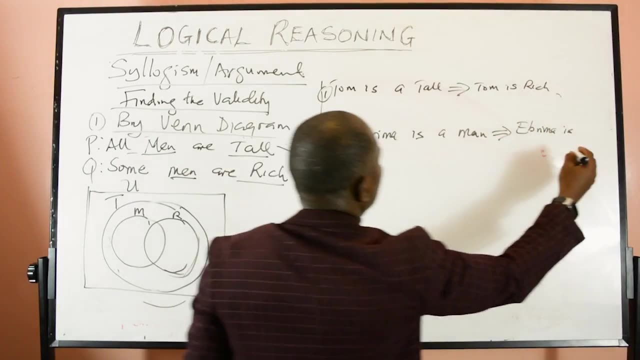 fat matter. okay, let's say not because i've used me, let me use ibu, ibu or ibrahima. ibrahima is a man, implies ibrahima is tall. so i want to look at this venn diagram and i i'm going to design my own way of solving. 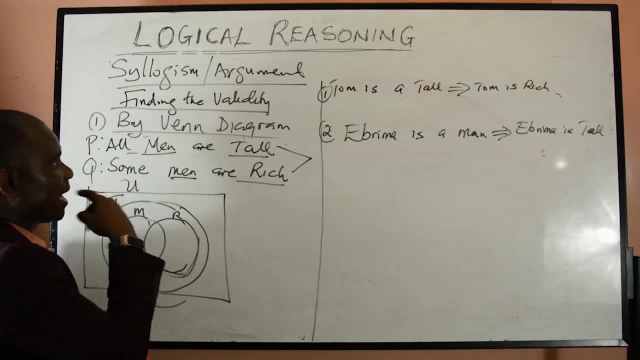 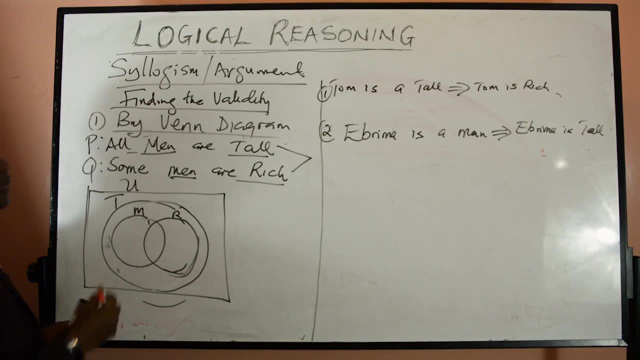 it. i want to find the validity of these two statements using this venn diagram. these statements are coming from here. we're using this assertion to get the validity, so let me first step is: according to my own uh design, you can follow up, you can see, verify that i. i said i can try to this um describe the various uh portions of this. 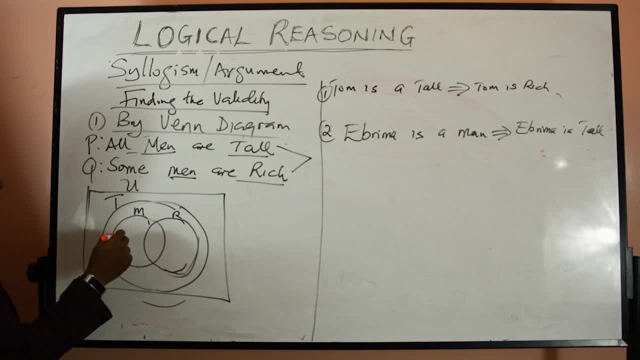 venn diagram. so i have a portion here, this room. i have another room somewhere here, i have another room here, another room here, so i can just leave the rooms. this room is the same as this room because they're occupying the same, it's the same space. so you see, here it is inside. 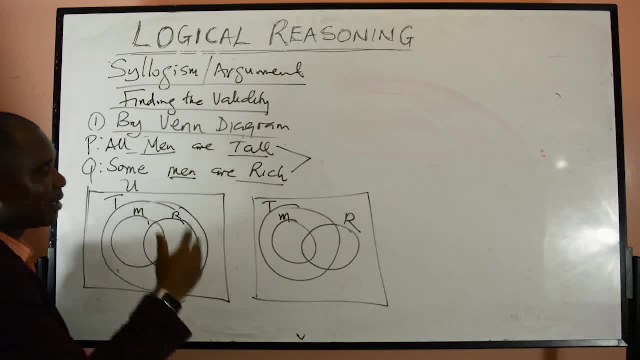 understanding this concept, For as much as it has a lot of grammar inside, here you have to find shortcuts to make the student understand. So I have designed a way for the student to understand this. This is my own opinion, So let's look at it and it is logically correct. I think so. 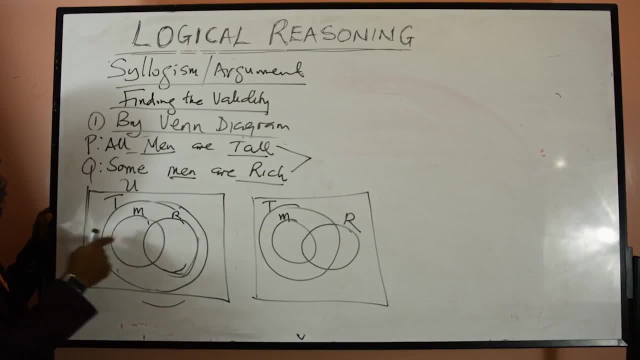 So we have A I'm going to find I'm going to label this component in this, So let's just concentrate on this one first and leave that, So that I don't get confused. Okay, Okay, Okay, I don't get to confuse you more. 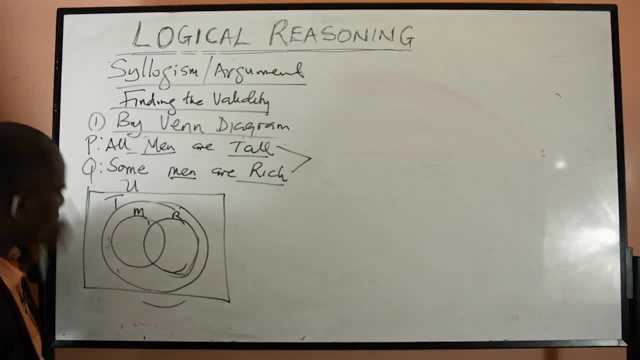 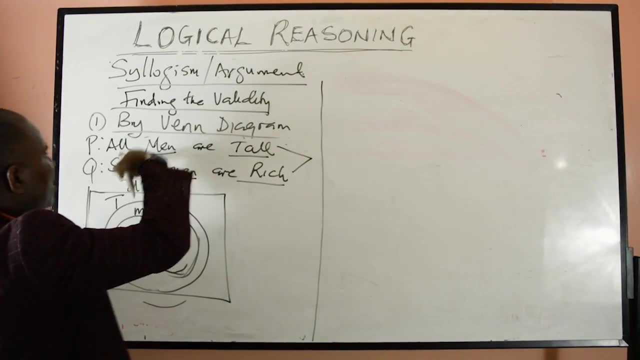 So we get this out. So I have already represented these two statements in there. So if I now write the questions, let's say I want to find the validity of the first question, Let's say, use your Venn diagram now to find the validity of the following statement. 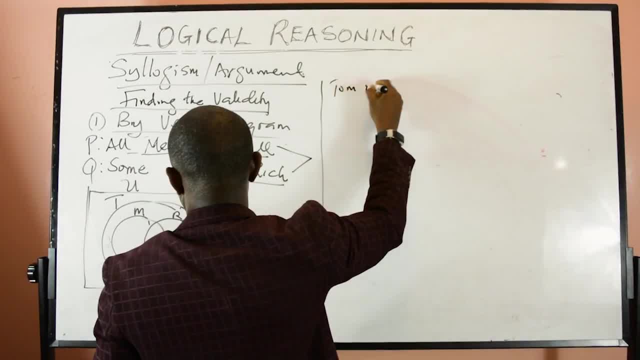 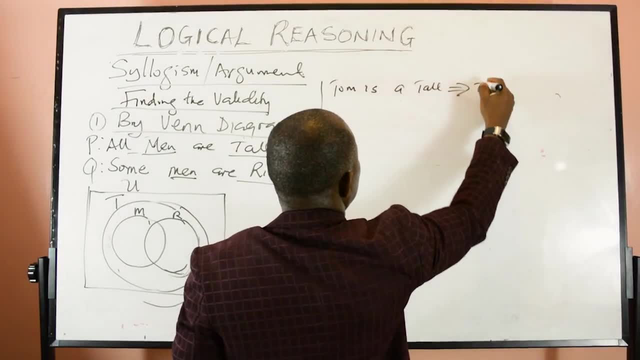 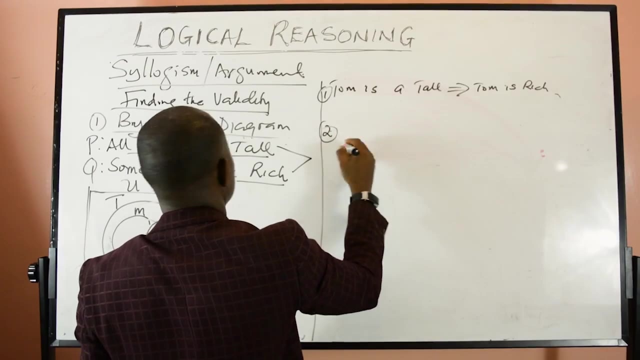 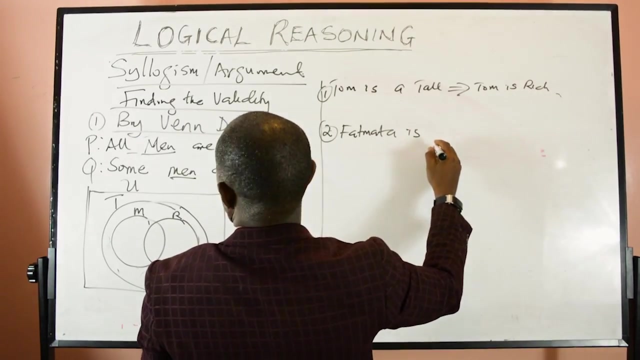 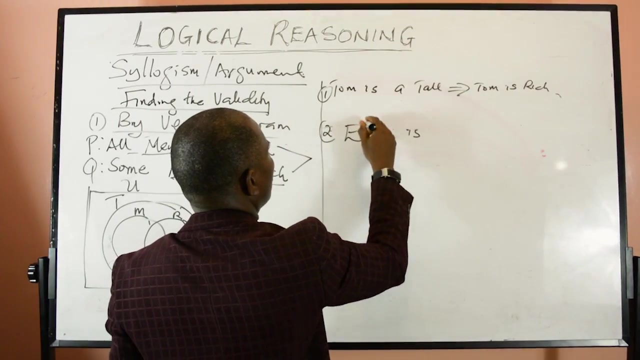 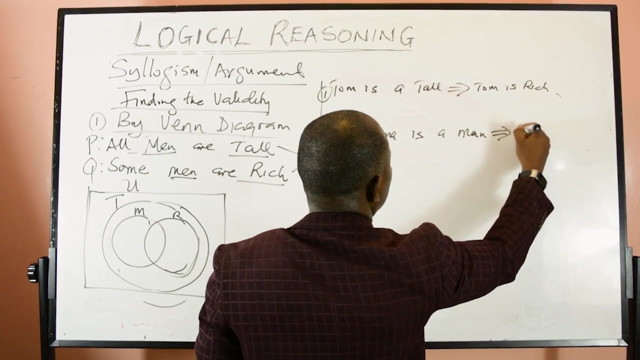 Let's say first: Tom, Tom is is tall implies Tom is rich. So I can also write, say Fatmata, Fatmata is Fatmata. okay, let's say not because I've used men, let me use Ibu, Ibu or Ibrahima. Ibrahima is a man, implies Ibrahima is tall. 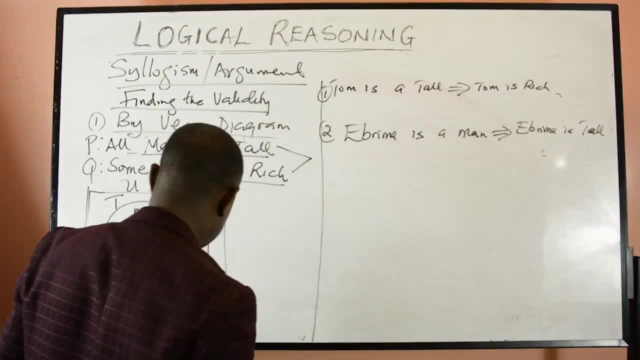 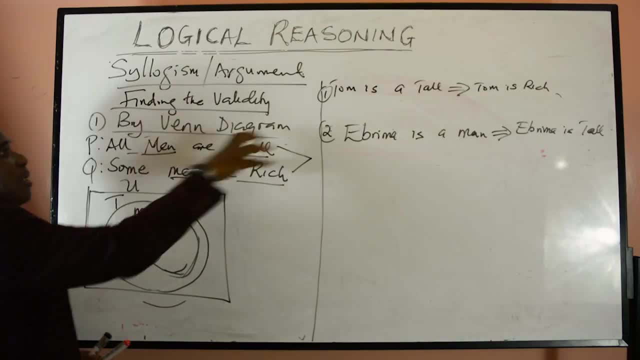 so I want to look at this Venn diagram and I'm going to design my own way of solving it. I want to find the validity of these two statements using this Venn diagram. These statements are coming from here. we're using this assertion to get the validity. 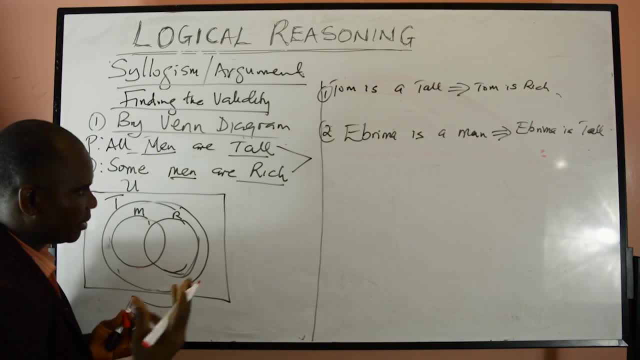 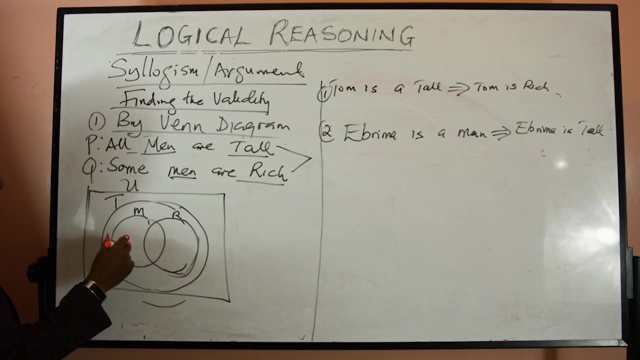 So let me first step is according to my own design. you can follow up, you can see, verify that. I said I can try to describe the various portions of this Venn diagram. So I have a portion here, this room. I have another room somewhere here I have another. 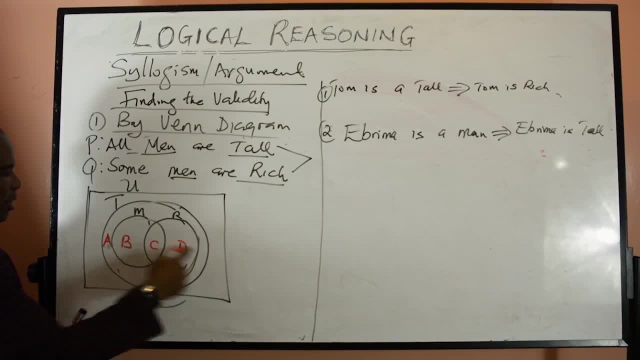 room here, another room here, so I can just label the rooms. This room is the same as this room because they are occupying the same, the same space. so you see, here it is inside one circle, this part is also inside one circle. 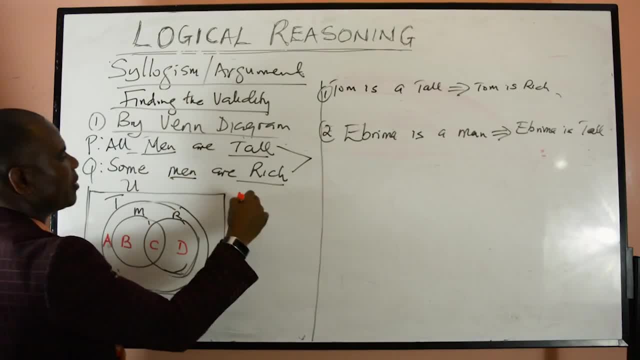 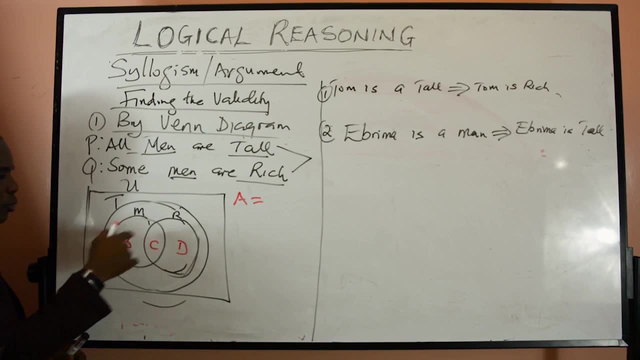 one circle. this part is also inside one circle, so i have to now define the members of each circle, member of each room here. let me call them rooms. this is room 1, room room 2, room 3, room 4. i call them room a, room b, c, d. so let me define the members that are inside room a, the members in 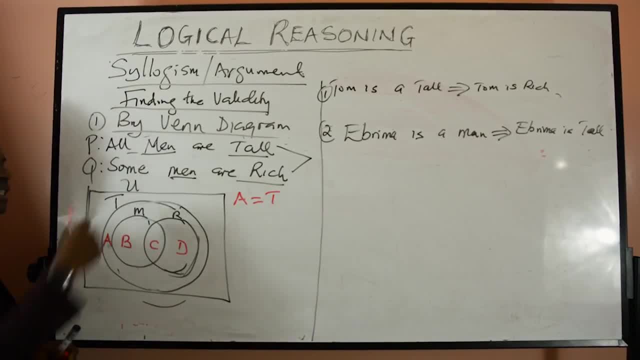 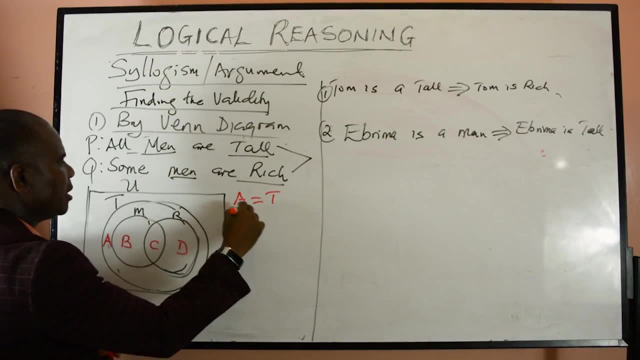 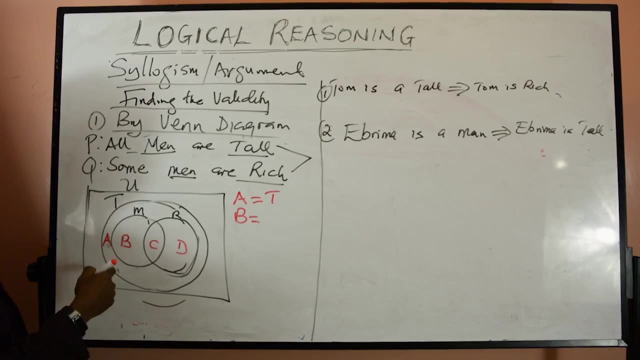 room a are all tall people, because a is only found inside the tall circle, so it is only encompassing the a. the a is inside the tall circle only, so we have the b. room b is encompassing two circles here. it has the main circle and it also has the tall circle, so we have m and t there now. 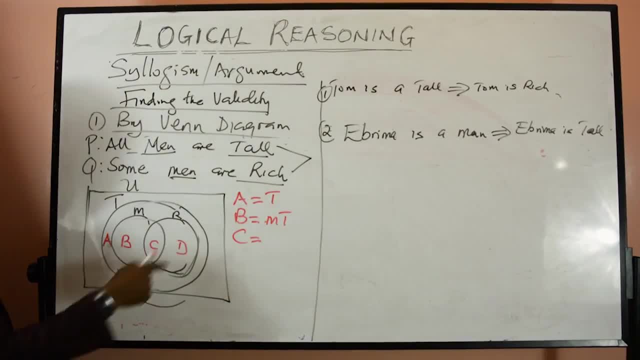 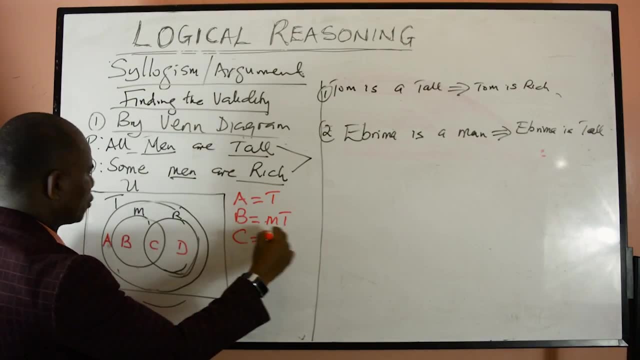 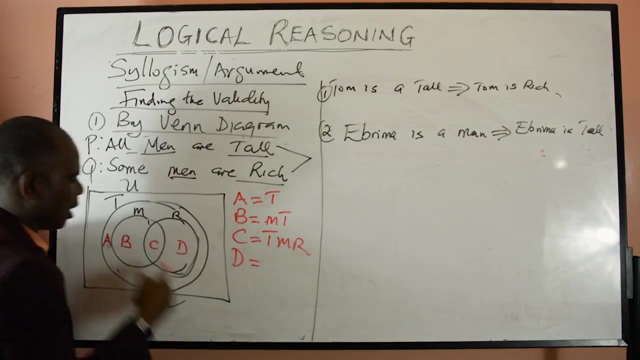 we have room c. room c contains the three circles. we have the tall. it's inside the tall circle. it's inside the main circle. it's also inside the rich circle. so you have tall m rich. that is room c. room c has all three circles put together. room d, room d has rich circle. it is inside the tall. 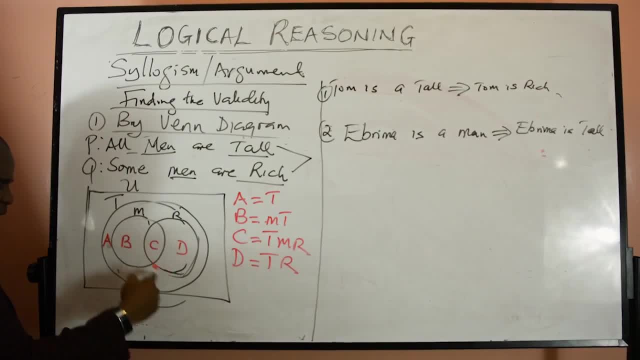 circle. so you have tall and rich circle. so you have tall and rich circle. so you have tall and rich inside. you have tall circle there, tall circle. that is where d is and d is also inside the rich circle. so you have the four rooms as i have labeled them. now you come look at this. i'm 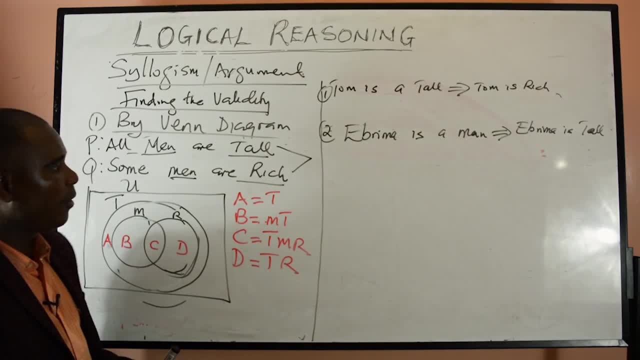 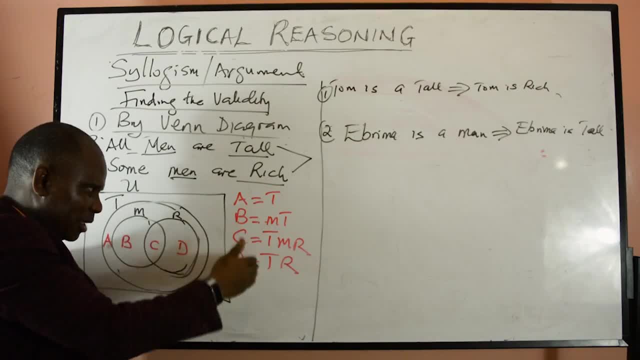 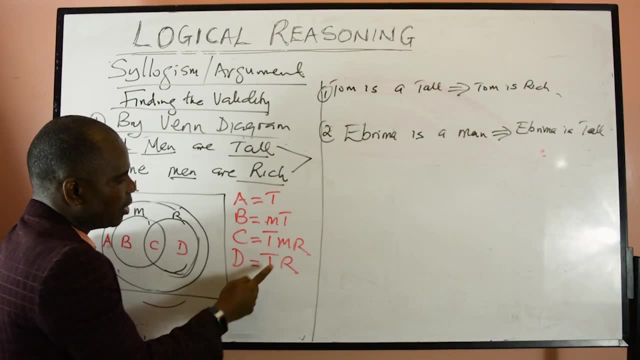 you. it makes my statement valid because the t is found all inside the room. but if i say all the rooms have m, it makes it invalid. because this room do not have m, this room do not have m. that statement becomes invalid because there is m. there's no m here. there's no m here. so it makes 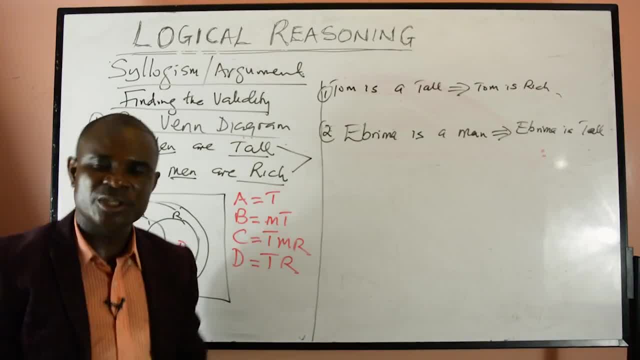 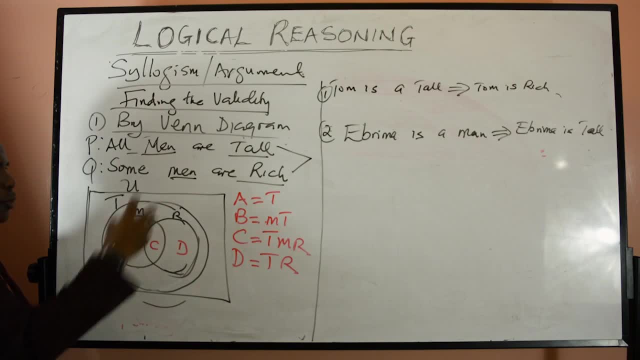 it invalid. so when once there is a question mark on my statement, it makes the statement invalid. so watch out here. this is simplified form of answering that question. first you locate the rooms and you try to identify which type of qualities are in certain rooms. and if you now look at the questions, if the questions 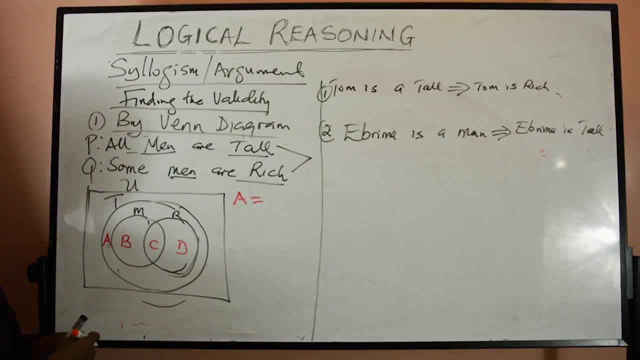 So I have to now define the members of each circle, member of each room here. Let me call them rooms. this is room one, room two, room three, room four. I call them room A, room B, C, D. So let me define the members that are inside room A, The members. 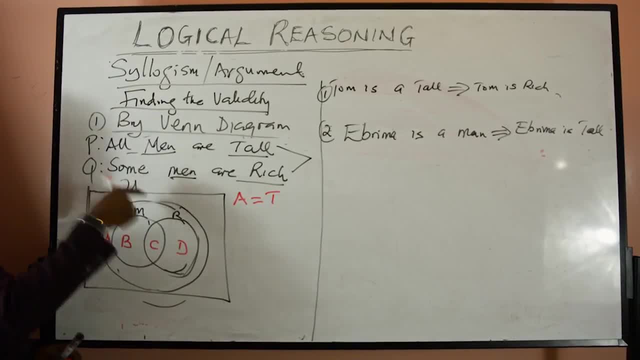 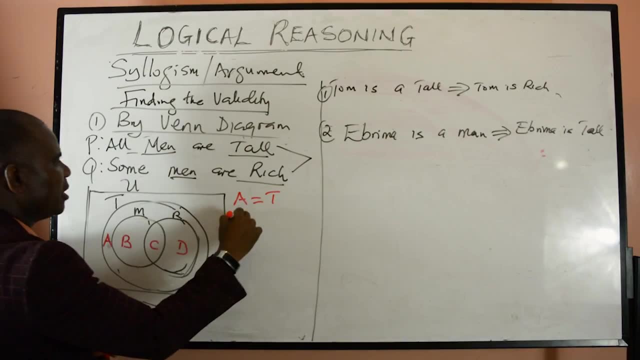 in room A are all tall people, because A is only found inside the tall circle, So it is only encompassing the A. the A is inside the tall circle only, So we have the B Room. B is encompassing two circles here. it has the main circle and it. 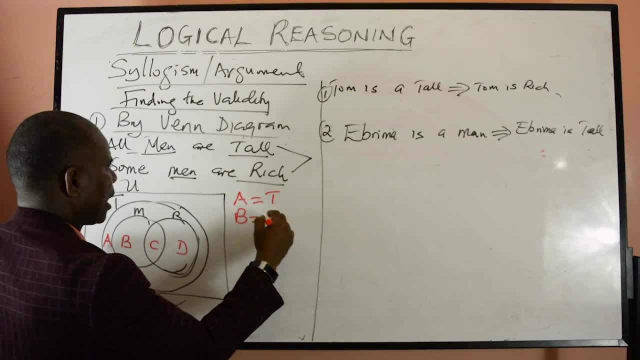 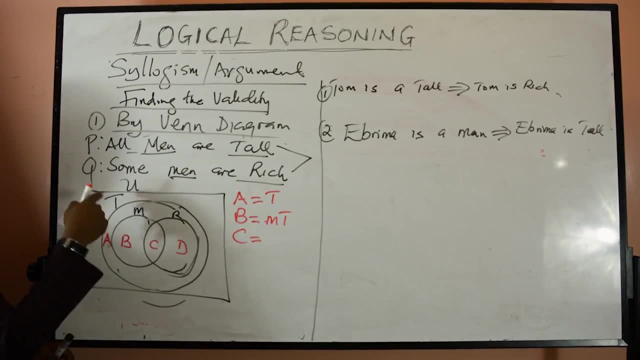 also has the tall circle. So we have M and T there. Now we have room C. room C contains the three circles. We have the tall. it's inside the tall circle, it's inside the main circle. it's also inside the rich circle. 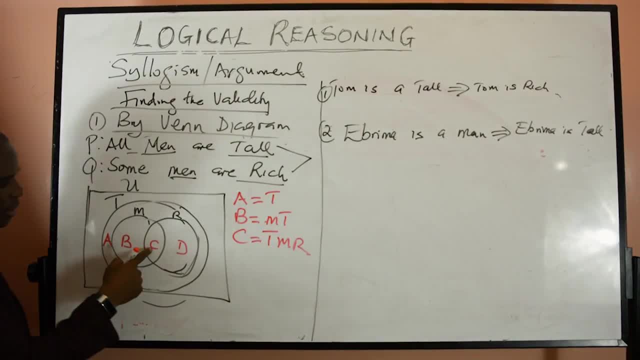 So you have tall M, rich. that is room C. Room C has all three circles put together, Room D. room D has rich circle. it is inside the tall circle. so you have tall and rich inside. You have tall circle there. tall circle that is where D is and D is also inside the rich. 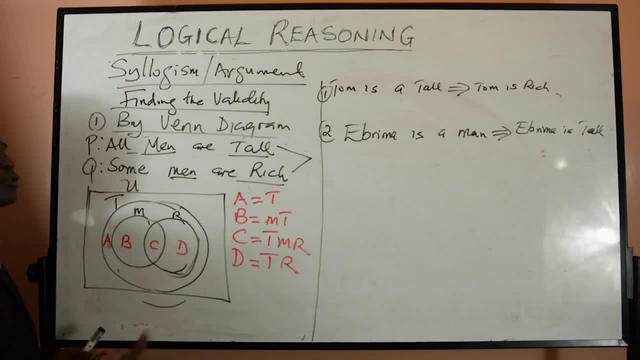 circle. So we have the four rooms as I have labeled them. Now you come, look at this. I'm coming to a chart. now Let's say, for instance, if I say there are four, if I say all the rooms are inside the 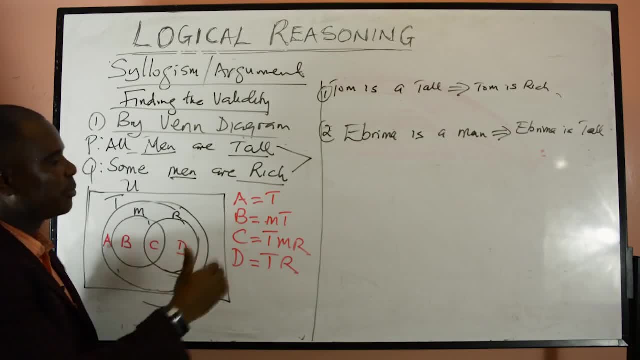 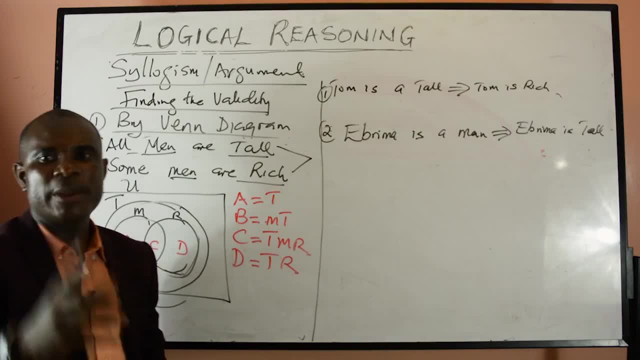 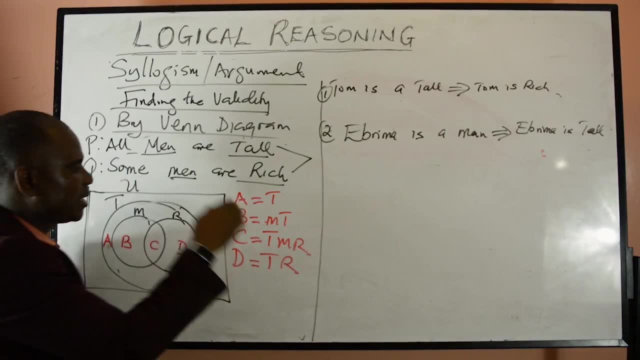 room. But if I say all the rooms have M, it makes it invalid. because this room do not have M, this room do not have M. that statement becomes invalid because there is M. there is no M here. there is no M here. 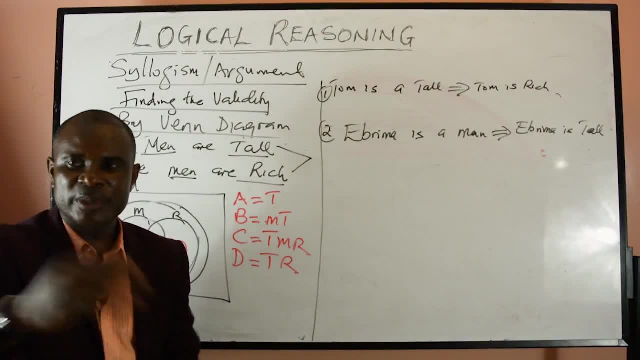 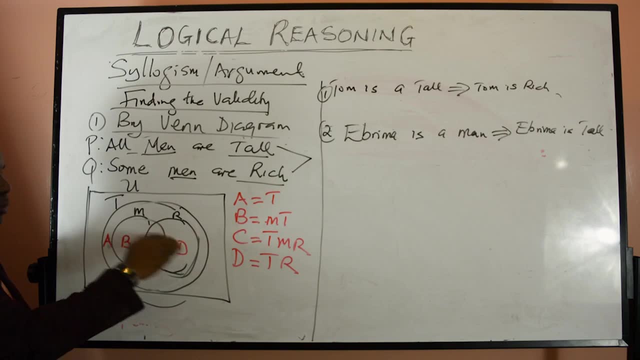 so it makes it invalid. so when, once there is a question mark on my statement, it makes the statement invalid. so watch out here. this is a simplified form of answering that question. first, you locate the rooms and you try to identify which type of qualities are in certain rooms. 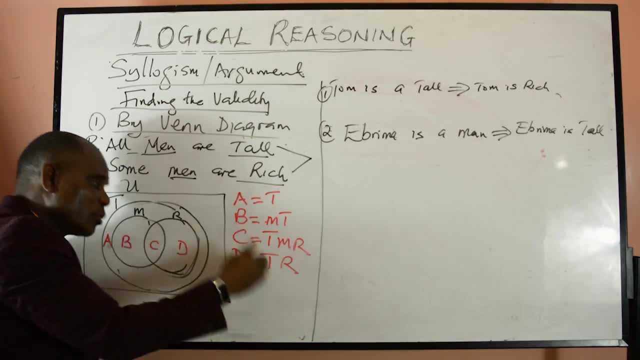 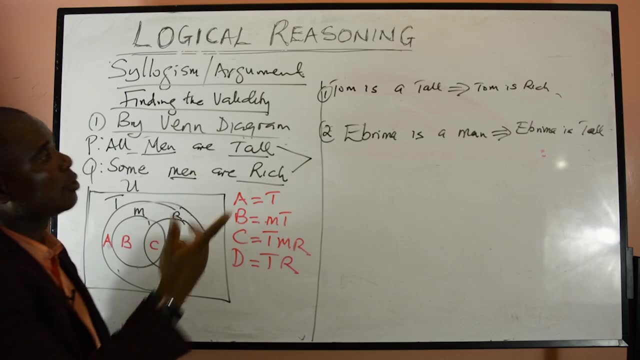 and if you now look at the questions, if the questions now go with whatever room you are bringing, then you can now see you're going to be able to identify the validity of the statement. let's do it to solve that tone is tall, so it means tom is inside the tall tackle. so i'm going to look. 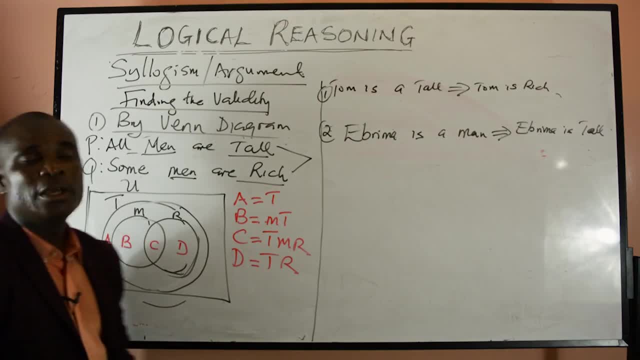 now go with whatever room you are bringing. then you can now see, you can be able to identify the validity of the statement. let's use it to solve that. tom is tall, so it means tom is inside the tall circle. so i'm going to look at the tall circle and look at all the rooms that are available in. 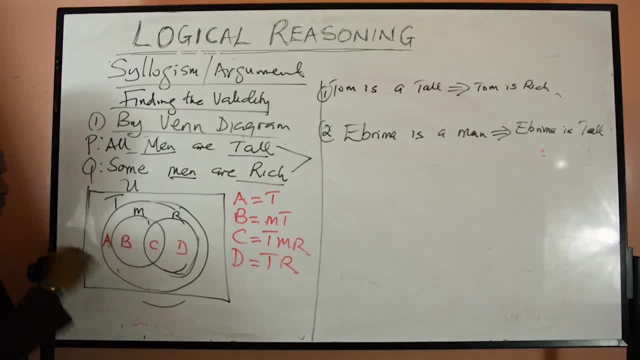 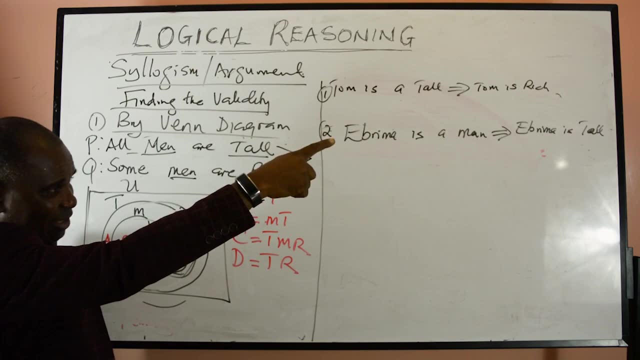 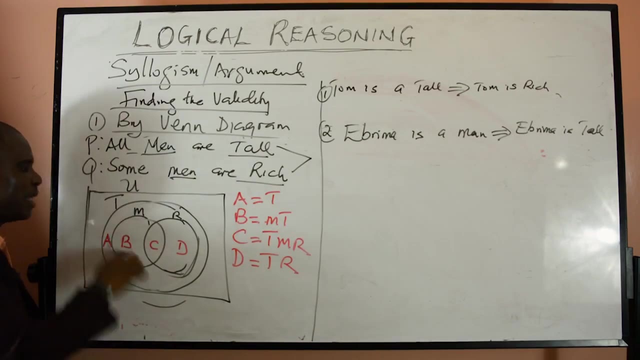 the tall circle. in the tall circle, the tall oval, all the rooms, all the letters are there. so if all the letters have are there, that is tom is rich. that's the conclusion. if all the letters have, are all the rooms have, are? it makes that statement valid. but if there is a room inside the tall 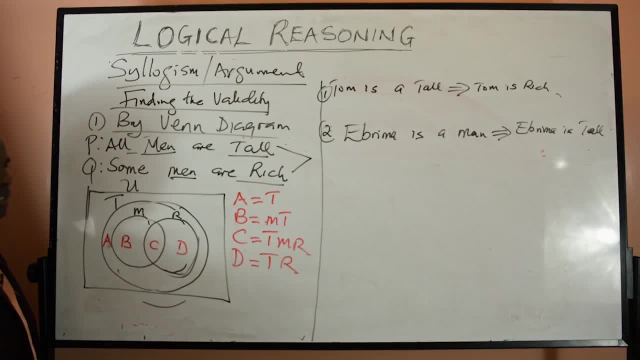 circle that do not have r. it makes that statement invalid. so let's check it out now. we have: a is inside the tall circle. m is inside this. b is inside the tall circle. c is inside the circle. d is inside the circle. so we can now conclude that all the rooms must have tall, but this guy. 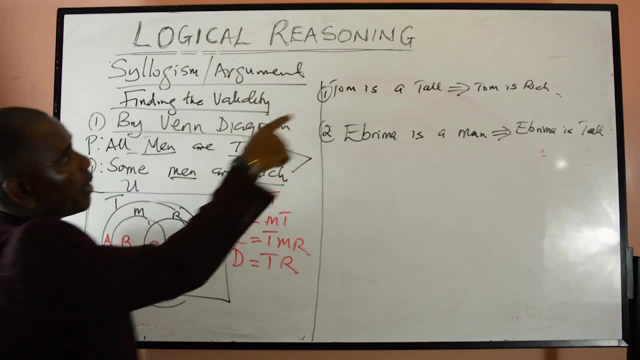 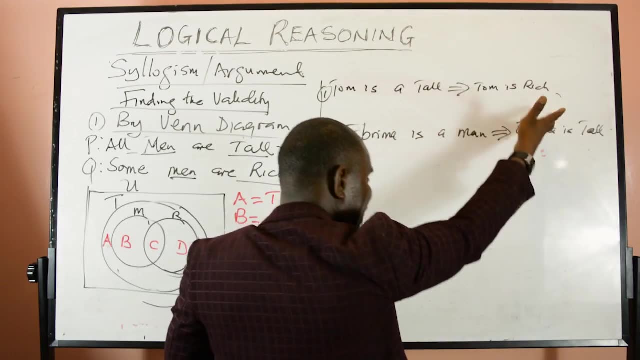 is. we have looked through the rooms. now. if we now conclude c, tom is a ton is tall, it means tom is inside the tall circle. it means that it implies that tom is rich. so that statement becomes an invalid statement because inside the total circle there is a room. 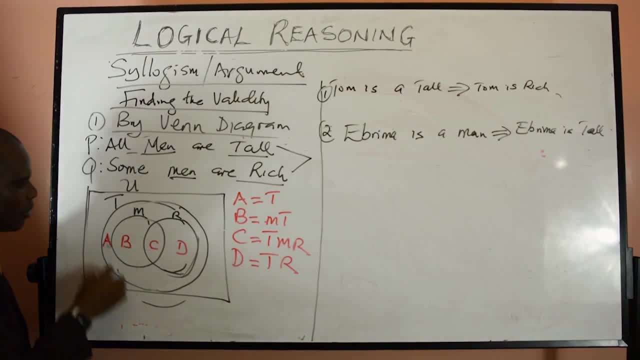 that do not have rich. there is a portion on the start circle that do not have the reach, that do not have rich there. so if you check it there, you can see that this portion here do not have the rich circle here workshop, who does not reach, here you circle does not reach. 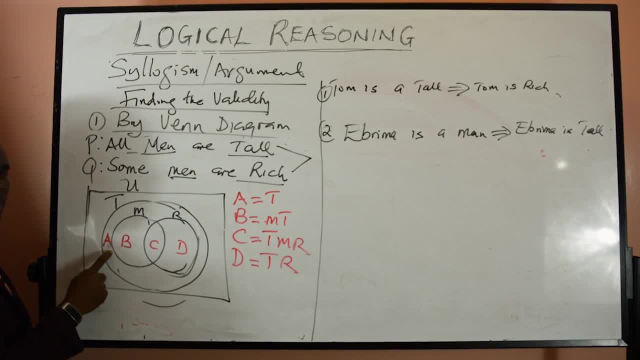 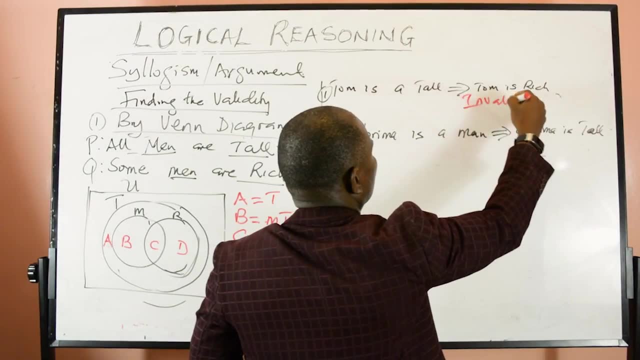 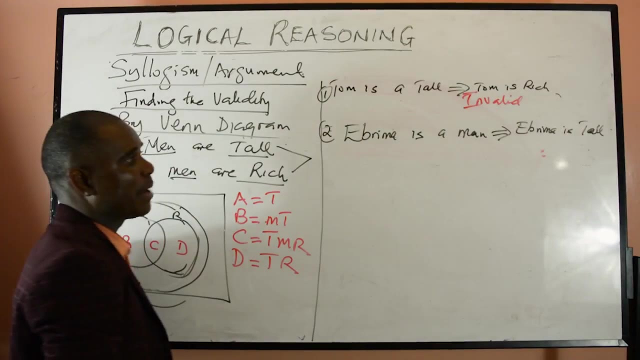 here, so it could be that stone can be inside b and tom coming inside a. so it makes that statement invalid. that is an invalid statement. so I call it invalid statement. so what else when once the conclusion is not supported there, then you make it an invalid. so let's look at a grandma. a grandma is a man, implies a. 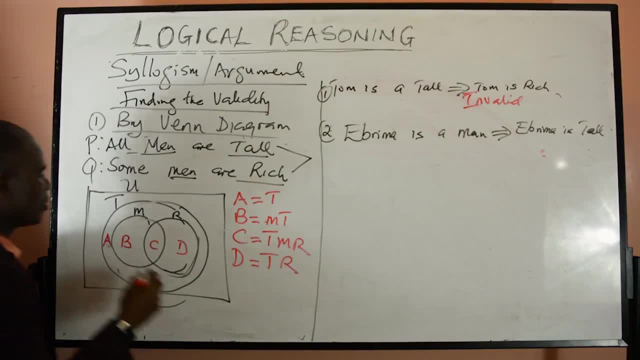 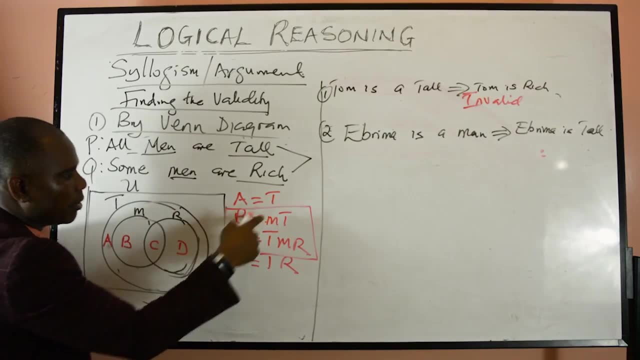 grandma is tall, so let's go to the man circle. we go to the main circle. the main circle contains B and C, so inside B and C circle we have therefore a. grandma is tall, so we see T appearing here and T appearing here, so it means that B even 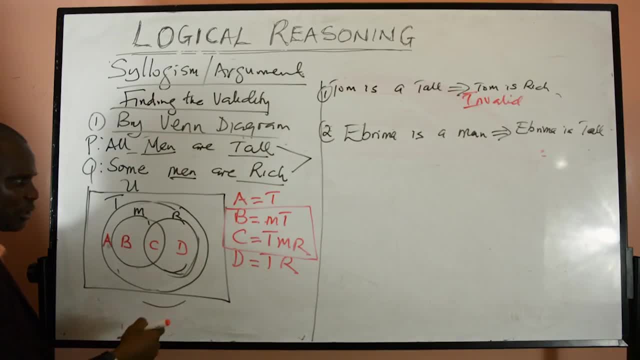 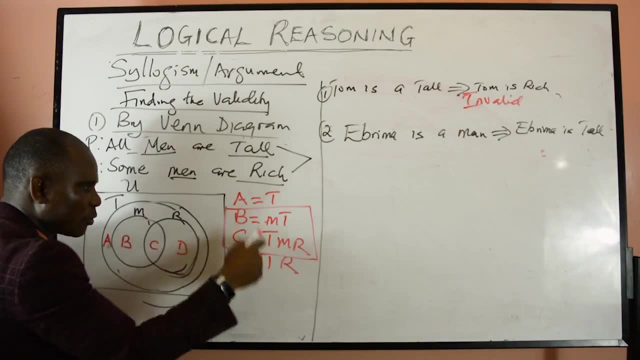 if a grandma was inside this room, it's gonna be classified as a tall person. if a bell insides the see you room is also good to be classified as a tall person, because T is found in boot of the rooms and the room, the room that contains the 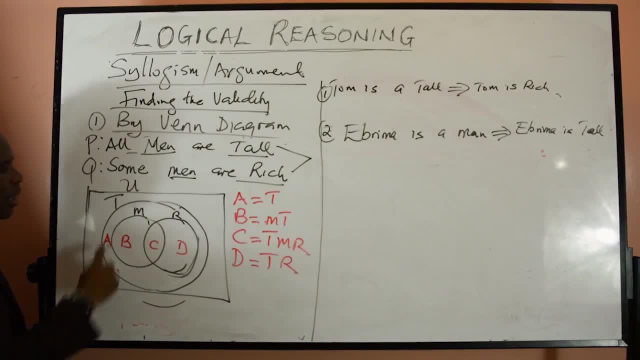 at the top circle and look at all the rooms that are available in the top circle. in the third circle, the tall over all the rooms, all the letters are there. so if all the letters have are there, that is, tom is rich. that's the conclusion. if all the letters have r, all the rooms have r, it makes that. 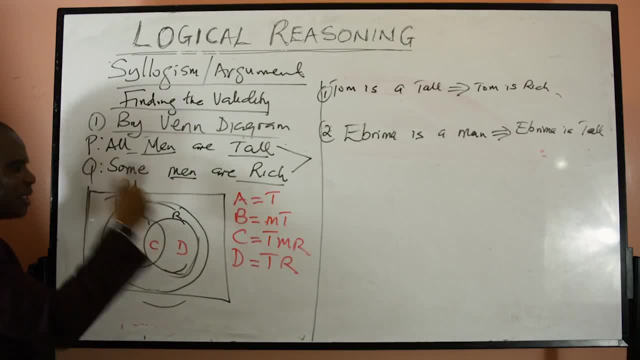 statement valid, but if there is a room inside the tall circle that do not have r, it makes that statement invalid. so let's check it out now. we have: a is inside the tall circle, m is inside this. b is inside the tall circle. c is a tall circle. d is a tall circle. so we can now conclude that all the rooms must. 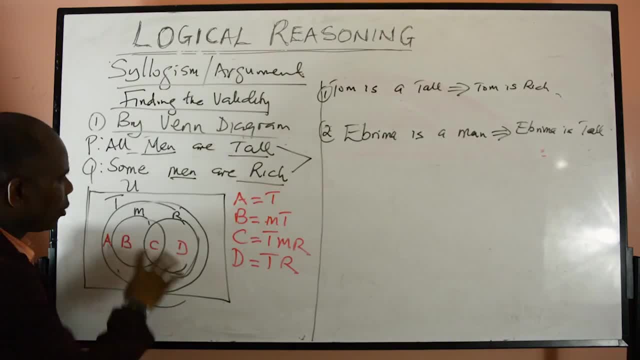 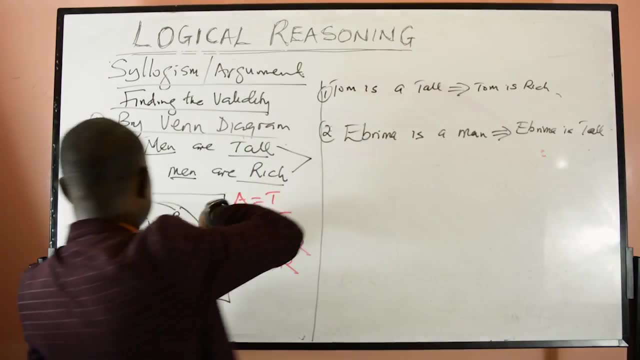 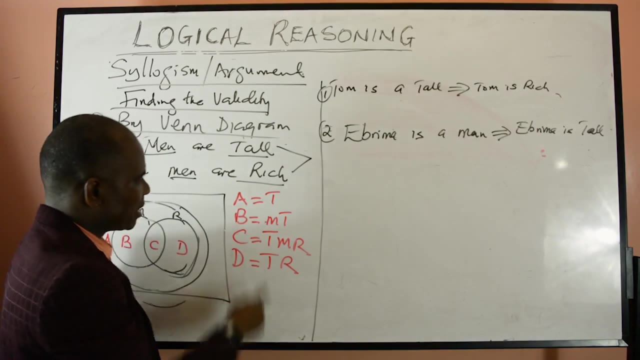 have tall, but this guy is. we have looked through the rooms. now, if we now conclude c- tom is a, tom is tall- it means tom is inside a tall circle. it means that it implies that tom is rich. so that statement becomes an invalid statement because inside the tall circle there is a room that do. 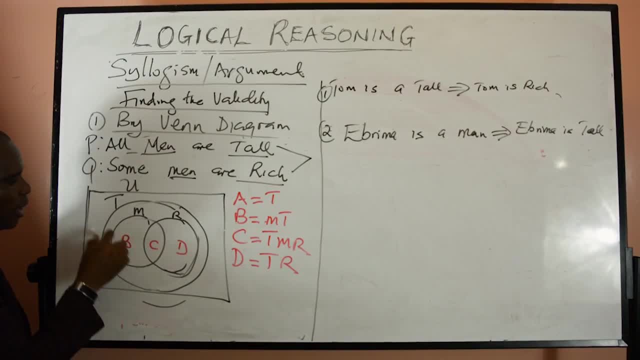 not have reach. there is a portion on this tall circle that do not have the reach, that do not have reach there. so if you check it there, you can see that this portion here do not have the rich circle here, recycle does not reach here. which circle does not reach here? so it could be that 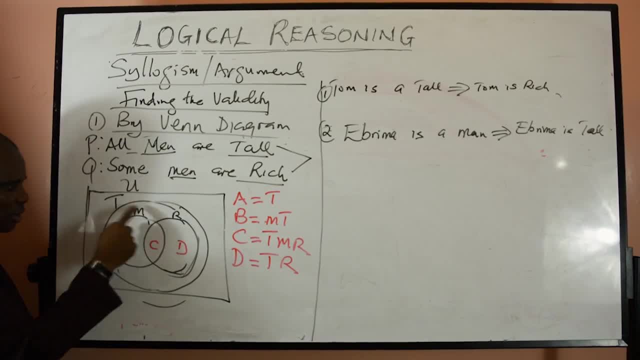 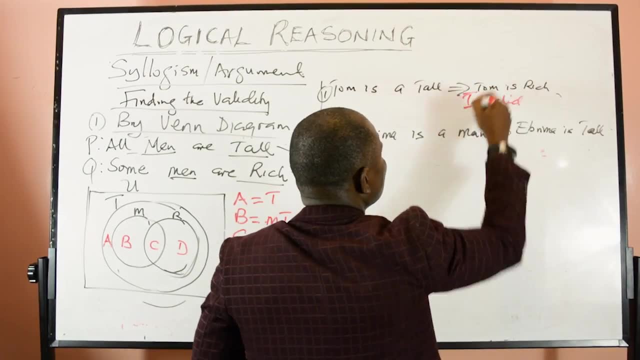 stone can be inside b and tom can be inside a, so it makes that statement invalid. that is an invalid statement, so i call it invalid statement. so watch out when, once the conclusion is not supported there, then you make it an invalid. so let's look at a. 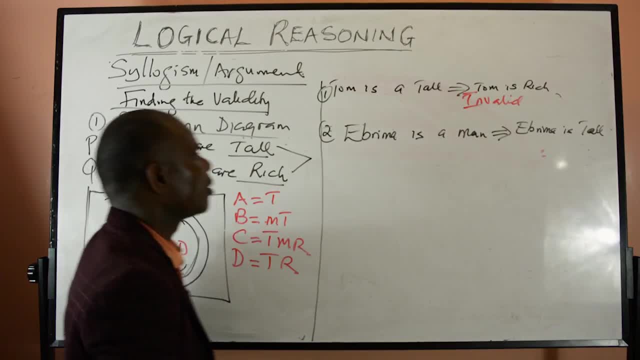 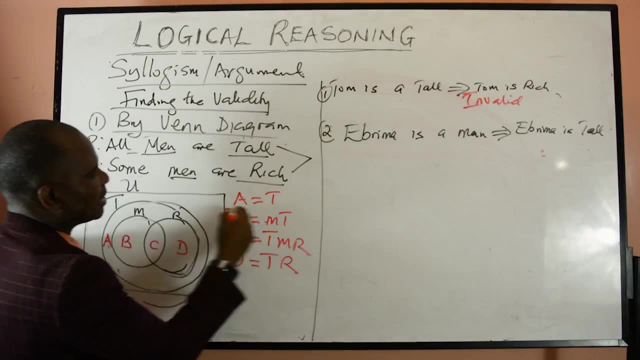 problem. well, the answer be: who is significant? then the answer be: UJ means when you are in a bad seat infью room, you are in a very bad place. at some point you are in a dopity zone, in a very bad situation. this first one is a good plan. so the question is: can we say these are our? 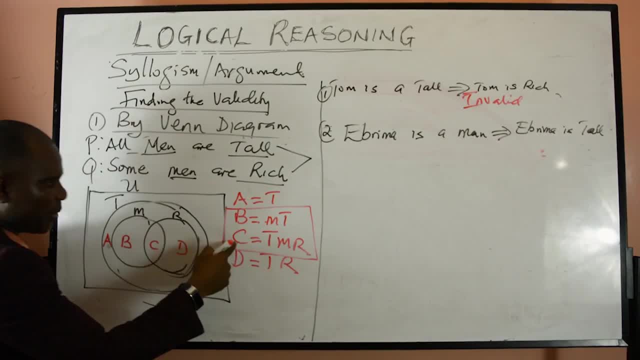 understanding inside this, then you call it a talk about uj. let's call them tactical if it is because we have to look in terms of where we live. let me put it in my own: so inside our, in our upfront problem, we have to look to the King around here to see if there is a problem with that, and let's Floyd. what type of problem do we have? let's look at the policeいますeli so we can see one talking about a problem with a person already, but we can also go through the background. p is a five- OVER, bumperخت means so we are planning a. 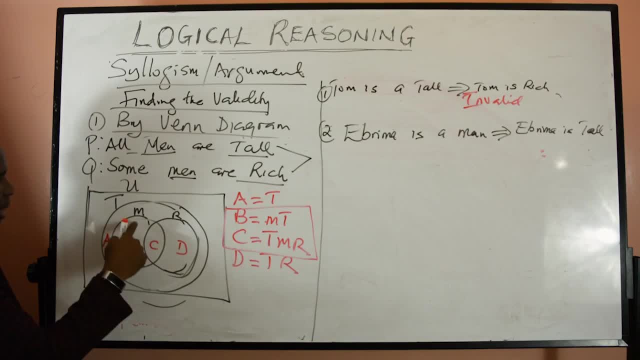 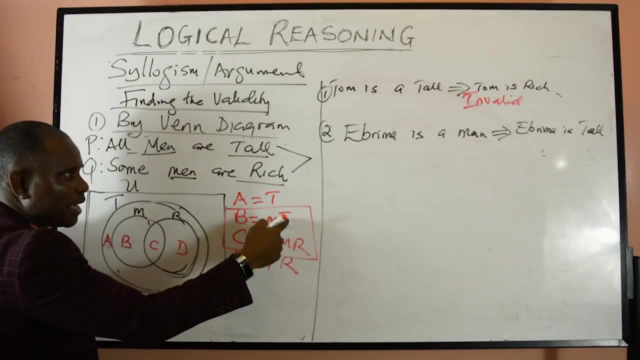 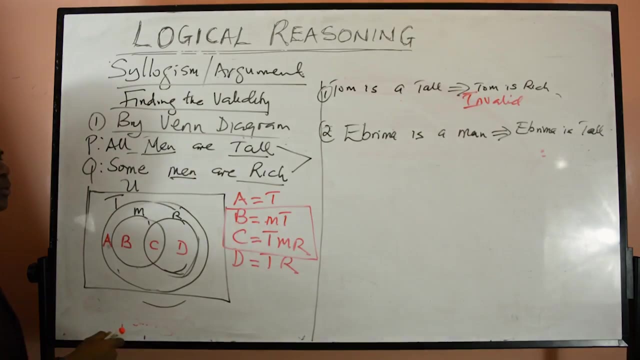 of the rooms and the room. the room that contains the main, the main room, contains two letters, main circle contains two letters, B and Z, and in that B room there is a tall person there. in the C room there's also a tall person there. so either rooms, when enter there, when I knock that room, I must have a tall person. 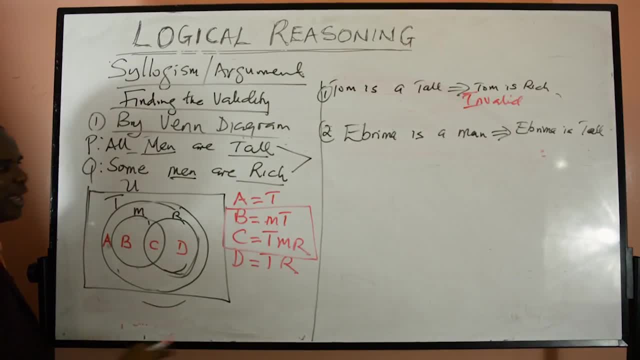 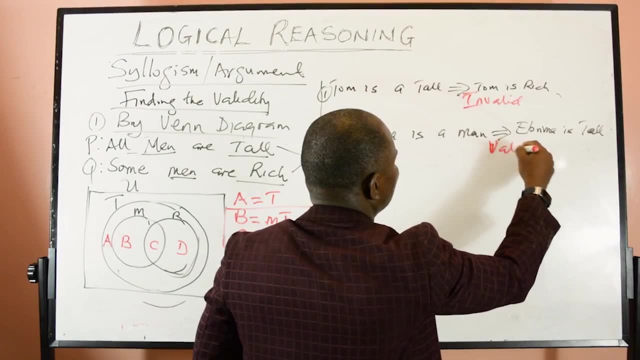 there. if a Bremer is inside this room will be classified as a tall guy. if a Bremer is inside this room, he'll be classified also as a tall guy, so he makes this statement valid. this statement is valid. so have one invalid and a valid statement. so now i'm. 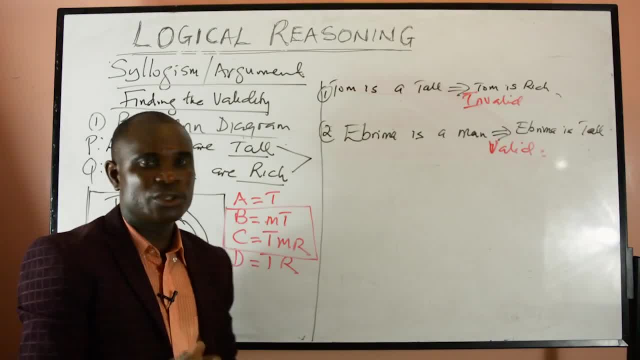 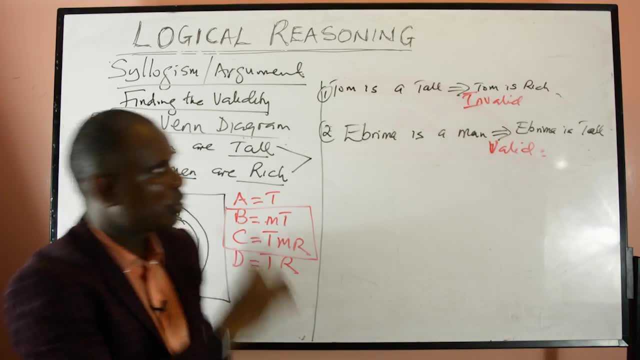 going to use this technique to solve the worst questions, so now keep watching and follow me up as you move with the questions now, with respect to your exam. so what out for the interpretation of my own method of solving this. you can have another form of solving it, but i just want to. 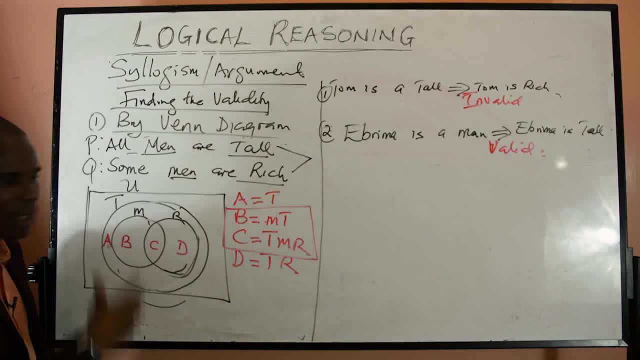 produce. i don't want to give you a very simplified way of solving these logical questions here. first you must establish the venn diagram. if you are supposed to find a validity based upon the venn diagram, then you must know the use of the word all, some and a few and none. you must be able to 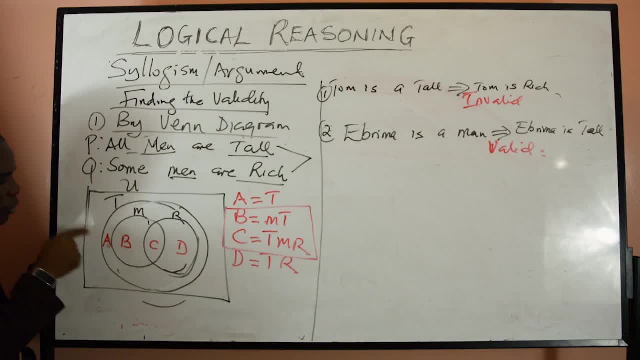 identify all of that when, once you are able to draw the venn, then you try to now label the venn, the component, the part of the venn diagram, with letters. you can use numbers there, i just use letters to make it simplified for you. so now you can use the letters and define which type. 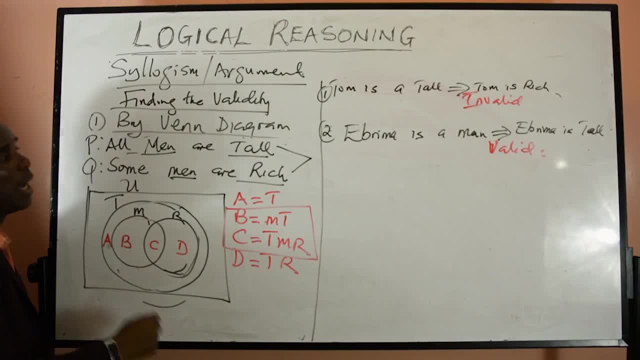 of human beings and in inside each of the rooms there- and you now look at this- the questions that are given. if the questions deviate from what is given to you, then you know what to put. you can put an invalid statement or valid, as the case may be, so. 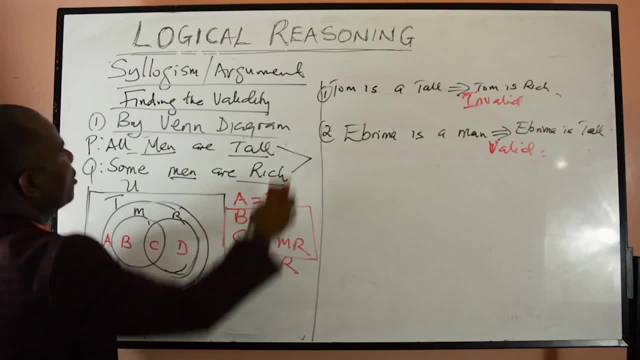 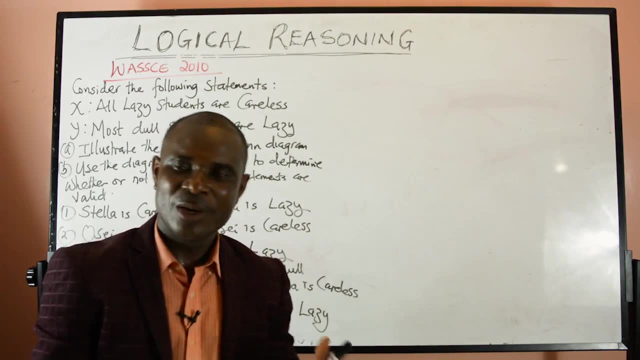 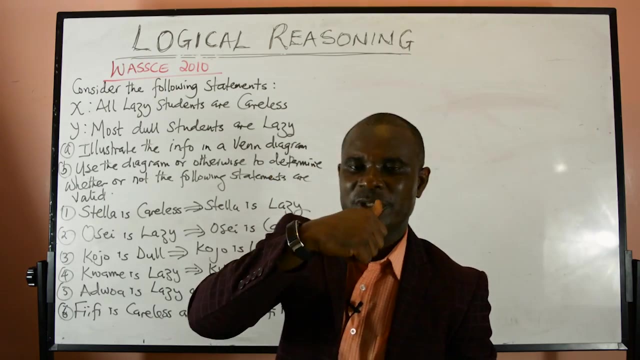 let's now use it to solve our worst questions. yeah, so now we move. all right, welcome back guys. we are still on this logic and reasoning and remember where we came from. we were able to establish the validity of a statement. we are trying to solve the validity of a statement based upon. 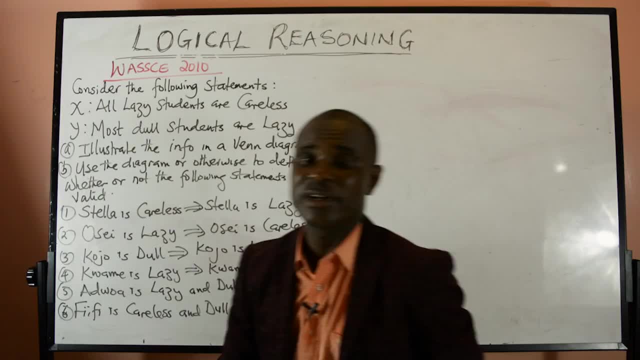 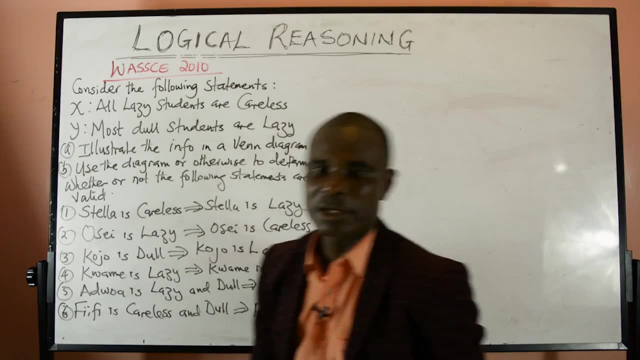 the venn diagram approach and i told you that that's one way we can find a validity. let's look at your uh exam questions. now is the west africa senior school certificate examination. that is like war, so it is 2010.. so let's look at it. 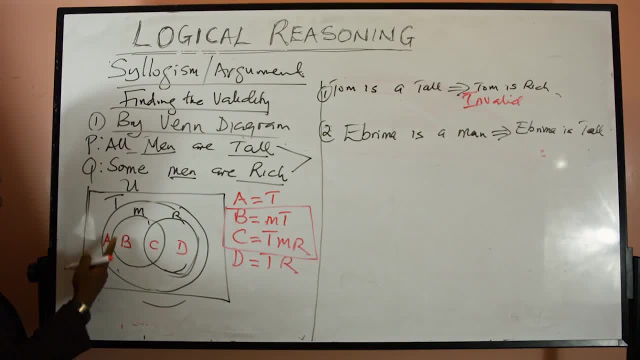 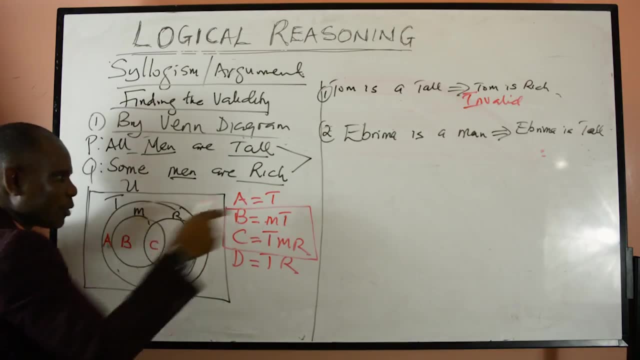 main. the main room contains two letters, men sako contains two letters, B and C, and adapter room. there is a tall person in there and they see room. there's also a tall person there, so either rooms to enter there. when i knock down room i must have a tall person there if ibrahima is inside this. 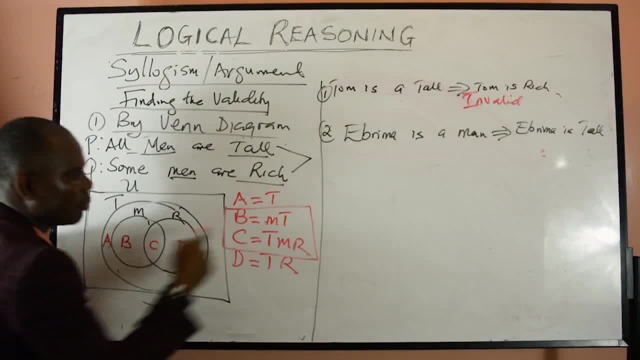 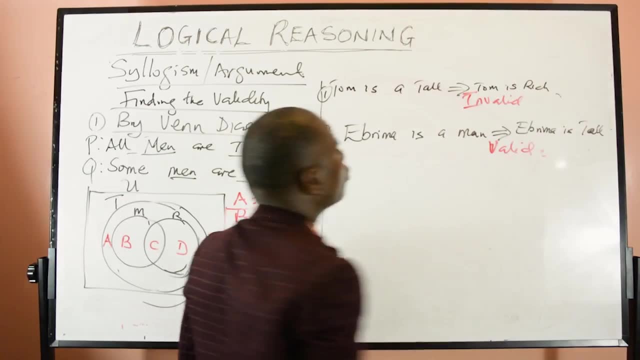 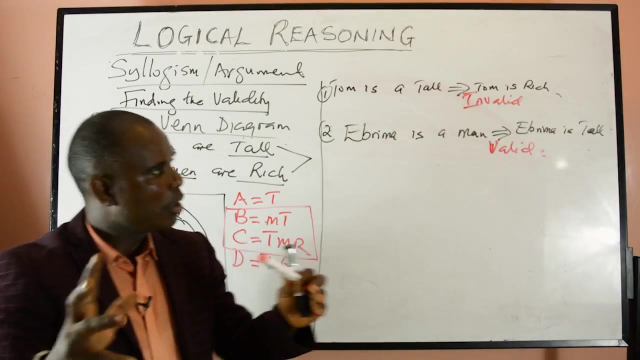 room, he will be classified as a tall guy. if ibrahima is inside this room, he will be classified also as a tall guy. so it makes this statement valid. this statement is valid. so have one invalid and a valid statement. so now i'm going to use this technique to solve the worst questions. so now, 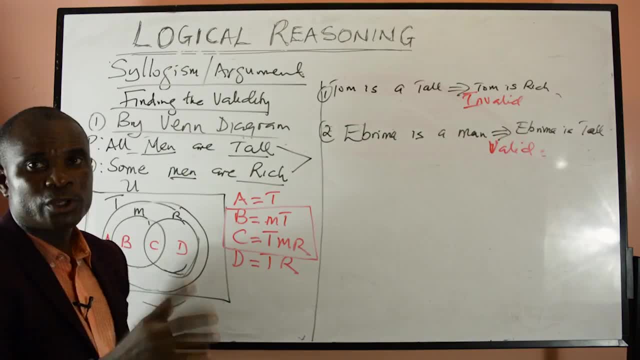 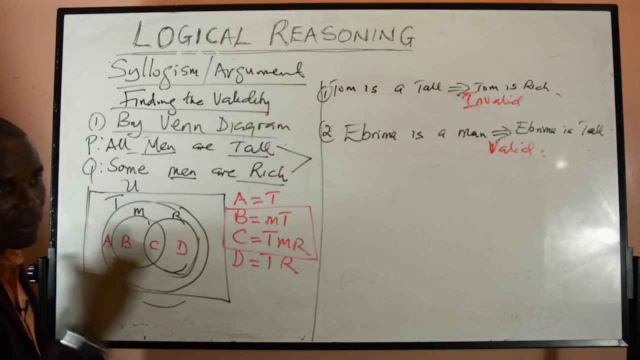 keep watching and follow me up as you move with the questions now with respect to your exam. so what out for the interpretation of my own method of solving this. you can have another form of solving it, but i just want to produce. i don't want to give you a very simplified way of solving these. 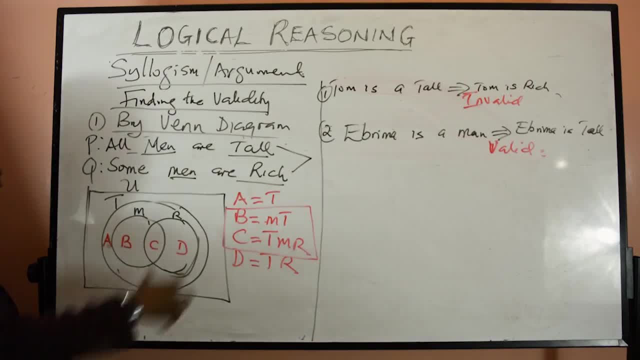 logical questions here. first, you must establish the uh venn diagram. if you are supposed to find a validity based upon the venn diagram, then you must know the use of the word all some, and if you are known, you must be able to identify all of that when, once you are able to draw the 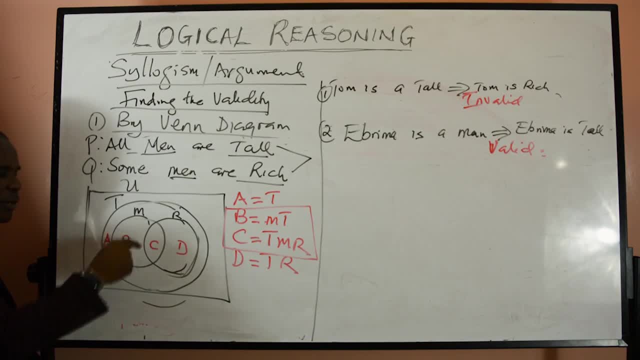 venn. then you try to now label the venn, the component, the part of the venn diagram, with letters. you can use numbers there, i just use letters to make it simplified for you. so now you can use the letters and define which type of human beings and in inside each of the. 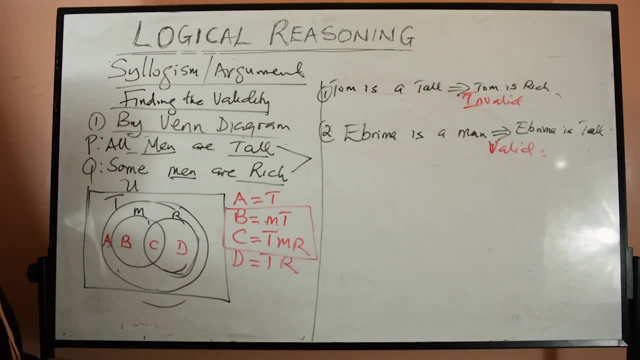 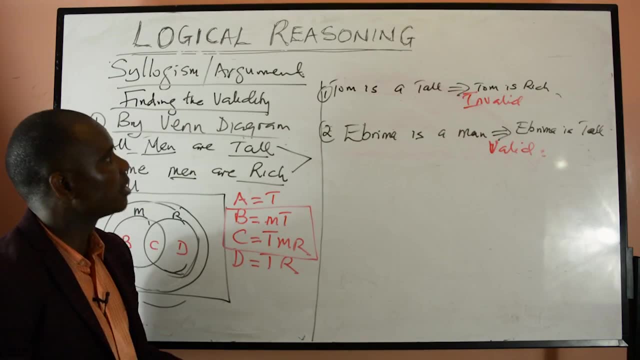 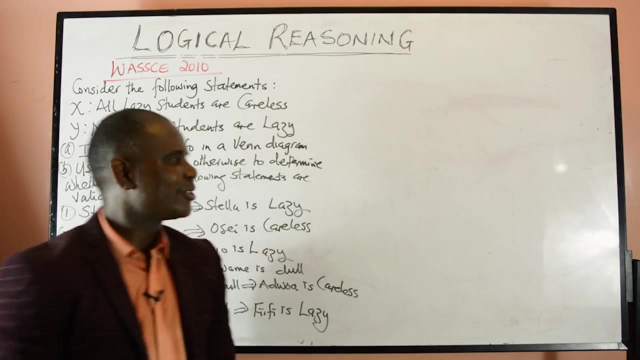 rooms there and you now look at this: the questions that are given. if the questions deviate from what is given to you, then you know what to put. you can put an invalid statement or valid, as the case may be, so let's now use it to solve our questions. yeah, so now we move. all right, welcome back, guys. we. 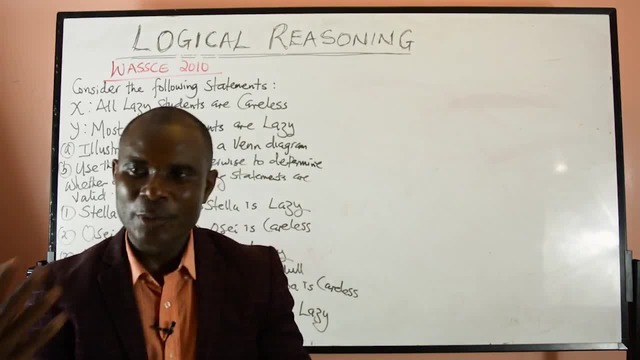 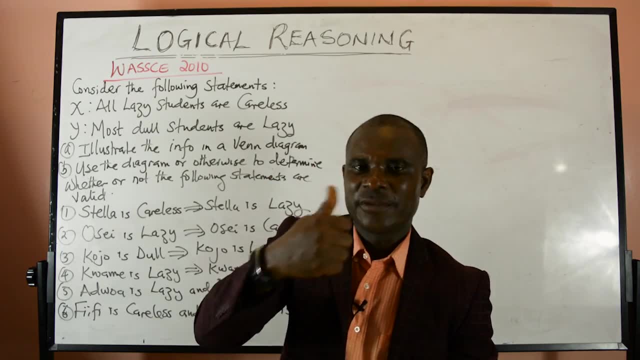 are still on the this logic and reasoning and remember where we came from, we are able to establish the validity of a statement. we are trying to solve the validity of a statement based upon the venn diagram approach and i told you that that's one way we can find a validity. let's look at your uh exam. 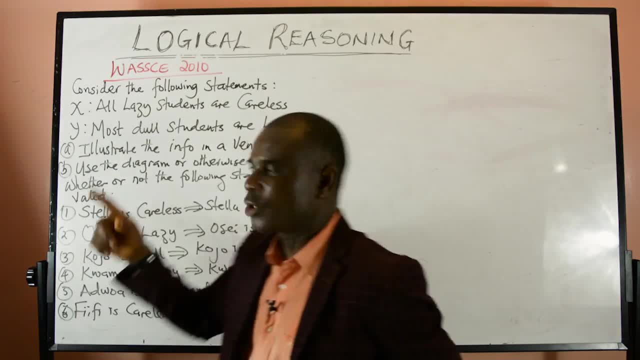 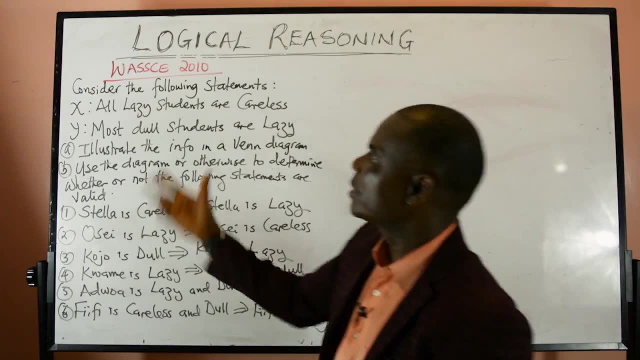 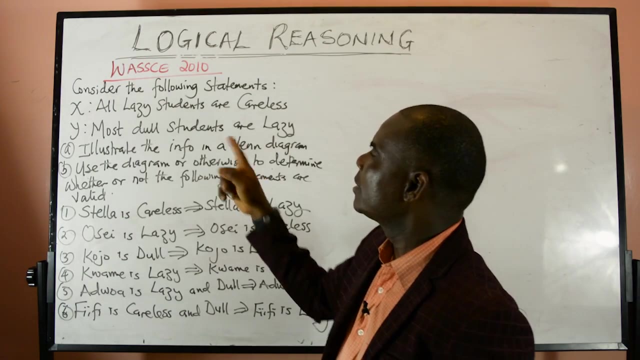 questions. now is the west africa senior school certificate examination. that is the war, so it is 2010.. so let's look at it. it is this. this question read say: consider the following statement: x is all students are careless. all lazy students are careless. now y says most those students are. 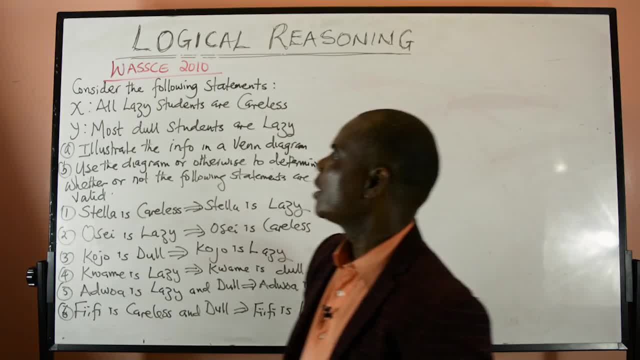 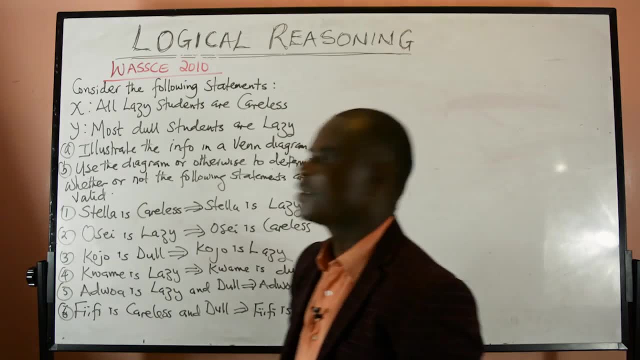 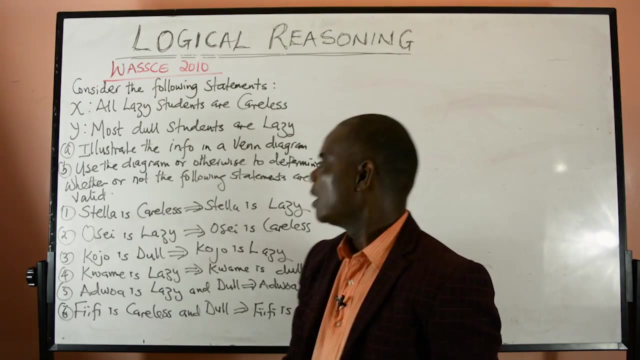 lazy and a question a says: illustrate the information in event diagram and b- use the diagram or otherwise to determine whether or not the following statements are valid. and first question is: stella is careless, implies this symbol means. implies implies stella is lazy. number two: oci is or oc is lazy. implies oc is lazy. 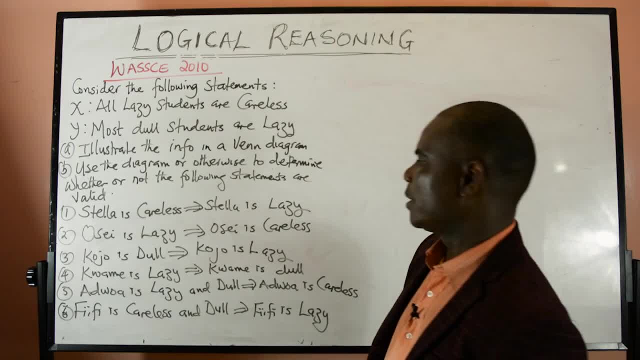 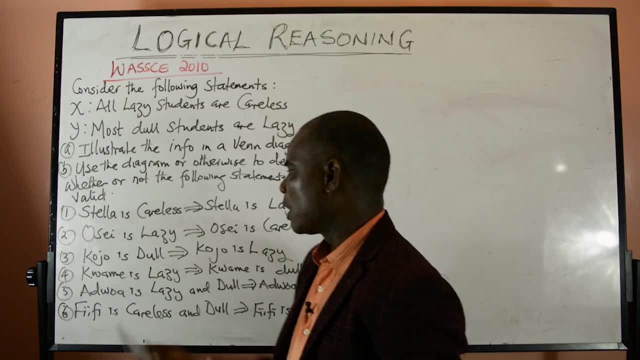 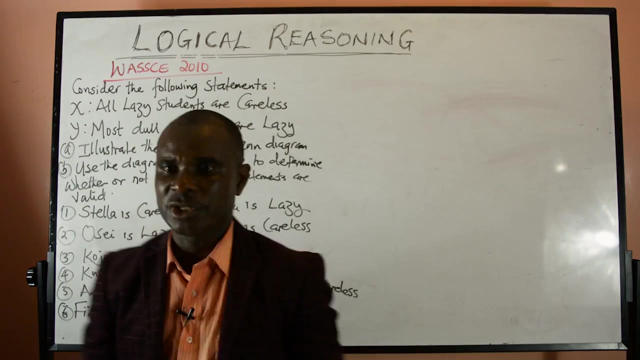 is careless. kujo is door implies kujo is lazy. kwame is lazy implies kwame is door. adwa is lazy and door implies otherwise careless. and finally we have fifi is careless and door implies fifi is lazy. now we've got a question. now i said um this: the my own approach to this is uh. 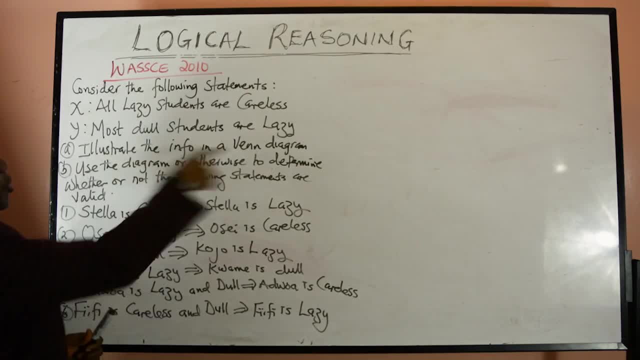 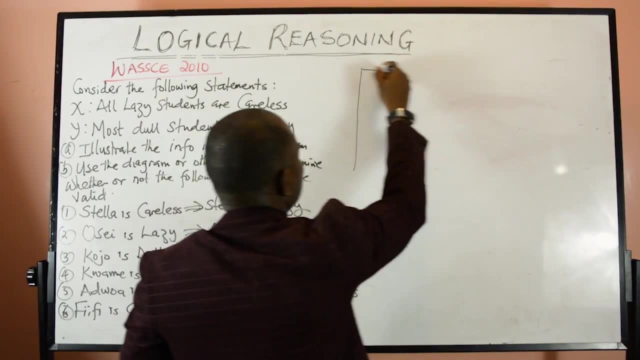 you first have to draw. the question has already told you to illustrate the information in the venn diagram. so the first thing is to draw the venn diagram. let's draw the venn diagram so we can use the venn diagram to find the validity of the statement. so we now have the venn diagram. i'll 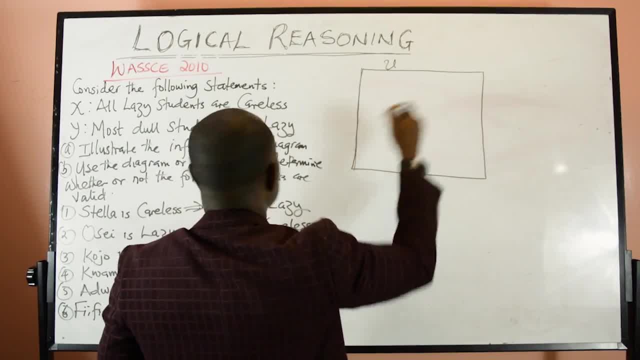 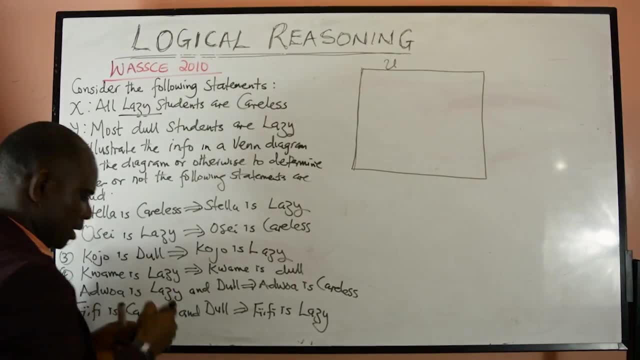 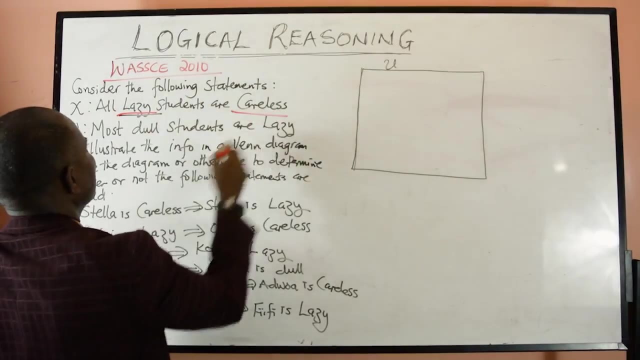 just draw that first for you here. so now we'll have the said. the first two, the first premise here, the first statement here will consider the following: let me give you another pen. yes, so i have. i identify the most important words in there: careless and all. so now the first. 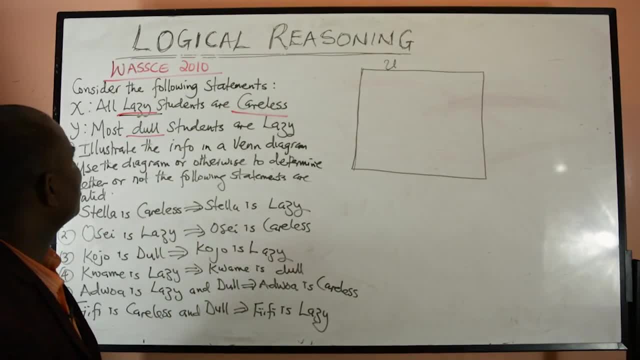 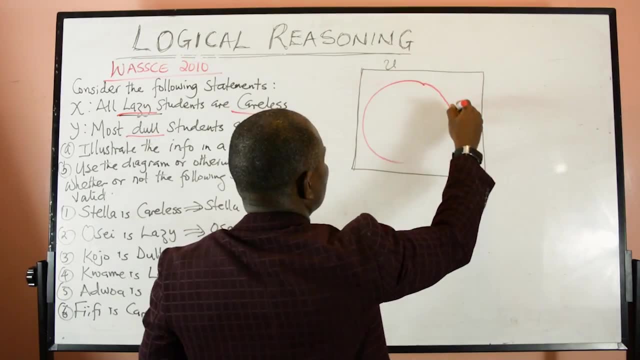 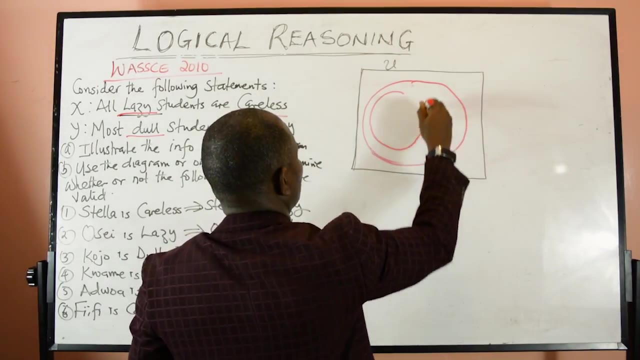 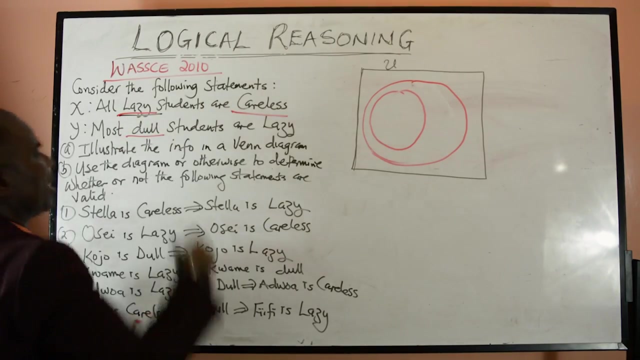 sentence always give us the two characters there. so let's look at all lazy students are careless. so i'm going to draw two things, two circles here, and you tell me which one is going to be embedded by the other. so we'll have. so, looking at this circle, we have all lazy students are careless. so since 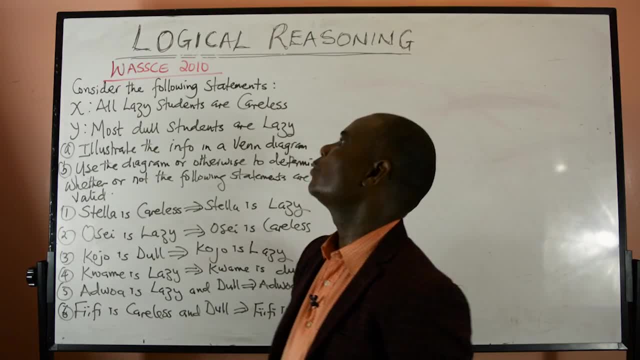 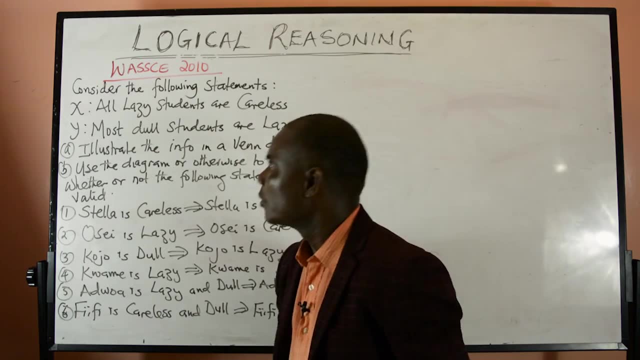 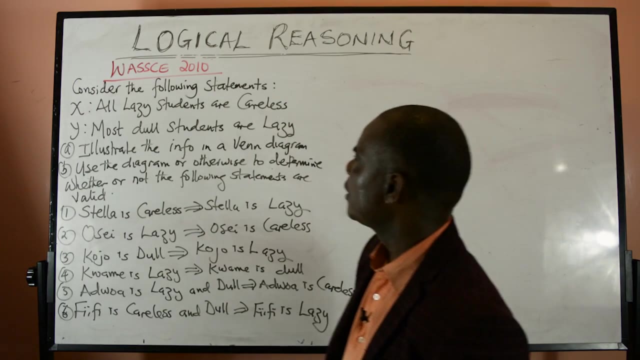 it is this. this question read: say: consider the following statement: x is all. statement: all students are careless, all lazy students are careless. now y says: most door students are lazy and a question. a says: illustrate the information in a venn diagram and b use the the diagram otherwise to determine whether or not the following: 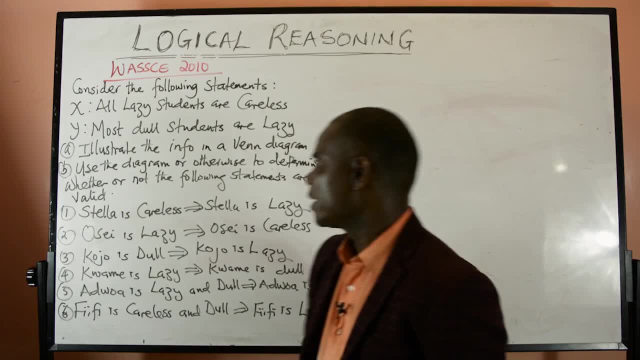 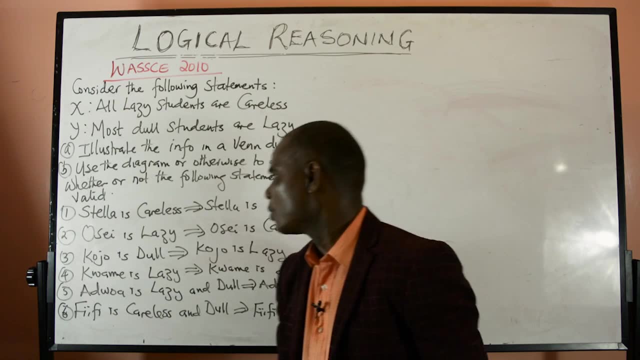 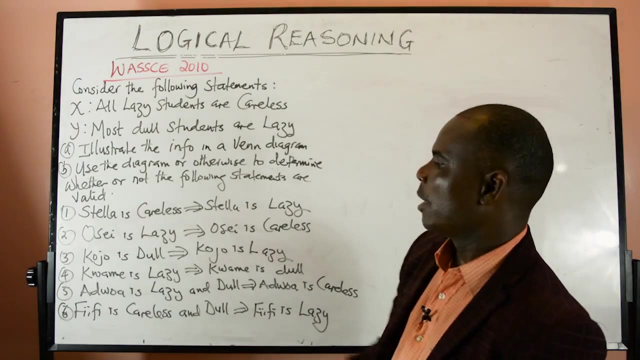 statements are valid. and first question is: stella is careless, implies this symbol means, implies, implies stella is lazy. number two: osai is or oc is lazy implies oc is careless. kujo is door, implies kujo is lazy. kwame is lazy implies kwame is door. adwa is lazy and door implies otherwise careless. 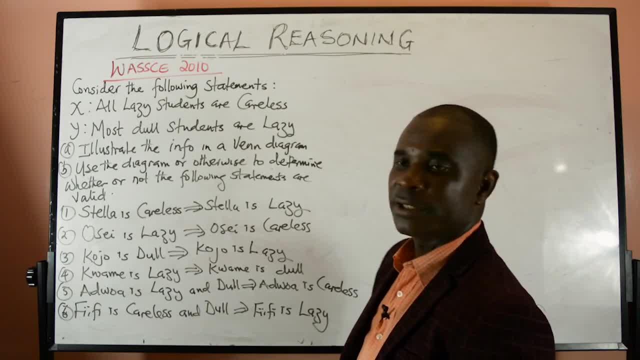 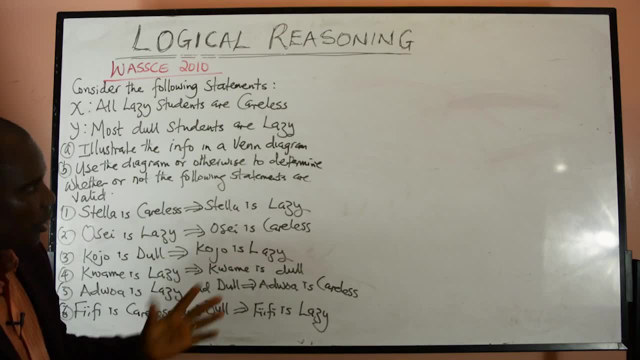 we have fifi is careless and door implies fifi is lazy. now we've got a question. now i said, um this, my own approach to this is: uh, you first have to draw. the question has already told you to illustrate the information in the venn diagram. so the first thing is to draw the venn diagram. 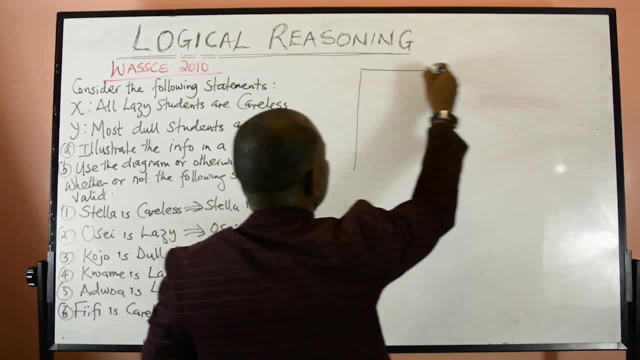 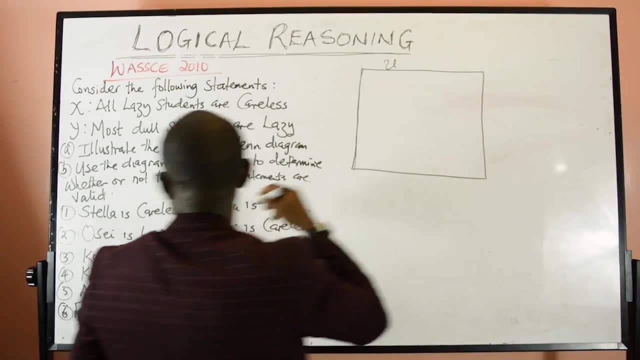 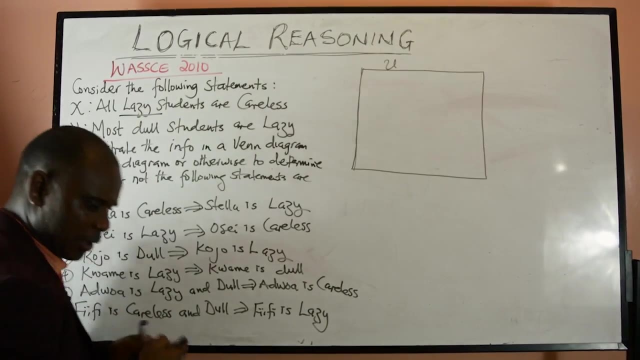 let's draw the venn diagram so we can use the venn diagram to find the validity of the statement. so we now have the venn diagram. i'll just draw that first for you here. so now we'll have the posted. the first sentence of the first sentence said the first two, the first premise here, the 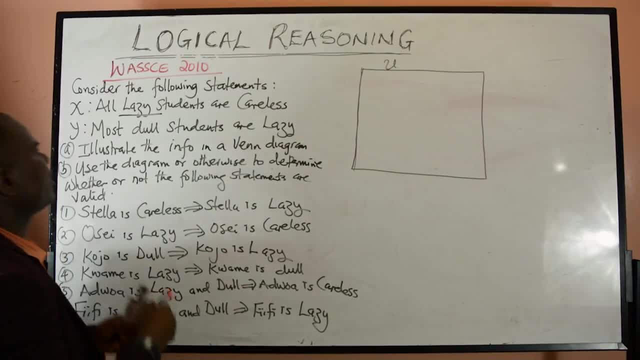 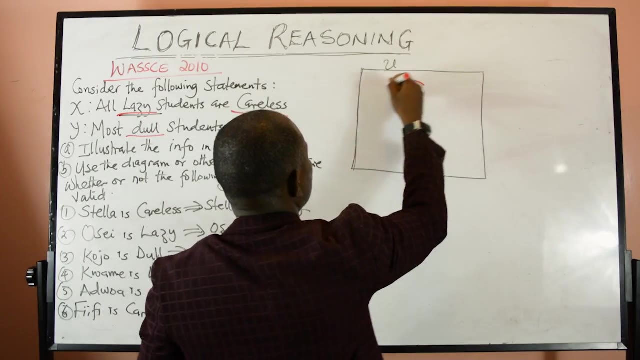 first statement here will consider the following: let me give you another pen. yes, so i have. i identify the most important words in there: careless and doll. so now the first sentence always give us the two characters there. so let's look at all this. students, atilles, i'm gonna draw. two things, two circles here, and you tell me which one is going to be embedded by the other. so we'll have the, the first sentence: zero, zero, point one, zero point one, zero, numbers 0. and then let's look at course, when you draw this first one, earth, and that's one pair of numbers, eight, five, one, eight. 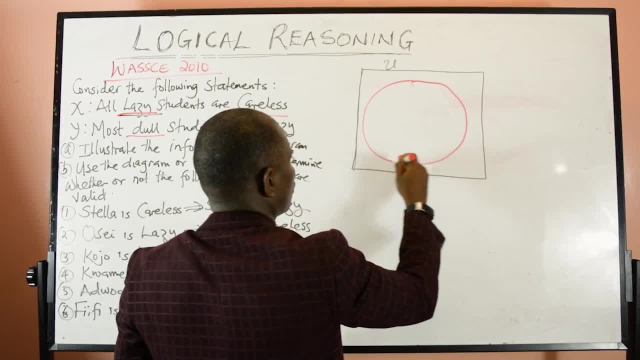 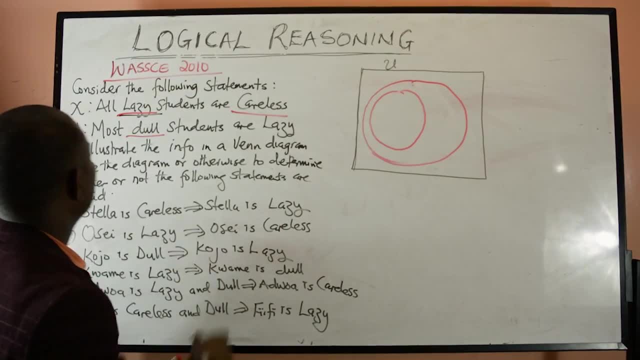 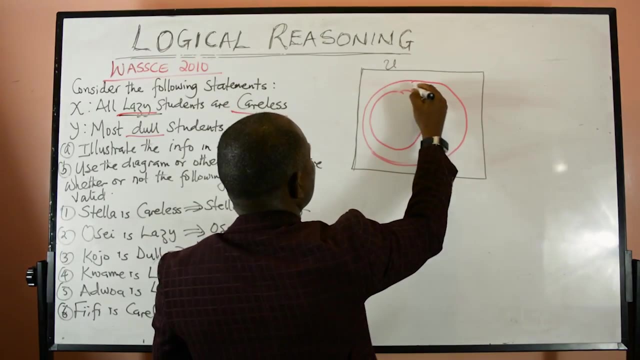 there the first key: ready consideration. and if there's nothing like that, i hold back. let's see how i've. so we have. so, looking at this circle, we have: all lazy students are careless. so since we say all lazy students are careless, then the lazy circle must be. 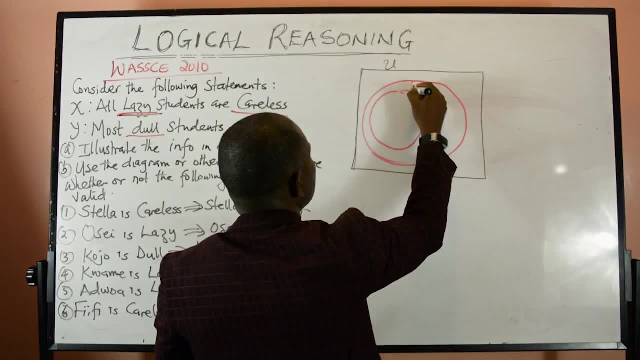 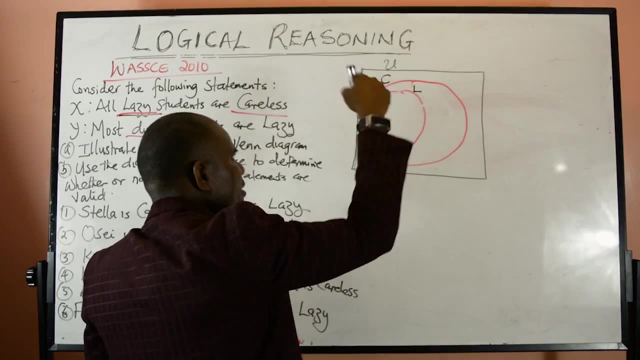 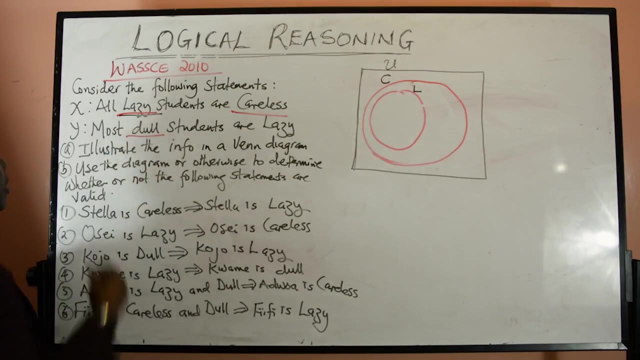 we say: all lazy students are careless, then the lazy circle will be. the first sentence must be inside the careless circle all lazy students are careless, or the lazy circle is swallowed by the careless circle, that's it. so now we come back here most door. remember i said some? 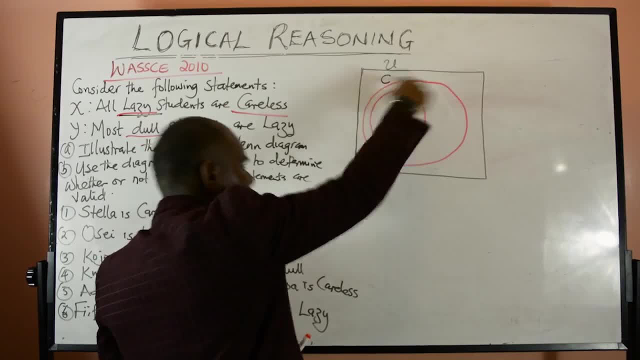 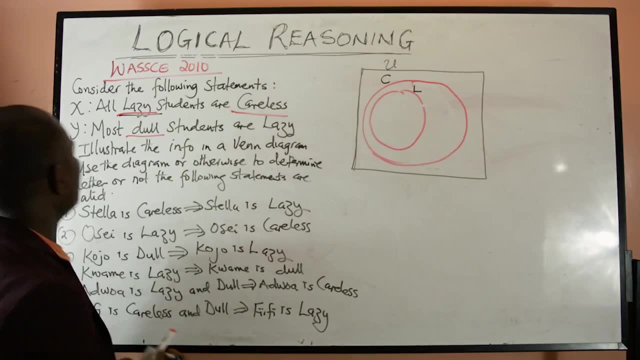 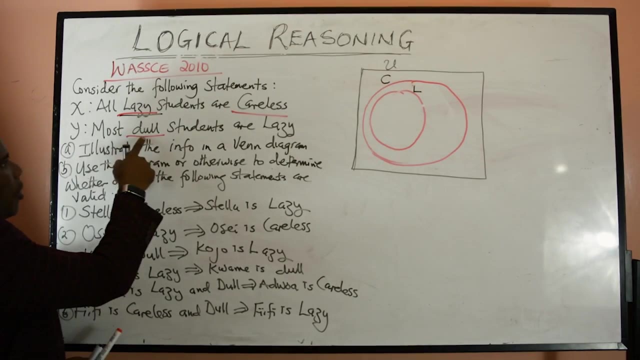 inside the careless circle. all lazy students are careless or the lazy circle is swallowed by the careless circle. that's it. so now we come back here: most door- remember I said so- if you many, most. these are all intercession. so most door students, most of students, are lazy. so there's gonna be an intercession between 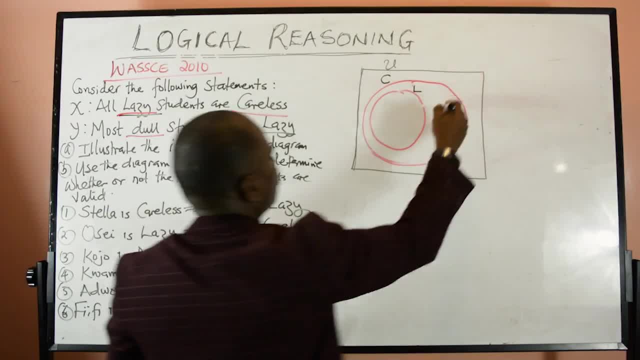 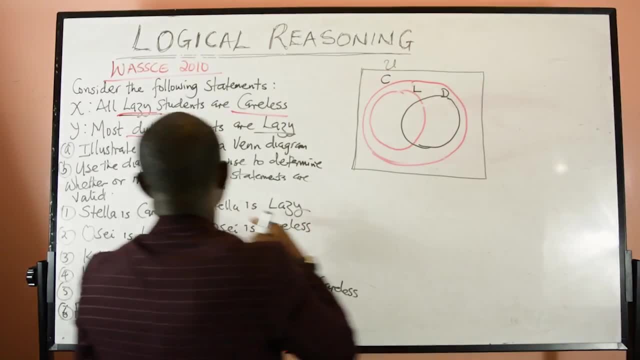 door and lazy, so it's going to be intercession here. so I just draw it intercession and nice. an intercession between door and lazy. that's what share. door students are lazy. most doors students are lazy, not all of them, so it's an intercession. 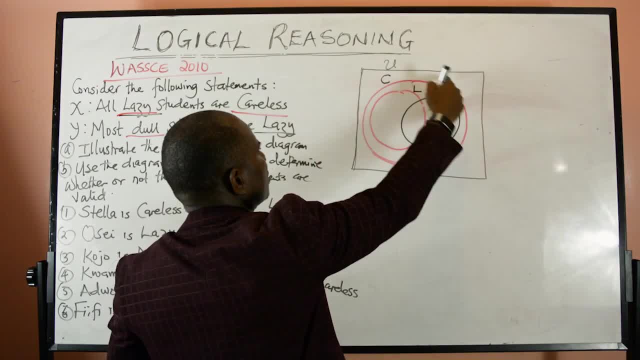 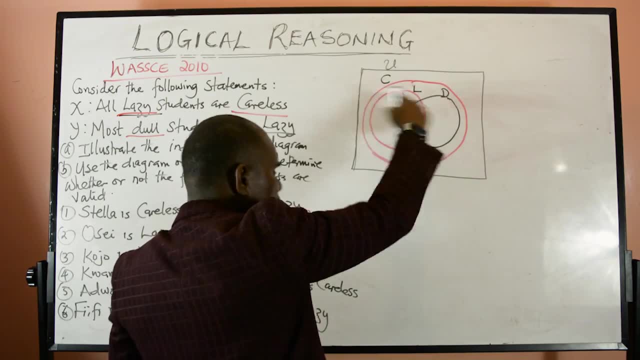 i just define those characters for you. so we have circles, that is the biggest circle, that is careless, and we say: all the lazy students are careless. so all the lazy students are found inside the careless circle and we have some of the door students are also found inside the lazy 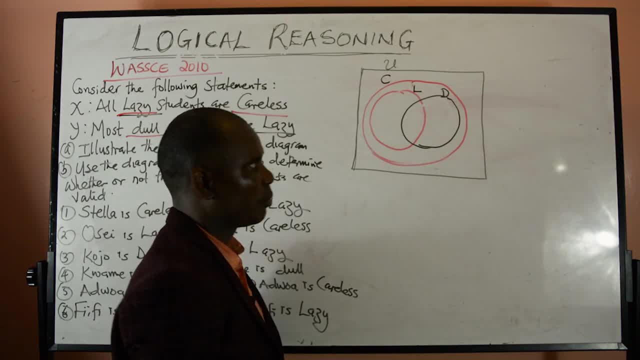 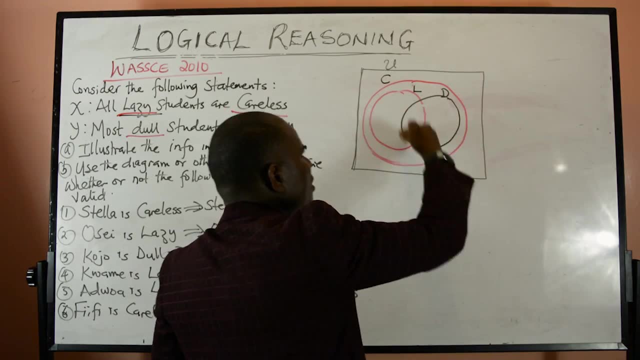 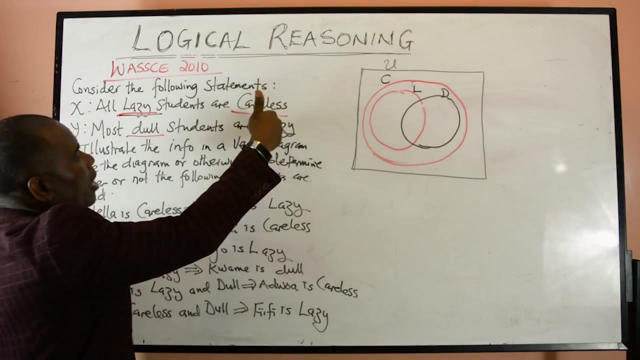 circle, but not all the door students are found inside the lazy circle. but we have done some according to my diagram here and i've done an assumption. i've assumed that all the door students are found inside the careless circle, meaning all the door students are careless students. that is my assumption. there is no indication here. there is no link between careless. 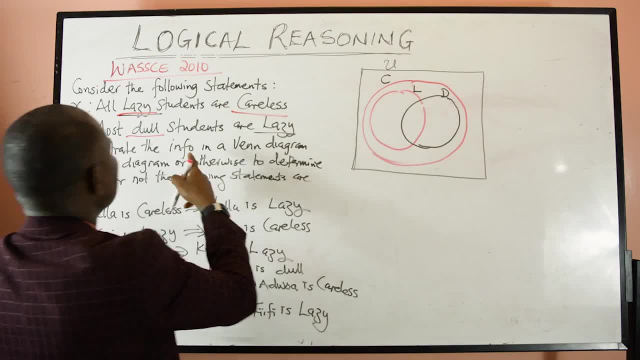 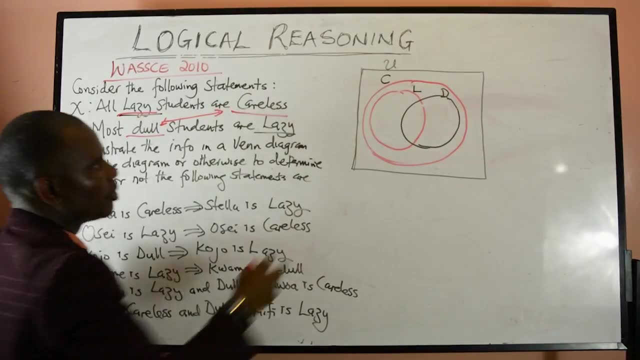 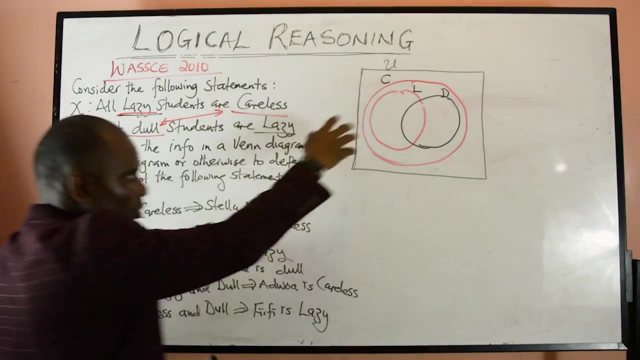 and lazy, careless and doll. there is a link between this: lazy link careless, lazy link doll, but there is no link between lazy and doll. so we have assumed that all the door students are careless. there is no, no link between doll and careless, but we are going to assume here that there is a. there is now. 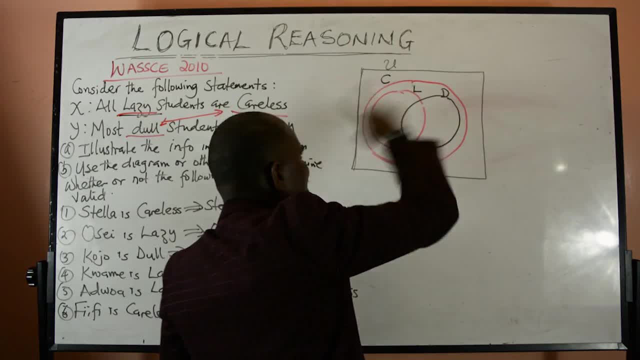 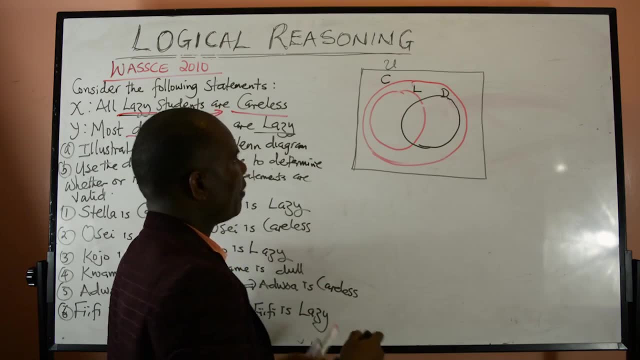 a link between them. that is all the door. students are found inside the killer circle. it's based upon your diagram that you'll be marked, so let's look at this now. so we have three compartments here. we have more than three events, so let me draw this properly. 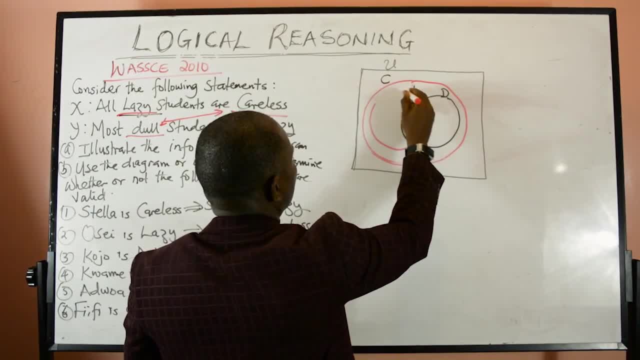 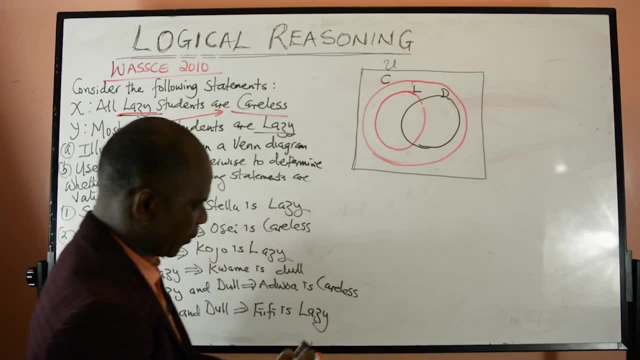 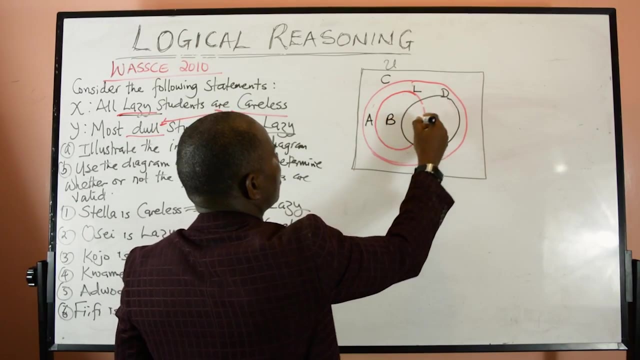 so you see, so i got a space from here. here i'll make the circle a little bit smaller here, so i have that. yes, so look at the. so first i said according to my one approach, i said you can first find liberally rooms in that over, so have four rooms in those overs there. 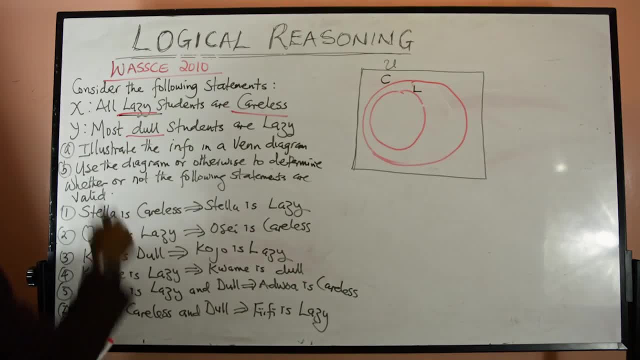 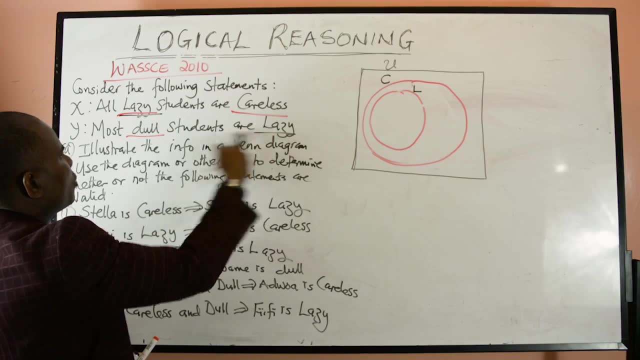 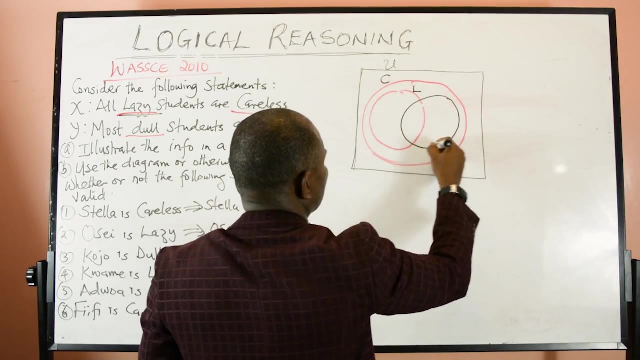 a few, many, most these are all intercession. so most dull students, most dull students, are lazy, so there's going to be an intercession between door and lazy. so it's going to be intercession here. so i just draw it intercession and it's an intercession between doll and lazy. that's what's here. doll students are lazy. 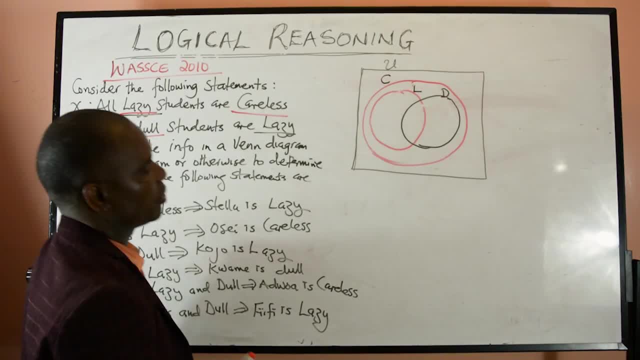 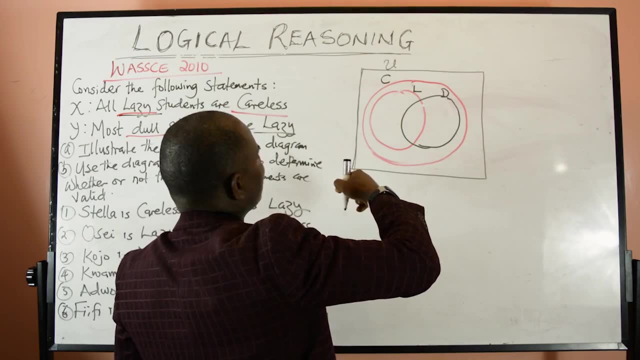 most dull students are lazy, not all of them. so it's an intercession. i just define those characters for you. so we have circles. that is the biggest circle, that is is careless, and we say: all the lazy students are careless. so all the lazy students are found inside the careless circle. 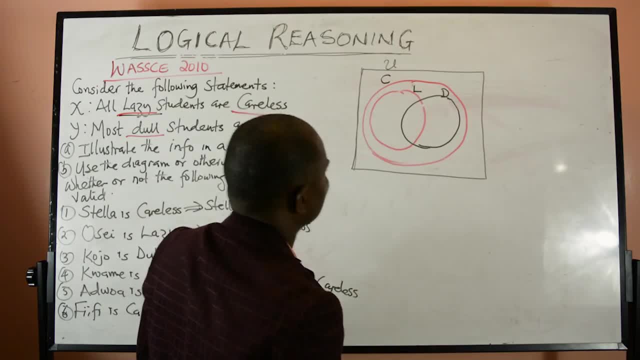 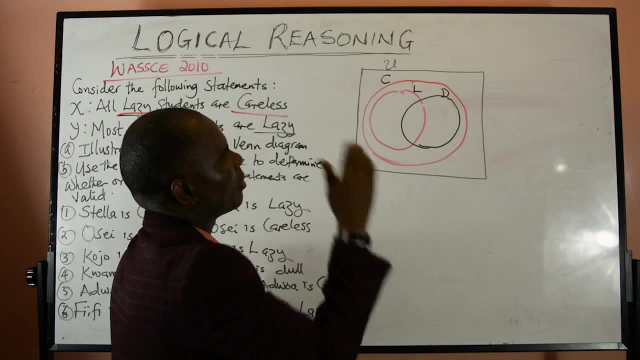 and we have. some of the dull students are also found inside the lazy circle, but not all the dull students are found inside the lazy circle. but we have done some according to my diagram here and i've done an assumption. i've assumed that all the dull students are found inside the careless. 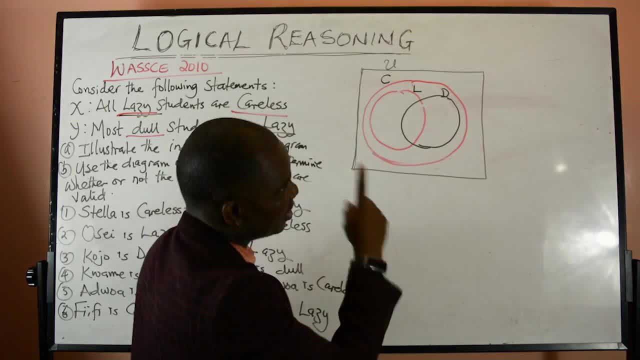 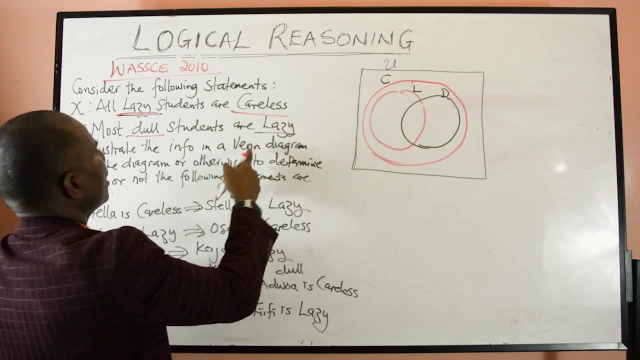 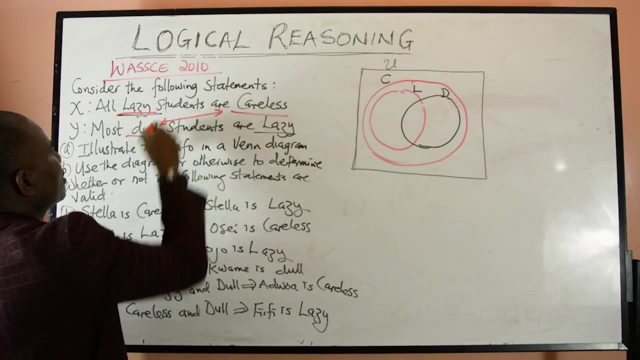 circle, meaning all the dull students are careless students. that is my assumption. there is no indication here. there is no link between careless and lazy, careless and all. there is a link between this lazy link careless, lazy linked doll. but there is no link between lazy and doll, so we have assumed. 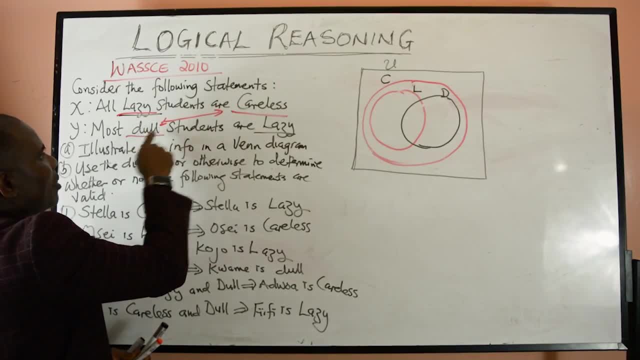 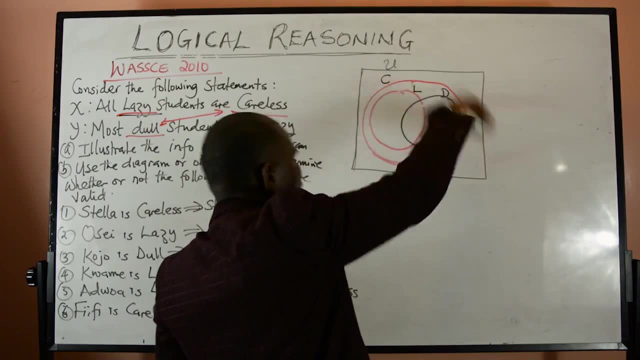 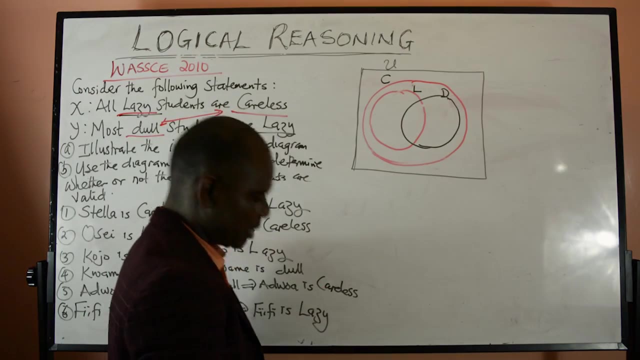 are careless. there is no, no link between door and careless, but we are going to assume here that they said there is now a link between them. that is all. the door students are found inside the killer circle. it's based upon your diagram that you be math, so let's look at this now. so we have three compartments here. we have 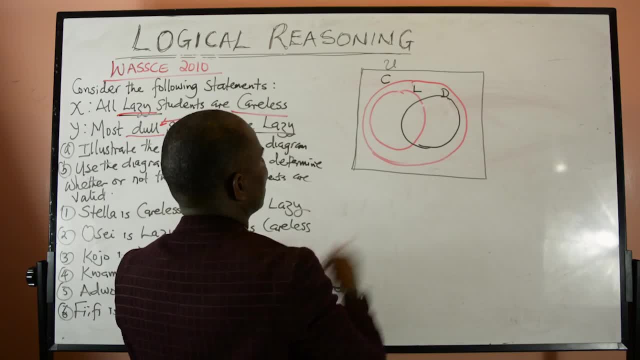 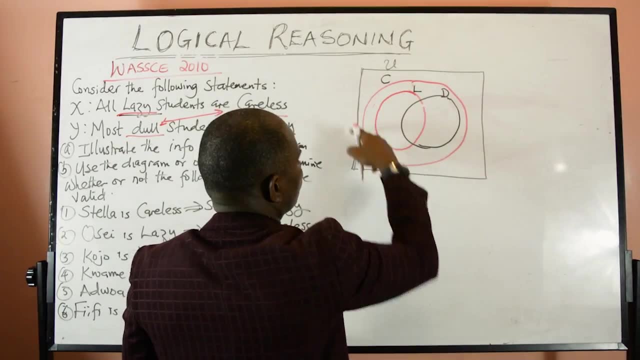 more than three events and let me draw this properly. so you see, so I got a space from here. here I'll make this up a little bit smaller. yes, so I have that. yes, so look at the. so first I said: according to my own approach, I said you: 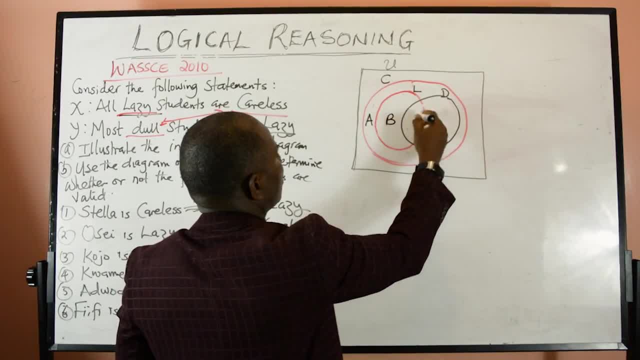 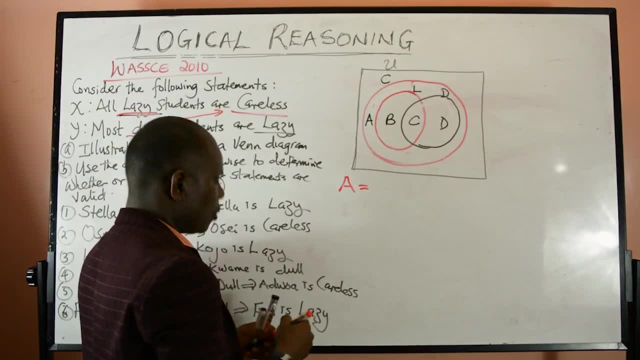 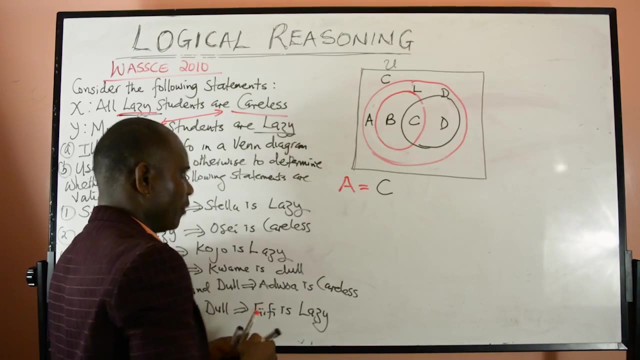 can first find, liberally, rooms in that over. so have four rooms in those overs there, so never leave at them. that is room a room. it contains which type of people is? it contains all the careless people, because he is found inside the killer circle and we have B, so let me just write all the letter C and D, so we 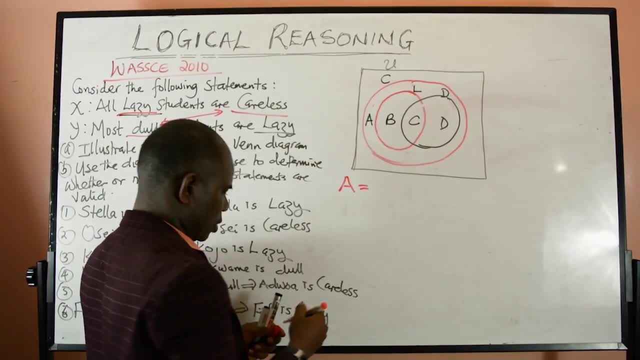 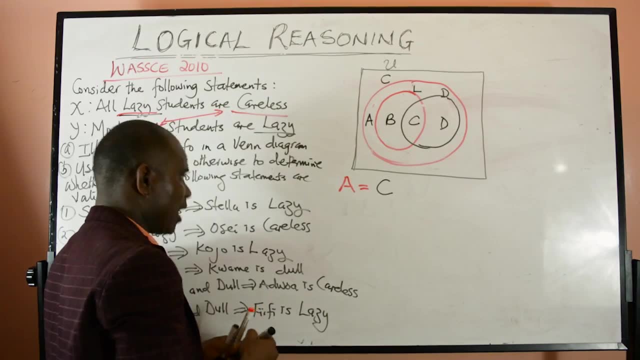 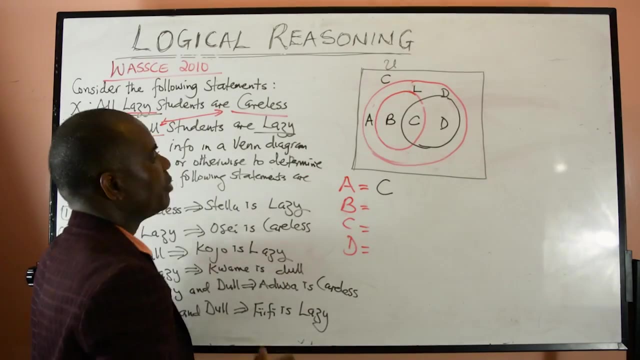 so let me leave them. that is room a room it contains. which type of people is? it contains all the careless people, because a is found inside a careless circle and we have b, so let me just write all the letter c and d so we'll be able to identify them. so now b is found inside two circles. it has. 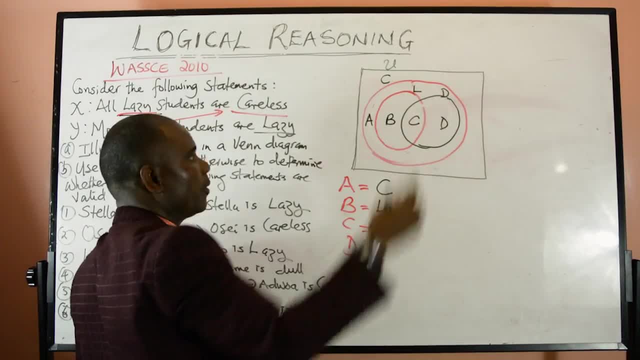 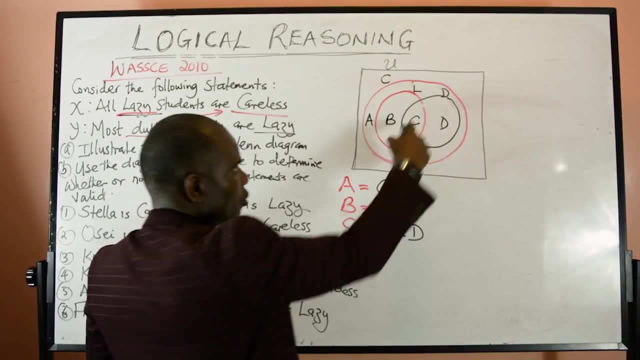 place and area. and third, there is also space. so e, c, c and d and d. they are the l circle and the c circle. c is found inside all three circle. it has the c circle, the l circle, the doll circle and d is found inside only two circles. a d letter d is found inside the two. 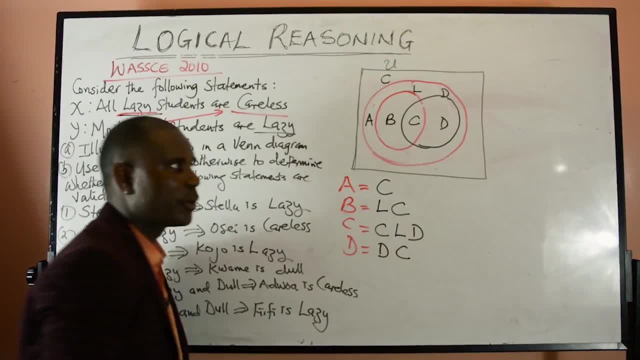 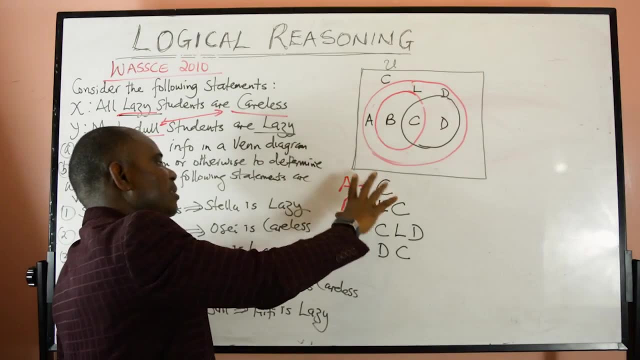 circles. it's found inside doll circle and careless circle. so we have already identified the kind of characters that are inside each of these circles. so now we we are looking at these assertions and look at the questions. i will try to see whether these statements are valid or not. so let's take 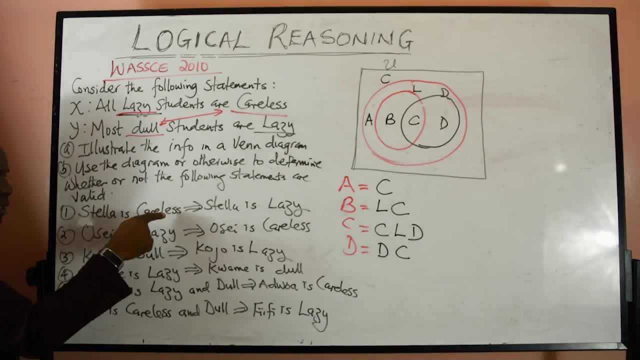 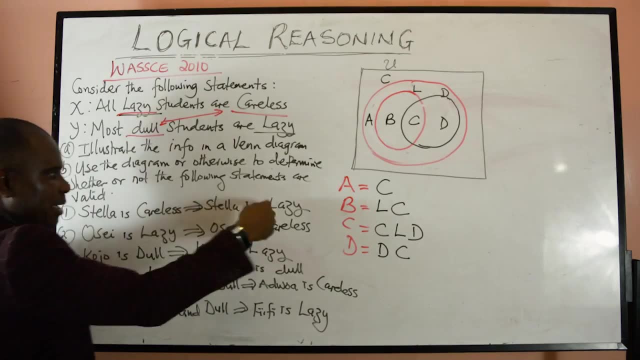 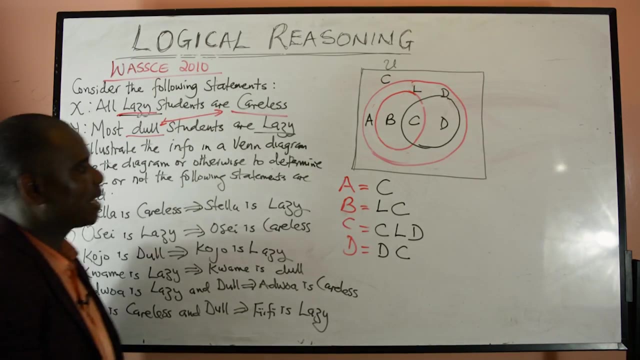 the first statement. it says stella is careless. it means stella is inside the careless circle. now let's watch. he says: therefore implies that stella is here, is lazy, so stella is careless. implies stella is lazy, so let's check out. now we look at for the careless circle, the careless 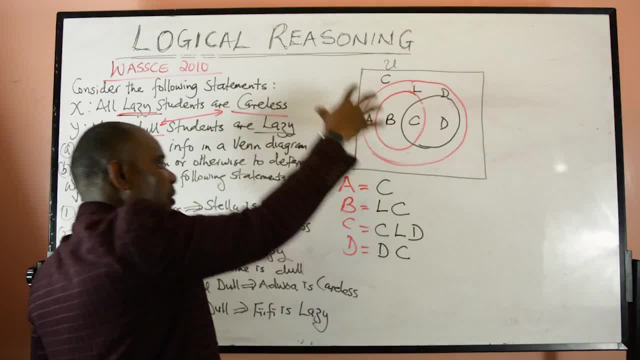 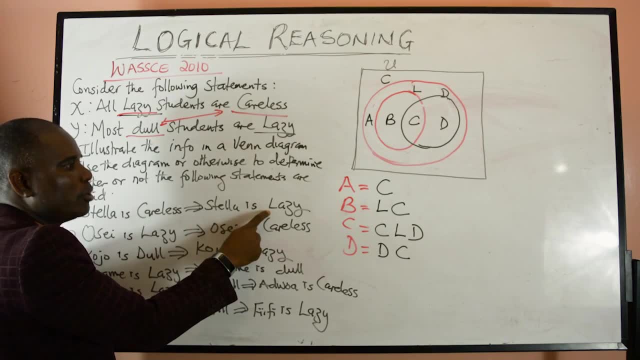 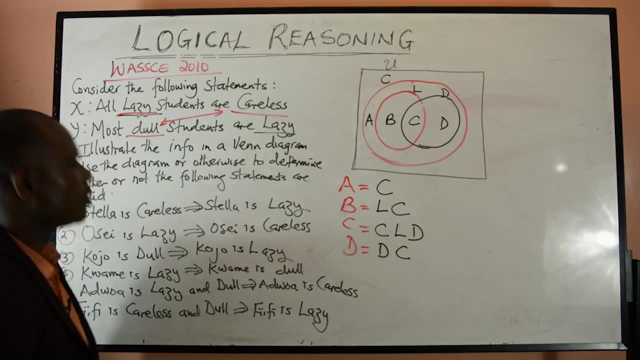 circle encompass all the letters, meaning it is involving all the letters. so if we can enter inside the letter every room here and we'll find l in all the rooms, then we can see this statement is valid. but if there is any room here that do not have l, it makes this statement invalid. 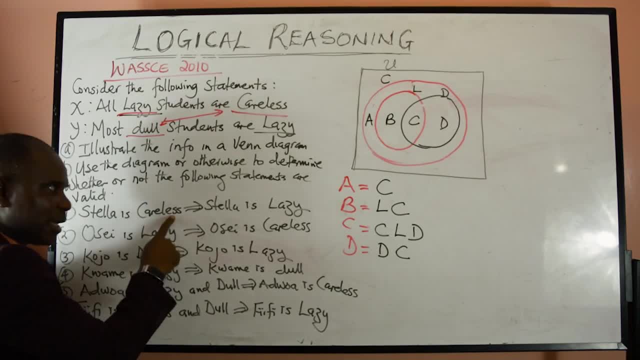 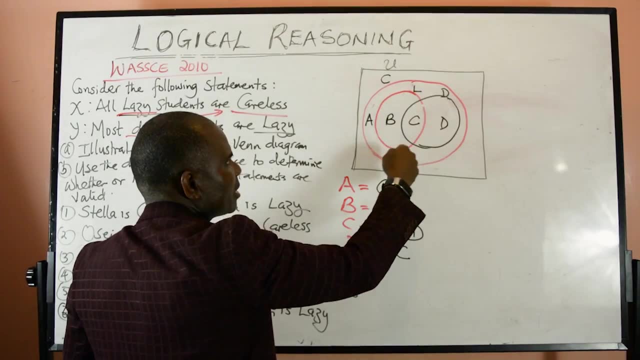 so let's check out now. we have got the careless circle and the careless circle involves all the letters, because all the letters are inside the secure circle. a is inside. careless circle b is inside. this is a careless circle c is a careless circle. d is a careless circle. now all the letters. 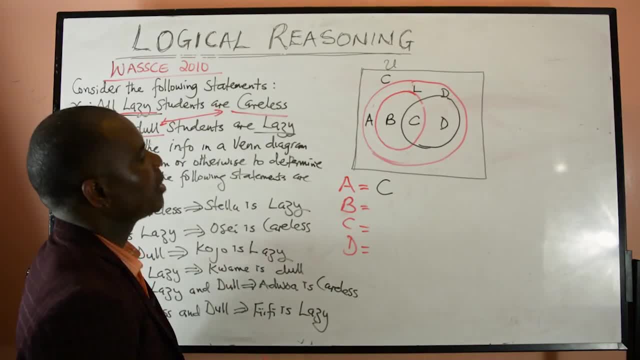 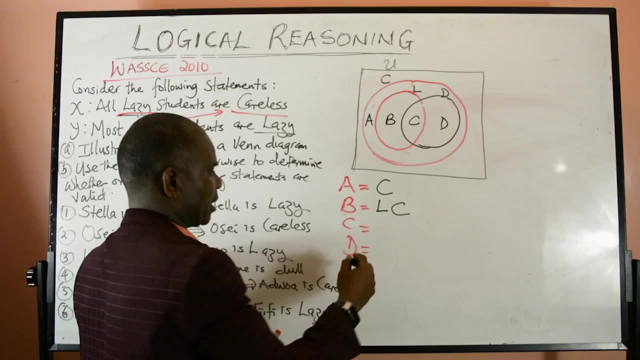 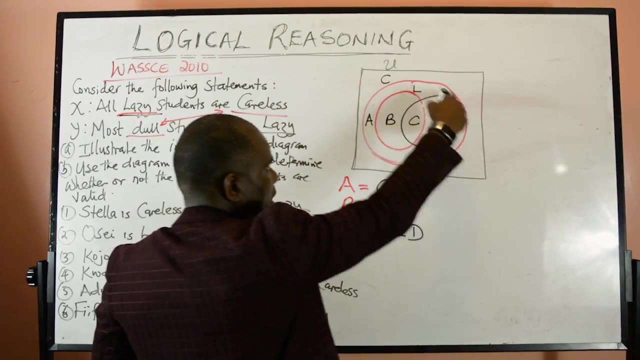 would identify them. so now, B is found inside two circles. it has the L circle and a C circle. C is found inside all three circle. it has the C circle, the L circle, the door circle and D is found. it's only two circles. a D letter D is found inside the two circles. 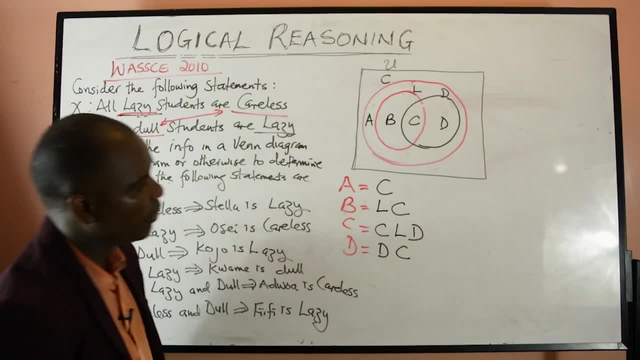 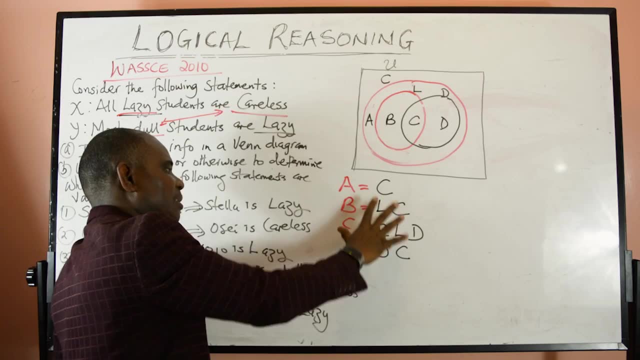 it's one inside door circle and killer circle. so we have already identified the kind of characters that are inside each of these circles. so now we we are looking at these assassins and look at the questions. I will try to see whether these statements are valid or not. so 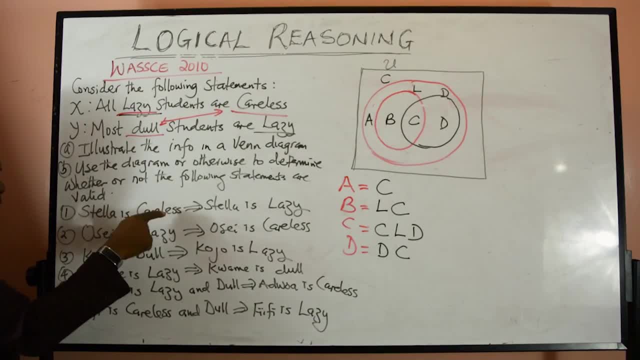 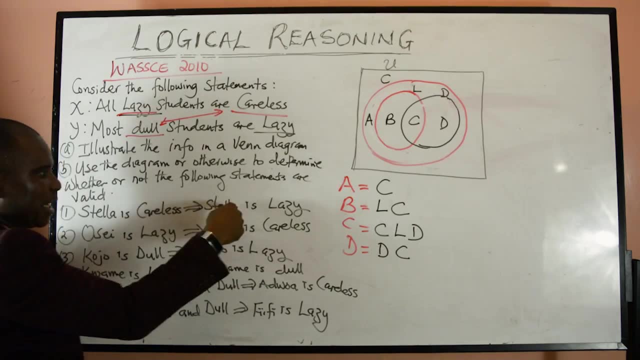 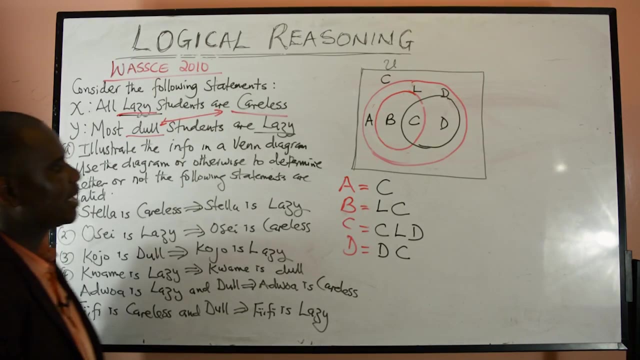 let's take the first statement. it says Stella is careless. it means Stella is inside the killer circle. now let's watch. this is therefore implies that Stella is care, is lazy. so Stella is careless implies Stella is lazy. so let's check out. now we look at for the killer circle, the killer circle and compass all the 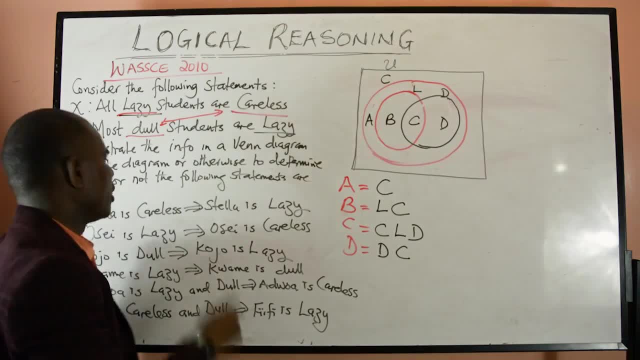 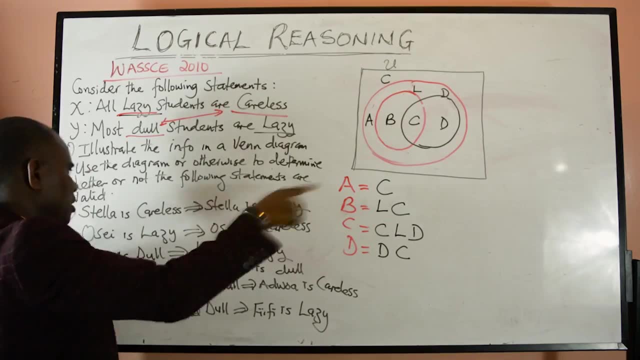 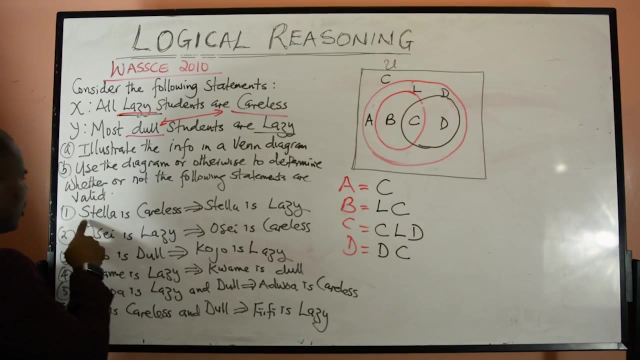 letters, meaning it is involving all the letters. so if we can enter inside the letter every room here, I will find L in all the rooms. then we can see this statement is valid. but if there is any room here that do not have L, it makes this statement invalid. so let's check out now. we have got the careless circle. 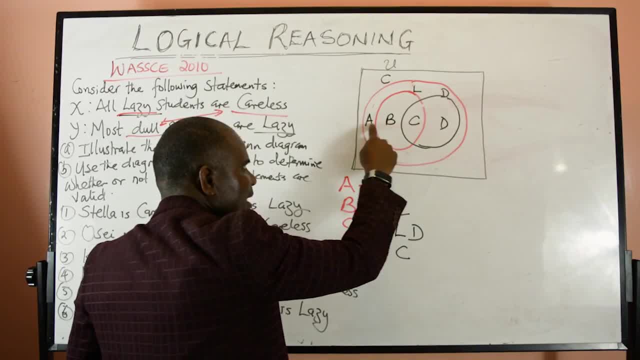 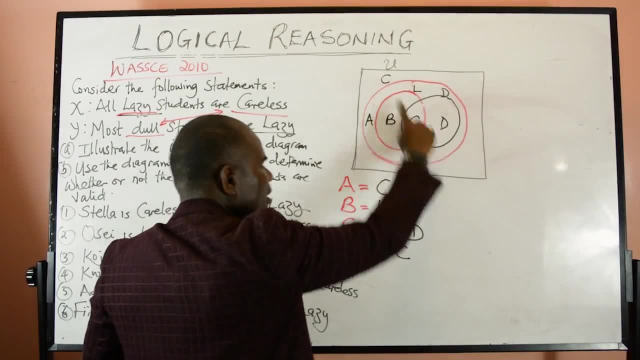 and the careless circle involves all the letters, because all the letters are inside a secure circle. a is a killer circle, B is a killer circle, C is a killer circle, D is a killer circle. now, all the letters, all the rooms are embedded inside a killer circle. now you cannot just jump up and down. 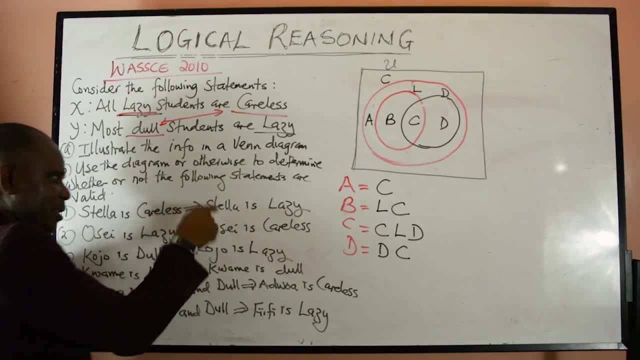 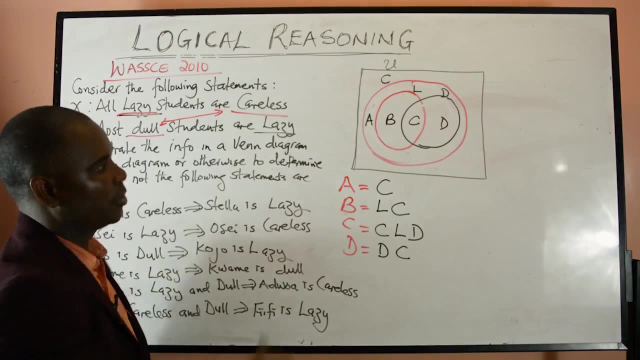 inside the killer circle now you cannot just jump up and down now see, therefore, Stella is lazy. it means that you can be inside the killer circle or you cannot be inside. the lazy circle is possible, here it is. let's look at the lazy circle. that is, the lazy circle is here. so now this guy said all: 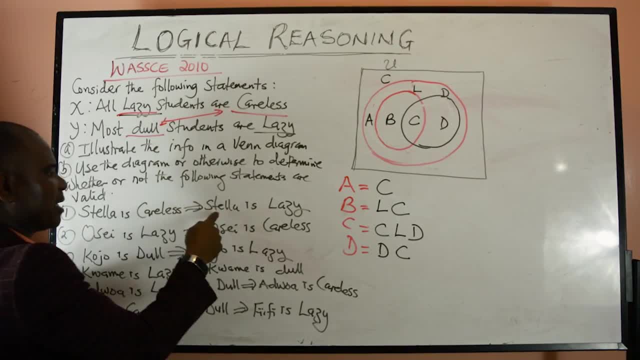 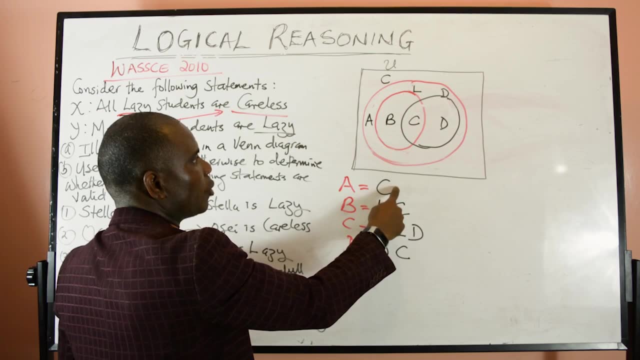 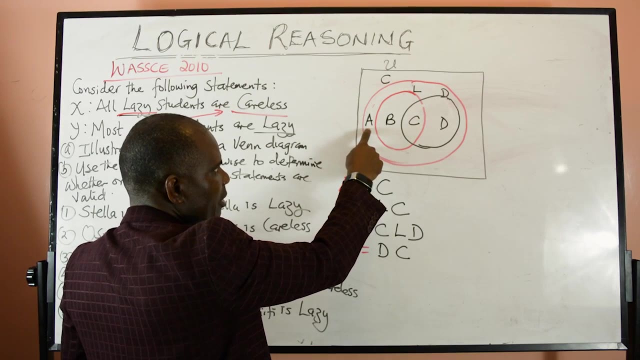 the Stella. Stella is careless implies that Stella is lazy. so if we check the killer circle, there is a room which do not have L this room a do have L check it here. this part is not inside the lazy circle, is out of the lazy circle, so you cannot see. this is valid because Stella is. 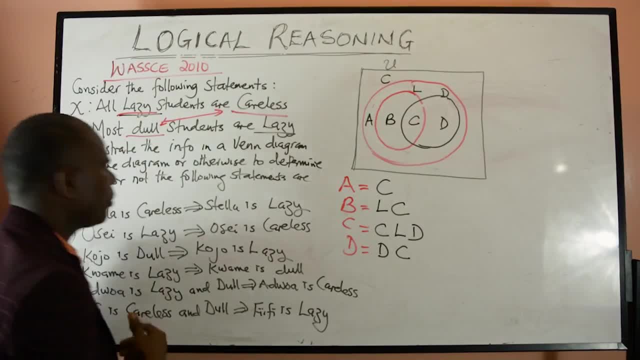 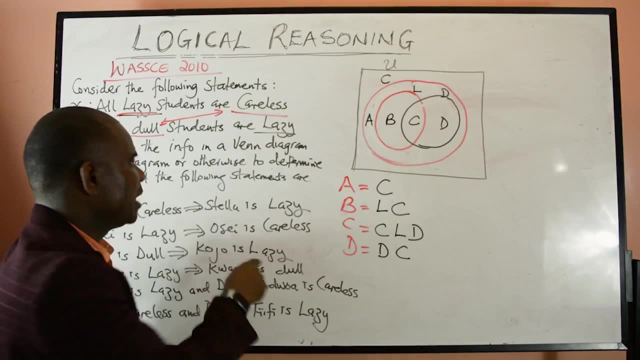 all the rooms are embedded inside the careless circle. now you cannot just jump up and now say, therefore, stella is lazy, it means that you can be inside the careless circle, but we cannot be inside the lazy circle. it's possible. here it is. let's look at the lazy. 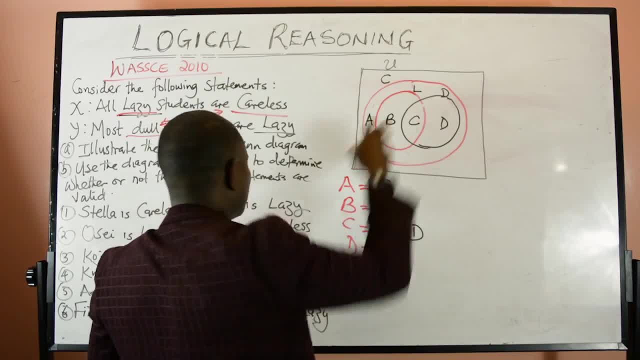 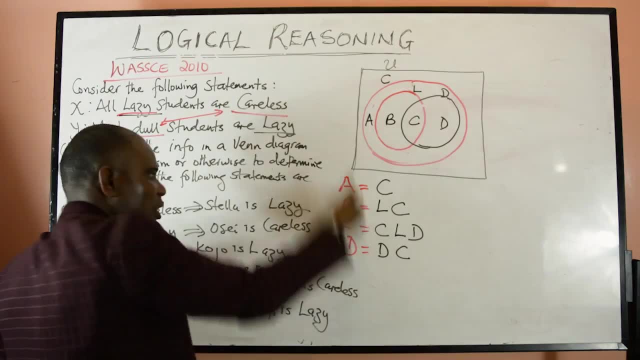 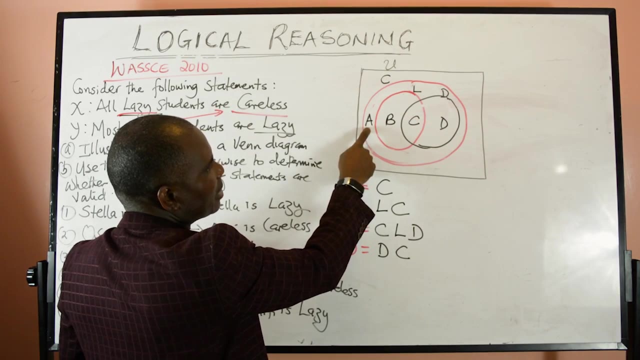 circle, that is, the lazy circle, is here. so now this guy said: all the stella. stella is careless implies that stella is lazy. so if we check the careless circle, there is a room which do not have l this room a do have l check it here. this part is not inside the lazy circle, it's out of the lazy. 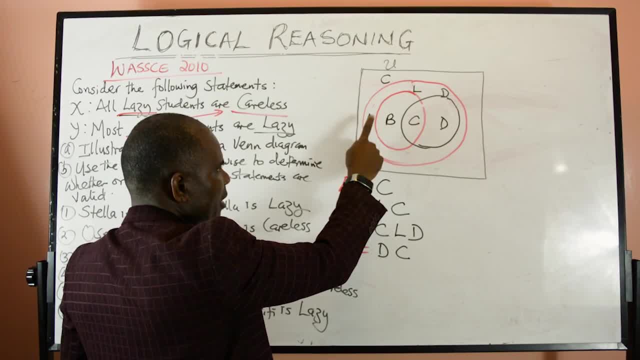 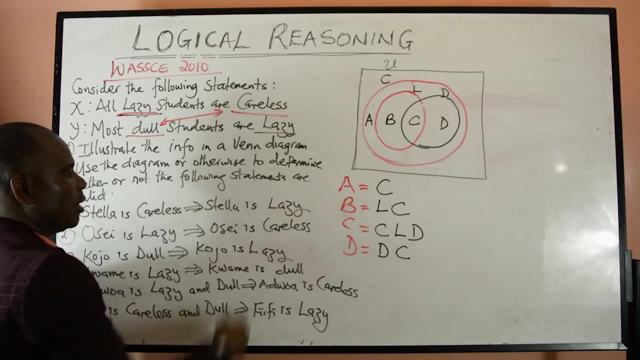 circle. so you cannot say this is valid because, stella, it's possible that seller will be in this room, and when seller is in this room, seller is not considered as a lazy person. so this assertion is going to be an invalid assertion. it's not even that even here d the room d, room d is inside the 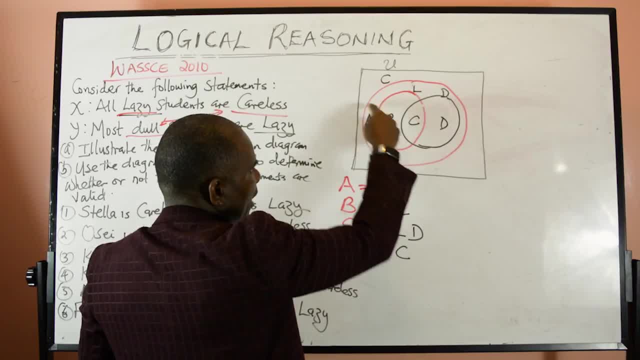 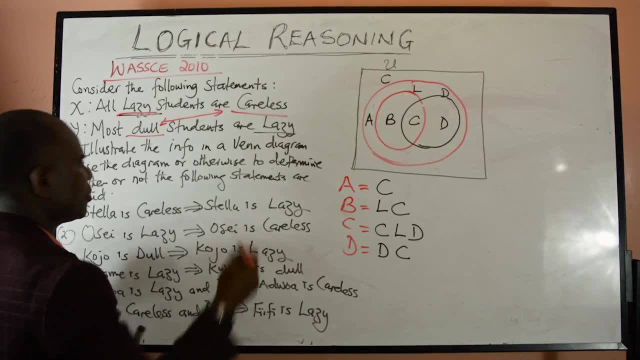 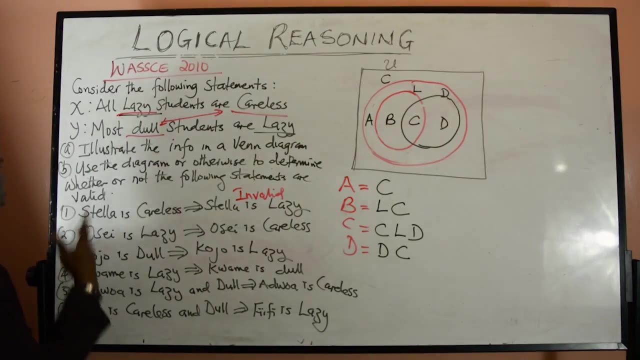 careless circle, but it's not inside the lazy circle. this is how to stop there. so room d is inside careless circle, but not inside the lazy circle. so it makes this assertion invalid. so this one is invalid. so we have an invalid assertion here. the conclusion here is invalid, so let's go to number. 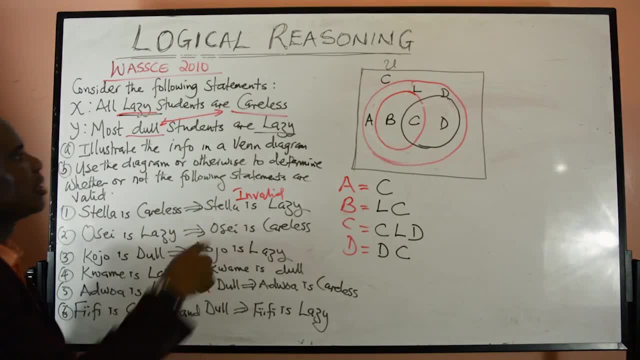 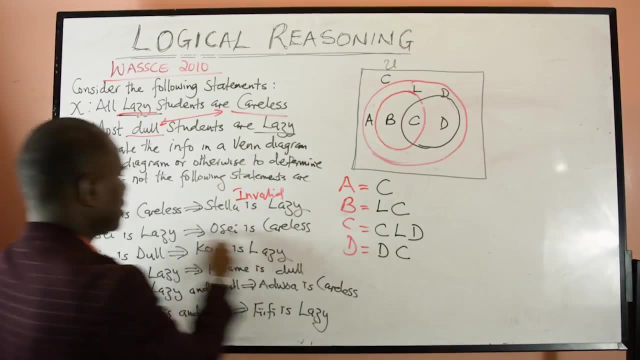 two is osai is lazy implies outside a scaless. is osai lazy lazy is b and c. you have b and c, so inside the b and c we look at for this c. inside the b and c, osai is lazy lazy contains b and c. 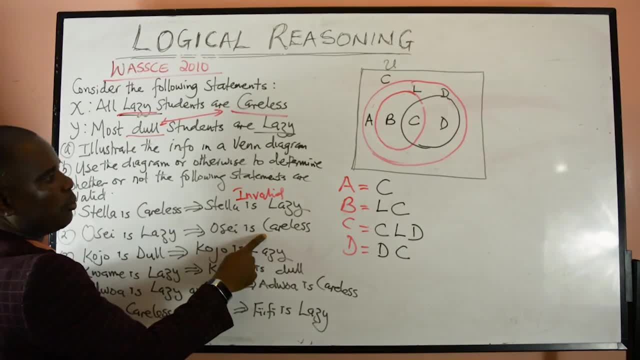 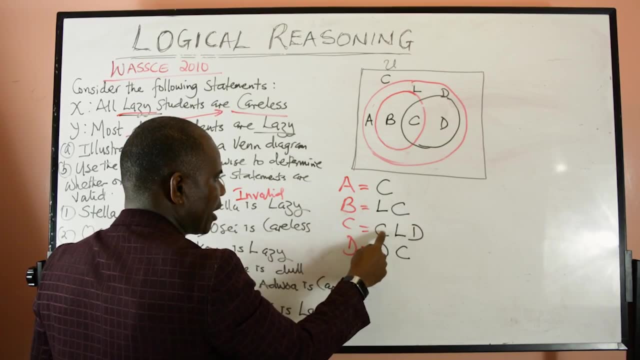 on b and c. so now, inside room b and c. if i have c in both of them, it makes it valid. that's correct. let's see here. let's see here, so osai can be inside here or here. so each other, any room you enter here, you are going to be considered a careless person because room. 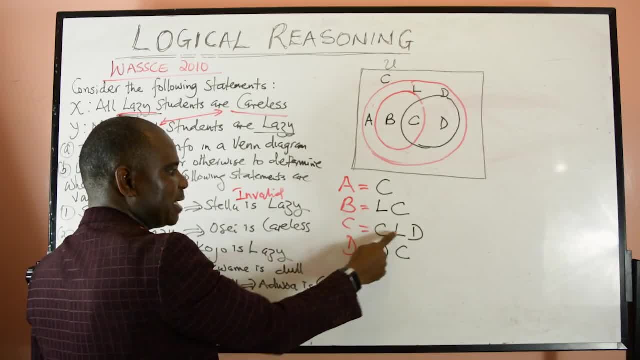 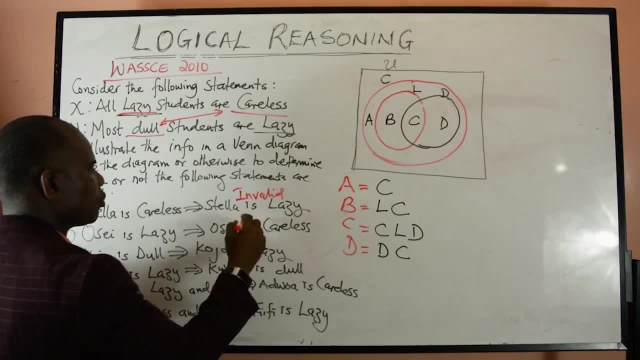 b has lazy and careless people, and europe c has careless and lazy people as well. so each any of the rooms you enter, osai enters, osai is going to be you consider as a careless person, so it makes this one valid. this is a valid assertion, so we call it valid arguments. this is valid in that case. 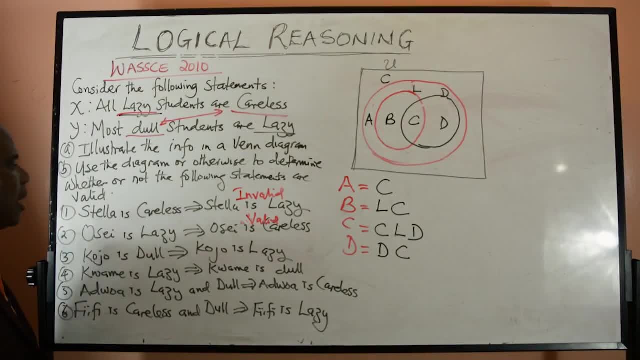 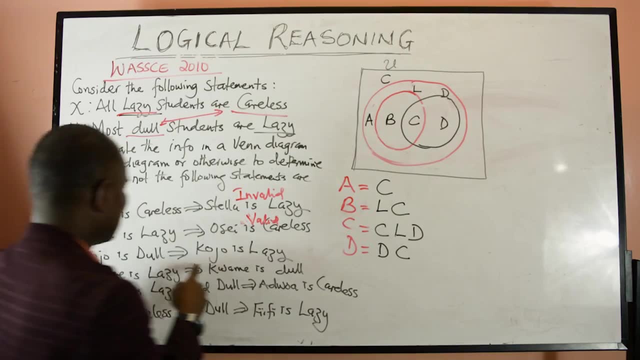 so we go to kojo. kojo is doll implies kojo is lazy, so we'll go to the doll circle. inside the doll circle we have c and d only, so we consider c and d. if i look at the c and d and find out that 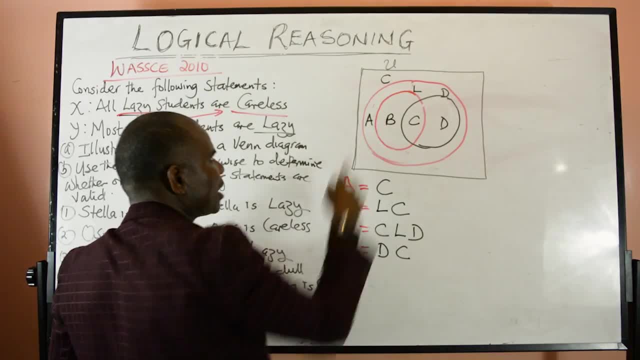 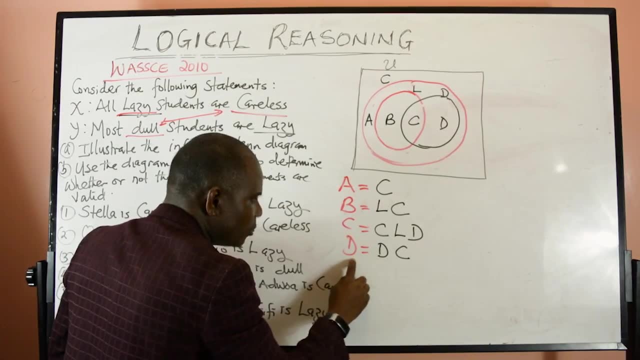 possible that Stella will be in this room and where Stella is, this room. Stella is not considered as a lazy person, so this assertion is going to be an invalid. assertion is not even that. even here D they do. D room D is inside the killer circle, but it's not inside a lazy circle. this is how to stop there, so 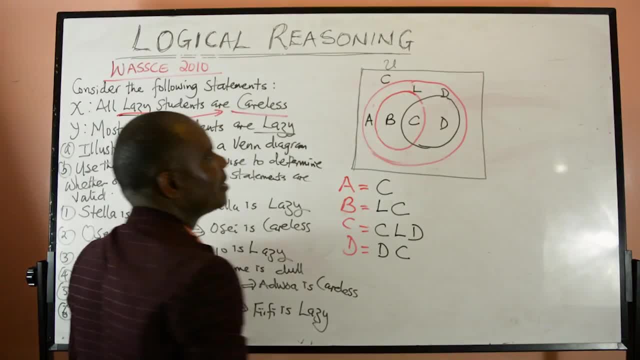 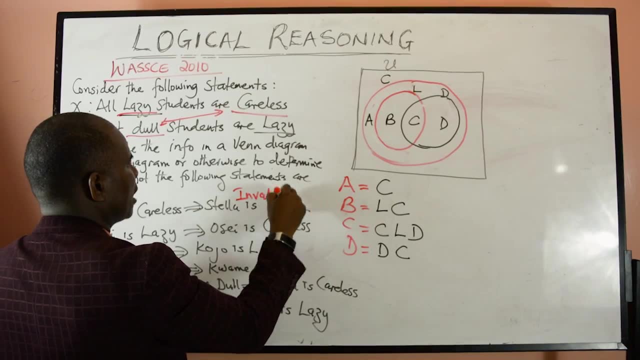 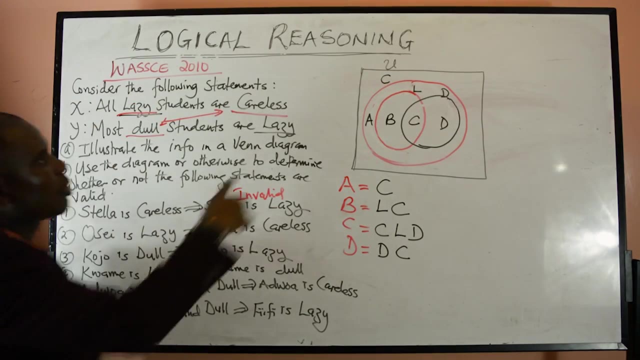 room D is inside killer circle but not inside the lazy circle, so it makes this assertion invalid. so this one is invalid. so this one is invalid. so this one is invalid. so we have an invalid assertion here. the conclusion here is invalid, so let's go to number two. is outside, is lazy in place outside, is careless, is outside. 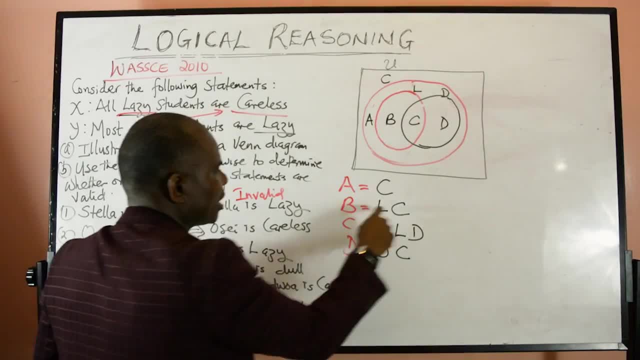 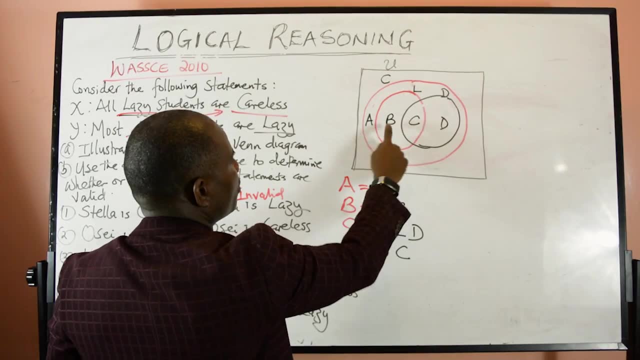 lazy lazy is B and C. you have B and C. so he said a, B and C. we look at for this. C inside the B and C or side is lazy lazy contains me and see you on B and C. so now is I will be and see if I have C in both of them. it makes it valid, that's. 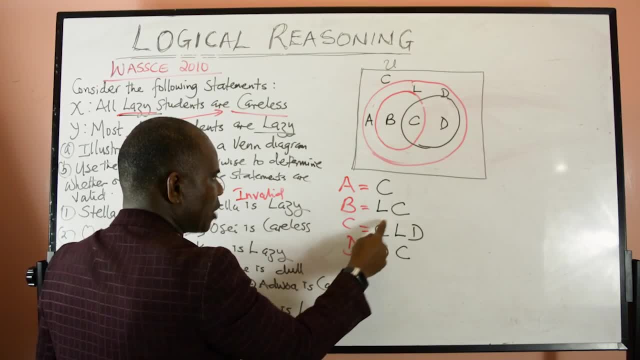 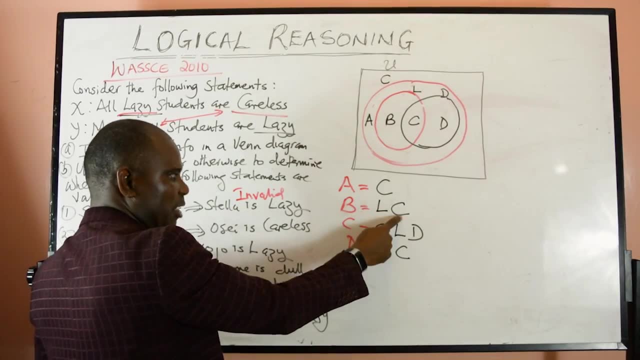 correct, they see here, they see here. so, aside, it can be inside here or here. so each other, any room you enter here, the is are going to be considered a careless person, because room B has lazy and careless people and you see, has careless and lazy people as well. so each, any of the rooms you enter outside and task. 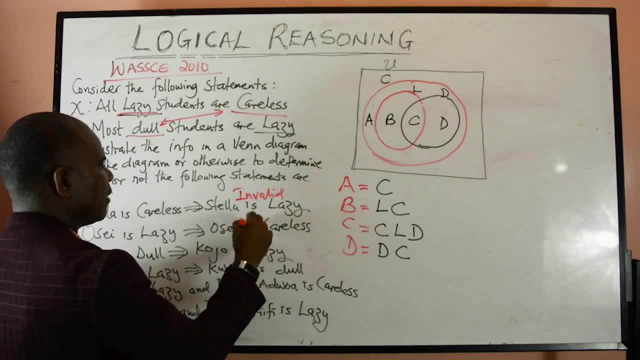 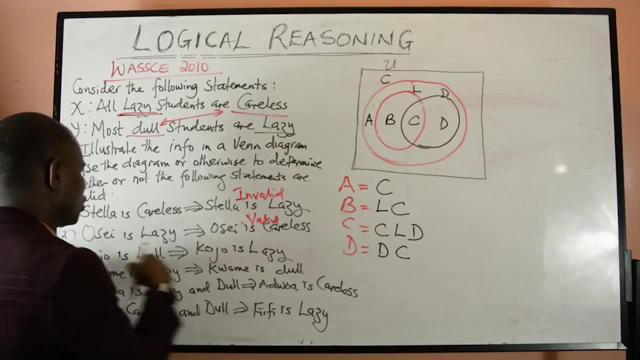 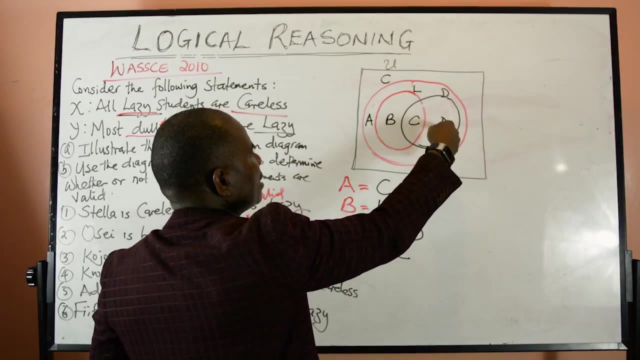 outside is going to be you considered as a careless person, so it makes this one valley. this is a valid assertion, so we call it valid arguments. this is valid in that case, so we go to: could you? could you install in place? could you install in place with your Rabbit ID? and any one of these signs of is lazy. so 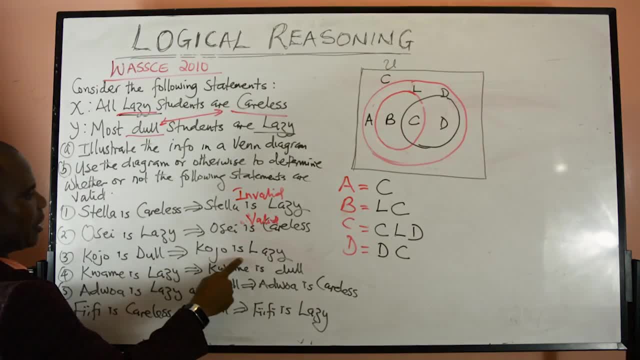 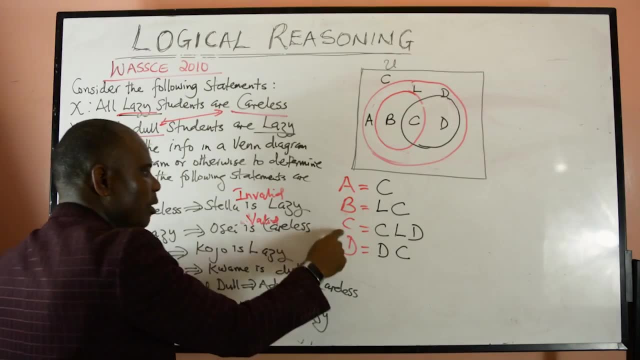 we'll go to. the dorsacle is a dorsacle. we have C and D only, so we consider C and D. if I look at the C and D and find out that boots I have lazy in boot C and D, then I can conclude that the statement is valid. but if there is a room between 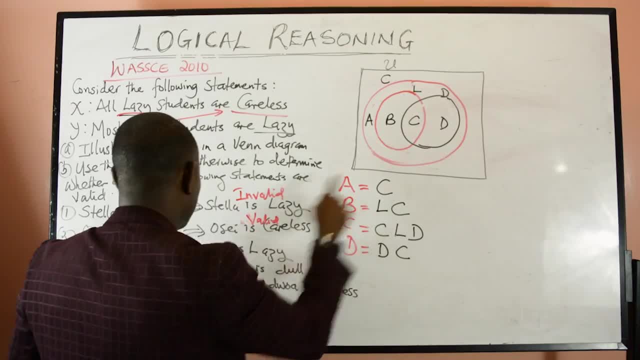 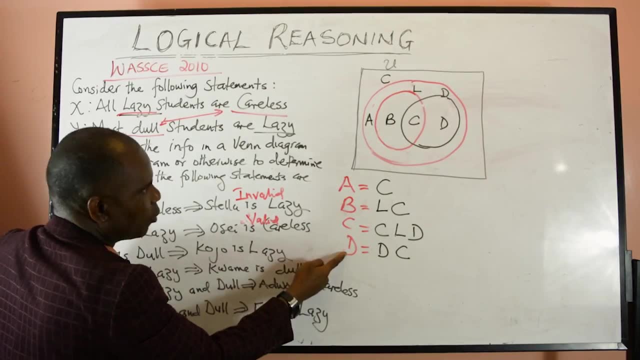 C and E. there is one of them that do not have L. it makes the whole statement invalid that that's what happened here. C and D are the one that are inside a daughter co the door fan to Isis and it said adult. we have C and D and inside our room, see, and the 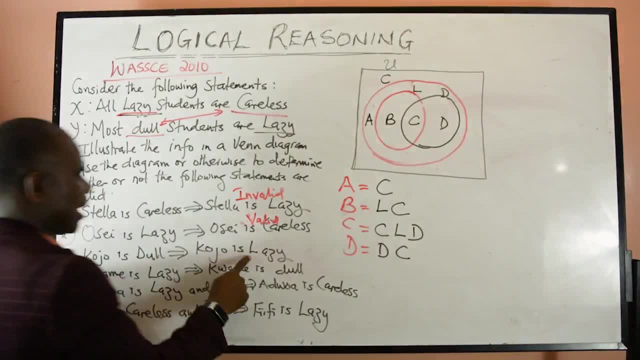 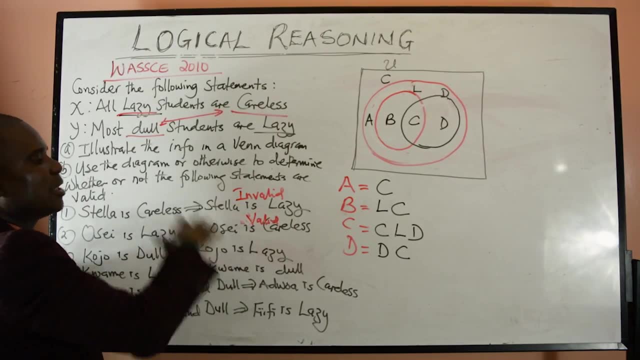 both. i have lazy in both c and d, then i can conclude that the statement is valid. but if there is a room between c and d, there is one of them that do not have l. it makes the whole statement invalid, and that's what happened here. c and d are the one that are inside the doll circle. 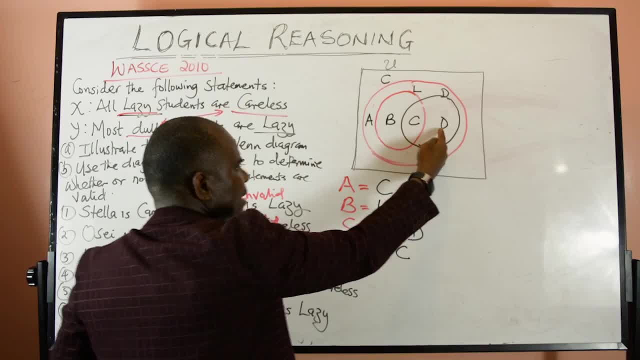 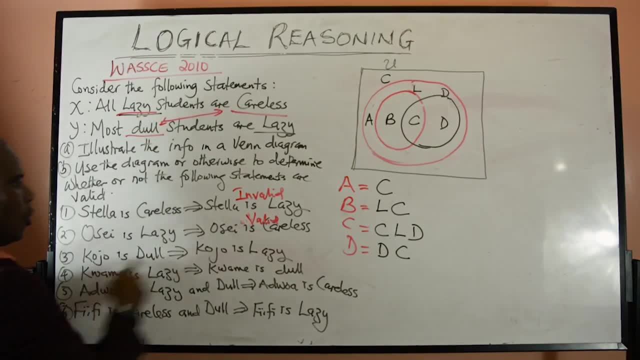 the doll circle is this, and inside the doll circle we have c and d, and inside that room- c and d- we don't have all lazy people in there. it is possible that the kojo was inside this room, and inside this room we don't have lazy people, so it means that that. 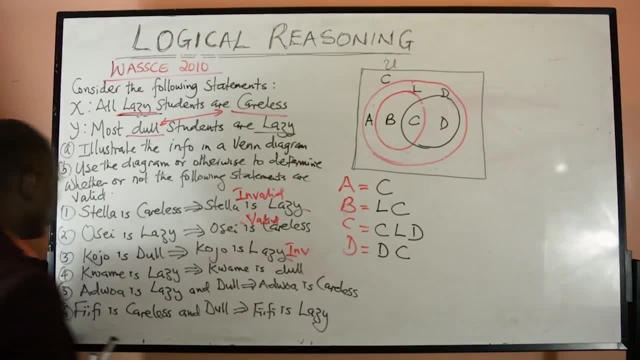 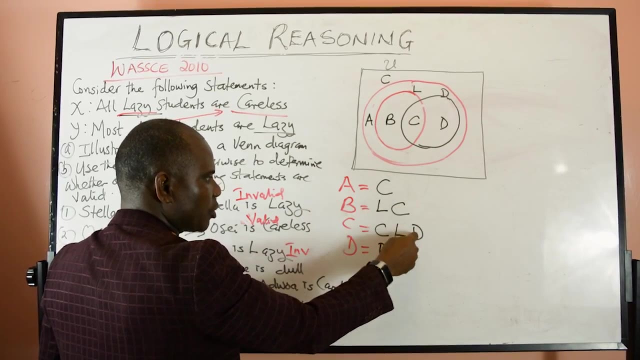 statement is invalid. so that is invalid as well. so look at kwame. kwame is lazy. if kwame is lazy, we look at the lazy circle: it's t, b and z implies that kwame is doll. so let's look at b and c. we don't have d inside here. b and c do not have d all through. if d was here, d was here, there will be a, d. 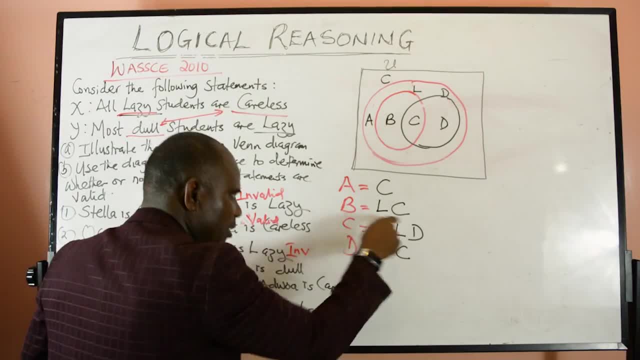 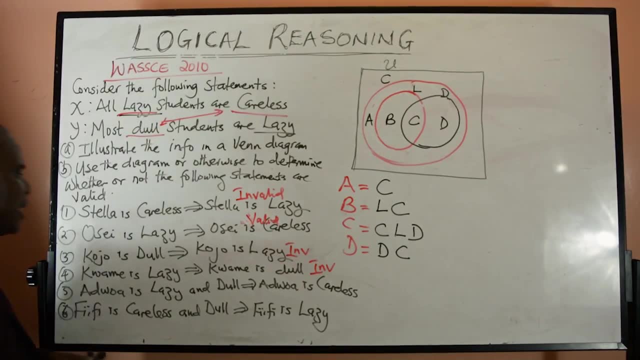 off like that, so we can assert that the statement is valid, because there is a room here that do not contain c, d, the. we can assert that this guy is invalid, so this statement is also invalid. you see, kwame is lazy implies kwame is daughter is invalid. let's look at hardware. hardware is lazy and door. 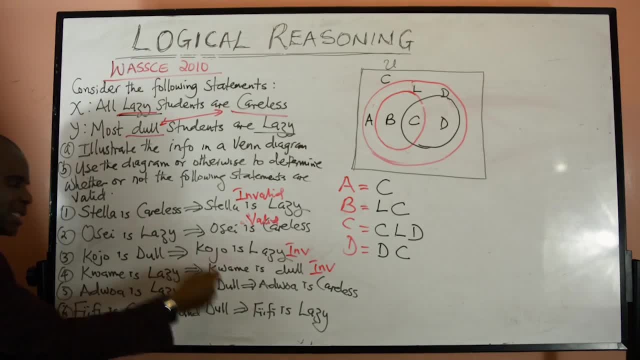 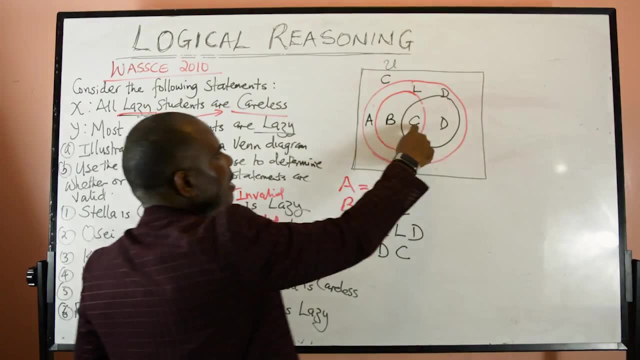 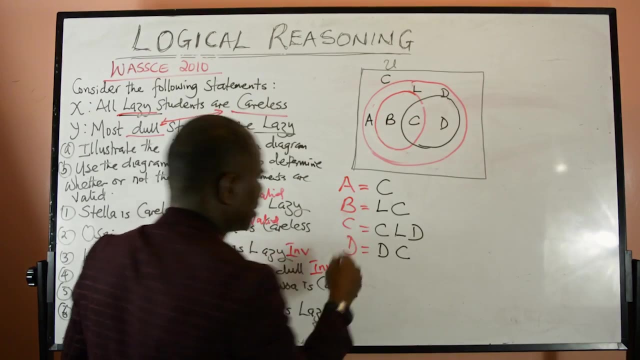 this is intersection. so look at, we are intersection of lizzie and through door. we are door and intersection circle where doll and lizzie sacco intersect and they are going to intersect at c. this is where door suckle and lazy p 그 intersect here. so it's the intersect. only one letter another type see. so look. 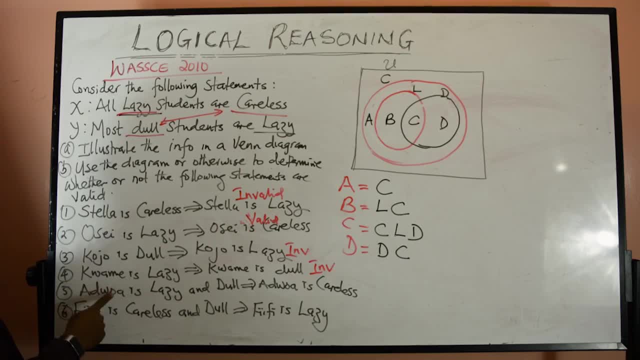 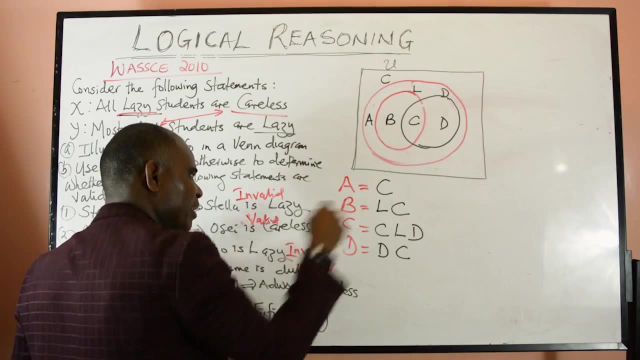 at the sea, inside the sea? no, now look at the question. it says bad what is lazy, and all implies otherwise careless. so let's look at see. see contains careless people. if I enter room, see, I will have a careless guy, a lazy guy and a dog guy. so 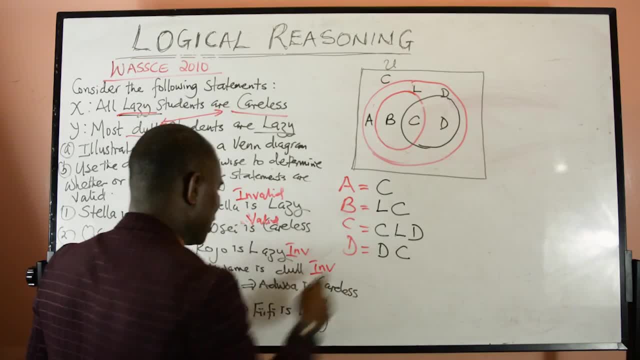 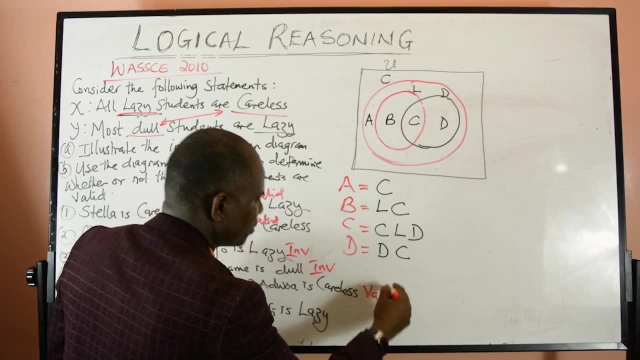 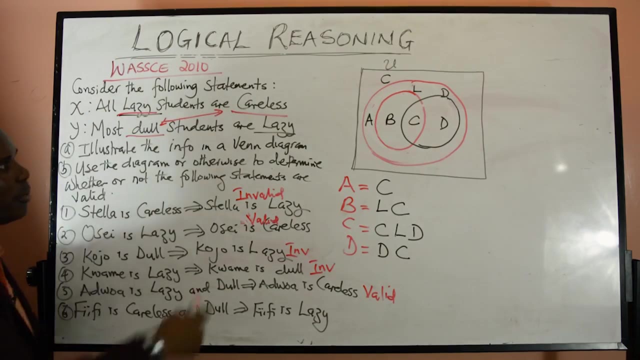 if I do, I enter the room, then it's possible that Edward is going to be considered as a careless person. so it makes it valid because there is a see inside, is rooms in serious or have valid assertion he a 50: 50 is careless and all this is also intersection between careless and all between the careless. 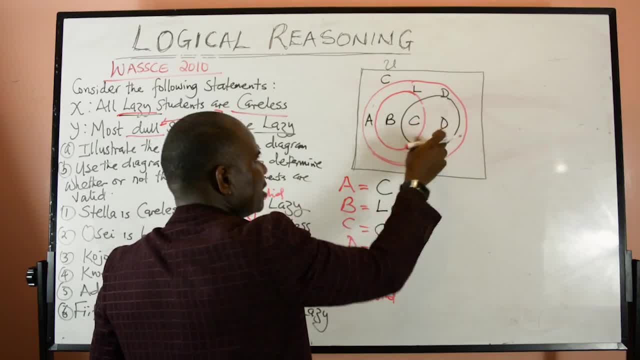 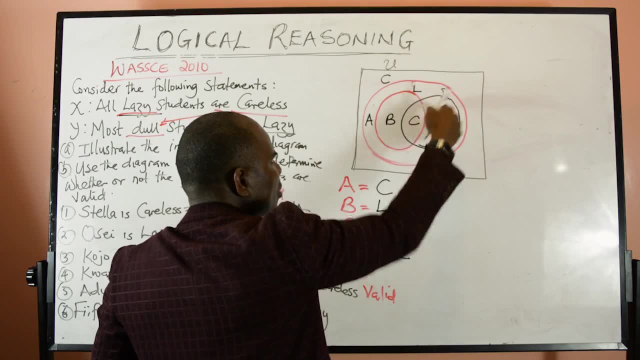 and the door Sunco. they overlap on C and D. it means the intersecting on C and D, because C and D is inside those aku is also inside the carles carco, so careless, and all are encompassing two of these letters, which is C and D. so let's check. 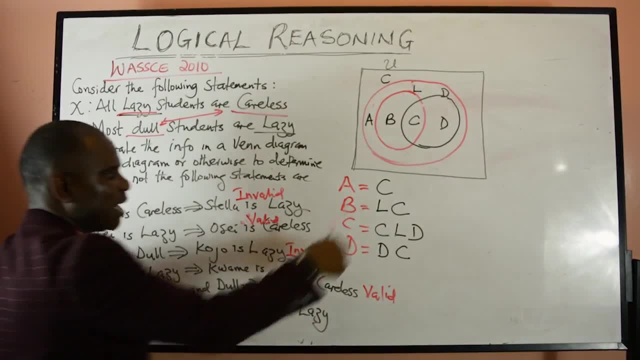 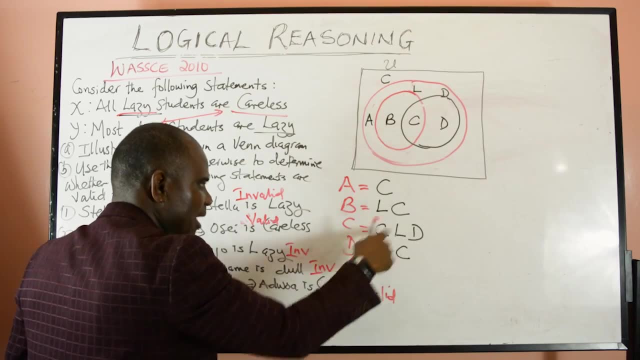 them out. see, and the question says Lizzy. if C and D contains lazy, then we make the key statement valid. but if there is a letter here that do not between c and d, there is a letter, a room that do not have l, that makes it invalid. and here is c and d, but here do not have l, so it 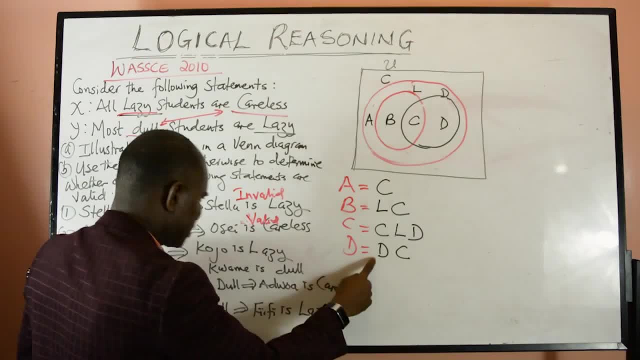 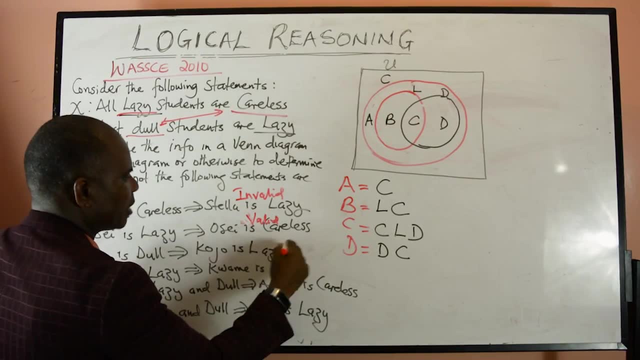 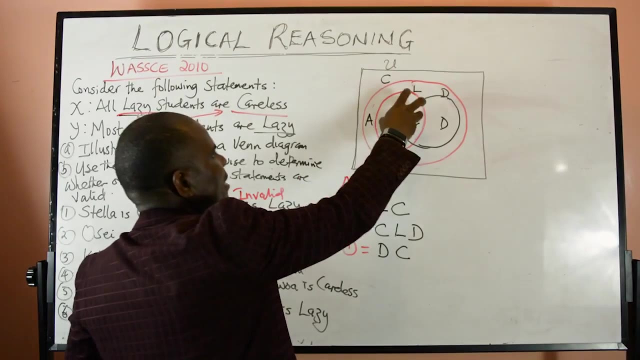 don't have all lazy people in there. it is possible that the kujo was inside this room, and inside this room we don't have lazy people, so it means that that statement is invalid. so that is invalid as well. so look at kwame. kwame is lazy. if kwame is lazy, we look at the lazy circle: it's t, b and t. 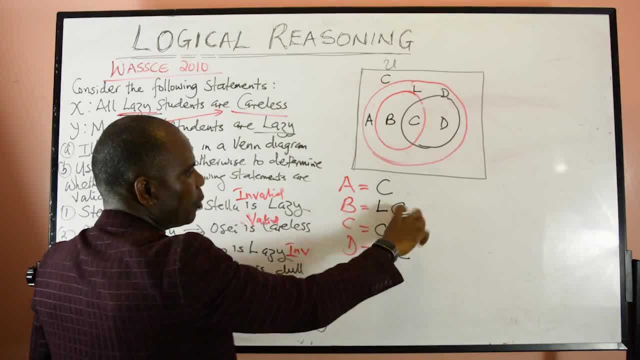 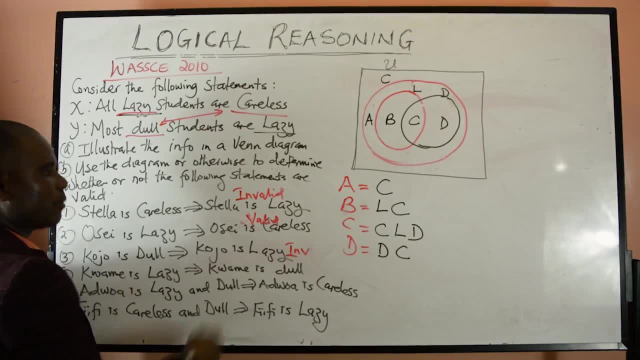 implies that kwame is door. so let's look at b and c. we don't have d inside here. b and c do not have d all through. if d was here, d was here, then we can assert that the statement is valuable, because there is a room here that do not contains a, d, then we can assert that this guy is invalid. so 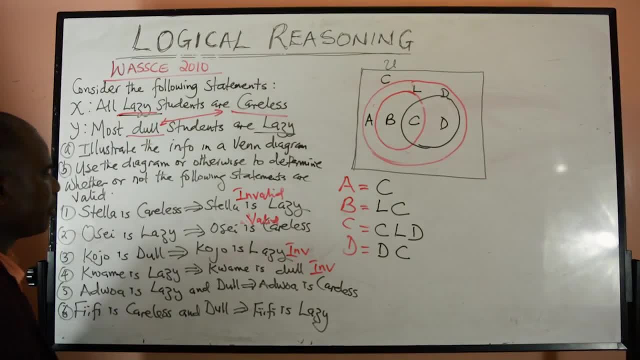 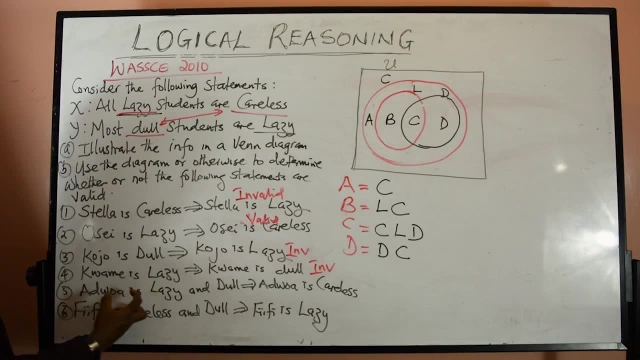 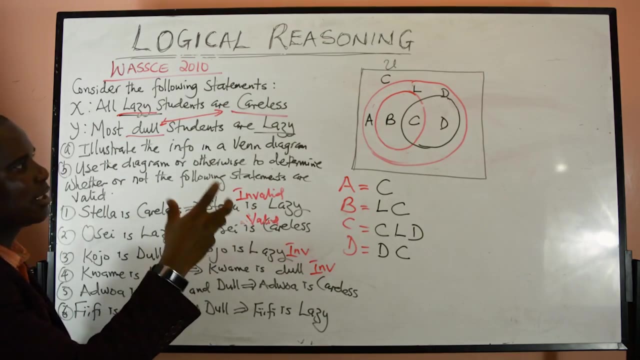 this statement is also invalid. you see, kwame is lazy implies kwame is door is invalid. let's look at hardware. hardware is lazy and door. this is intersection. so look at where intersection of lazy and door we are door and intersection circle inter, where doll and lazy circle intersects and. 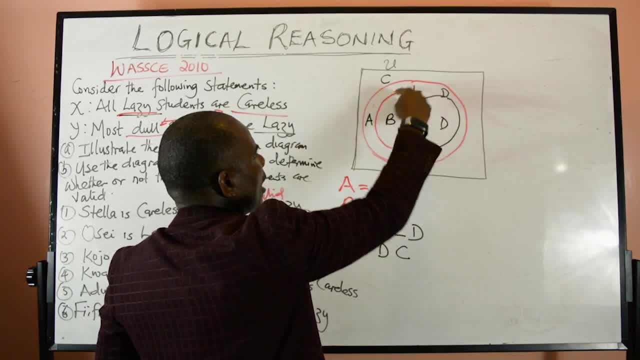 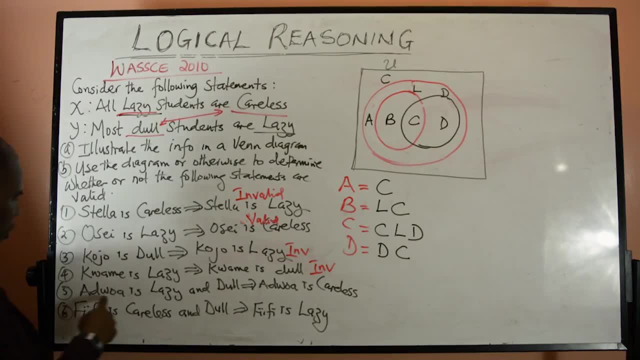 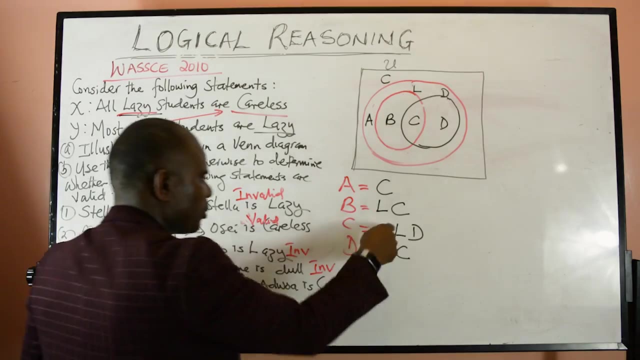 they are going to intersect at c. this is where door circle and lazy circle they intersect here. so they intersect on only one letter. now. letter is c. so look at the c inside the c now. now look at the question. it says hardware is lazy and all implies hardware is careless. so let's look at c. c contains careless people. if i enter room c, i 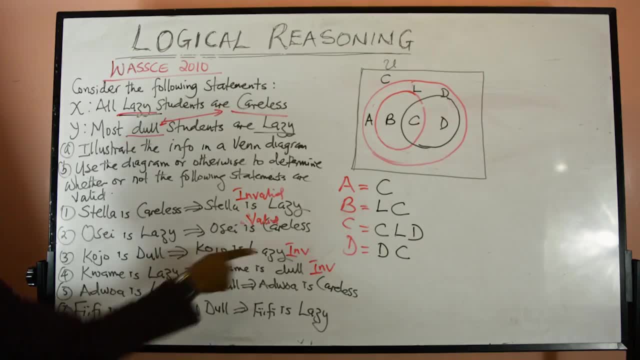 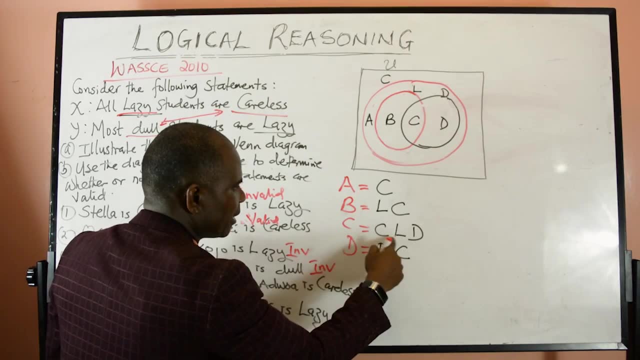 will have a careless guy, a lazy guy and a doll guy. so if hardware enter that room, then it's possible that ardua is going to be considered as a careless person. so it makes it valid because there is a c inside this room, c there. so have valid assertion here: fifi. fifi is careless and all this is also. 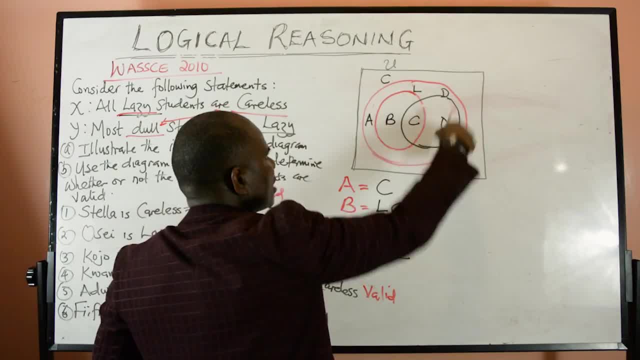 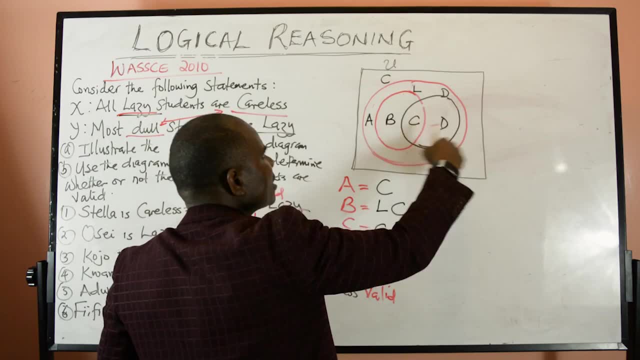 careless and all between the careless and the door circle. they overlap on c and d. it means they intersected on c and d because c and d is inside door circle is also inside the careless circle, so careless and all are encompassing two of these letters, which is c and d. so let's check. 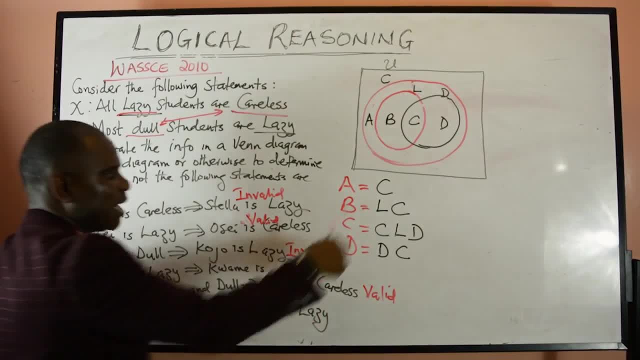 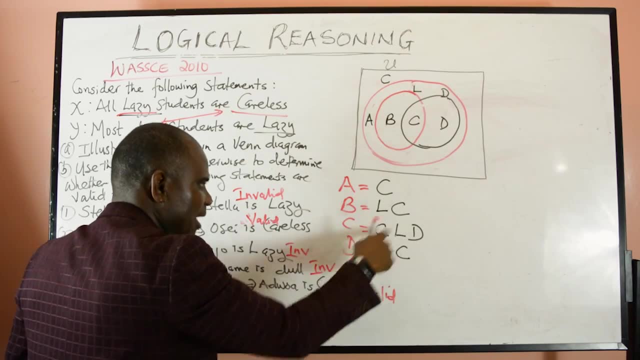 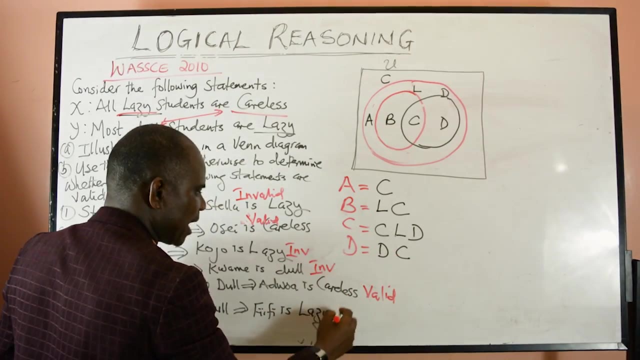 them out: c and d. now the question says lazy. if c and d contains lazy, they will make the statement valid. but if there is a letter here that do not between c and d, there is a letter, a room that do not have l, that makes it invalid. and here is c and d, but here do not have l, so it makes this guy.